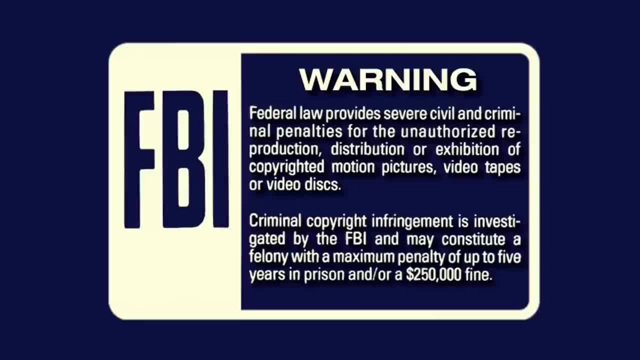 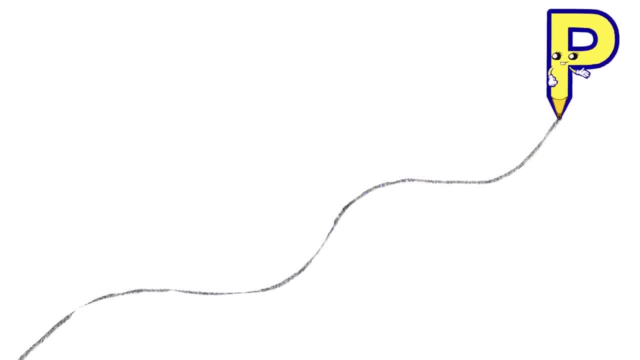 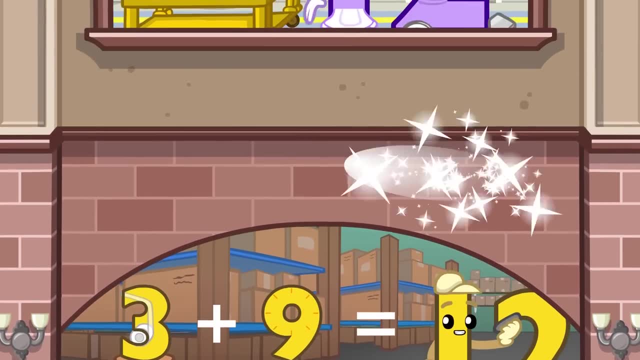 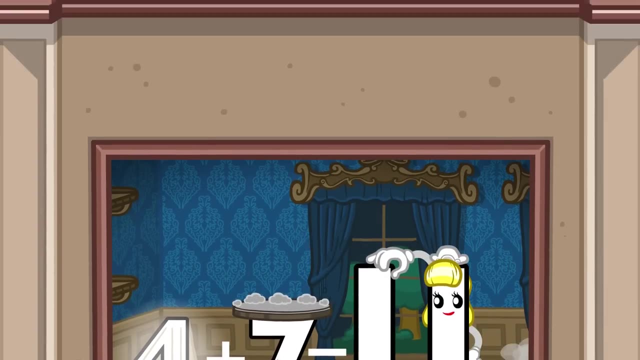 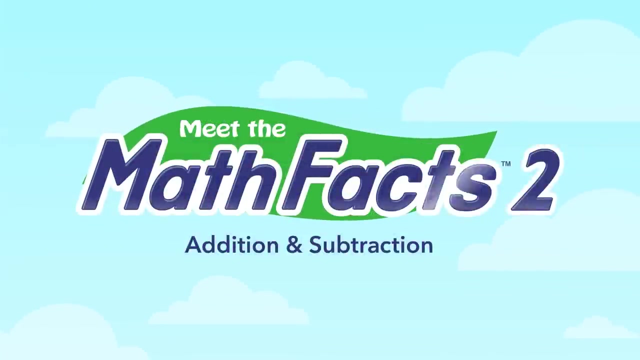 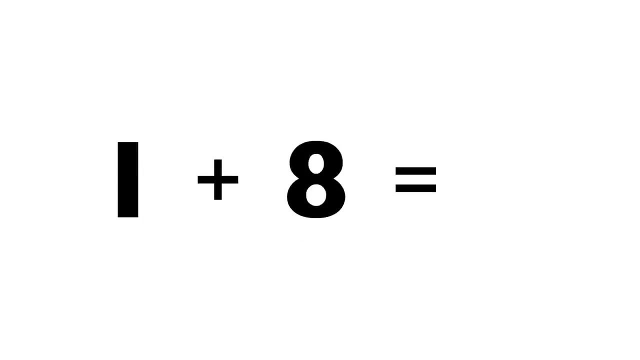 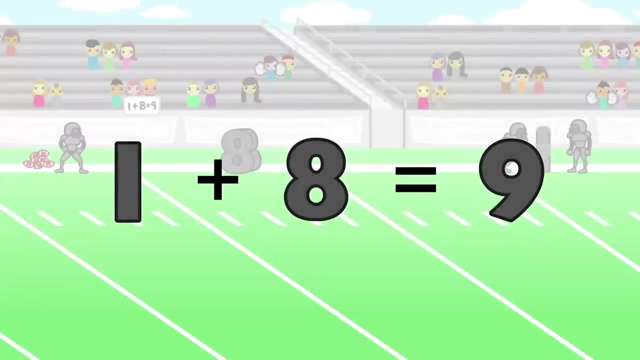 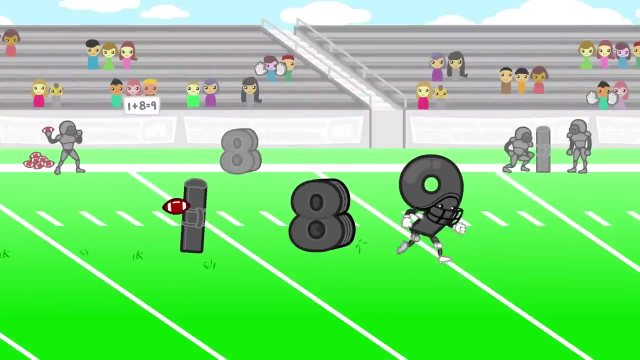 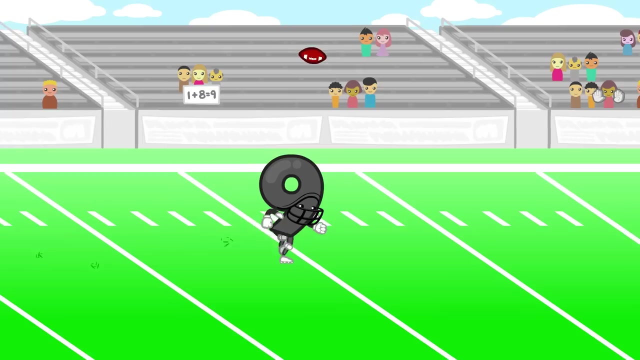 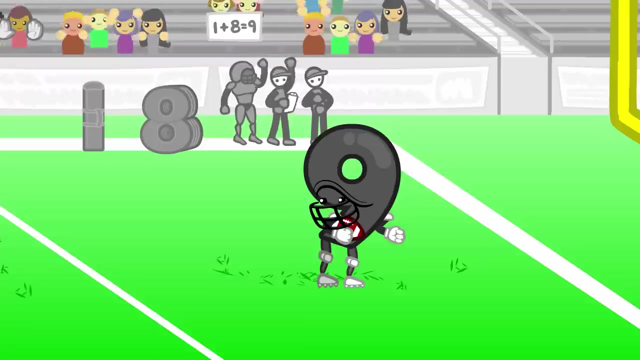 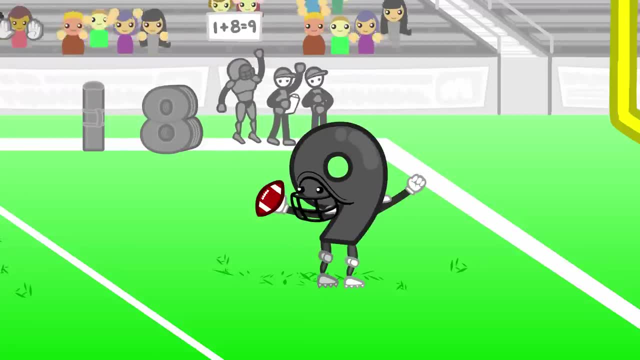 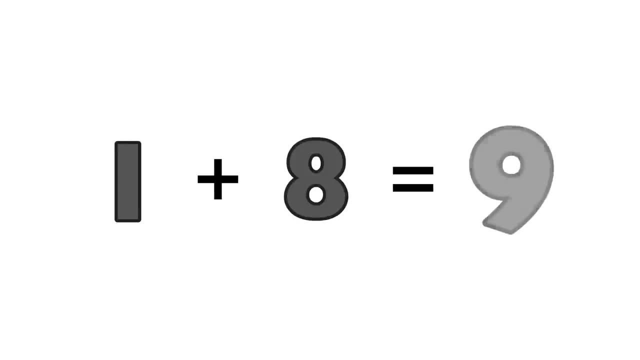 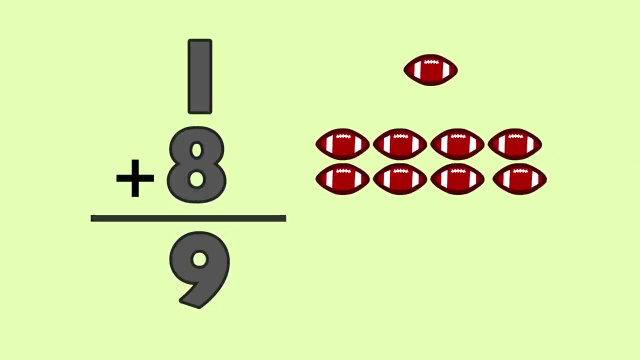 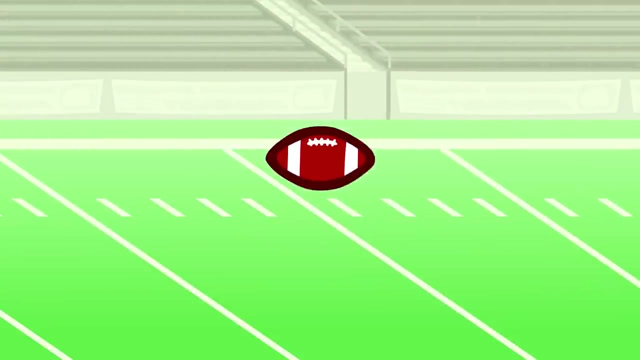 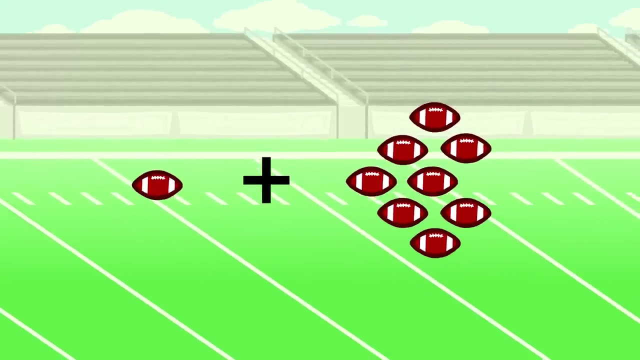 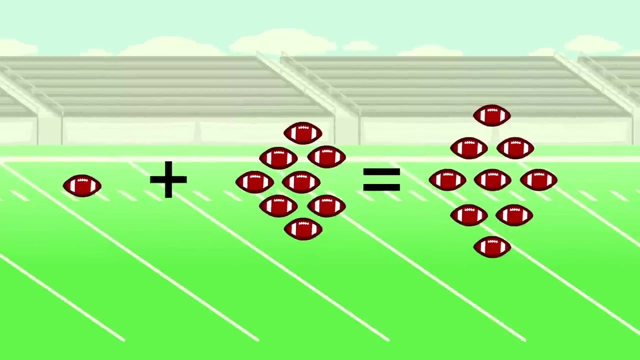 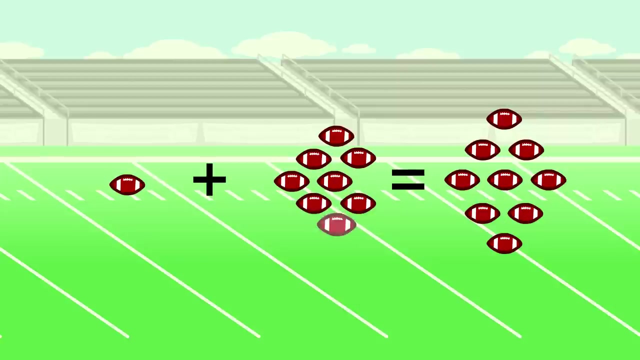 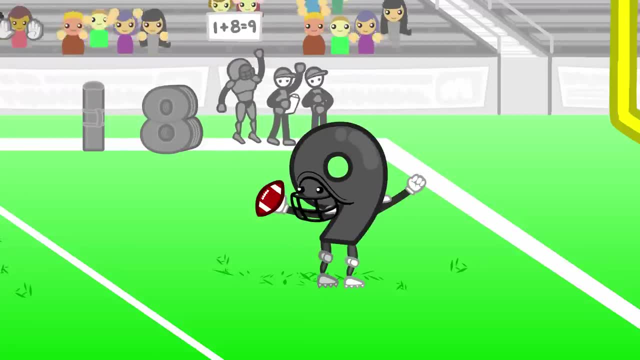 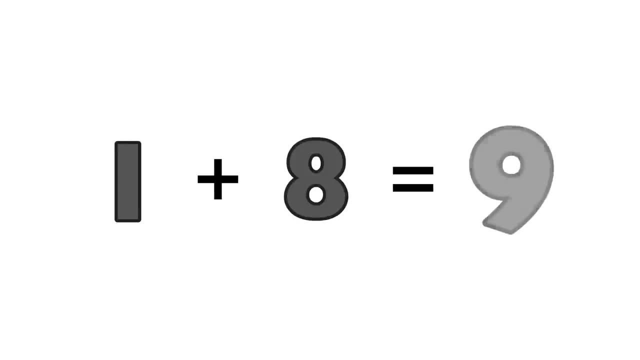 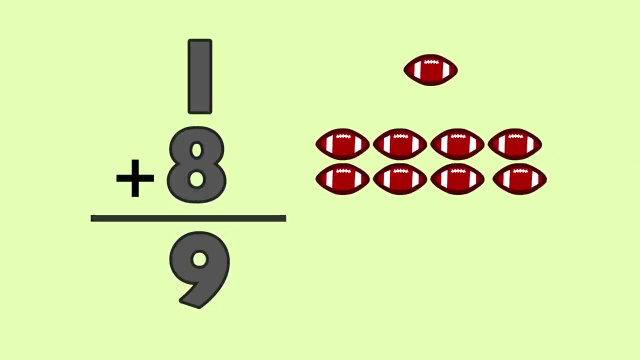 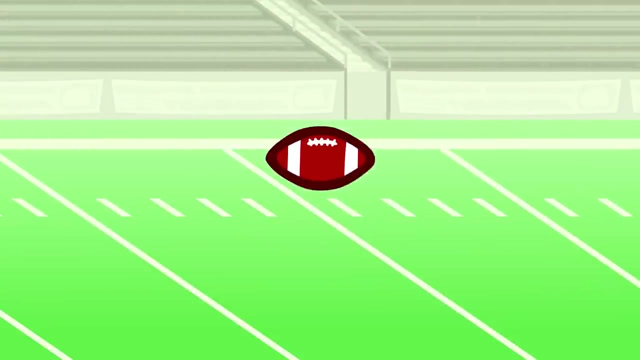 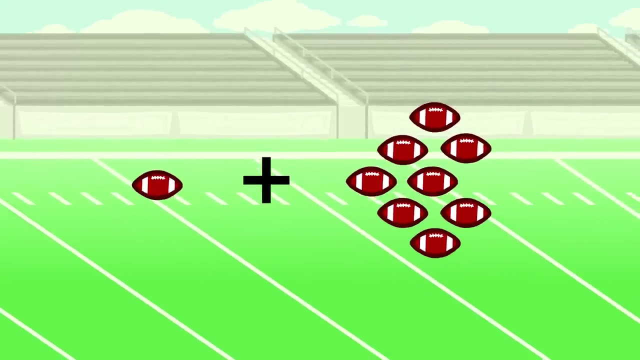 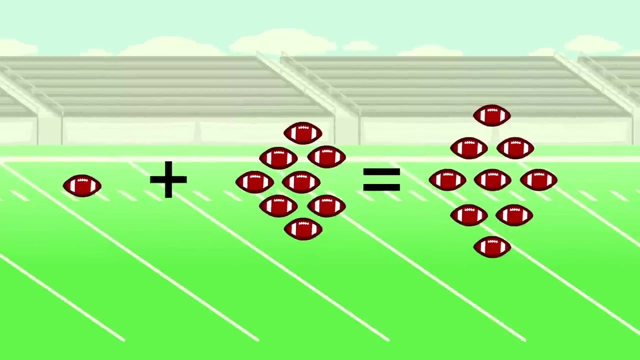 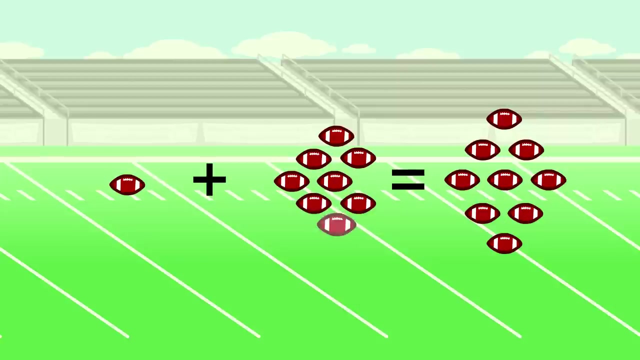 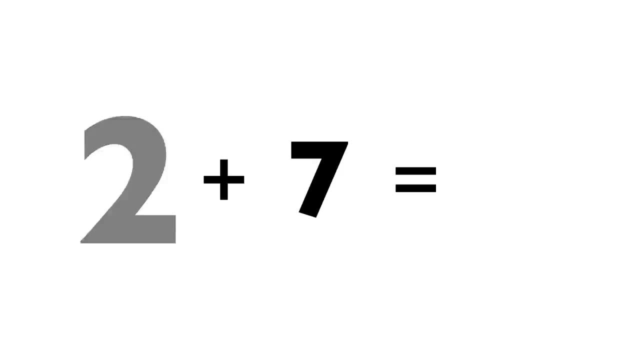 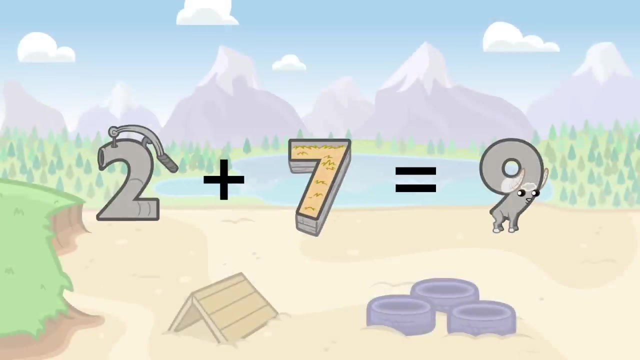 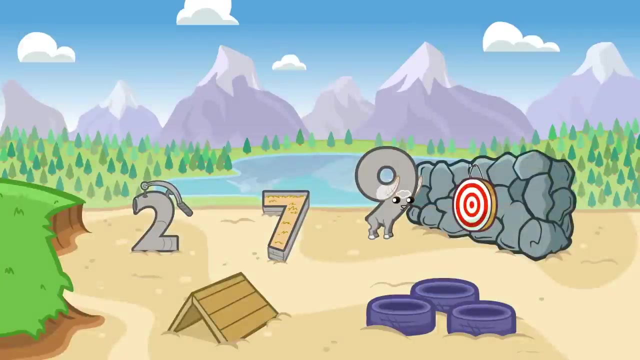 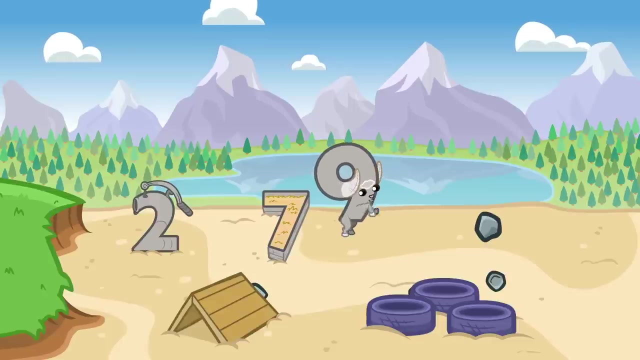 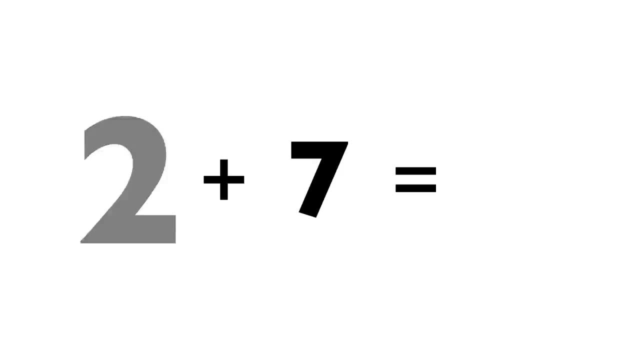 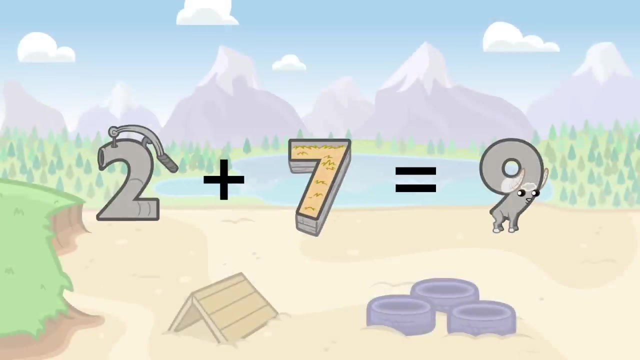 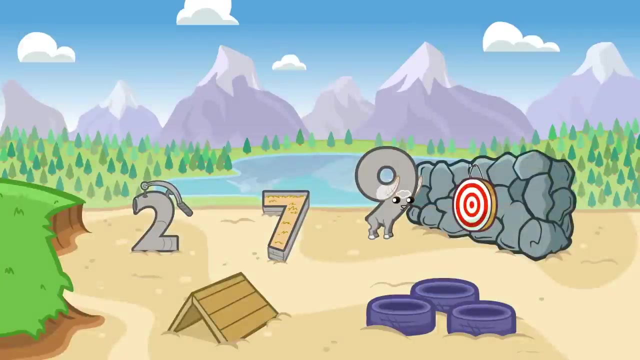 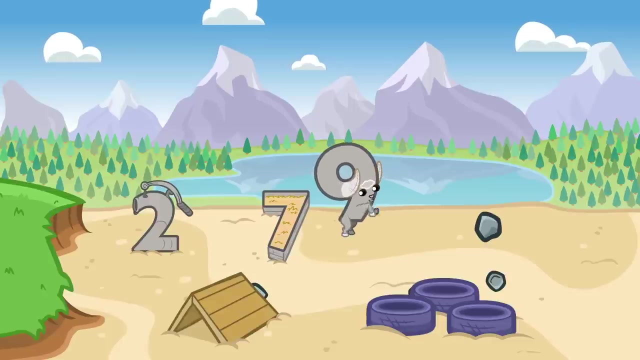 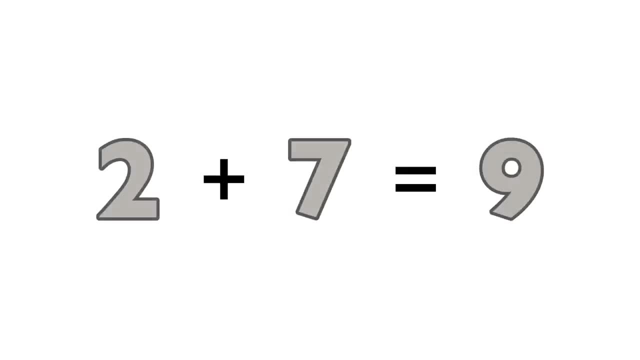 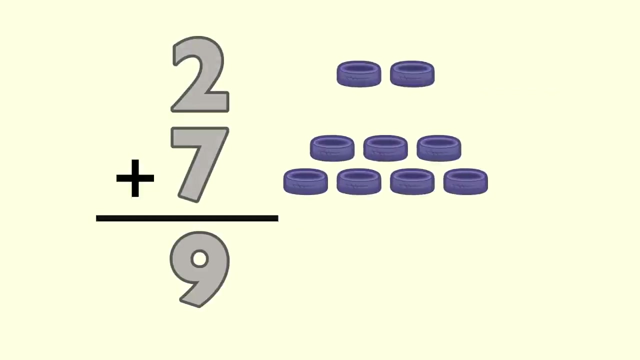 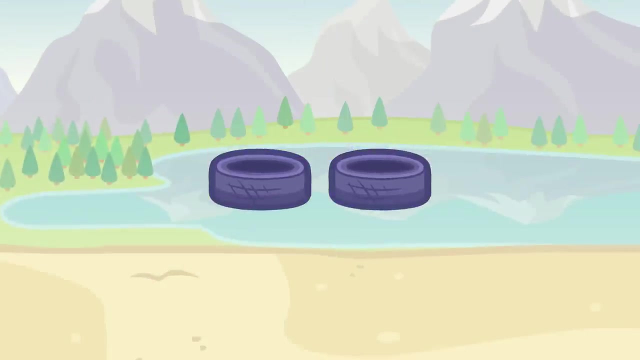 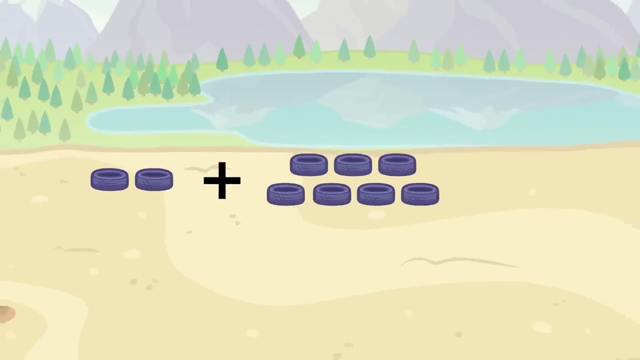 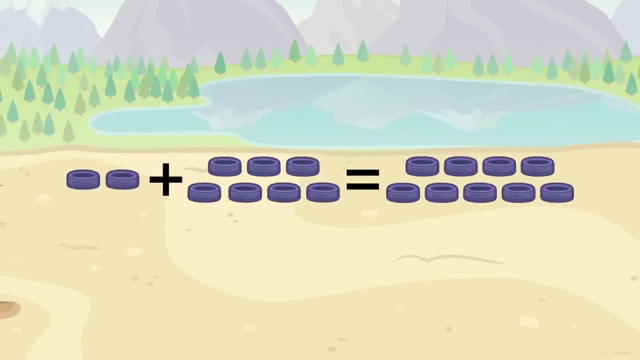 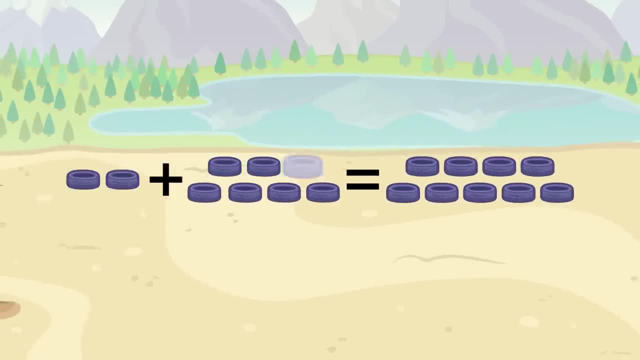 1,, 2,, 3,, 4,, 5,, 6,, 7,, 8,, 9.. 2 plus 7 equals 9.. 5,, 6,, 7,, 8,, 9, equals 1,, 2,, 3,, 4,, 5,, 6,, 7,, 8,, 9.. 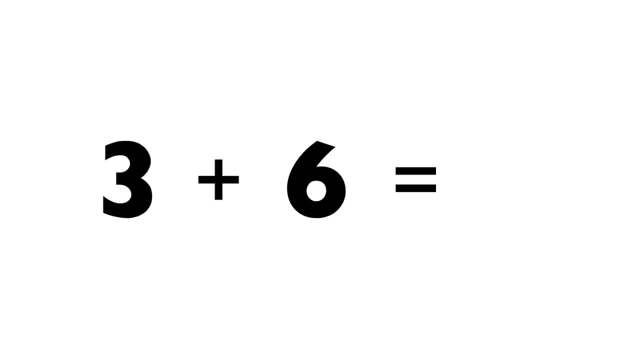 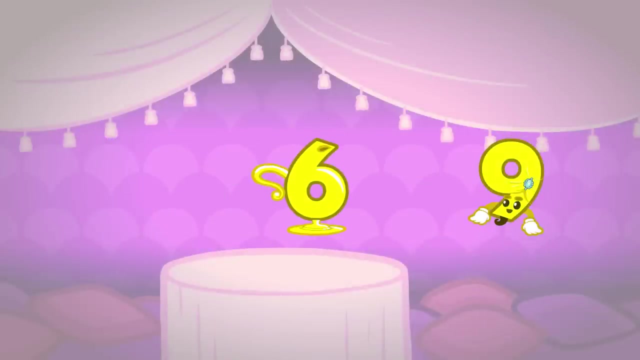 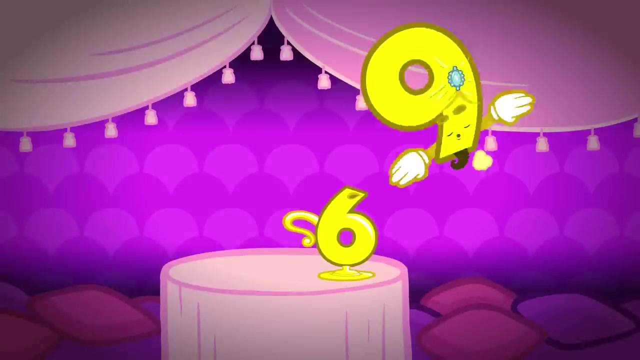 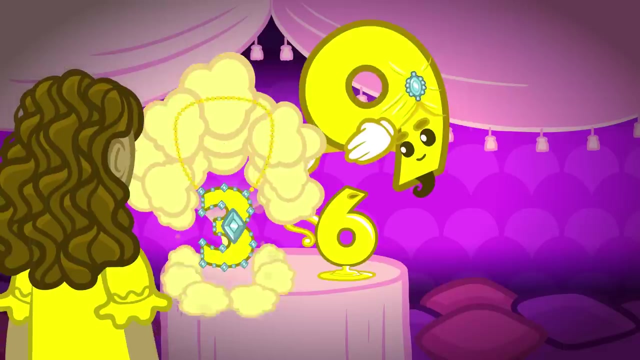 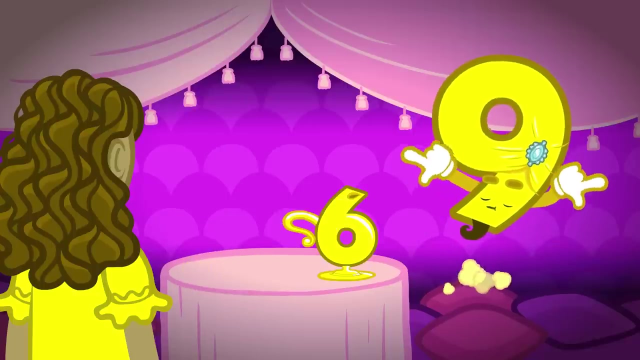 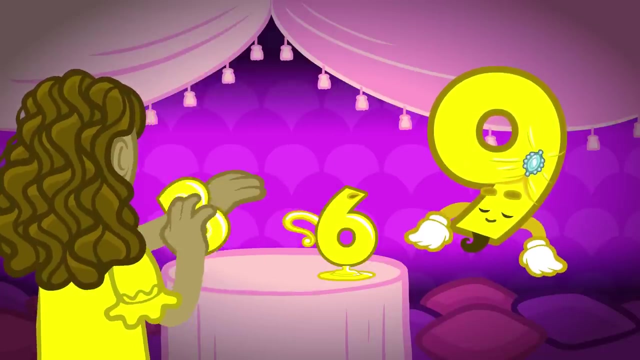 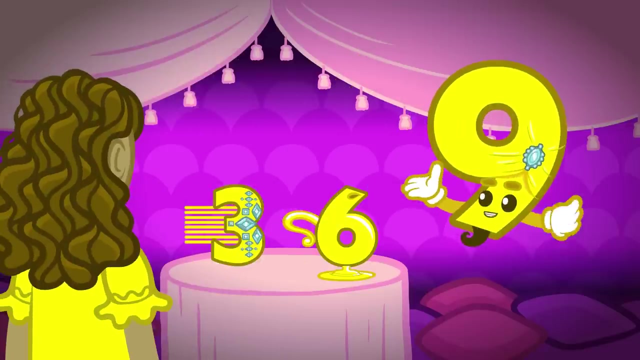 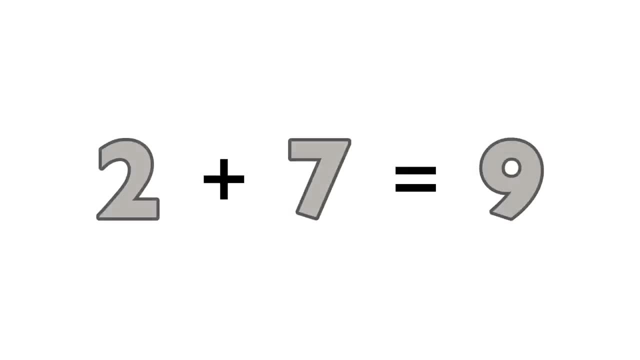 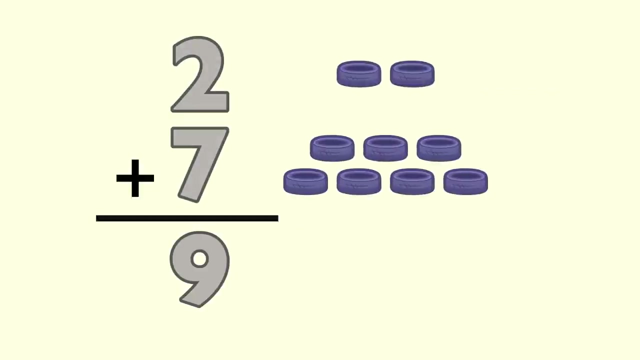 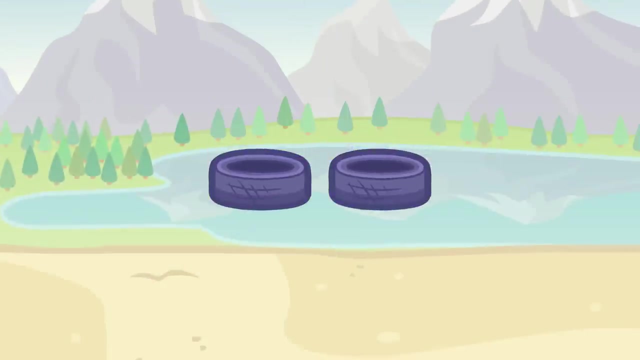 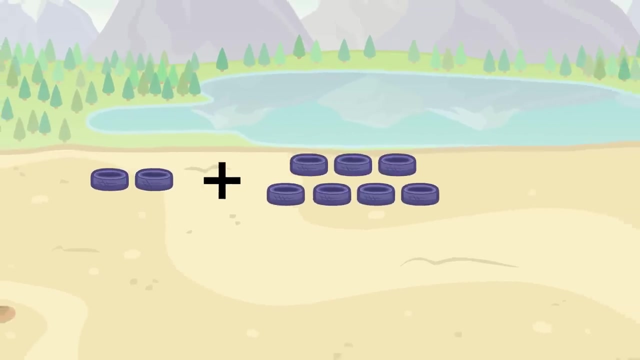 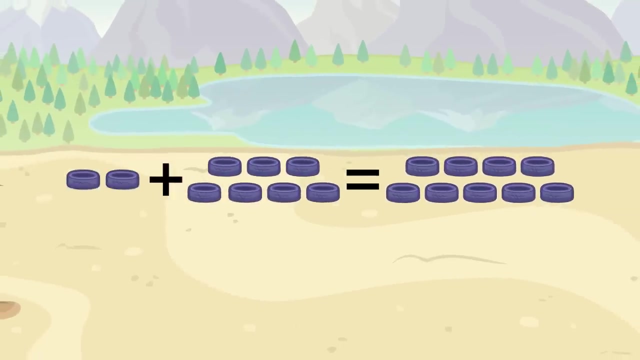 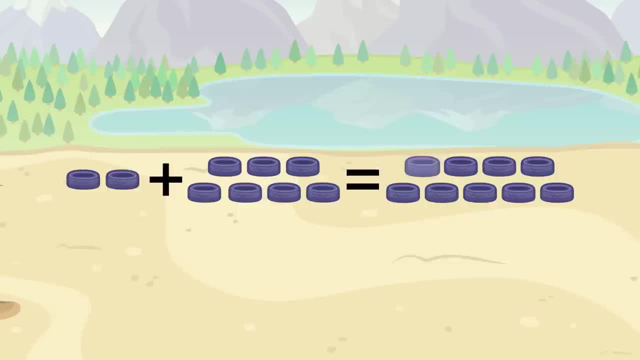 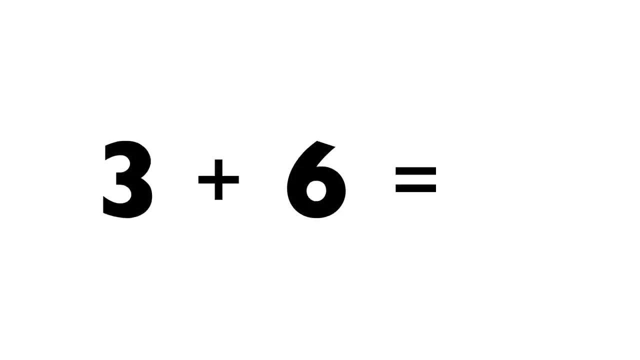 5, 6, 7,, 8, 9, equals 1,, 2,, 3,, 4,, 5,, 6,, 7,, 8, 9.. 3 plus 6 equals 3 plus 6 equals 9.. 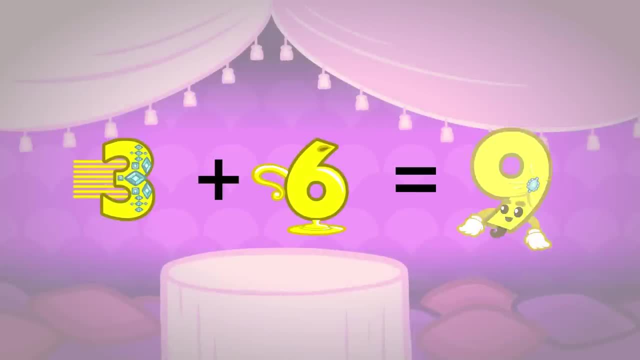 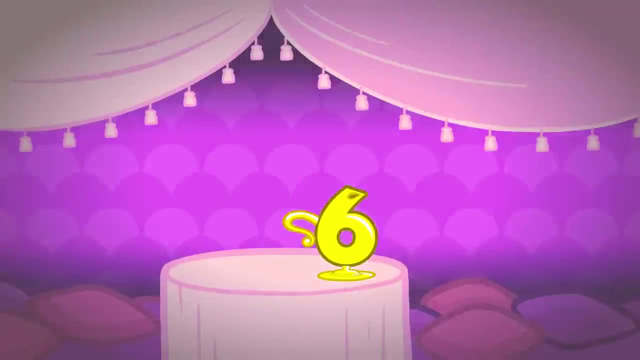 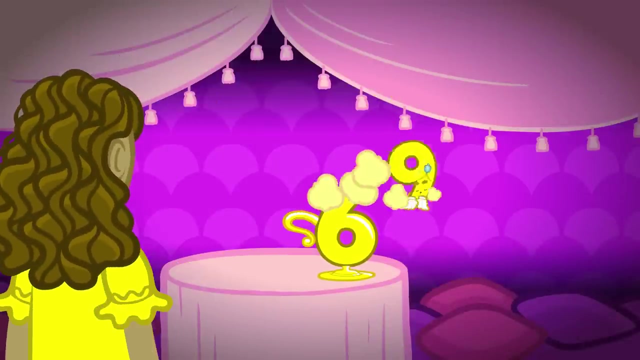 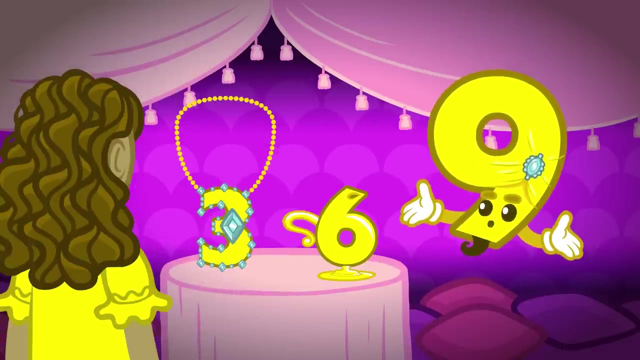 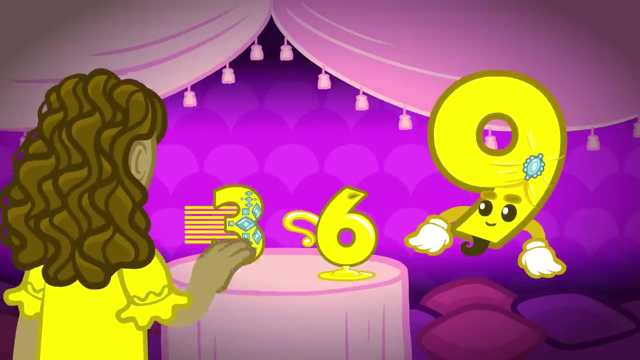 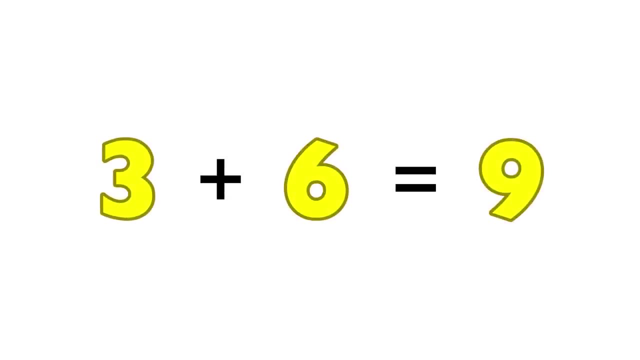 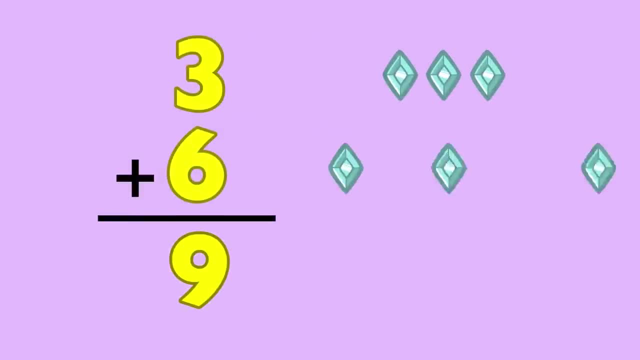 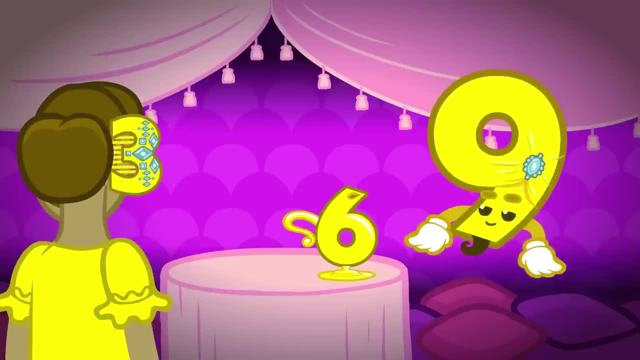 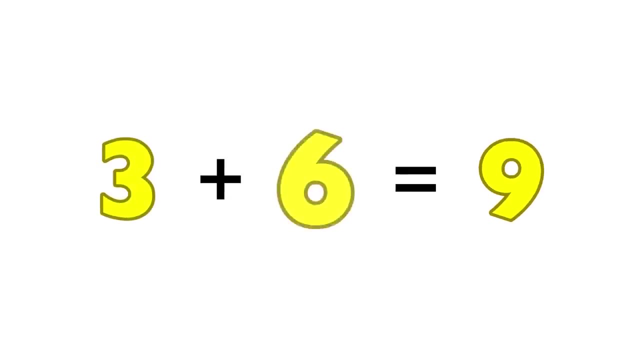 3 plus 6 equals 9.. 3 plus 6 equals 9.. 3 plus 6.. 3 plus 6 equals 9.. 3 plus 6 equals 9.. 3 plus 6 equals 9.. 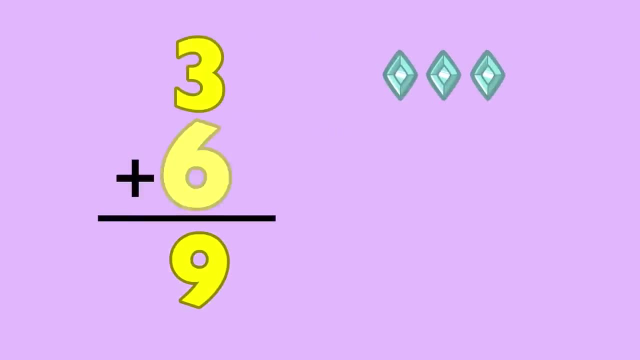 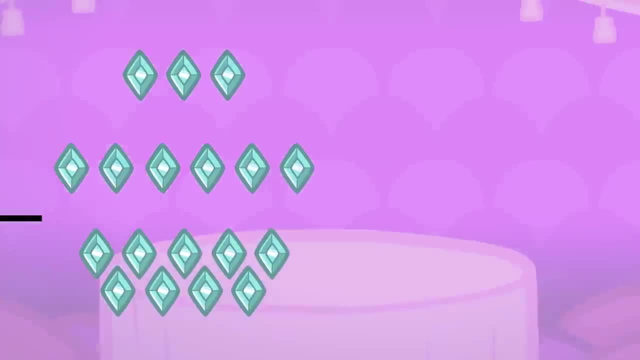 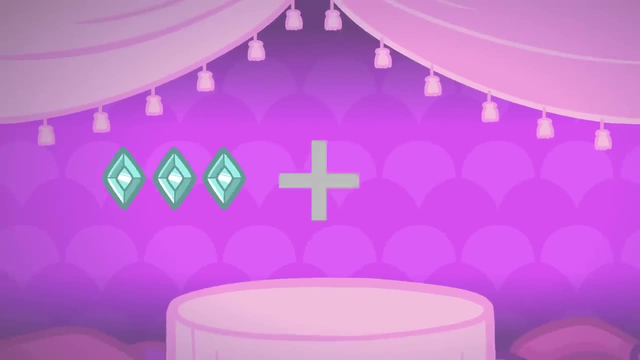 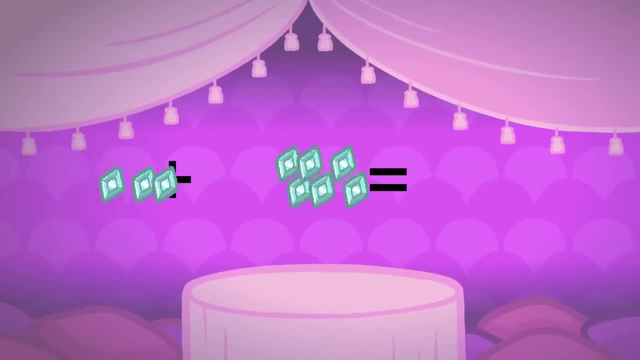 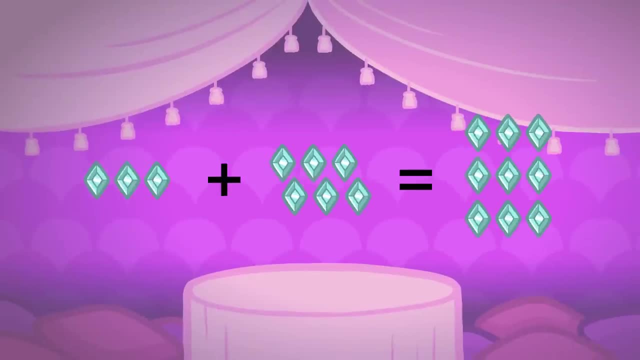 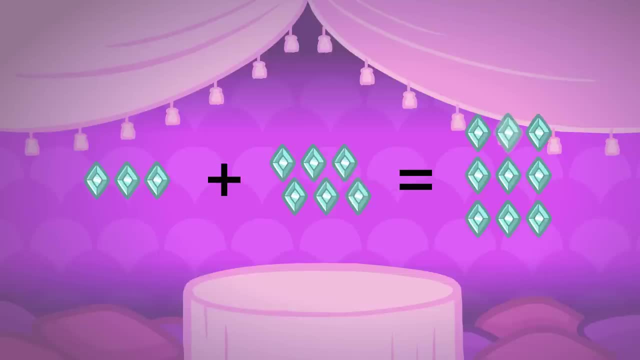 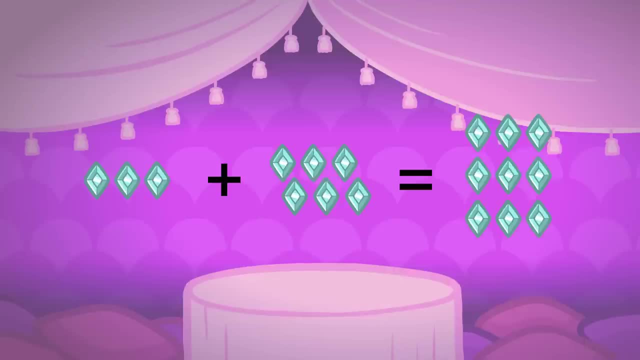 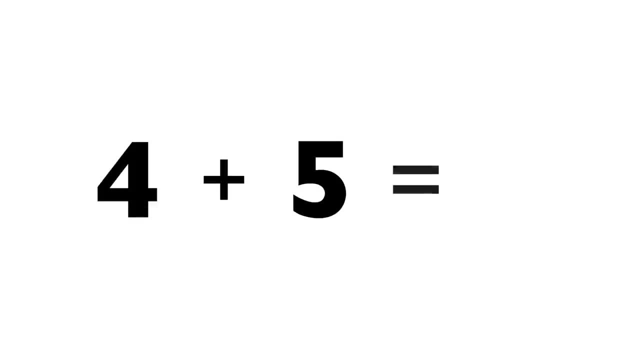 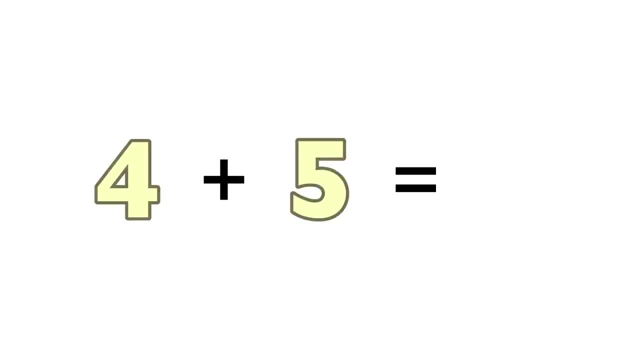 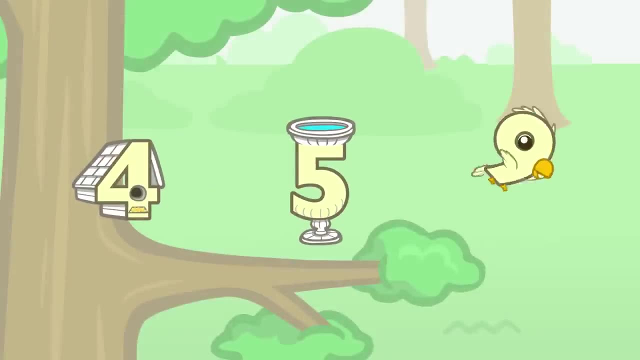 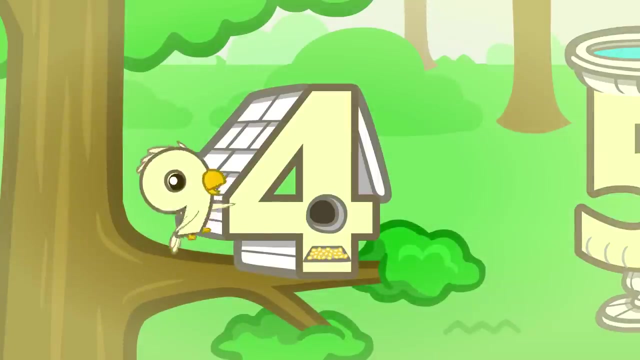 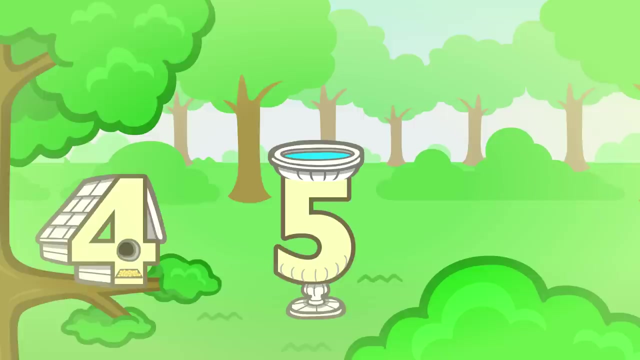 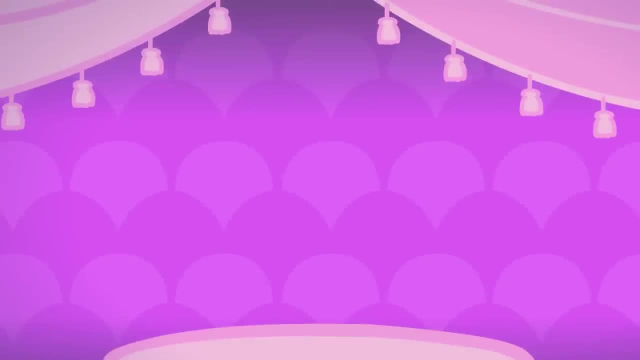 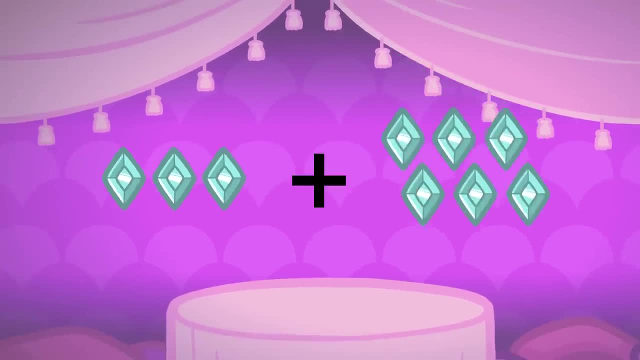 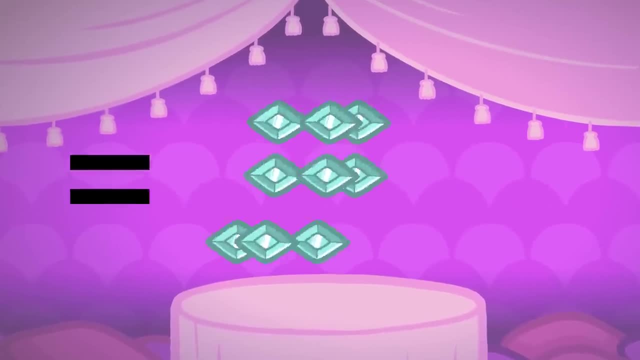 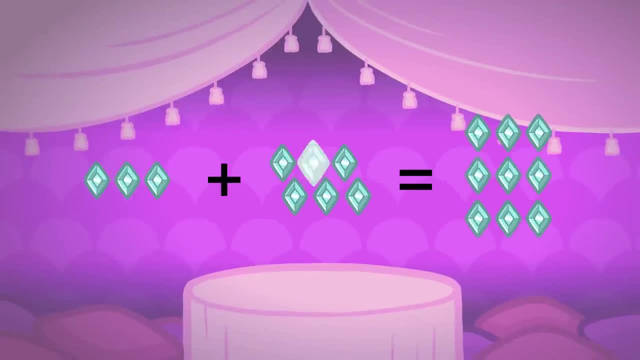 1,, 2,, 3,, 4,, 5,, 6,, 7, 8, 9 equals 1,, 2,, 3,, 4,, 5,, 6,, 7,, 8, 9. 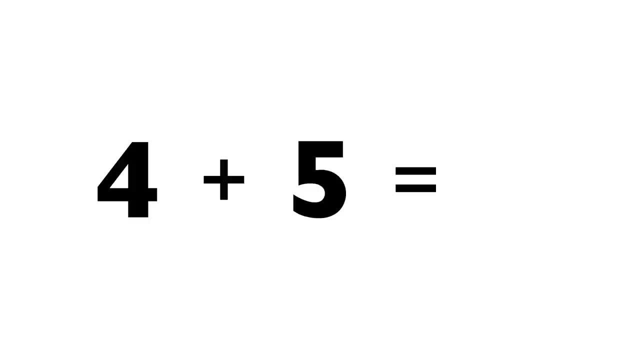 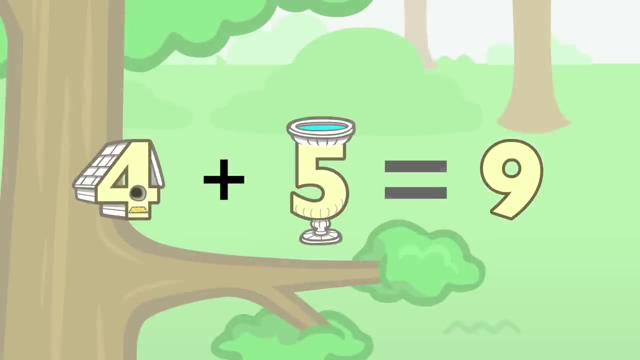 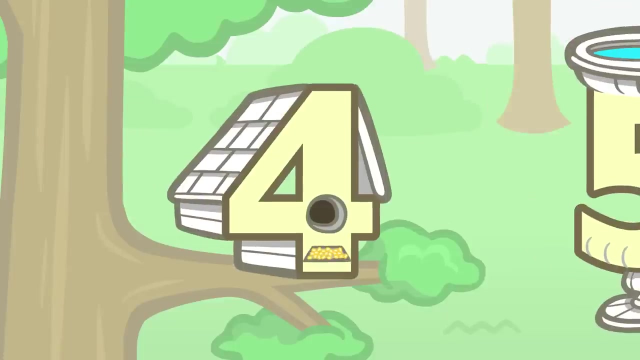 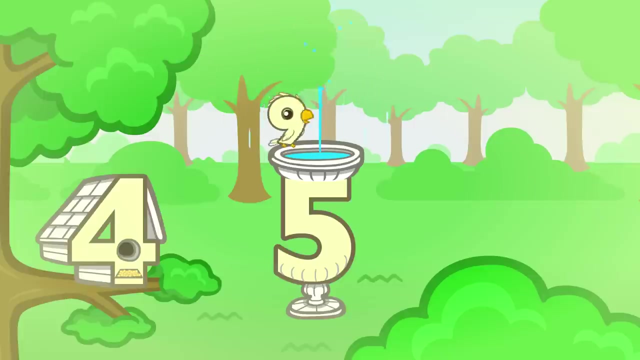 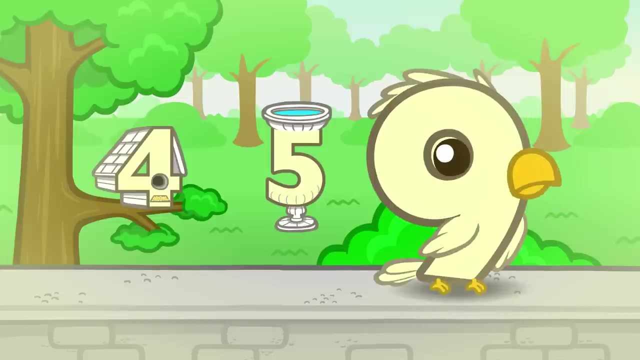 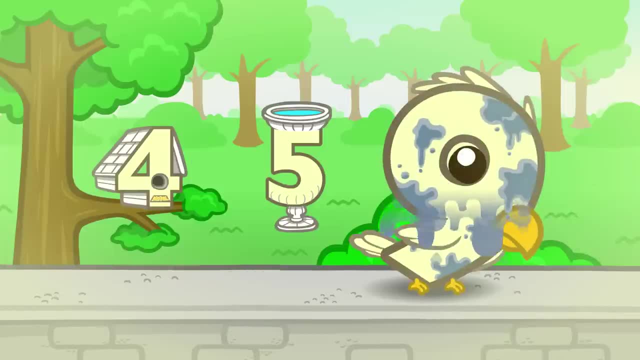 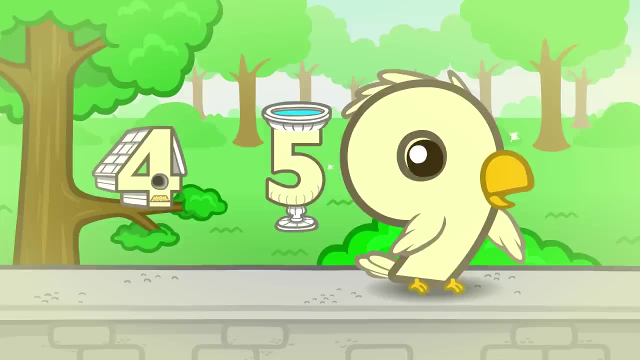 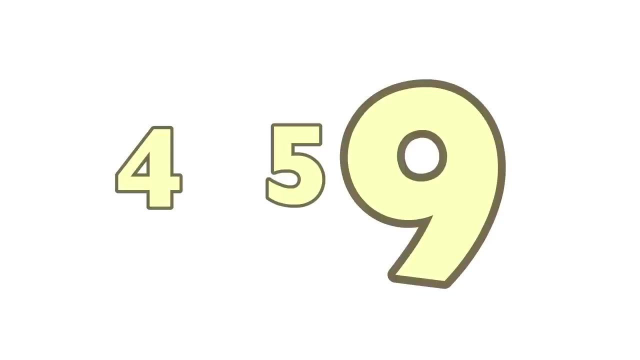 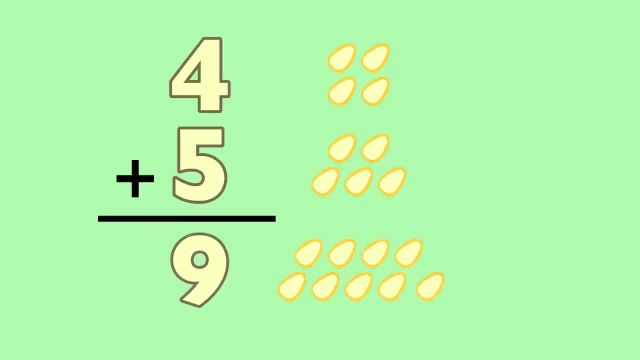 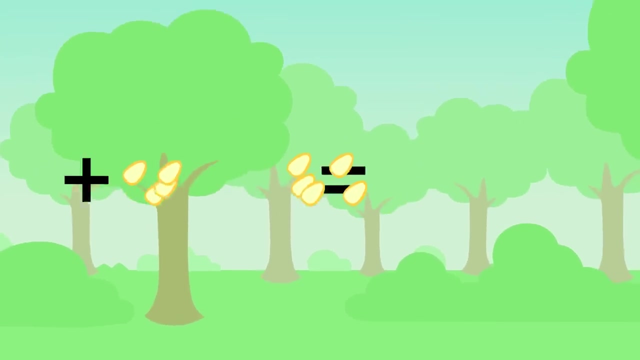 9 4 plus 5- equals 5- equals 9, 4 plus 5- equals 9, 4 plus 5- equals 9, 4 plus 5, equals 9, 9. 9 4 plus 5- equals 9, 9. 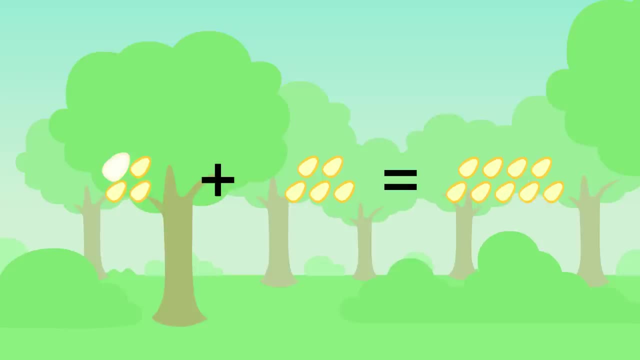 9: 1,, 2,, 3,, 4,, 5,, 6,, 7, 8, 9 equals. 1, 2,, 3,, 4,, 5,, 6,, 7,, 8, 9 equals. 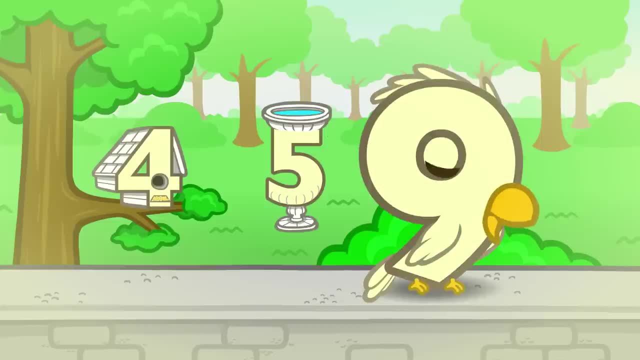 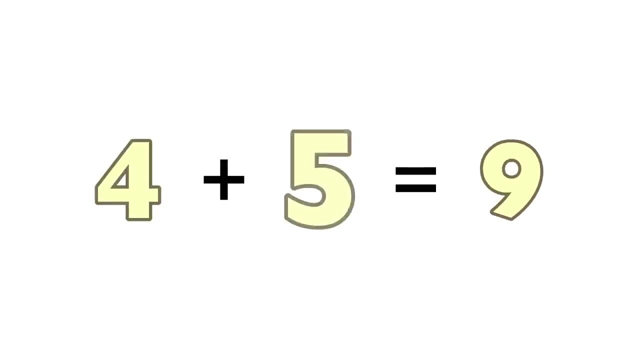 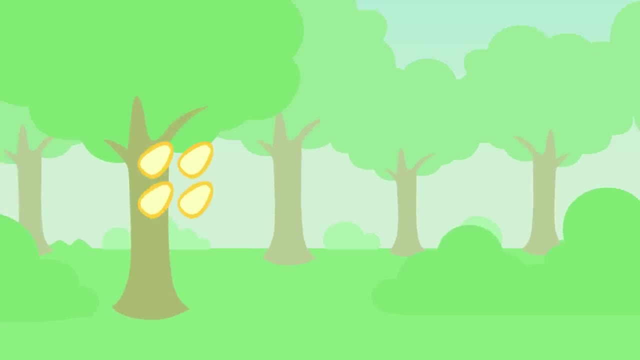 4 plus 5 equals 9.. 4 plus 5 equals 9.. 1,, 2,, 3,, 4,, 5,, 6,, 7,, 8, 9 equals 1,, 2,, 3,, 4,, 5,, 6,, 7,, 8, 9.. 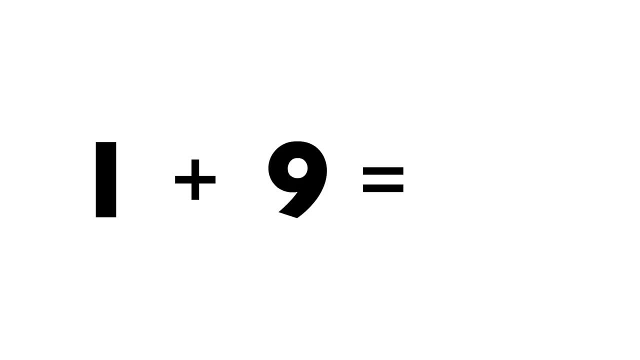 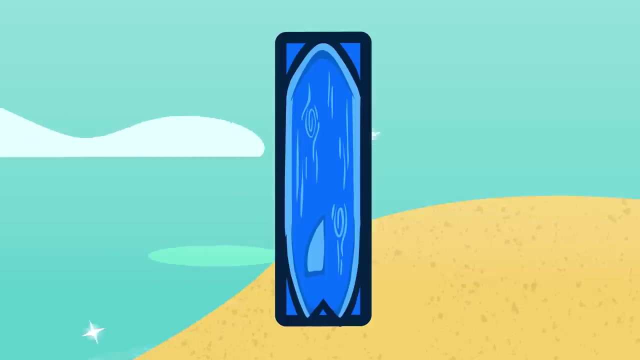 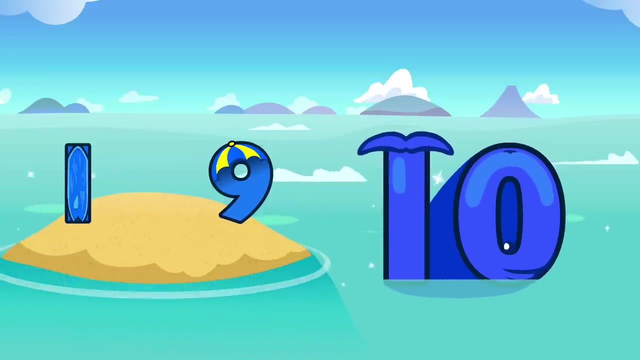 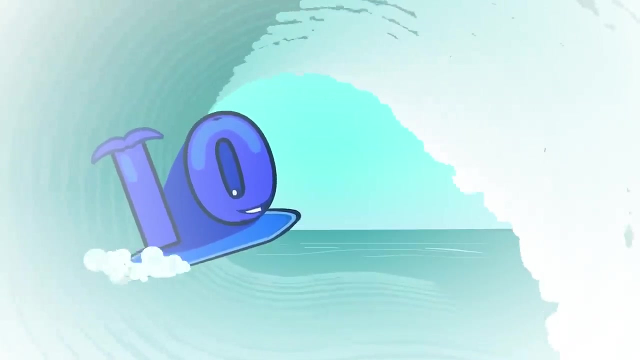 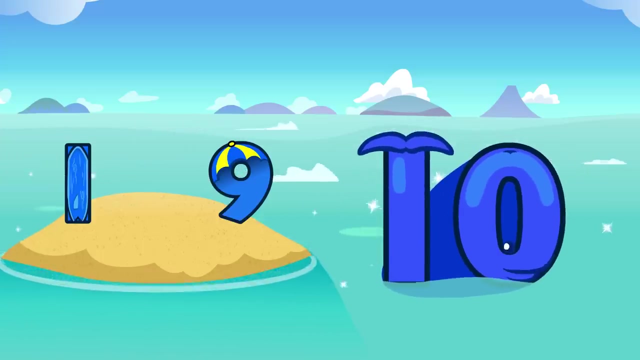 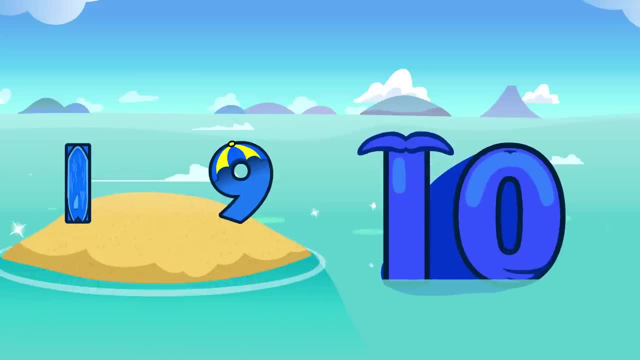 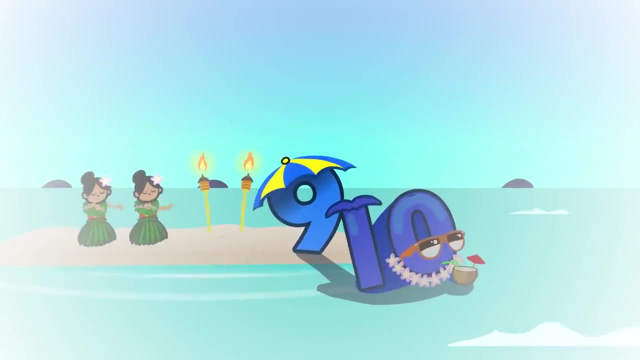 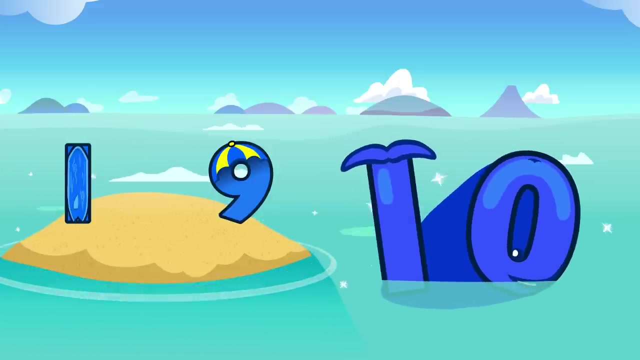 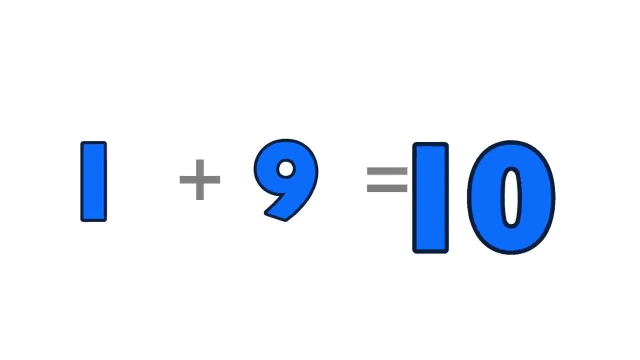 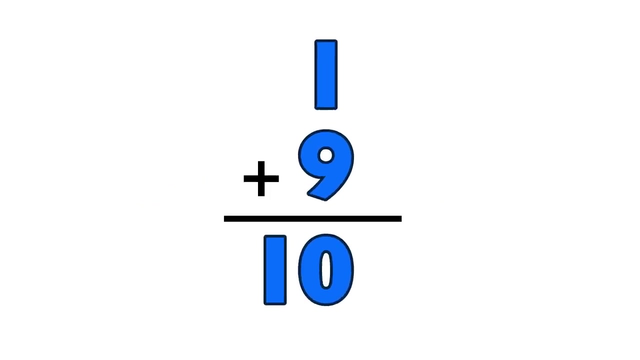 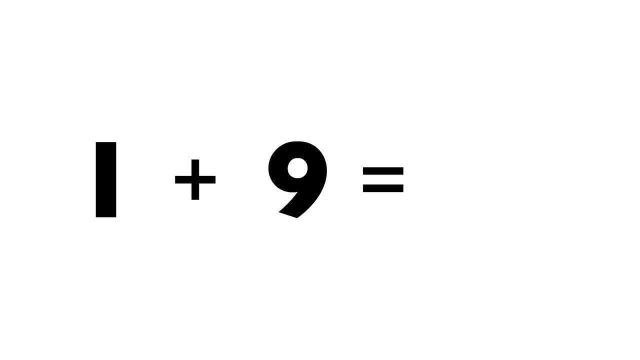 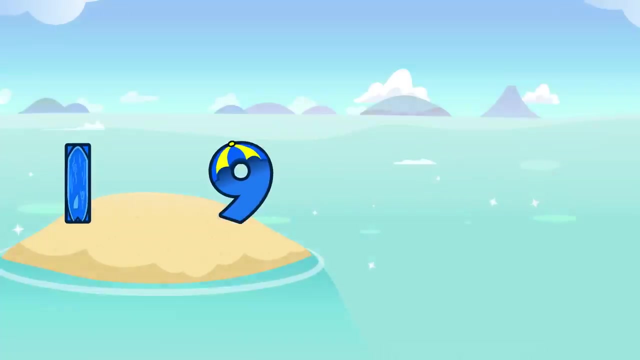 1,, 2,, 3,, 4,, 6,, 7,, 8, 9, 9 equals. 1 plus 9 equals. 1 plus 9 equals 10. 1 plus 9 equals 10. 1 plus 9 equals. 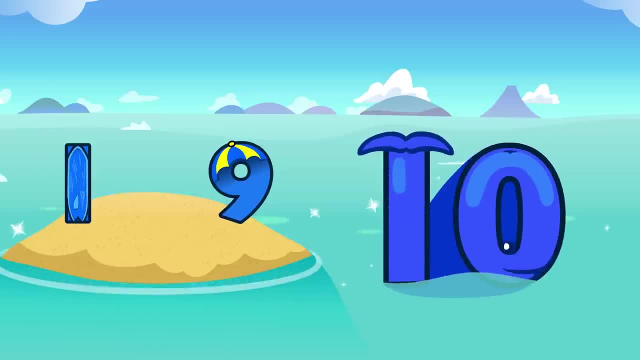 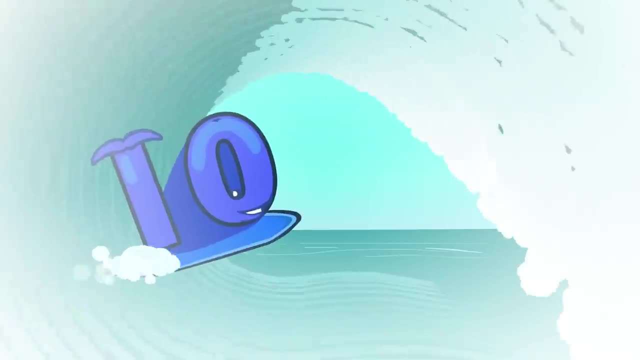 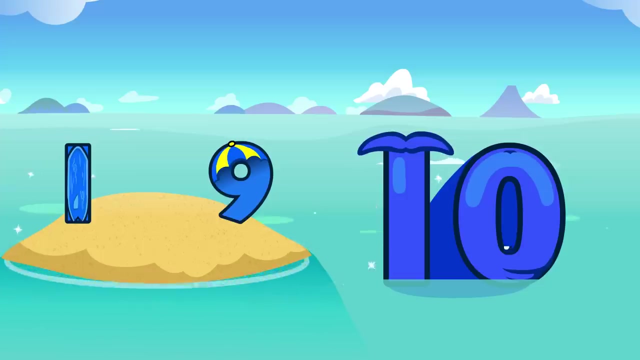 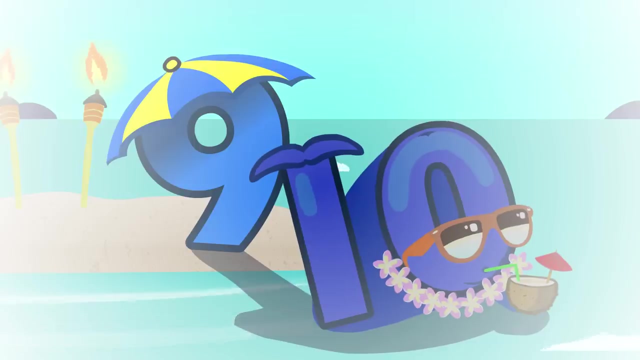 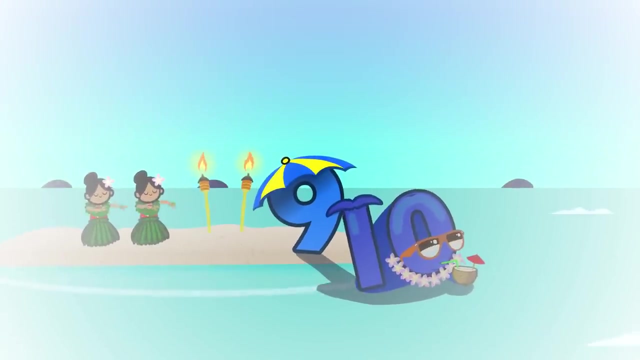 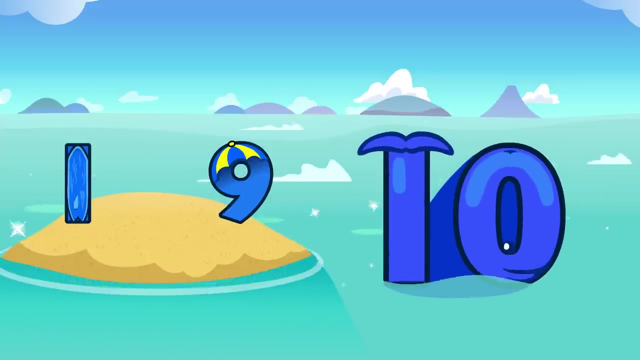 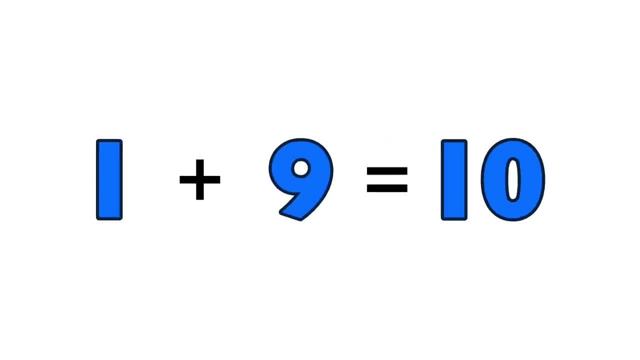 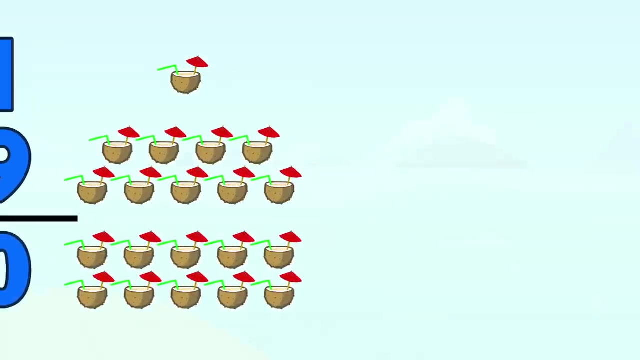 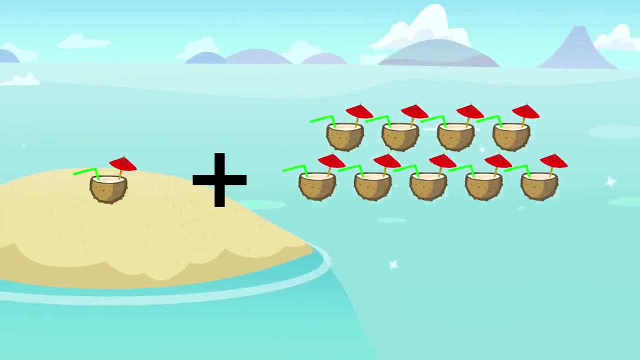 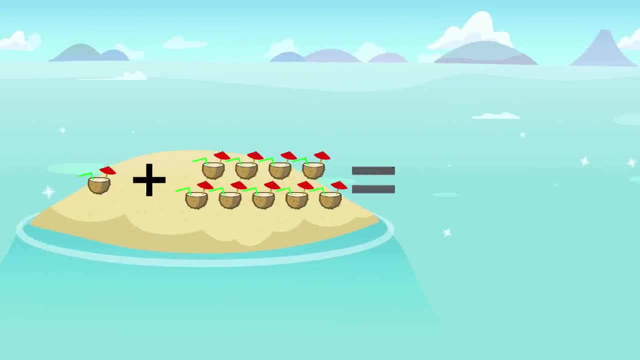 1 plus 9 equals 10, 9 equals 10! 1, 2,, 3,, 4,, 5, 6,, 7,, 8, 9, 10 equals 1, 2, 3,. 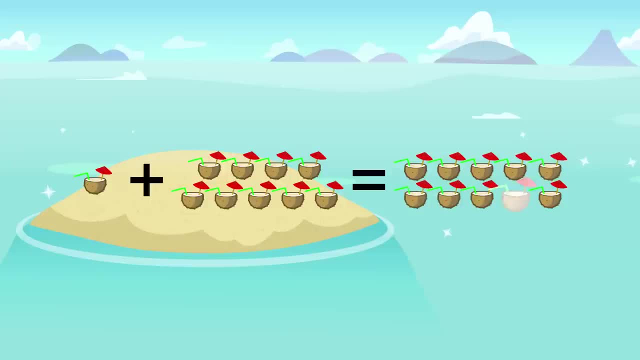 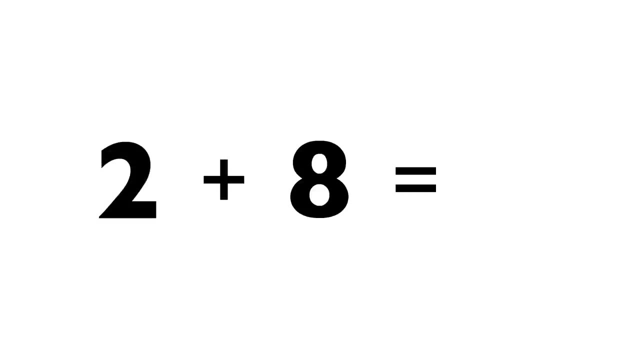 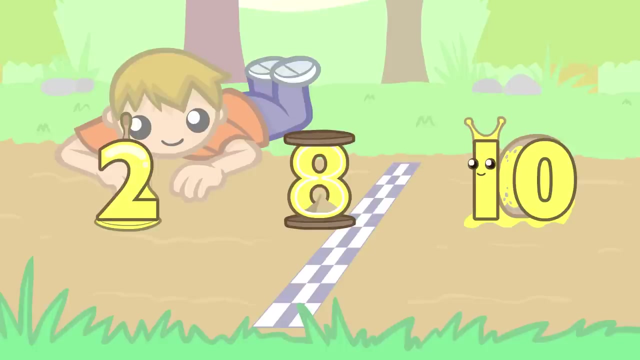 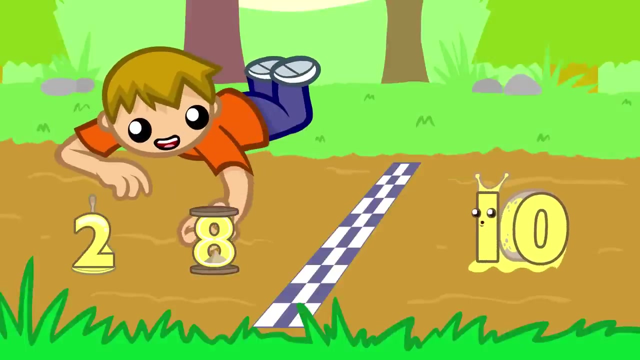 4,, 5,, 6,, 7,, 8,, 9,, 10.. 2 plus 8 equals 2 plus 8 equals 10.. 2 plus 8 equals 10!. 2 plus 8 equals 10. 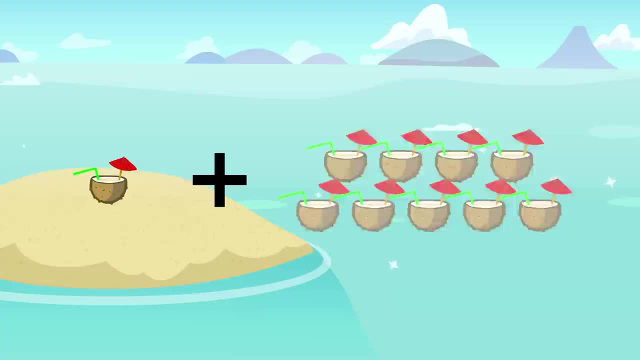 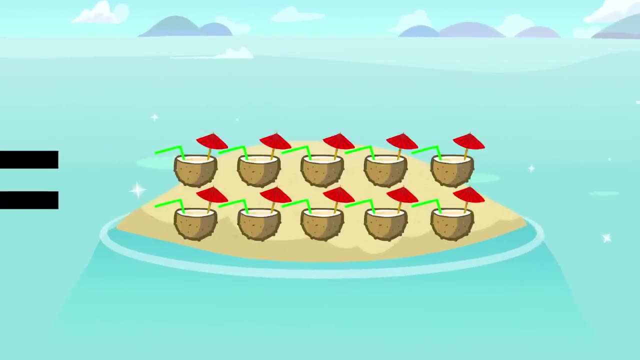 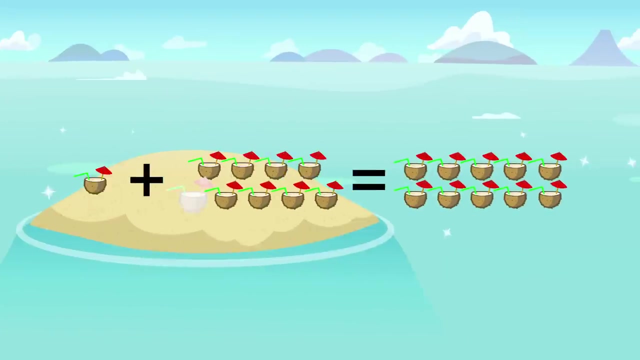 1 plus 9 equals 10: 1,, 2,, 3,, 4,, 5,, 6,, 7,, 8,, 9, 10 equals 1,, 2,, 3,, 4,, 5,, 6,, 7,, 8,, 9, 10.. 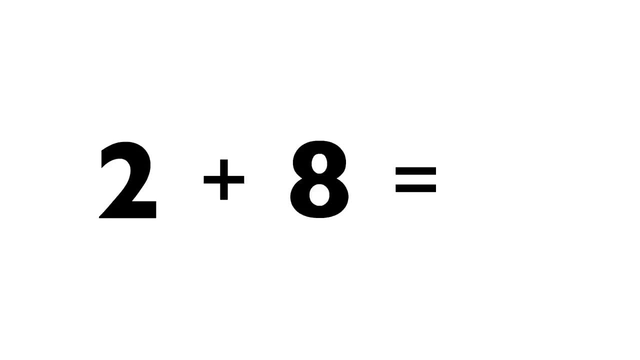 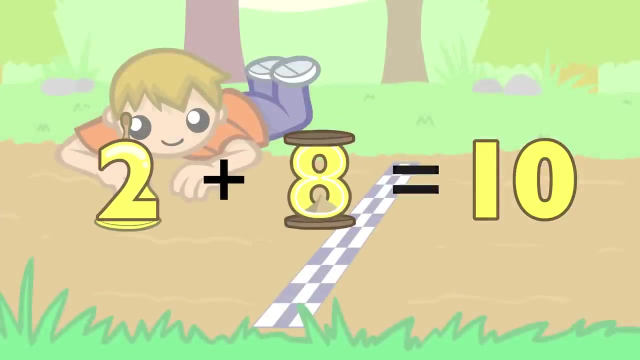 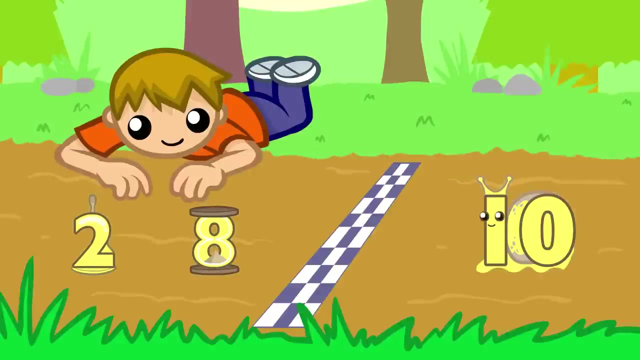 1,, 2,, 3,, 4,, 5,, 6,, 7,, 8,, 9, 10.. 1, 2,, 3,, 4,, 5,, 6,, 7,, 8,, 9, 10.. 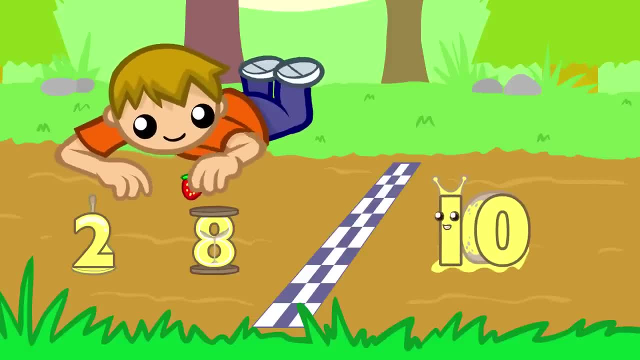 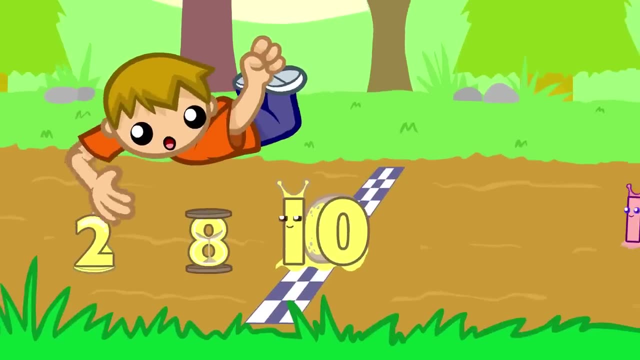 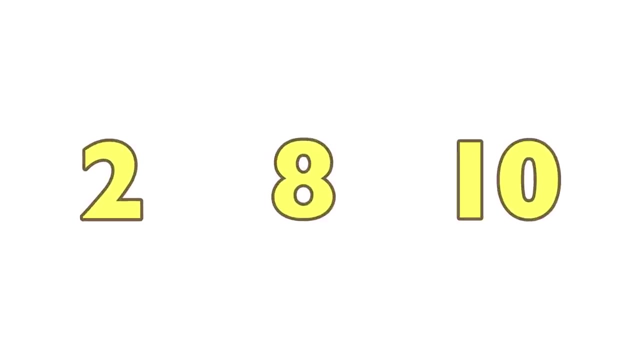 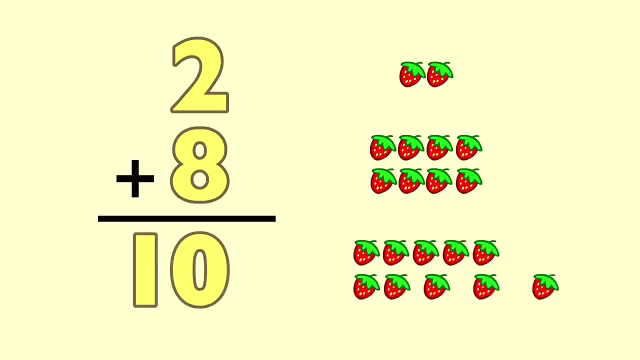 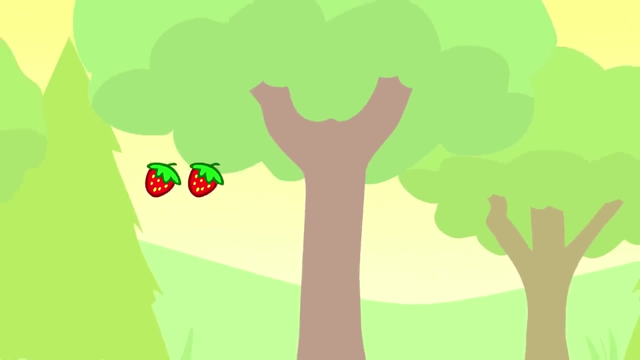 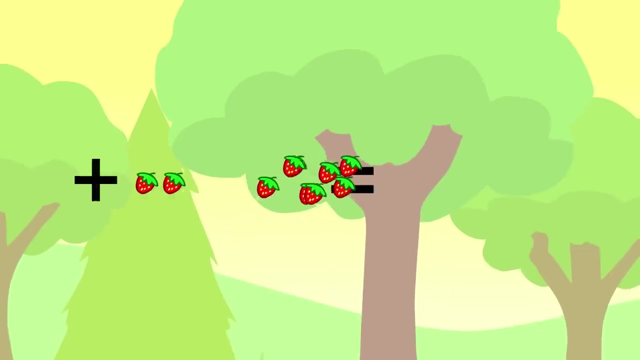 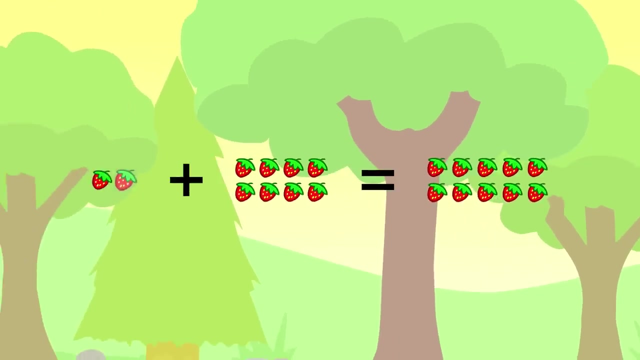 1,, 2,, 3,, 4,, 5,, 6,, 7,, 8,, 9, 10.. 2 plus 8 equals 10, 2 plus 8 equals 10. 1,, 2,, 3,, 4,, 5,, 6,, 7,, 8,, 9, 10. 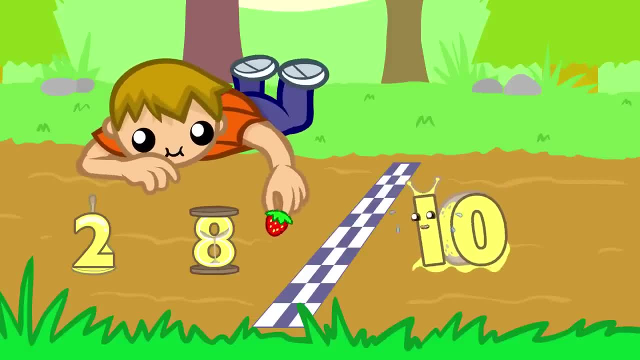 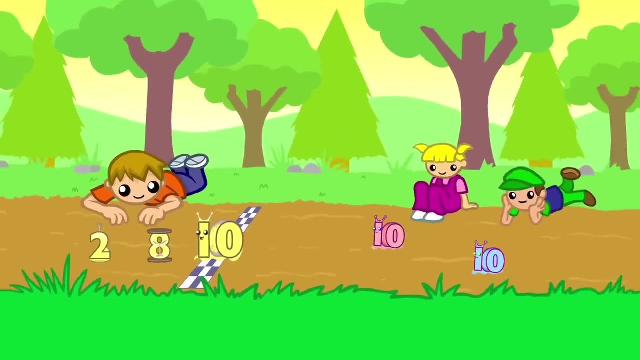 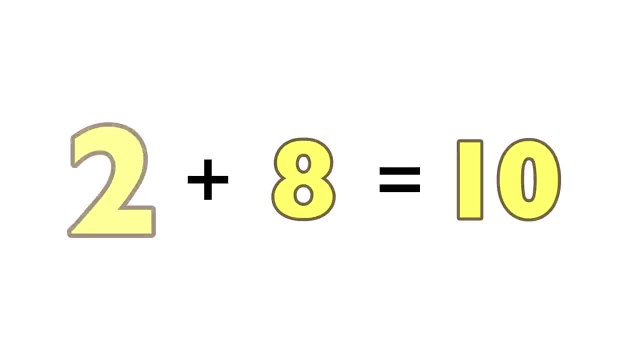 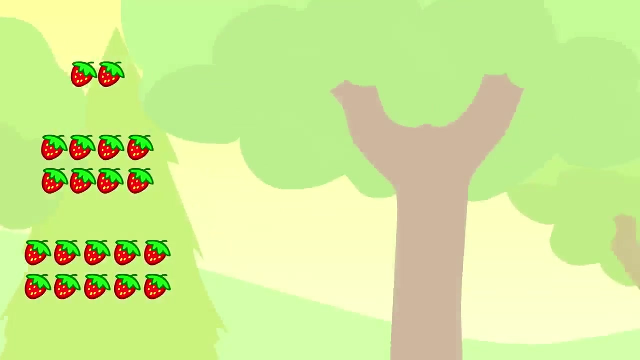 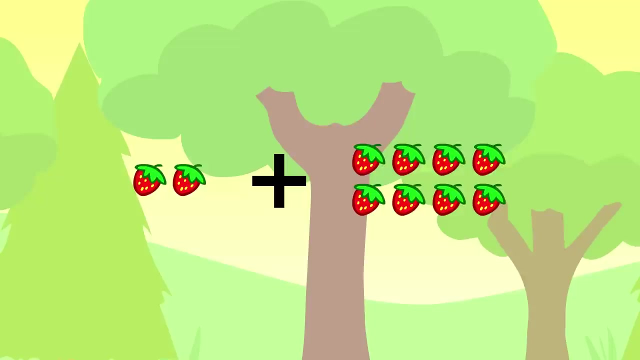 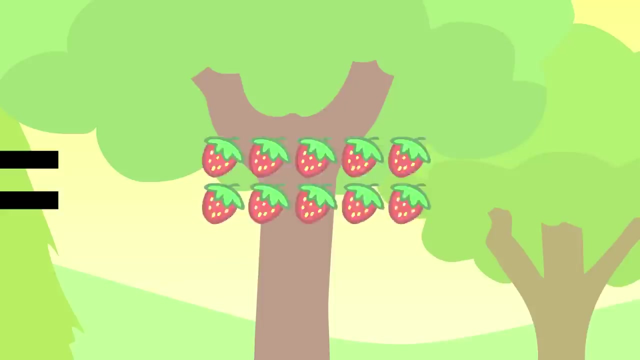 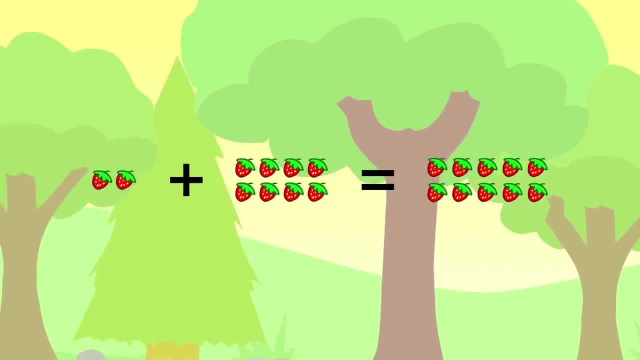 2 plus 8 equals 10.. 1,, 2,, 3,, 4,, 5,, 6,, 7,, 8,, 9, 10 Equals 1,, 2,, 3,, 4,, 5,, 6,, 7,, 8,, 9, 10. 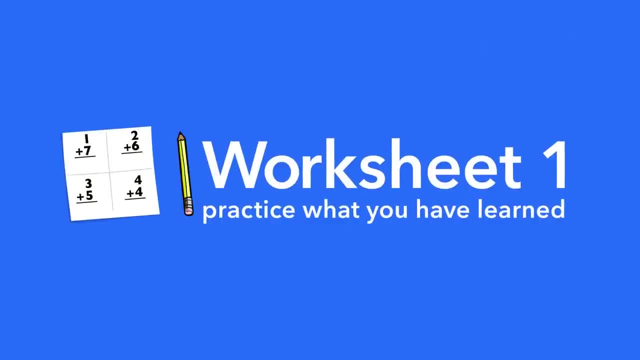 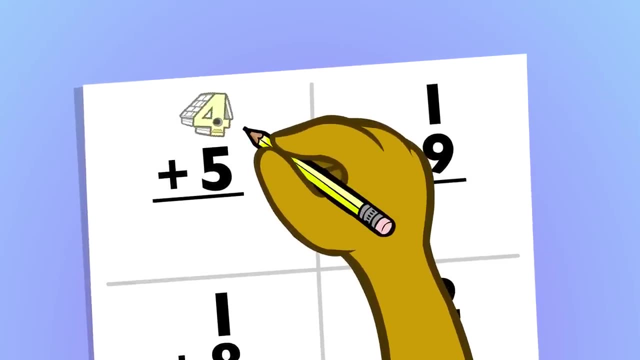 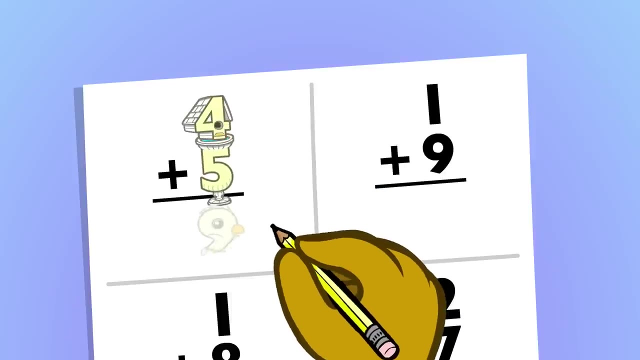 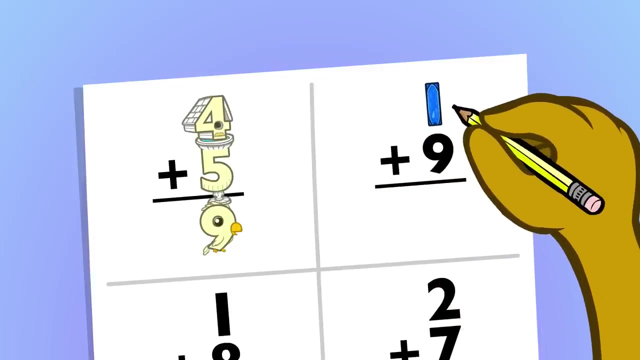 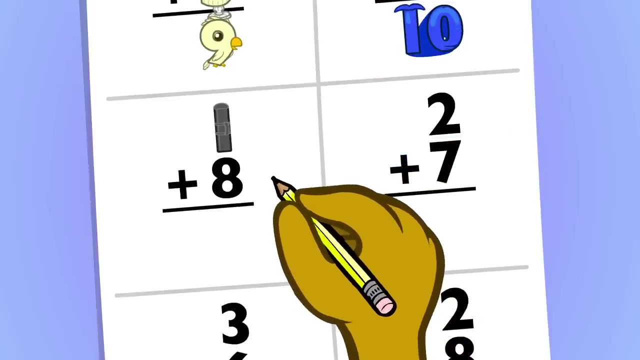 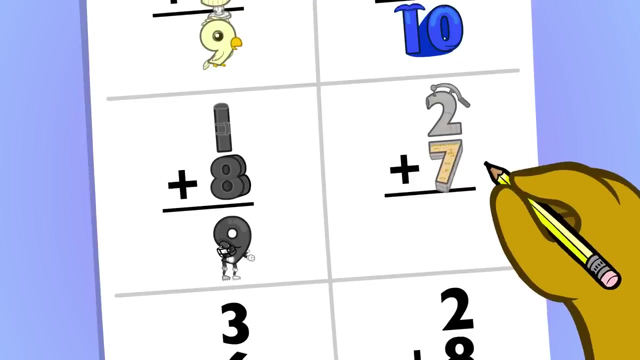 1,, 2,, 3,, 4,, 5,, 6,, 7,, 8,, 9,, 10 Plus 9- Equals 10. 1 Plus 8: Equals 9. 2 Plus 7- Equals 9. 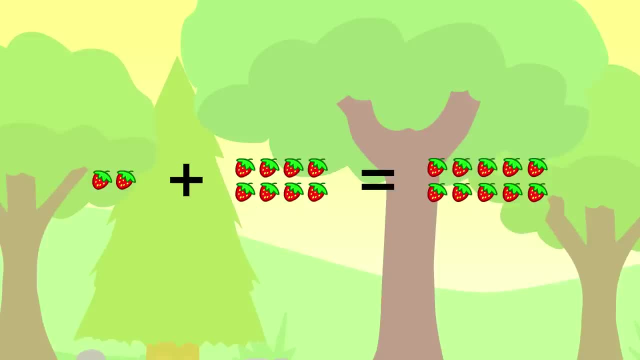 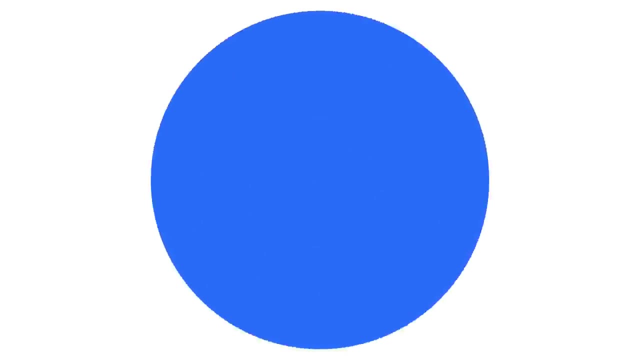 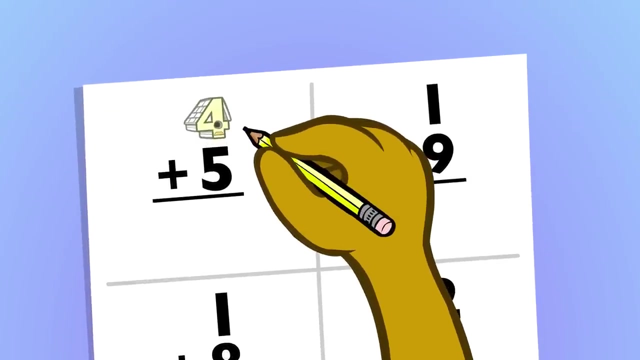 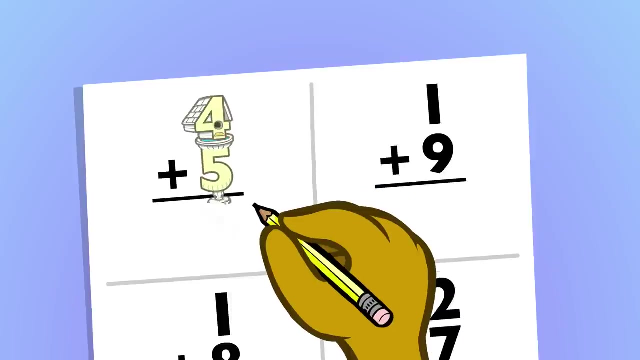 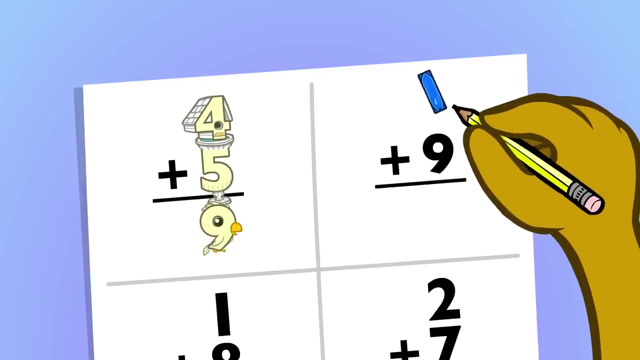 equals 1,, 2,, 3,, 4,, 5,, 6,, 7,, 8,, 9,, 10, 4, 4, 4, 4 plus 5 equals 9. 1 plus 9 equals 10. 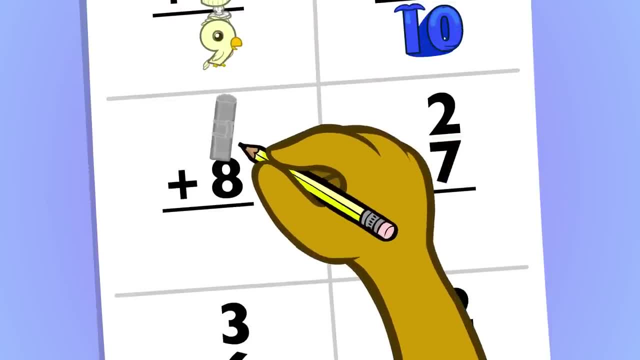 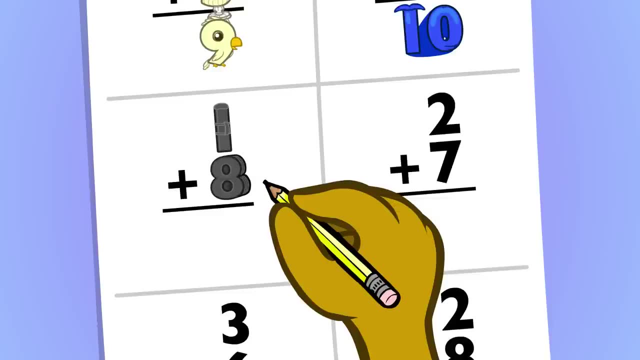 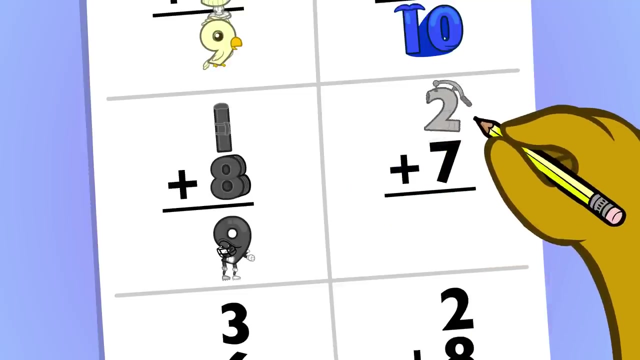 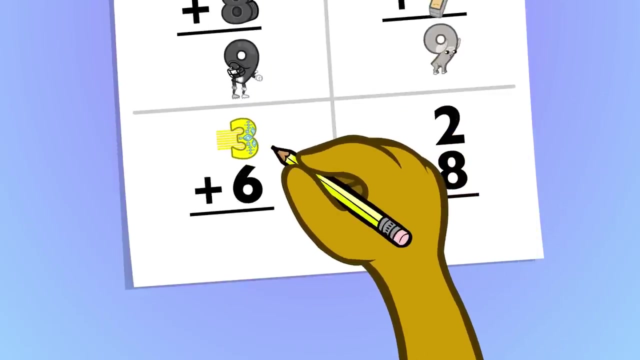 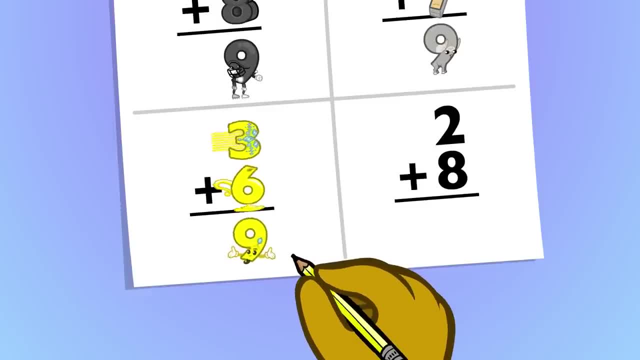 5 plus 7 equals 3 plus 8 is 1, 2, 3, 4,, 5, 6 isn't everything. 3, 3 plus 6 equals 1 plus 7 equals 32: 2, 3 plus 7 in total. 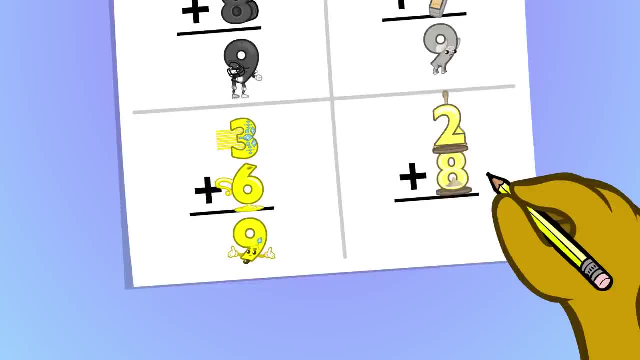 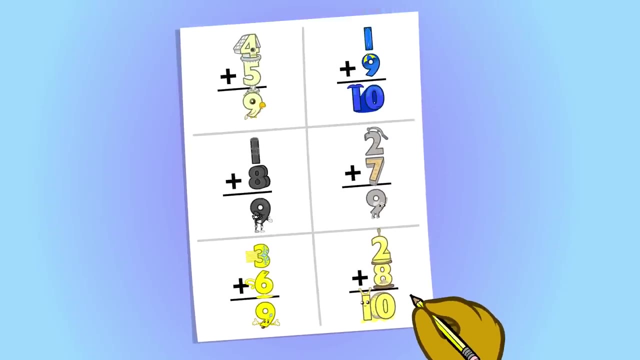 16: 2, 2, 8, 8 collection 9, 4, 4, 4, 3, 2, 2. 4, 3, 2, 4, 9, 2 plus 8 equals 10, 3, 2, 2, 1. 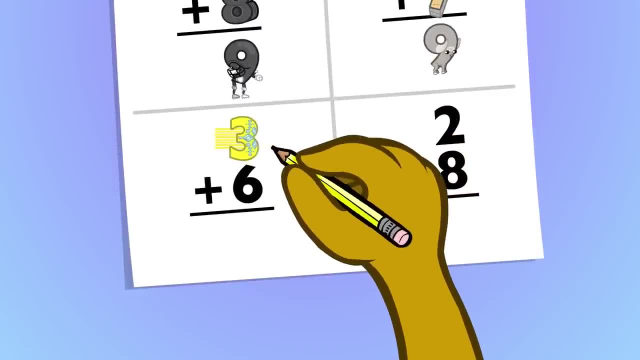 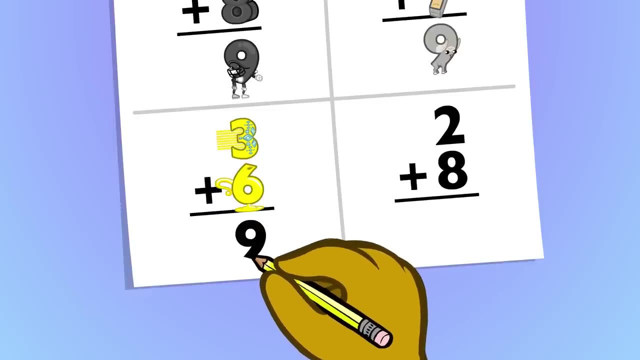 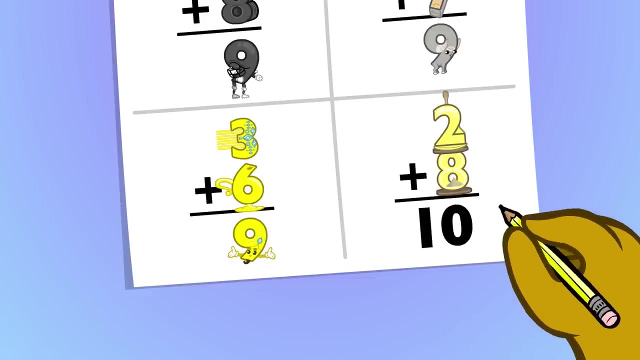 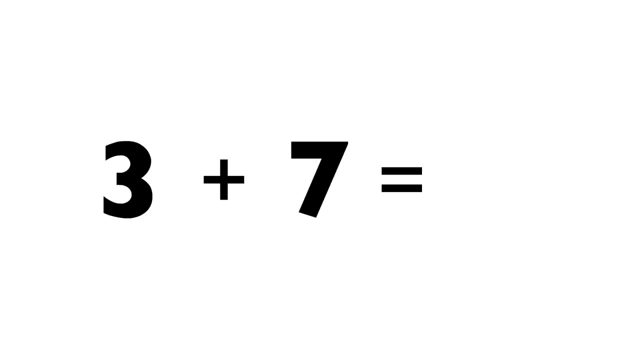 3, 4, 5 Plus 6. Equals 9, 2 Plus 8. Equals 2, 3, 4, 5, 6, 7, 7, 8, 9, 10, 10. 1, 2, 3, 4, 3, 3. 2, 3, 2, 4, 3, 10, 10, 2, 2, 3, 10, 3, 3 plus 7 equals 10.. 3 plus 7 equals 10.. 3 plus 7 equals 10.. 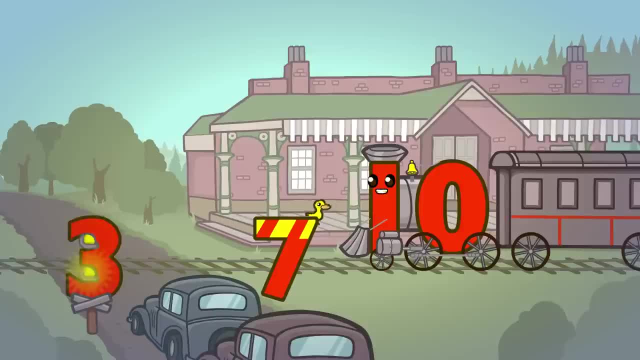 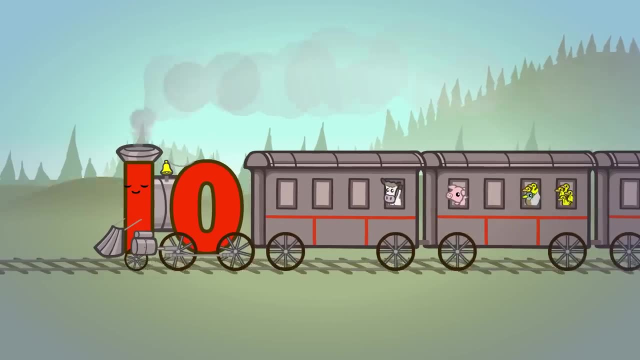 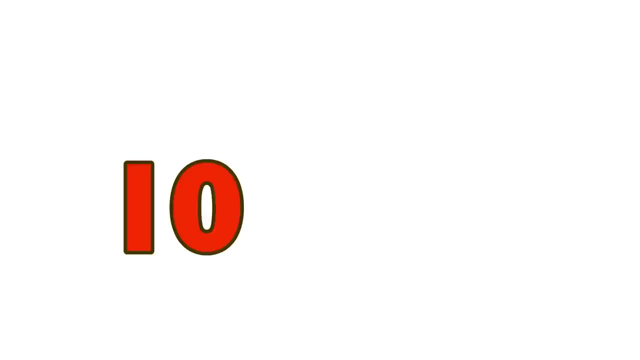 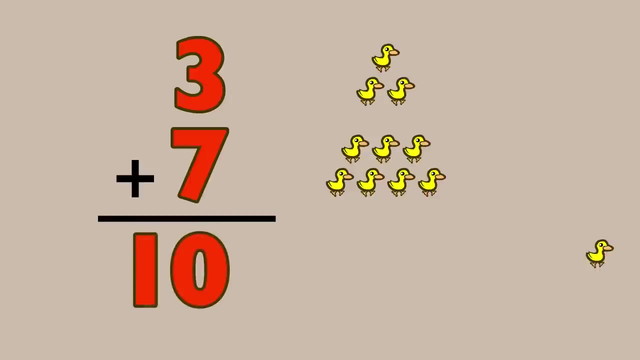 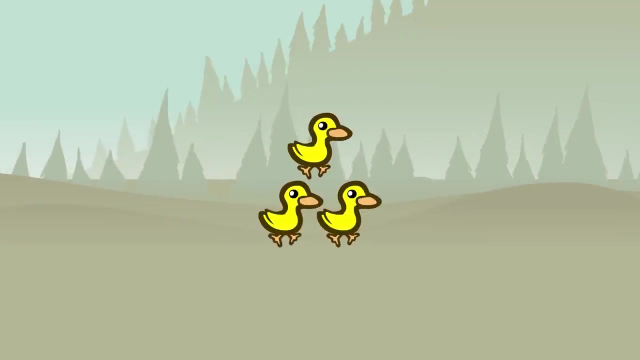 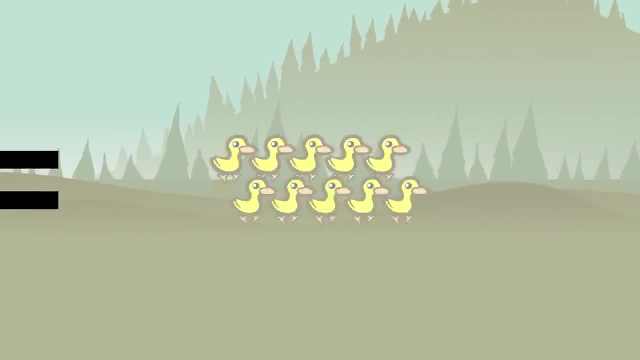 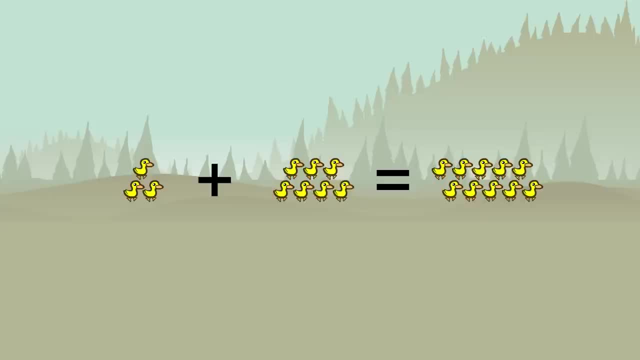 1,, 2,, 3,, 4,, 5,, 6,, 7,, 8,, 9, 10.. 7, 8, 9, 10 equals 1,, 2,, 3,, 4,, 5,, 6,, 7,, 8,, 9, 10.. 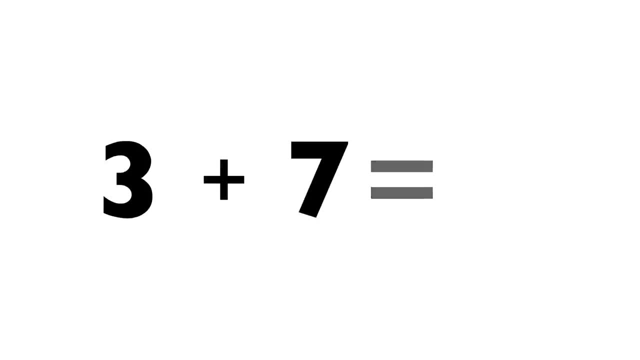 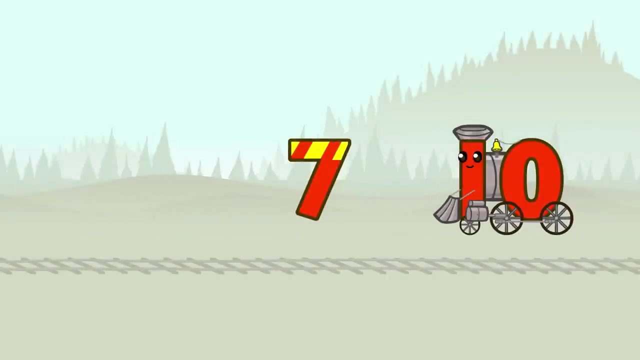 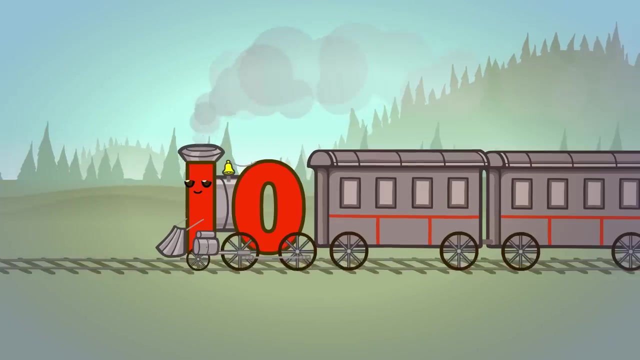 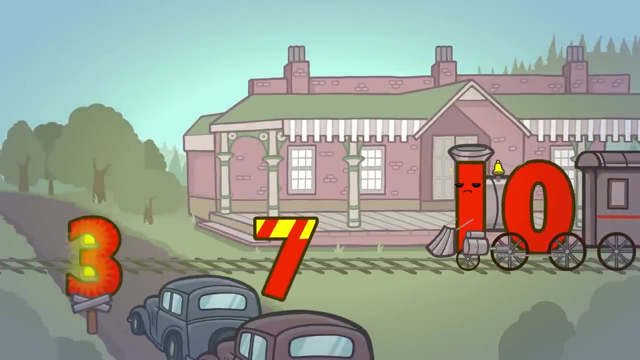 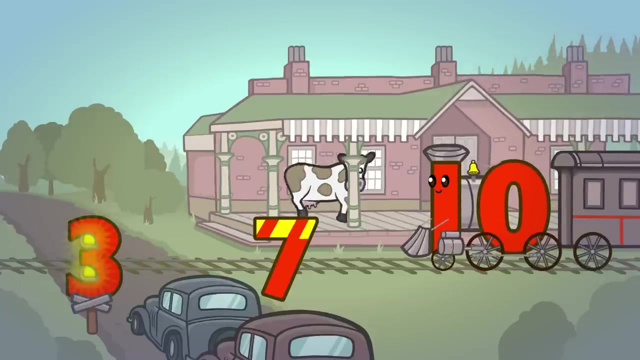 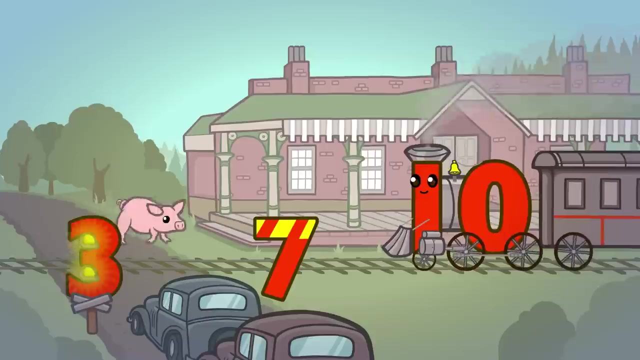 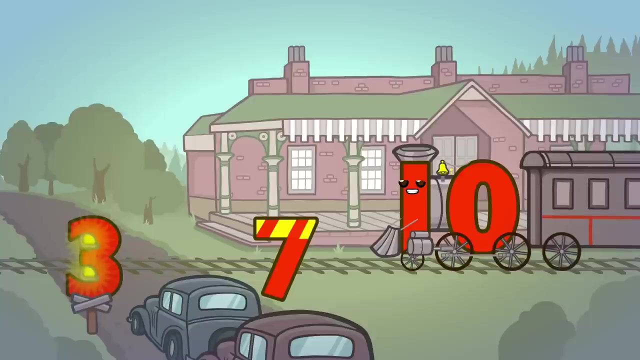 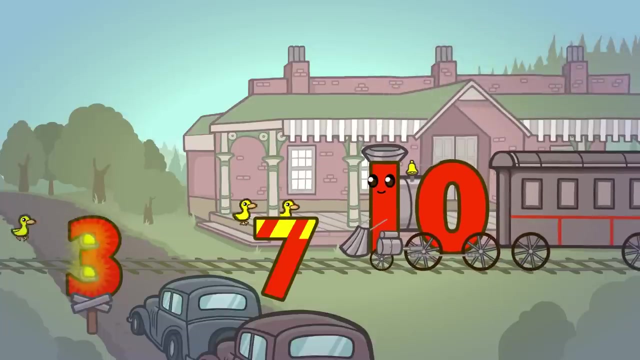 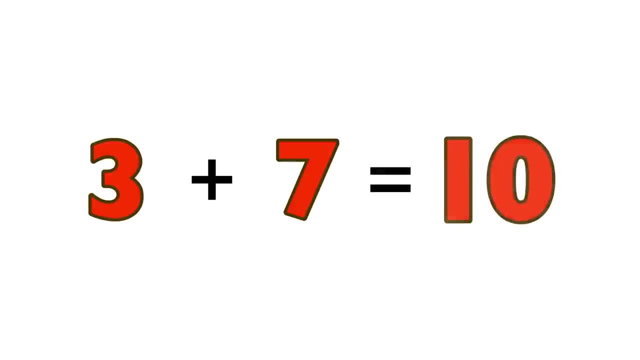 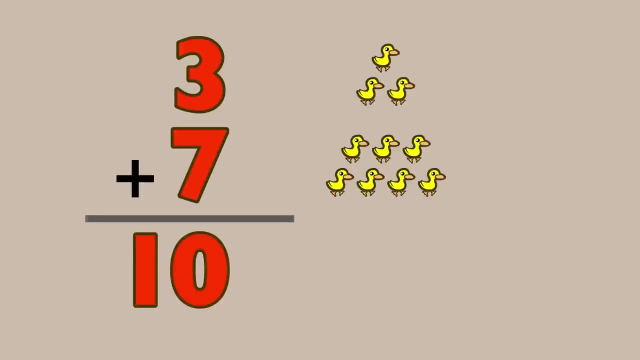 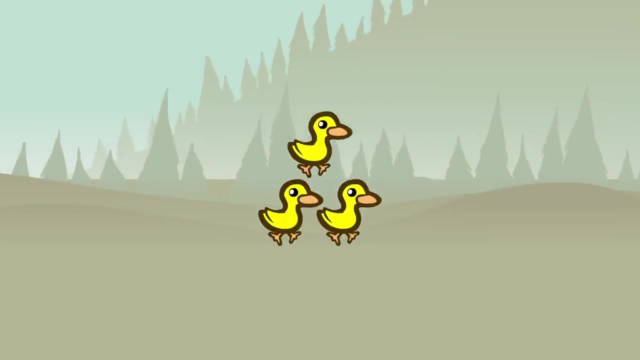 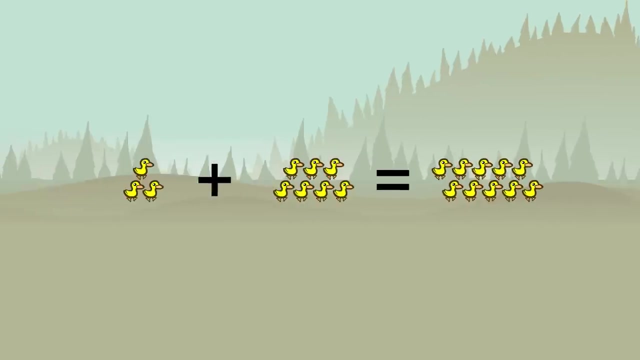 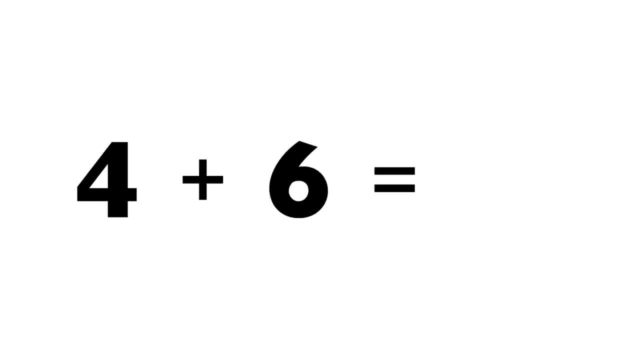 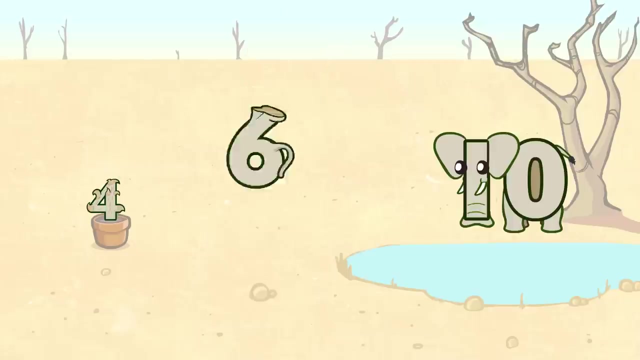 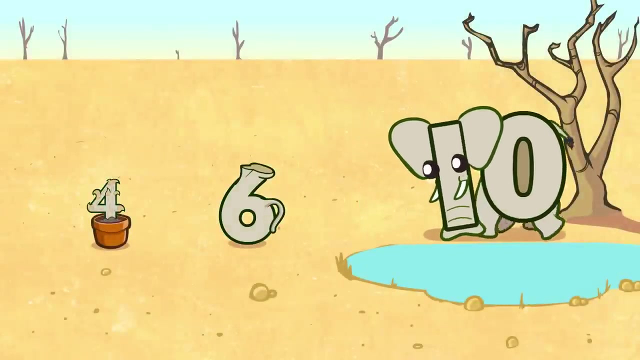 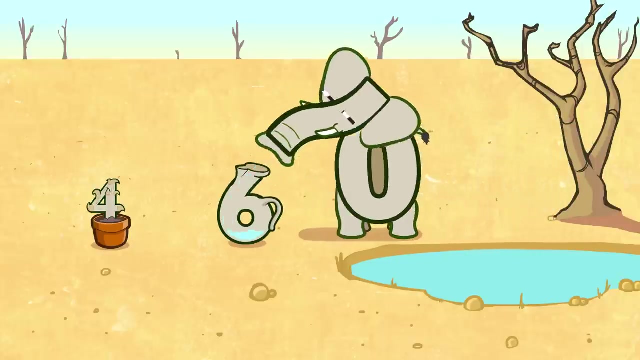 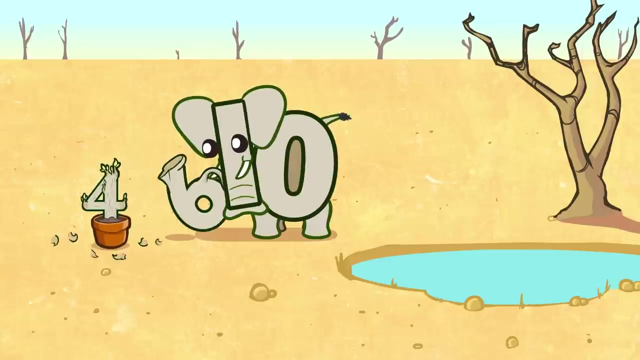 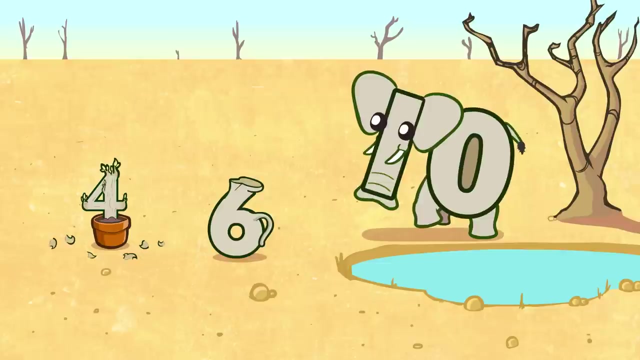 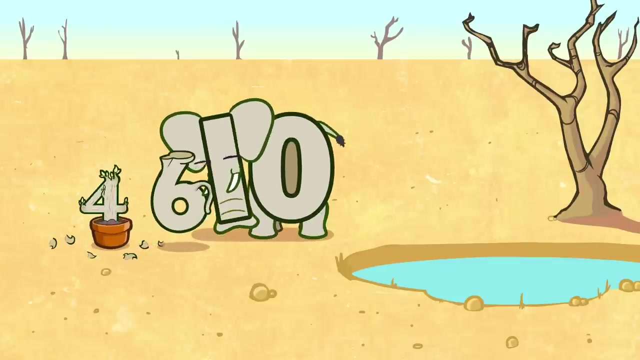 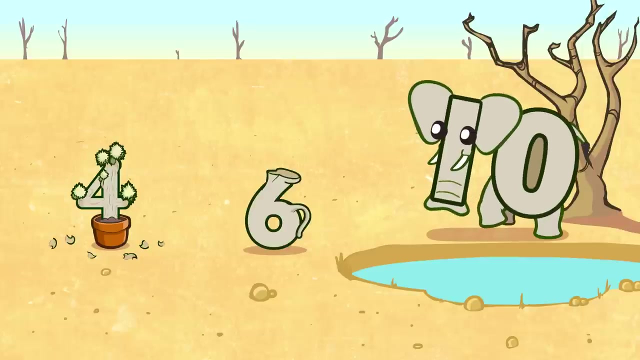 4 plus 6 equals. 4 plus 6 equals 10.. 4 plus 6 equals 10.. 4 plus 6 equals 10.. 4 plus 6.. 4 plus 6 equals 10.. 4 plus 6 equals 10.. 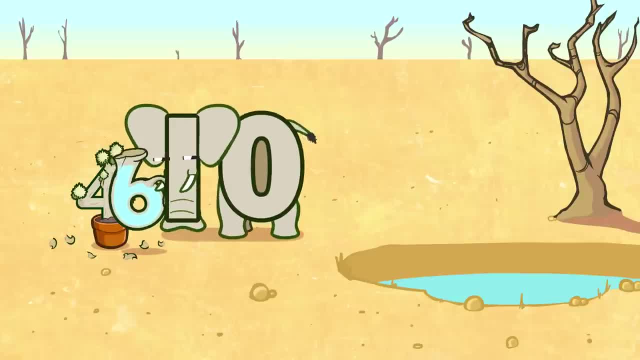 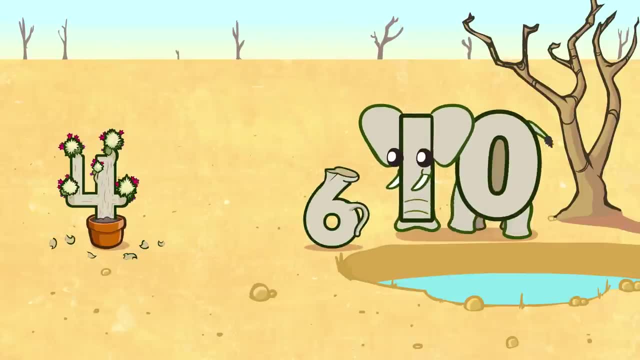 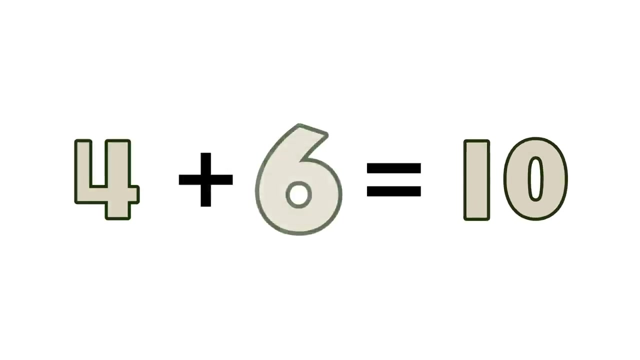 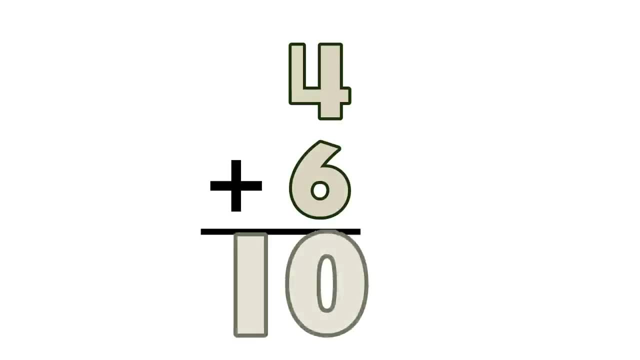 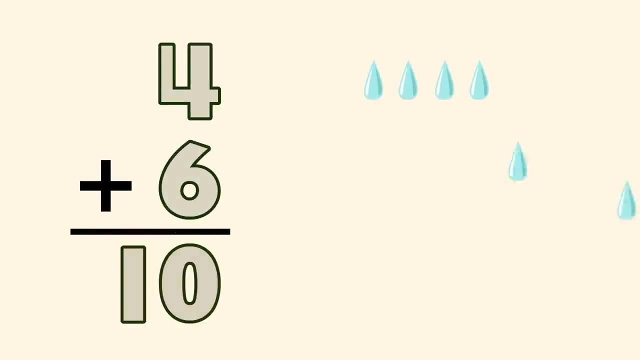 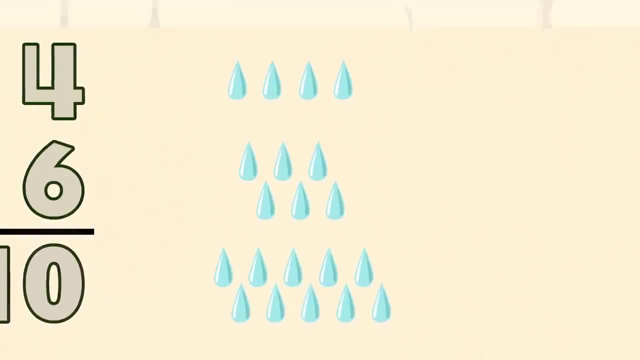 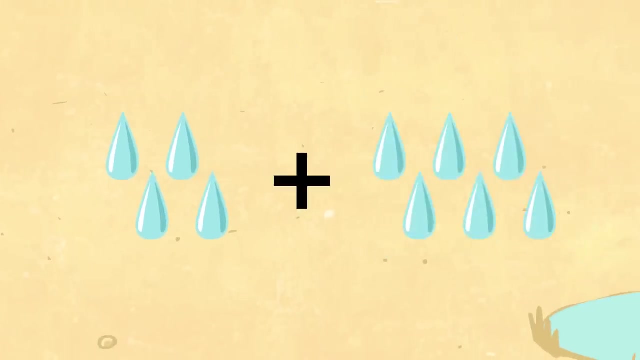 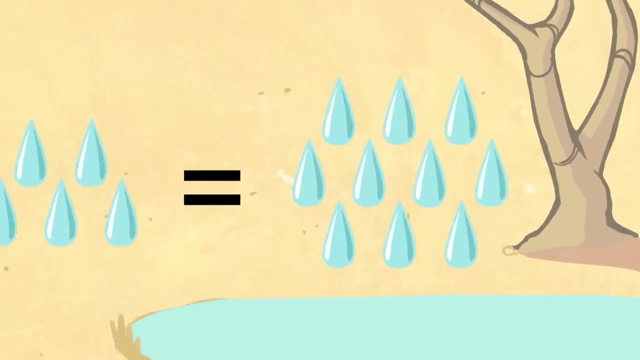 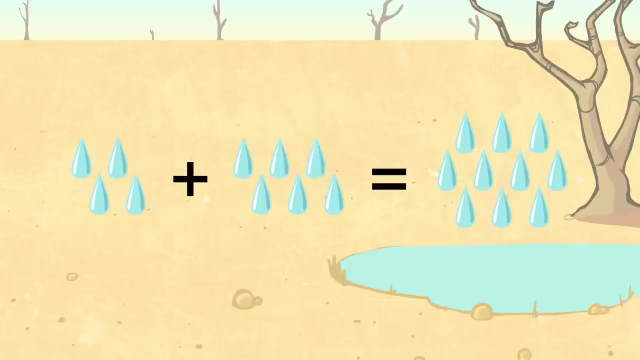 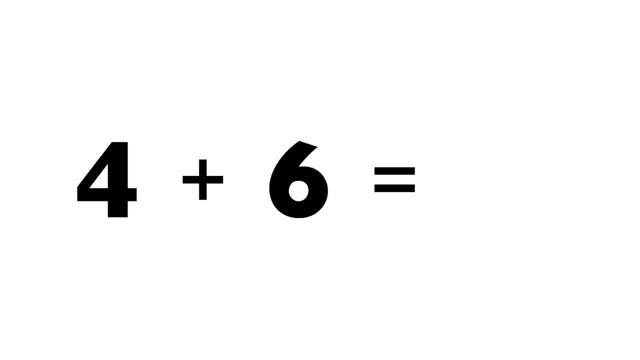 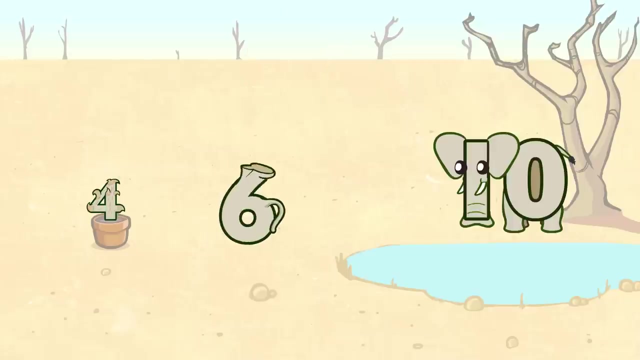 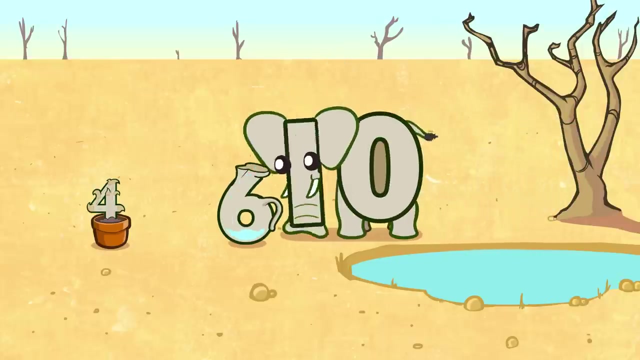 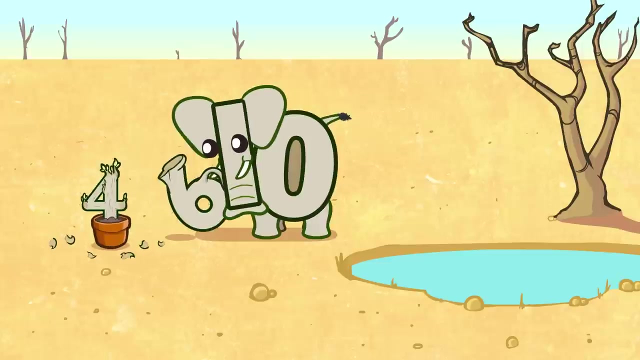 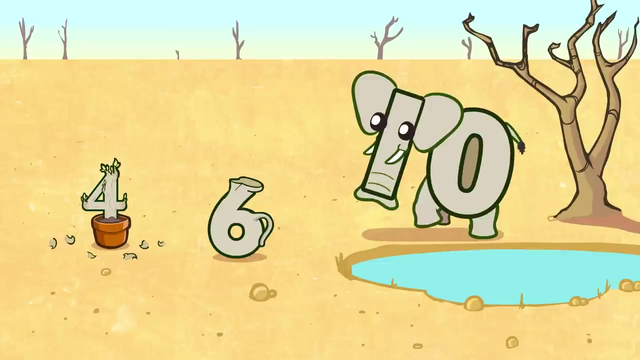 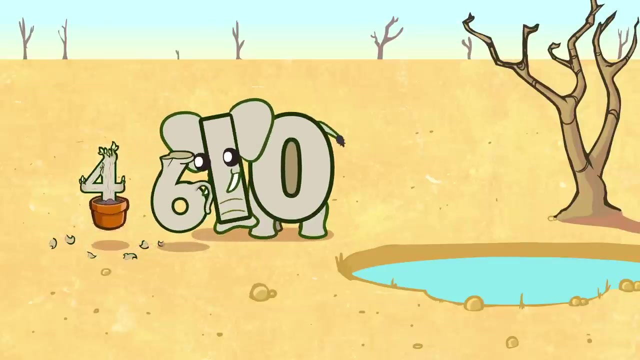 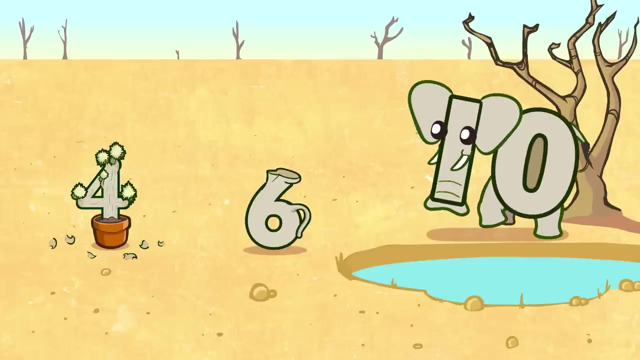 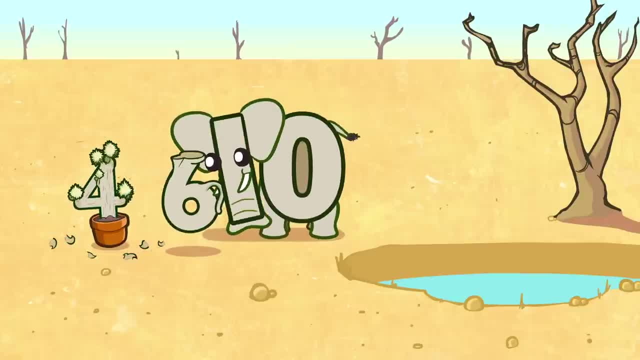 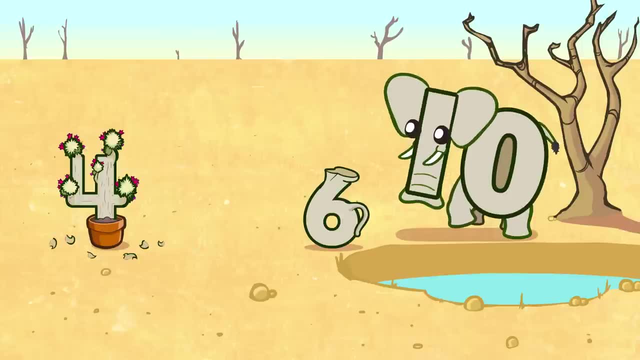 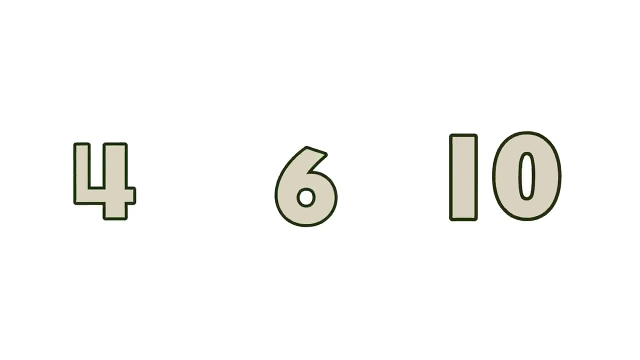 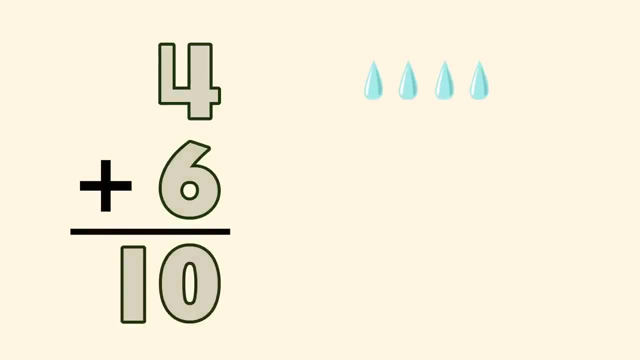 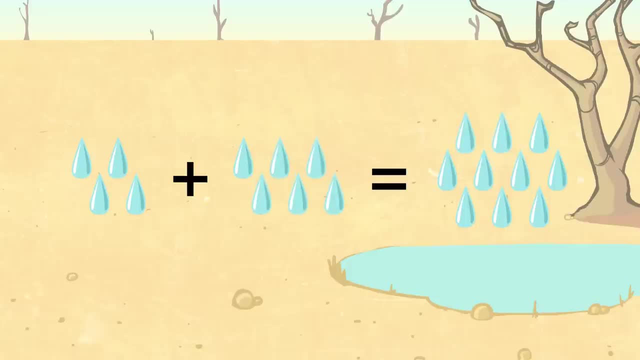 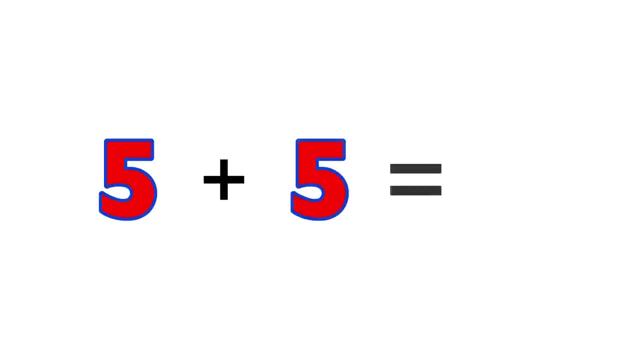 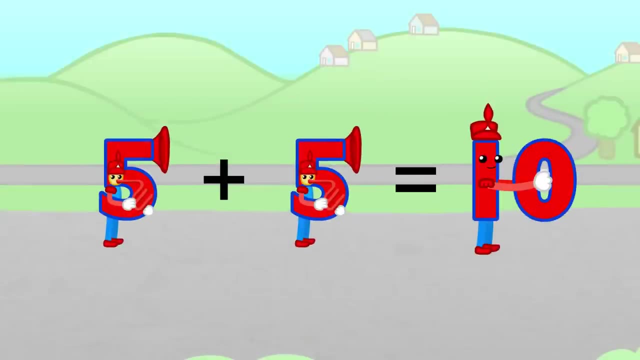 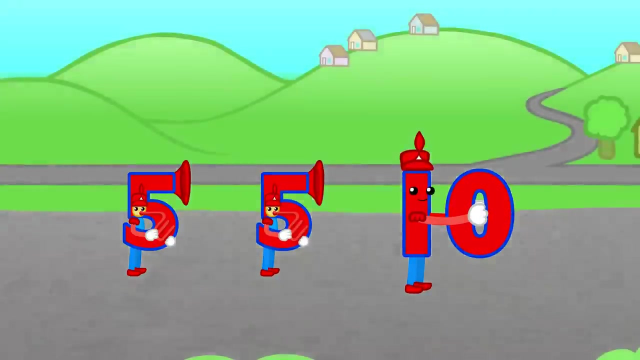 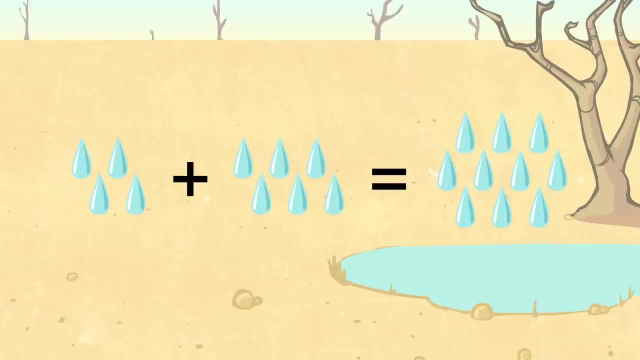 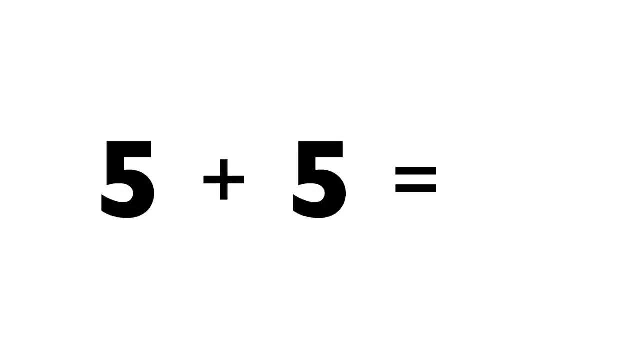 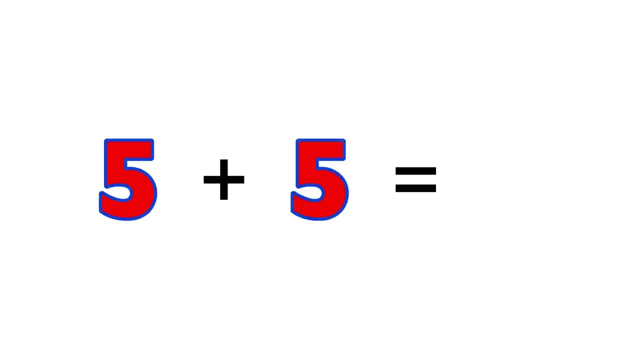 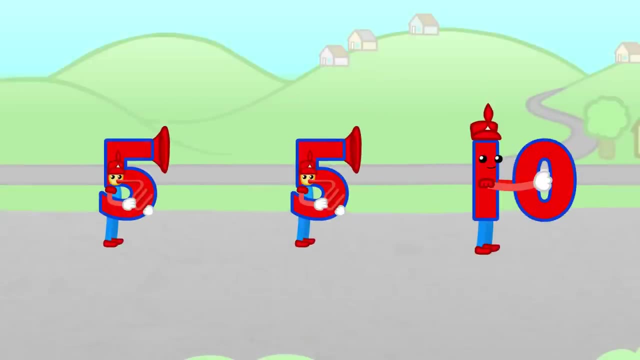 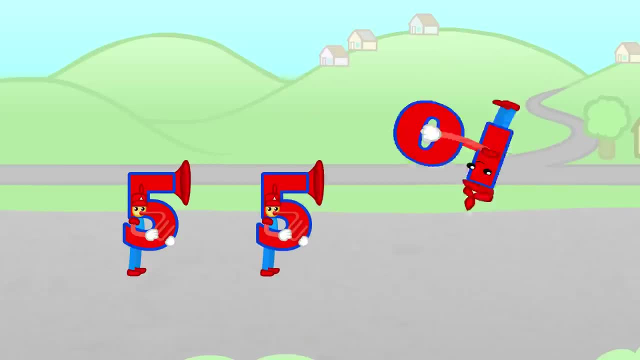 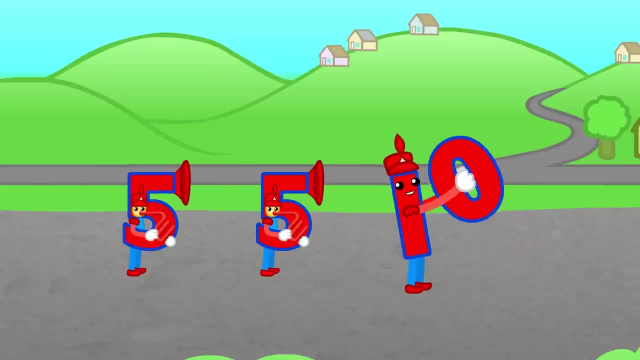 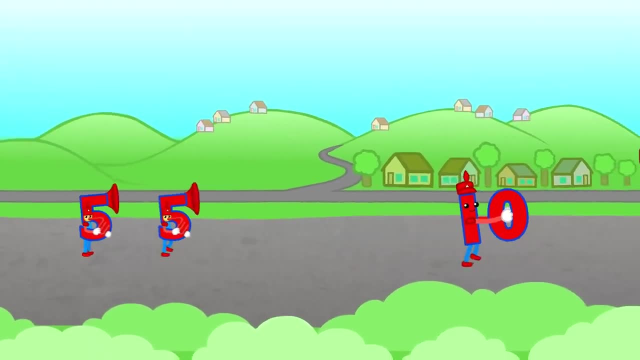 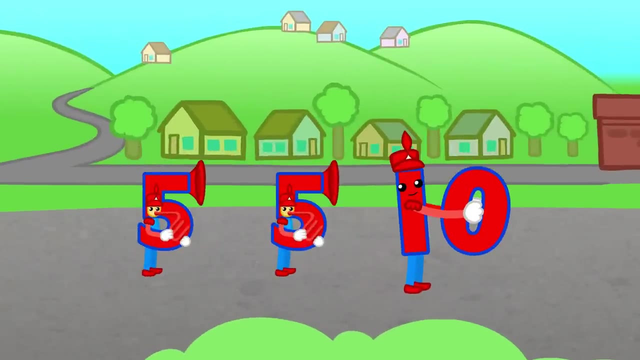 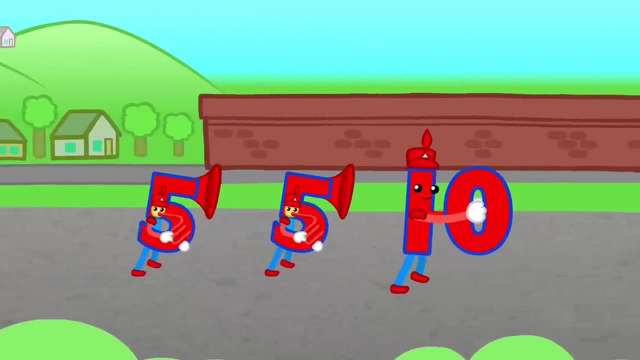 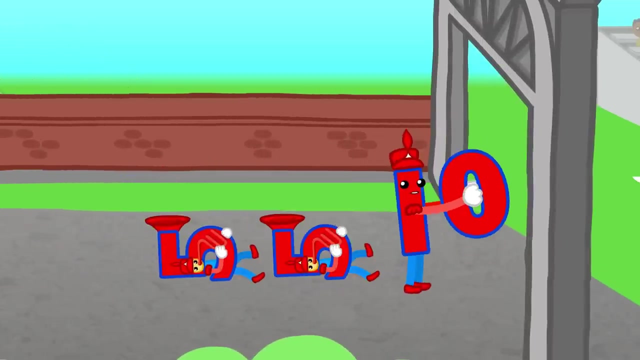 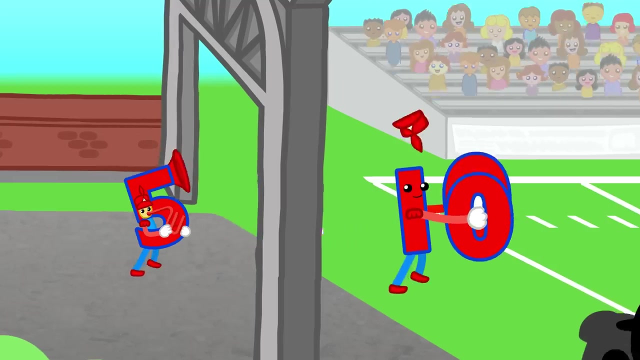 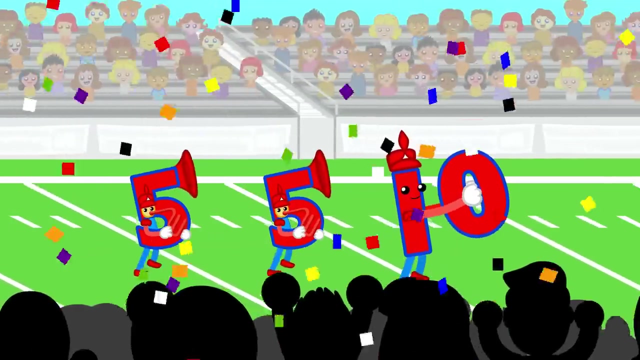 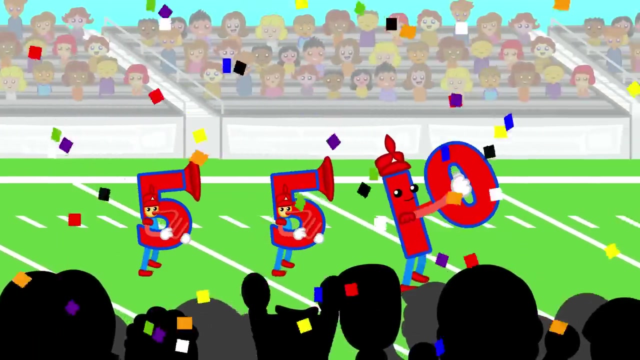 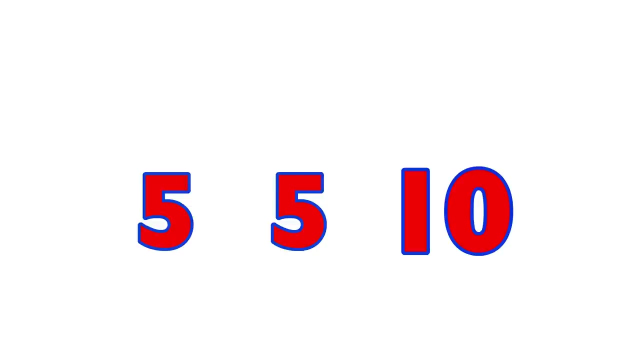 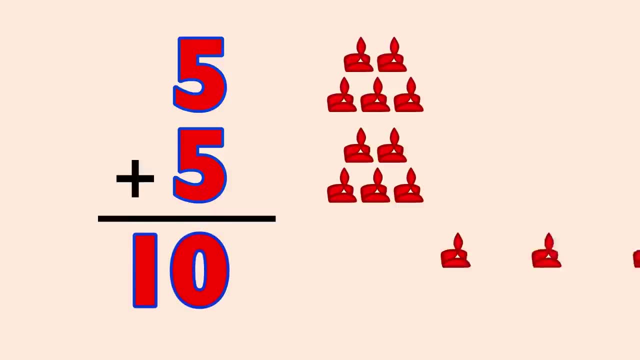 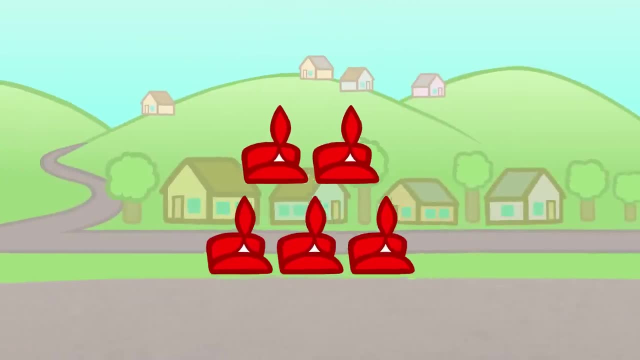 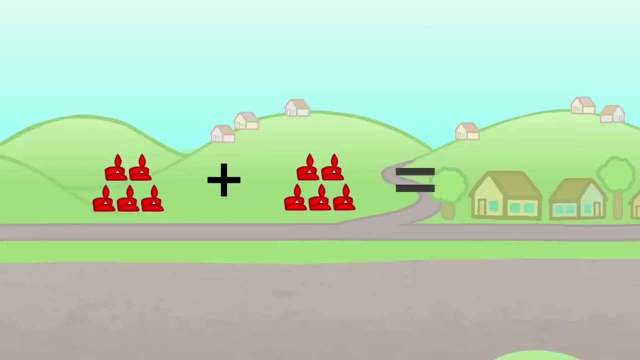 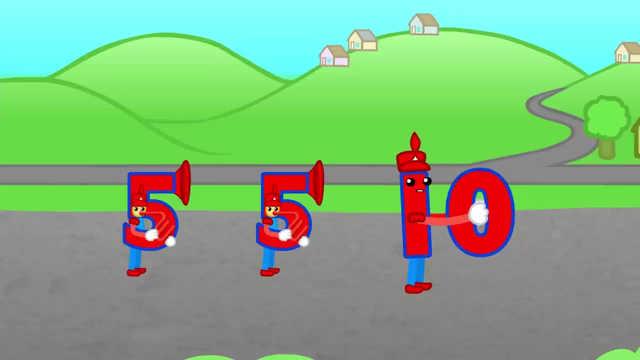 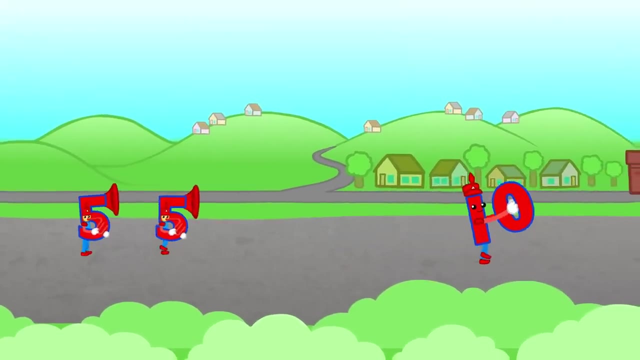 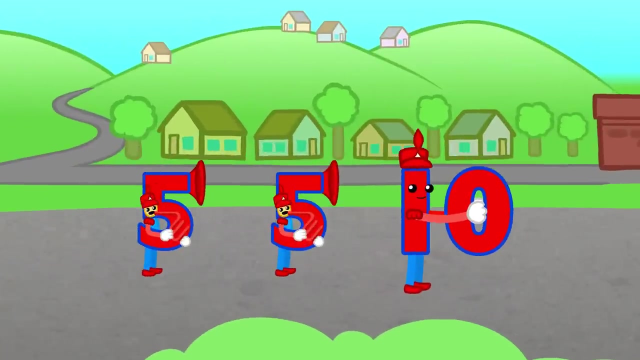 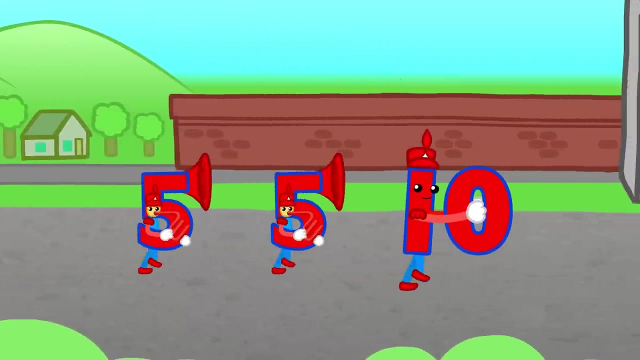 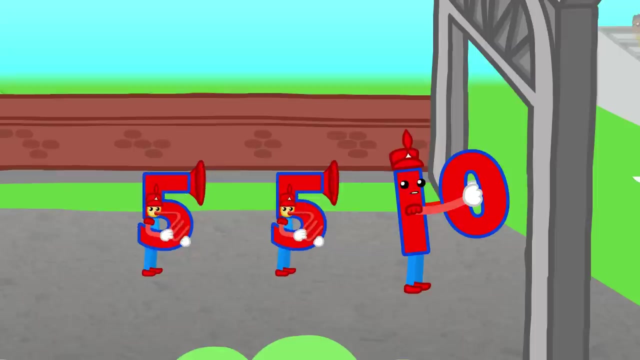 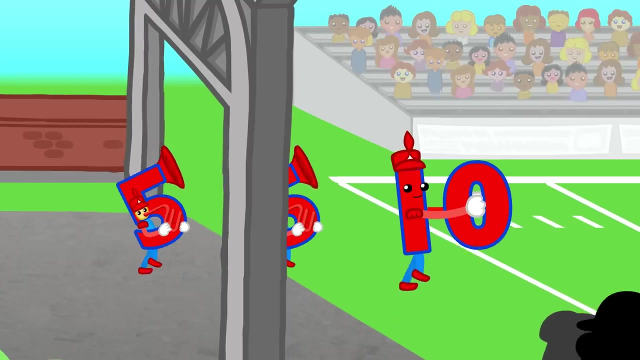 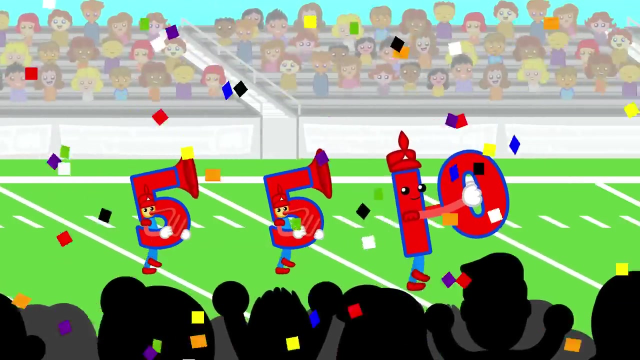 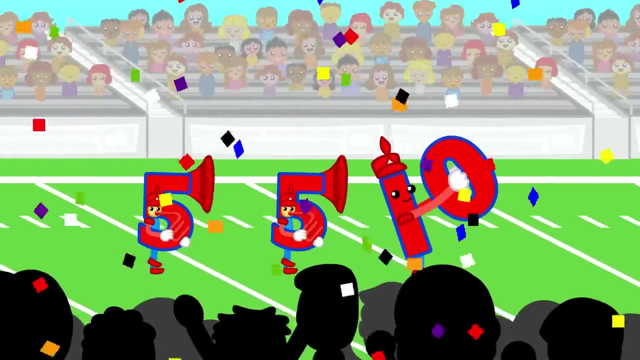 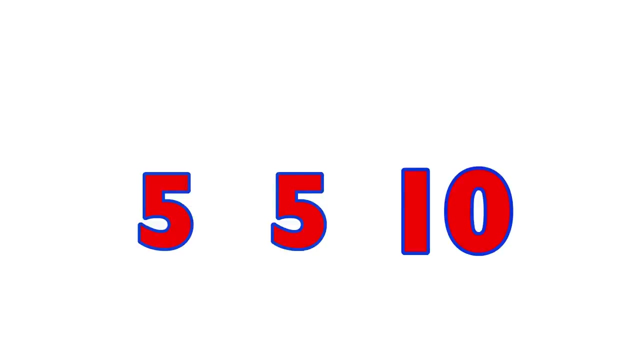 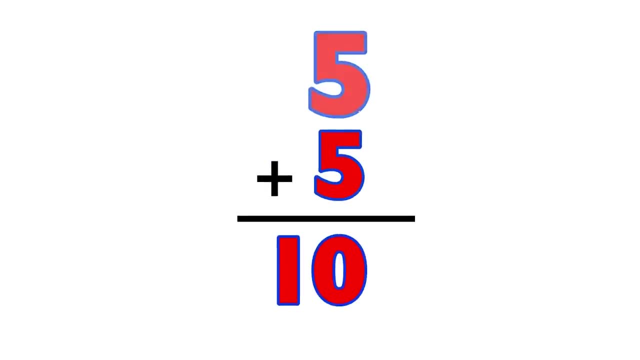 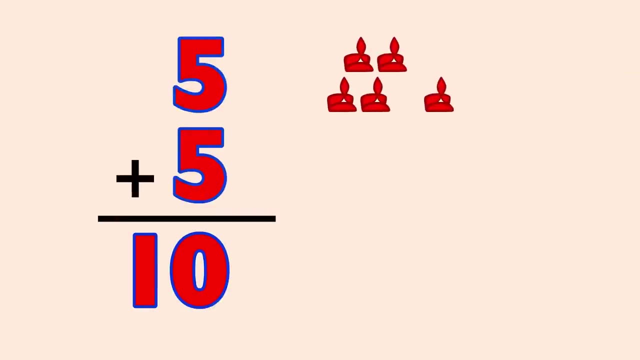 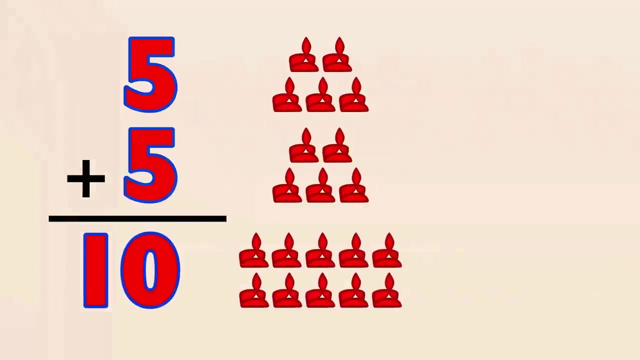 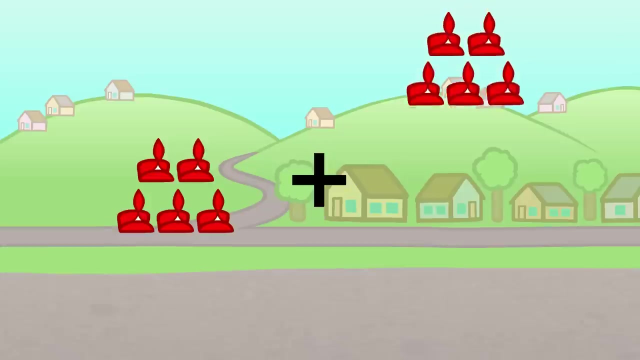 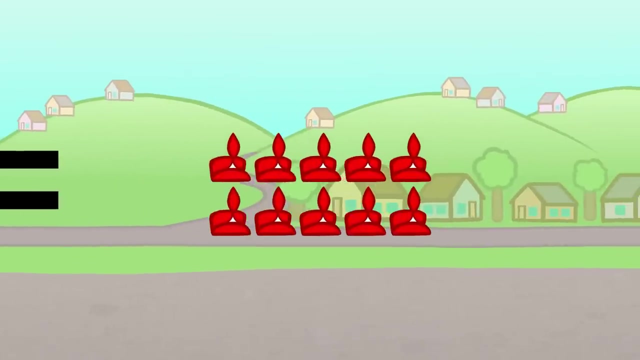 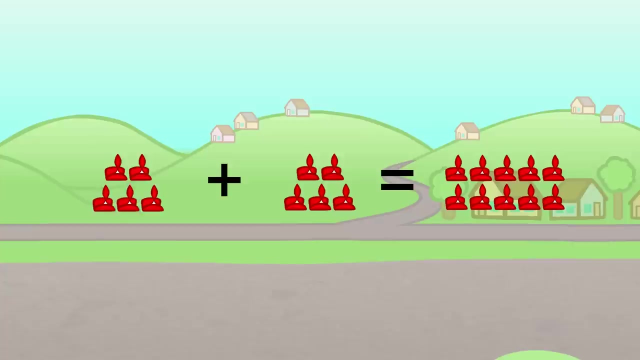 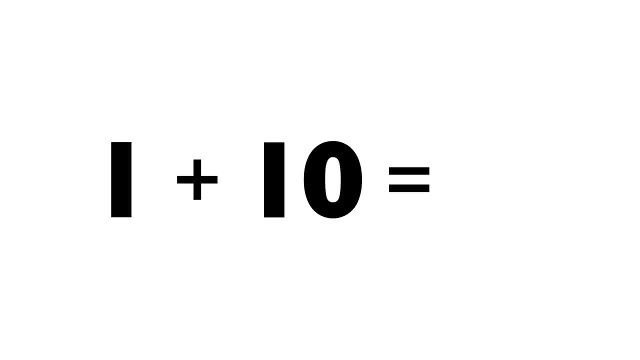 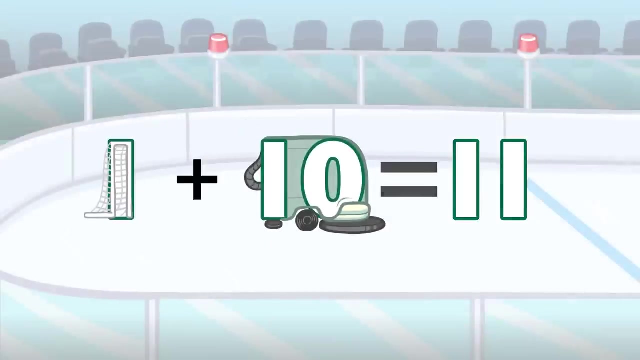 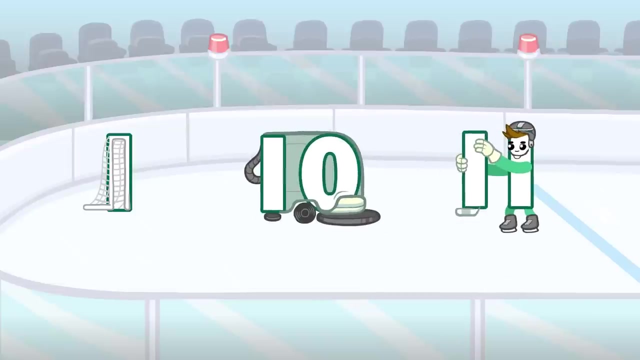 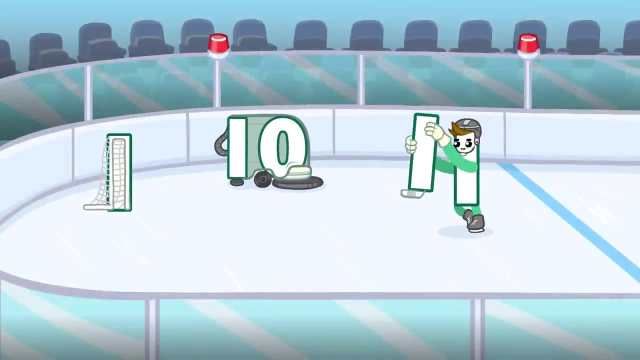 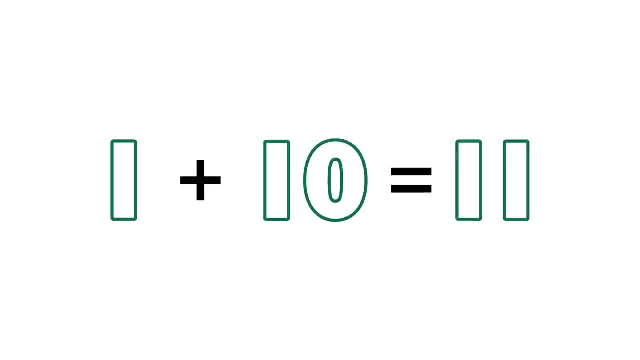 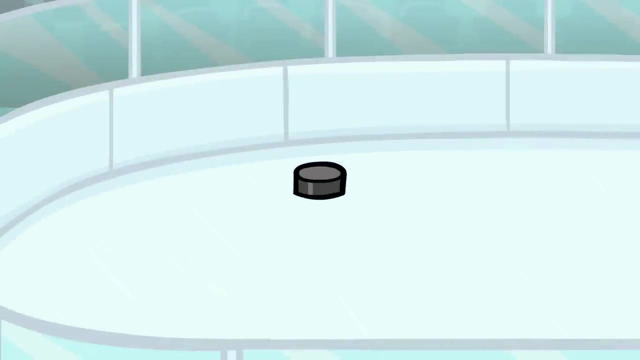 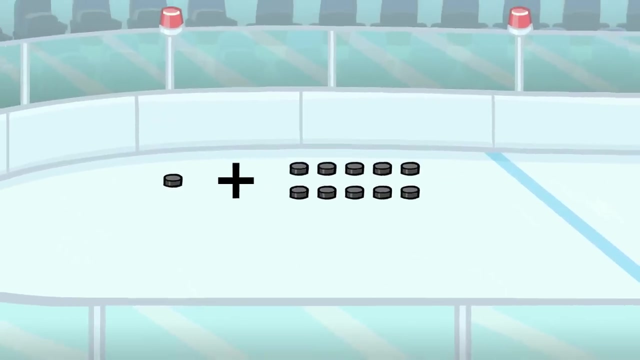 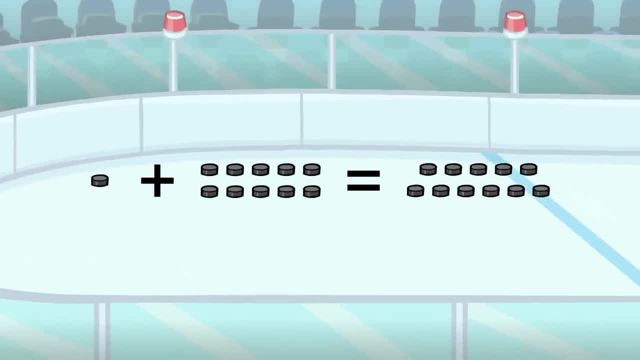 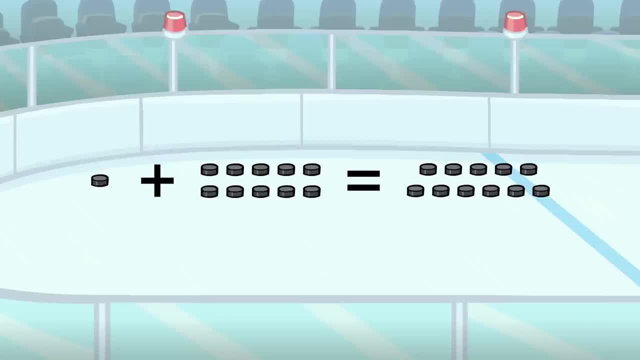 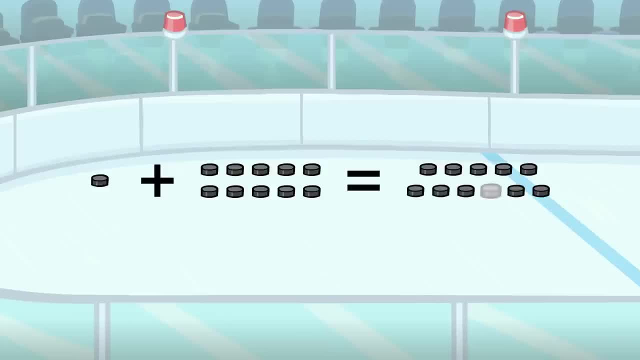 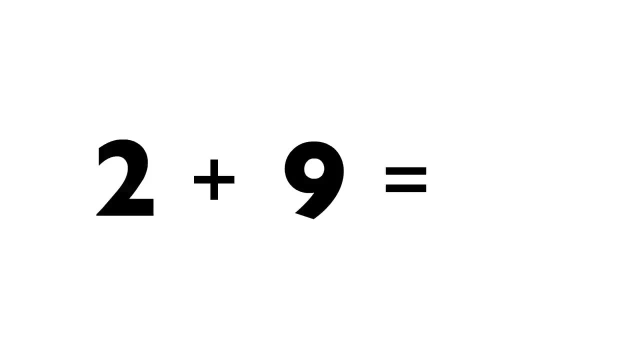 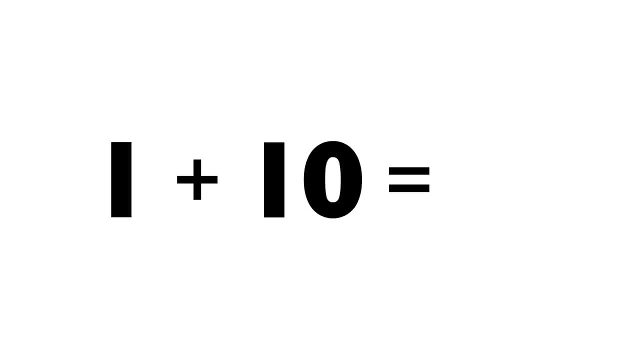 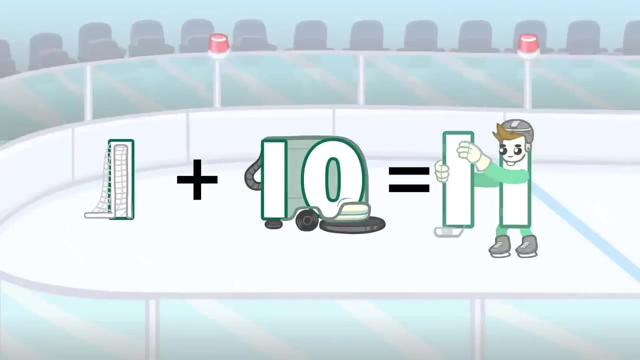 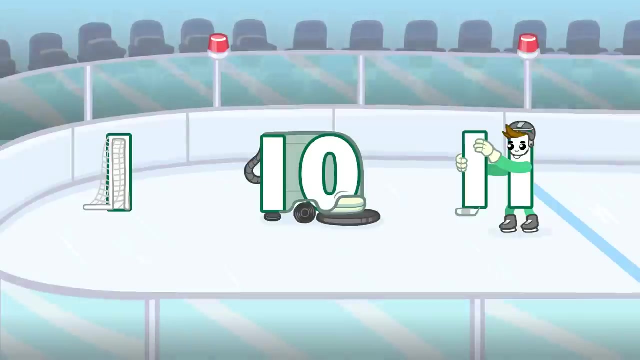 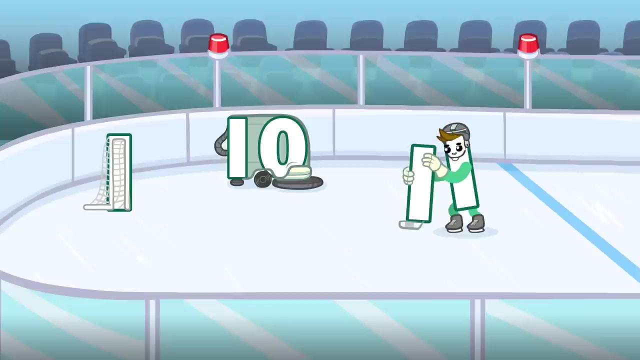 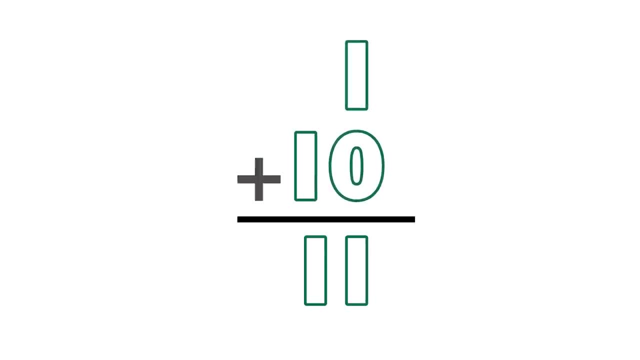 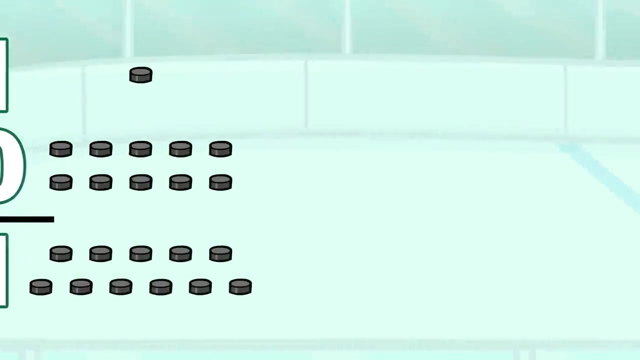 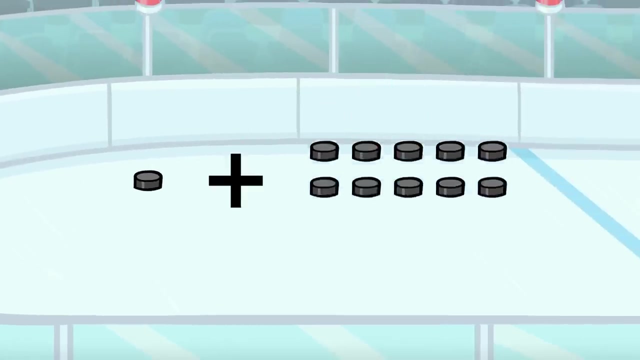 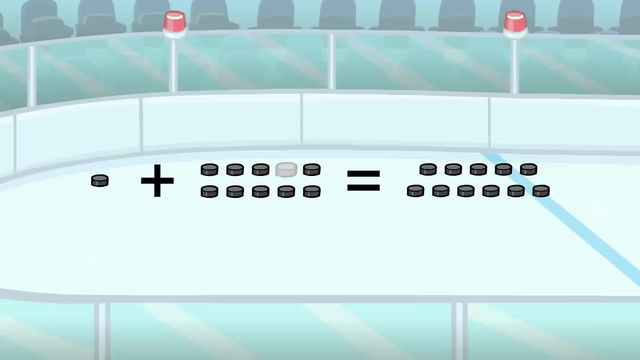 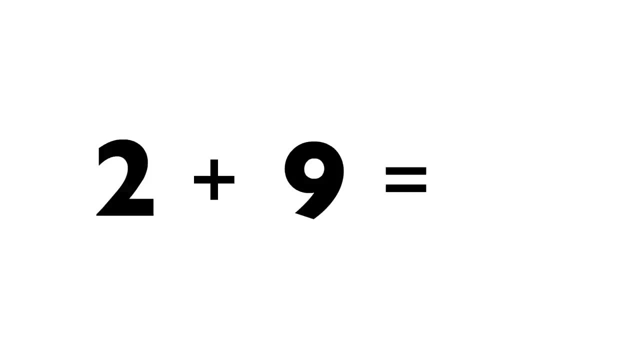 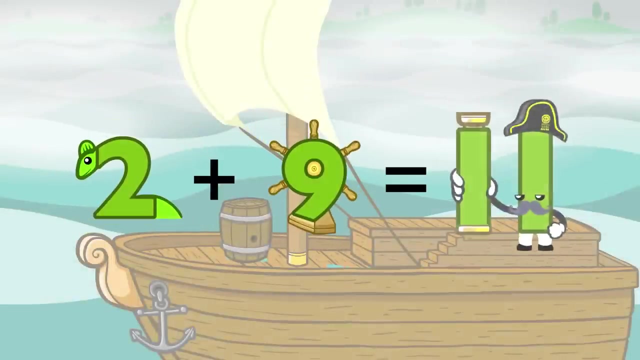 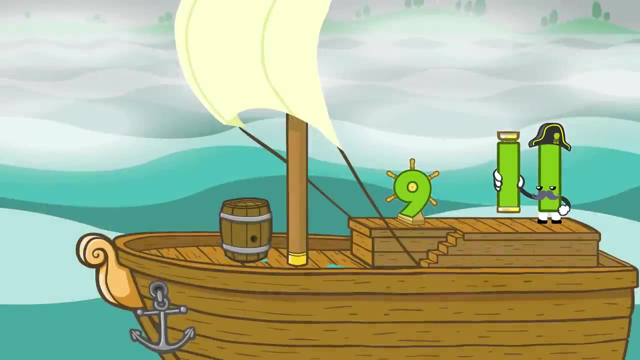 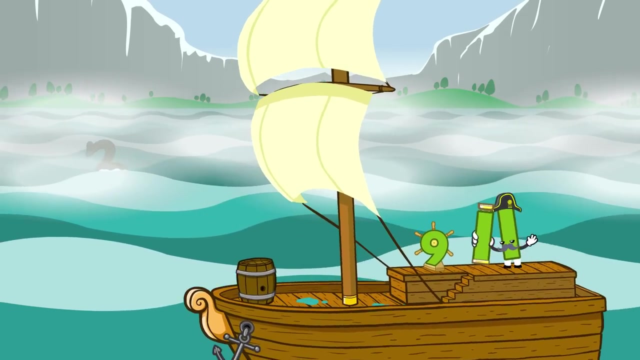 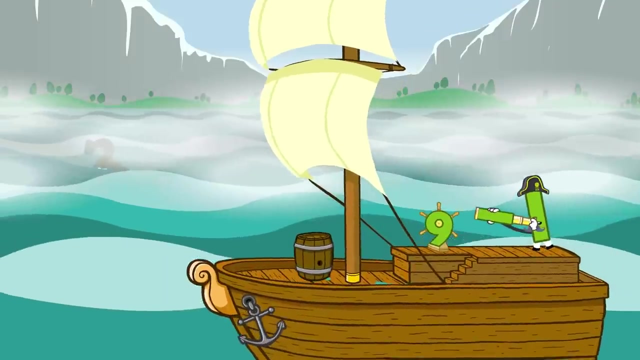 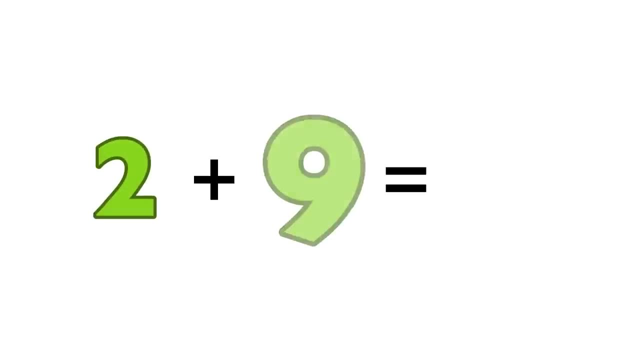 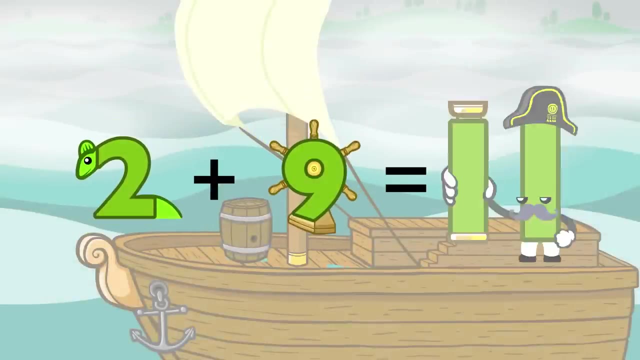 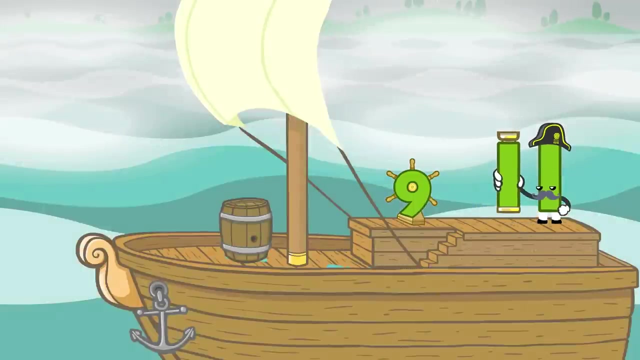 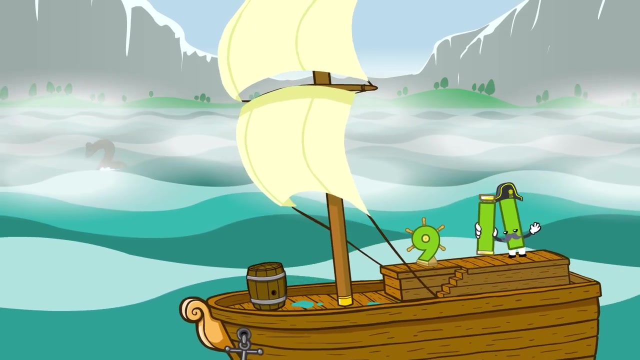 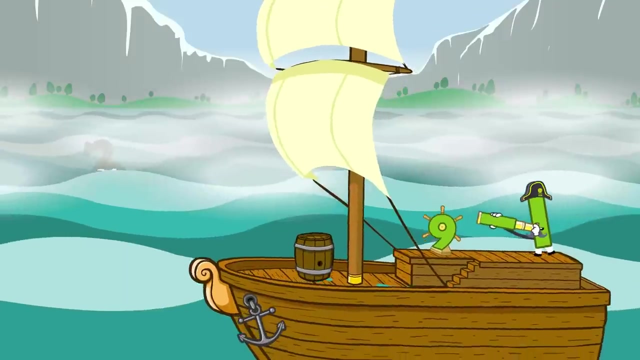 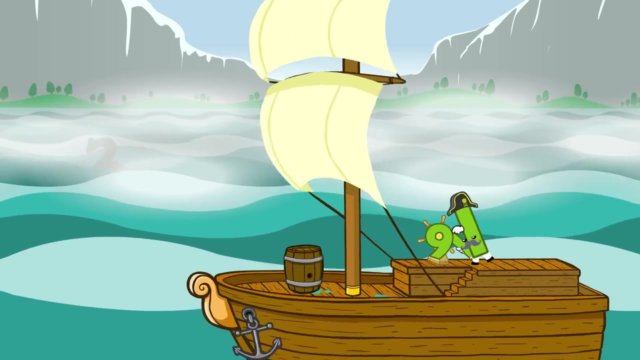 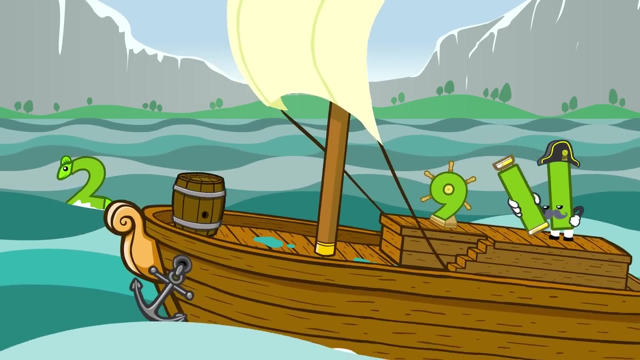 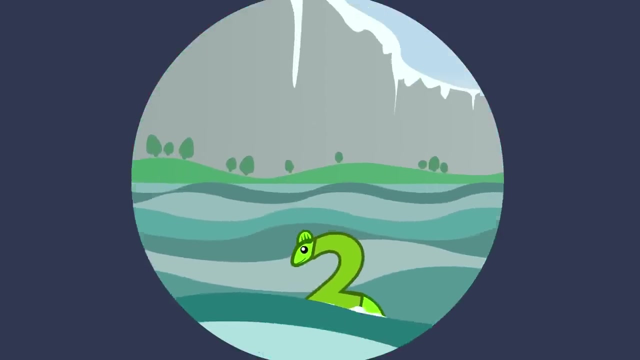 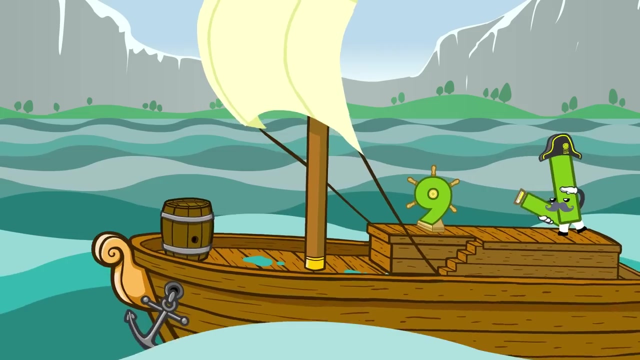 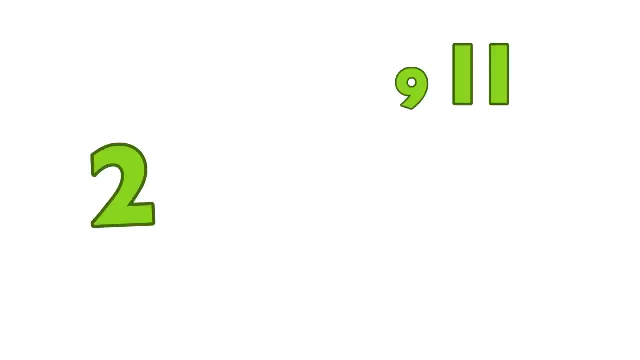 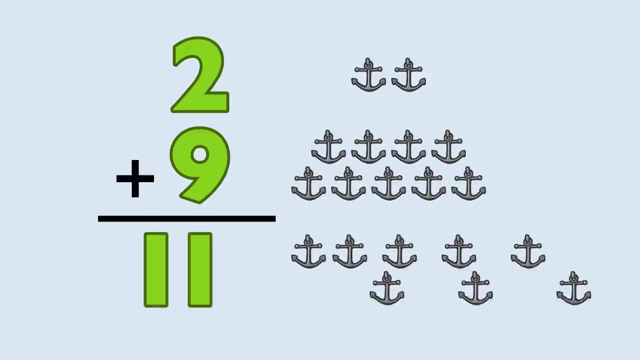 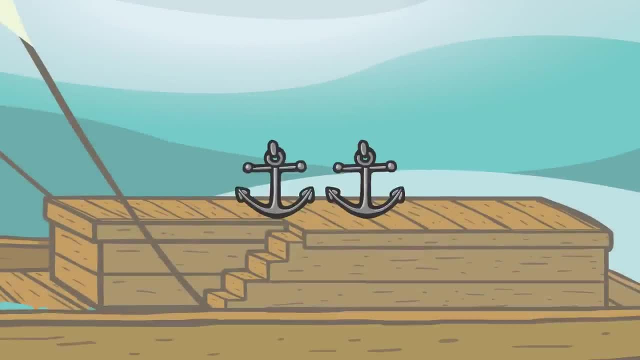 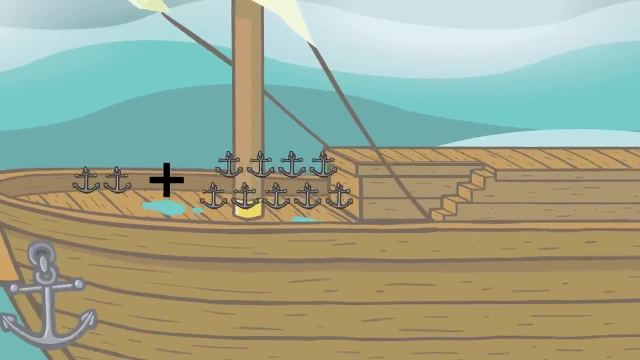 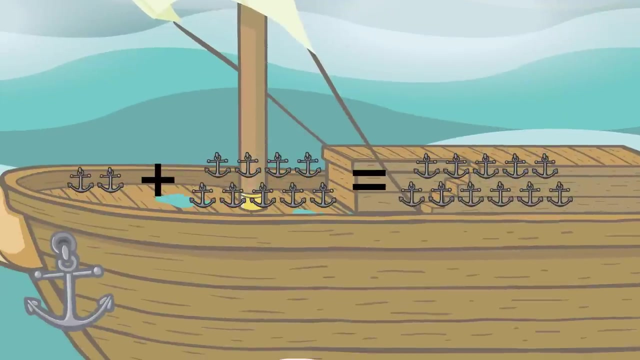 2 Plus 9 Equals 11: 1, 2, 3, 4, 5, 6, 7, 8, 9, 10, 11 Equals 1, 2, 3, 4, 5, 6, 7, 8, 9, 10. 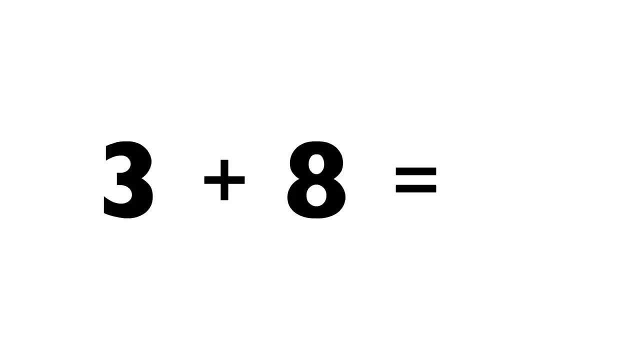 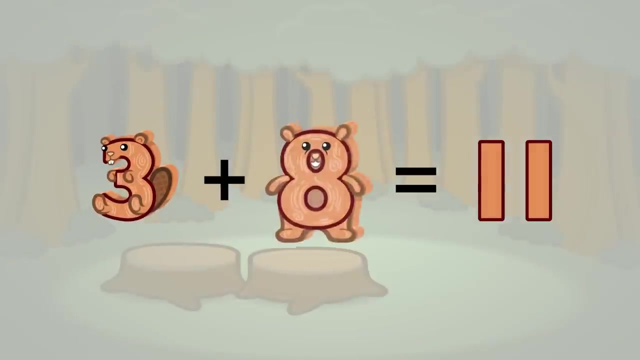 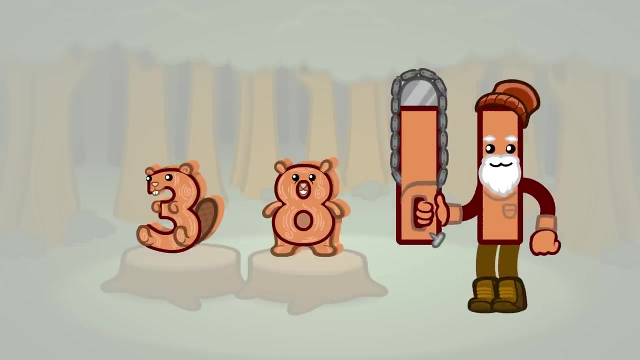 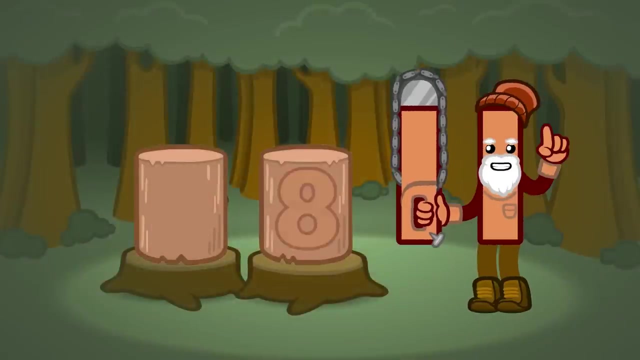 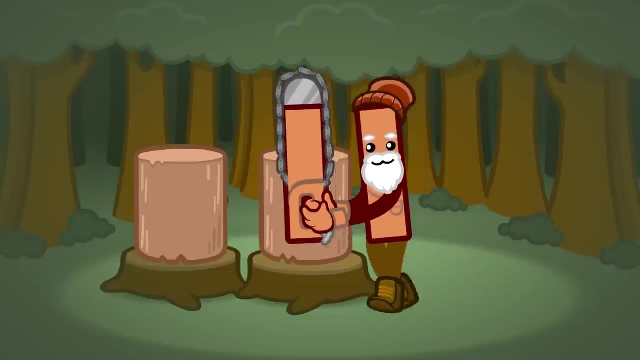 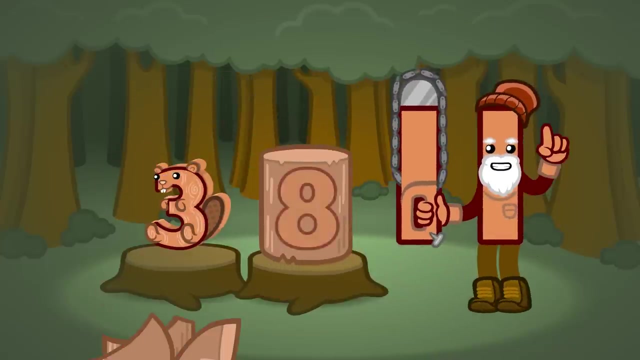 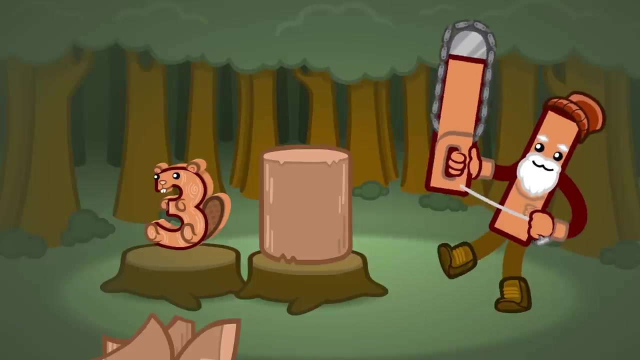 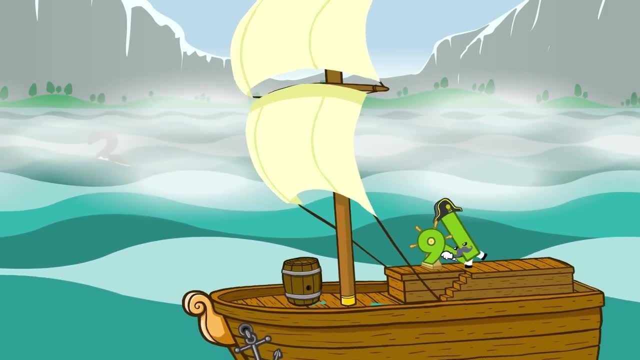 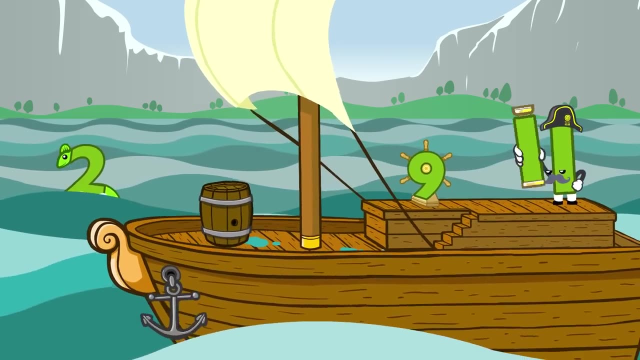 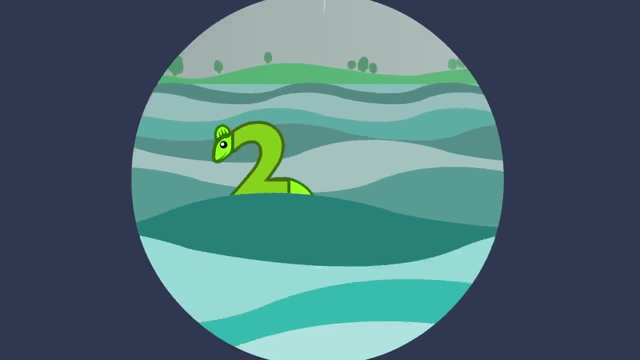 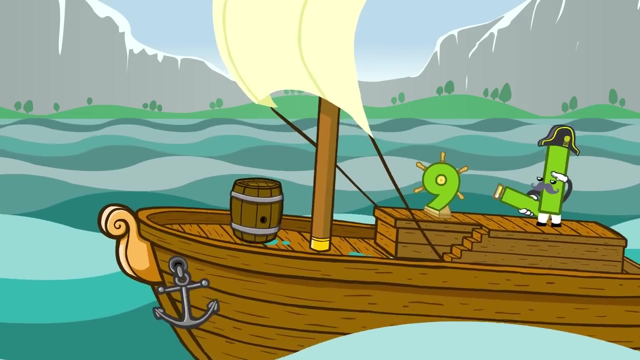 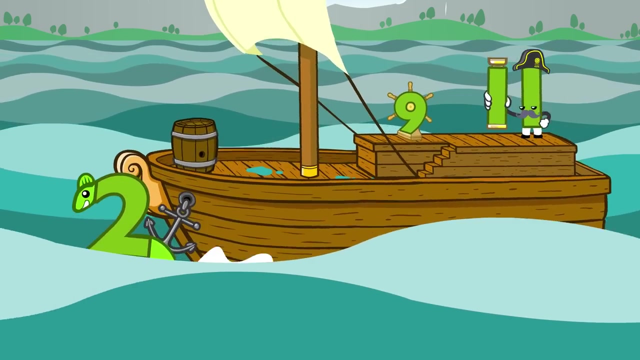 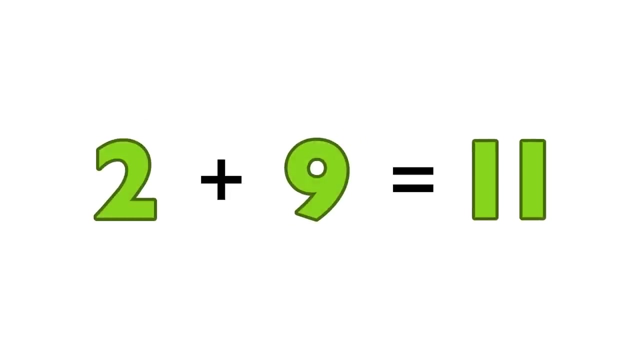 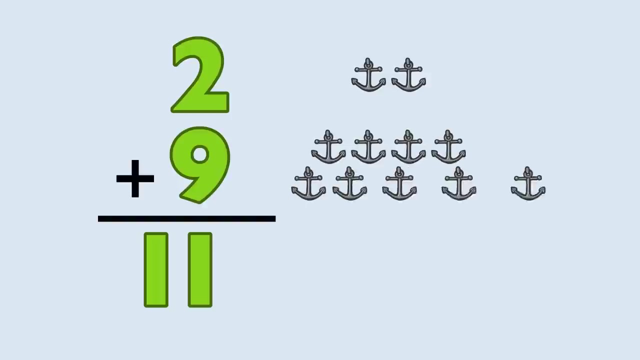 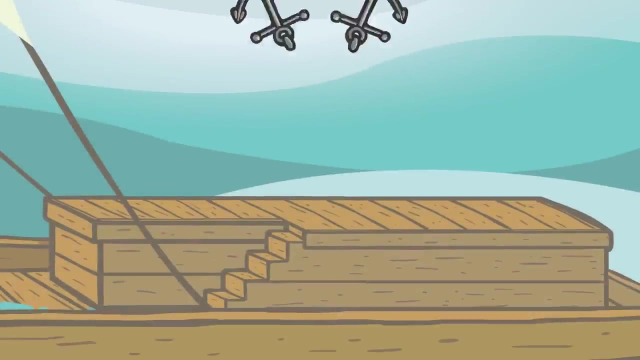 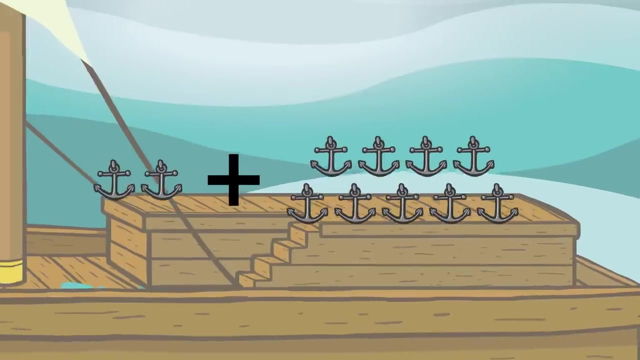 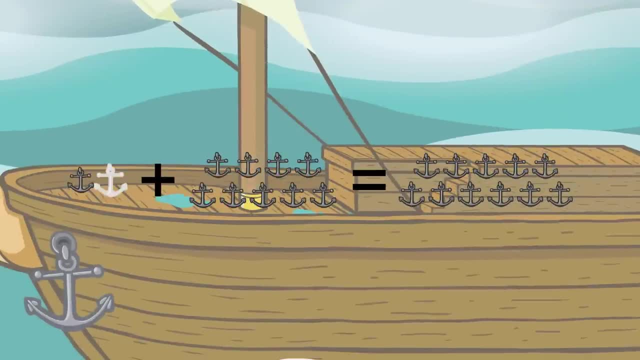 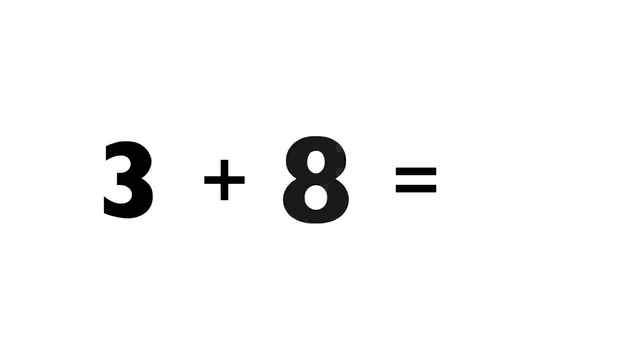 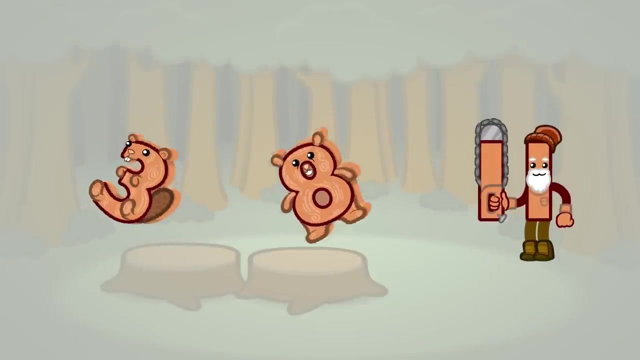 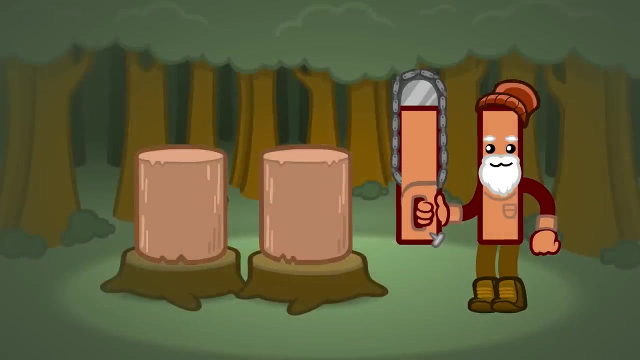 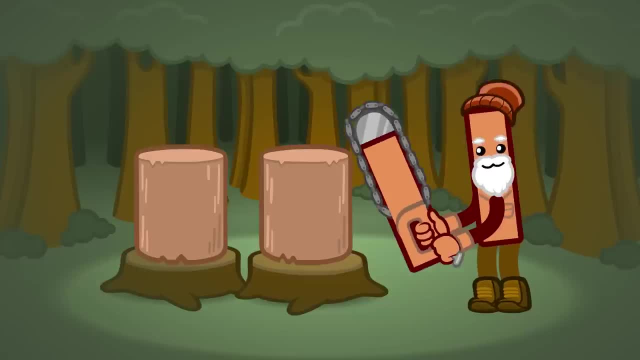 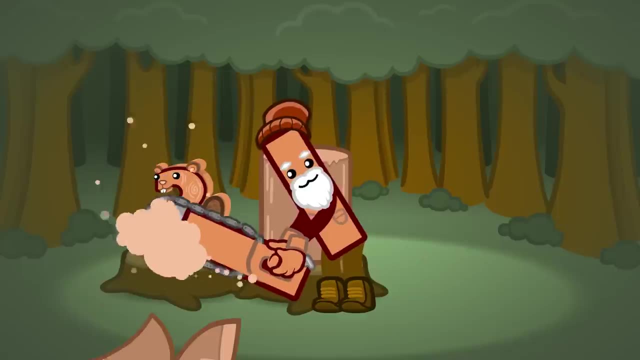 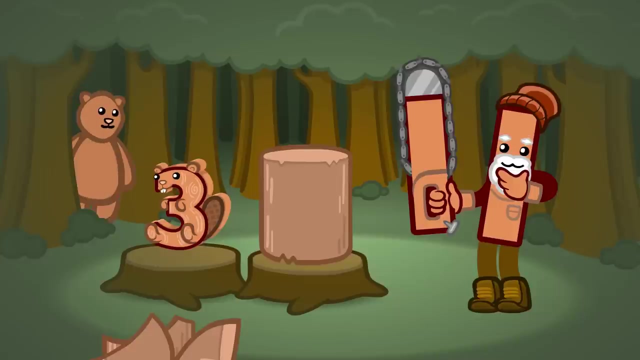 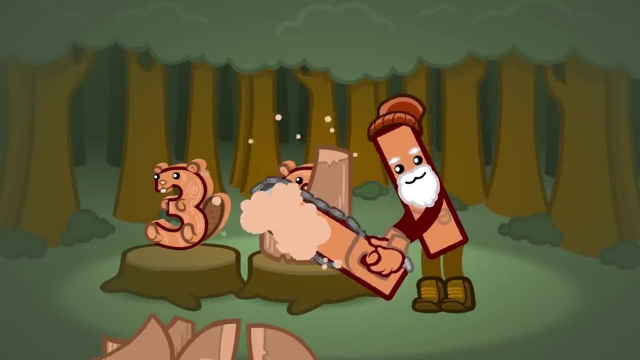 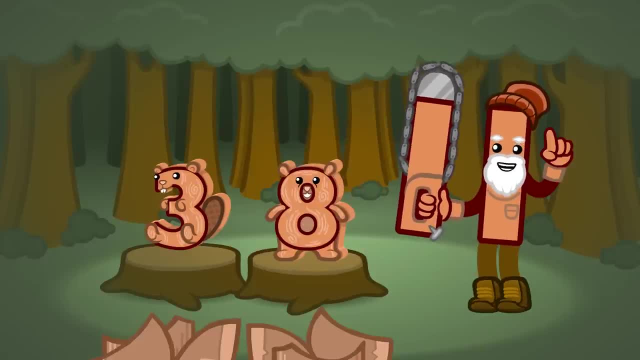 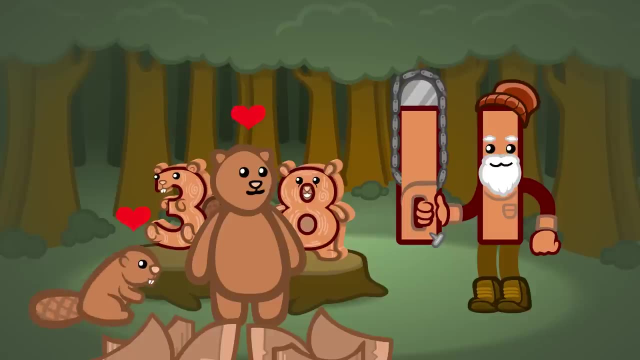 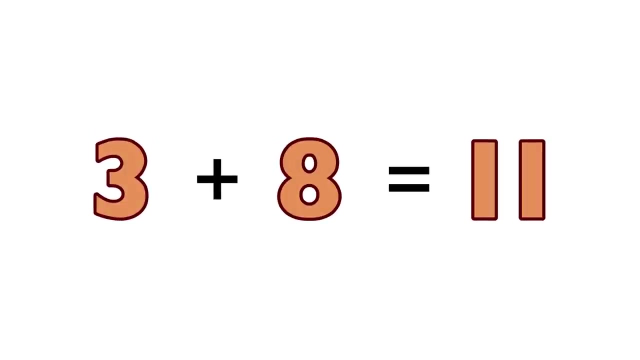 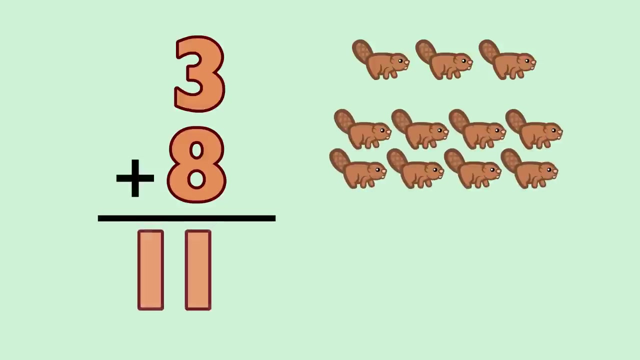 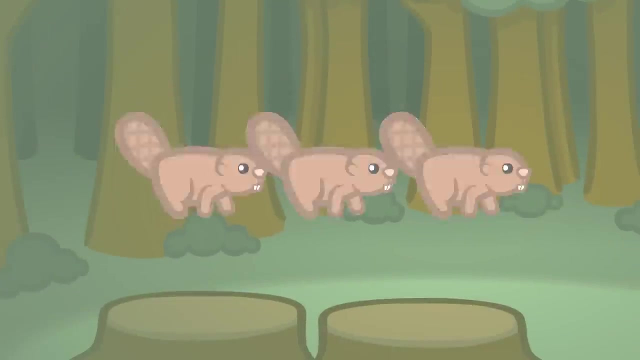 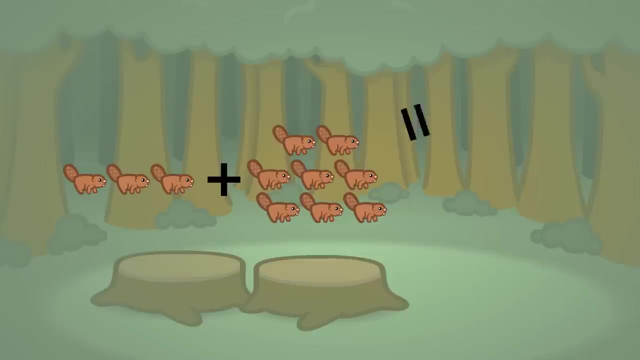 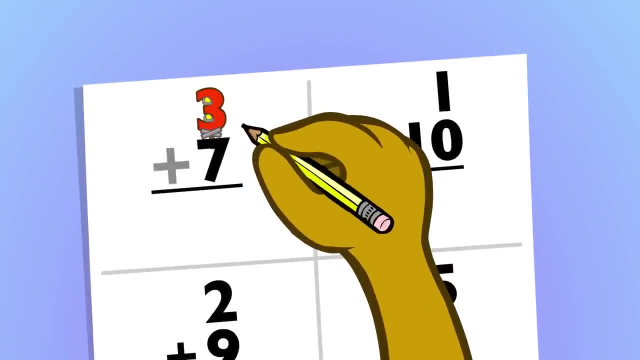 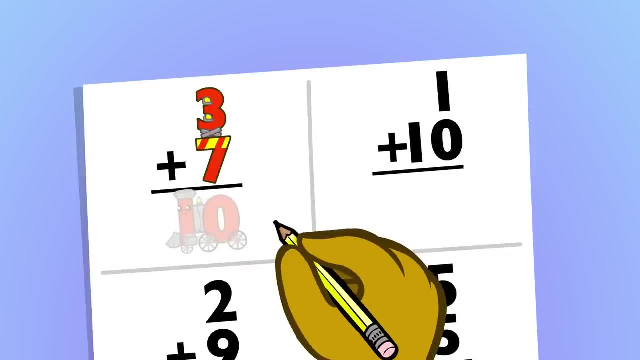 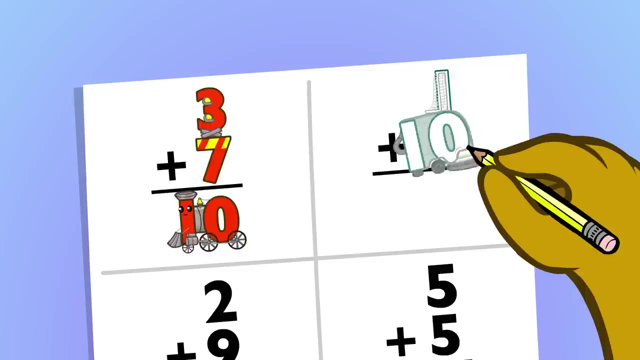 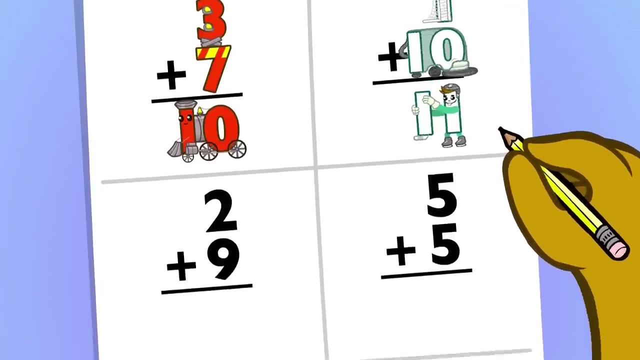 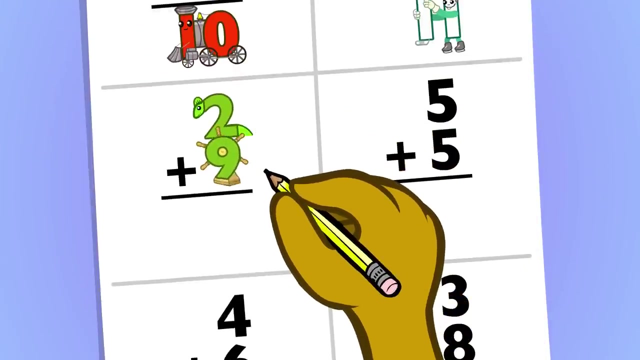 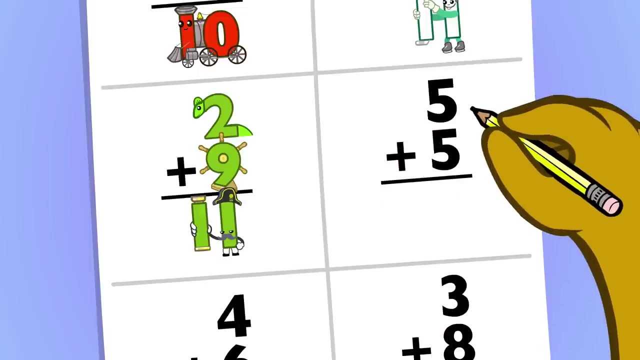 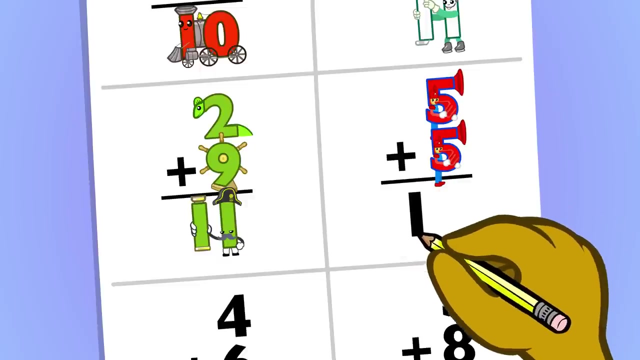 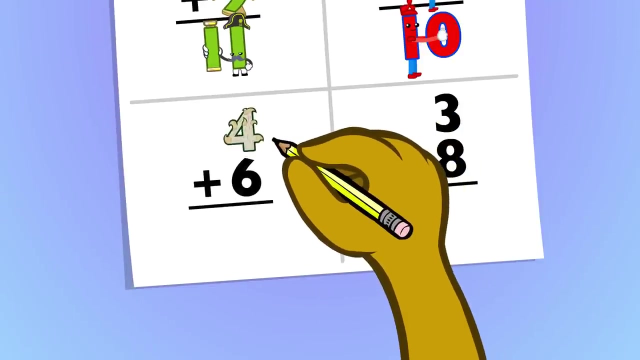 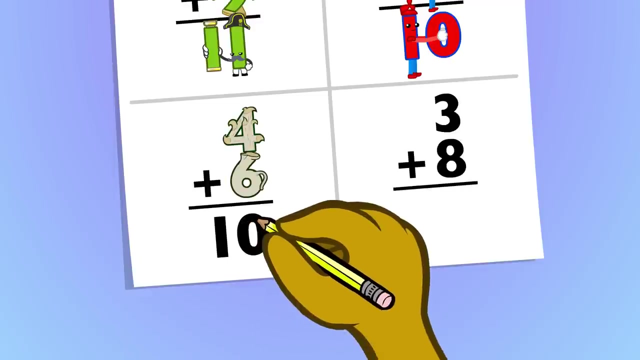 3 plus 7 equals 10.. 1 plus 10 equals 10.. 11.. 2 plus 9 equals 11.. 5 plus 5 equals 10.. 4 plus 6 equals 10. 10.. 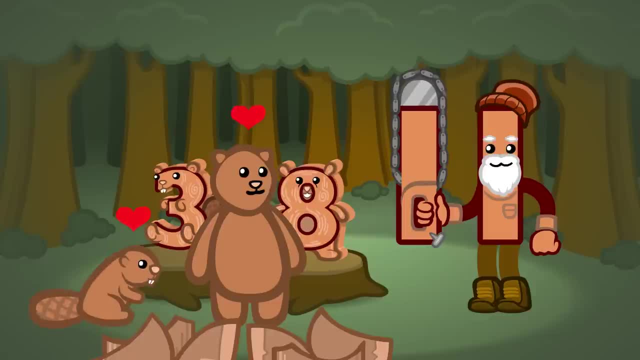 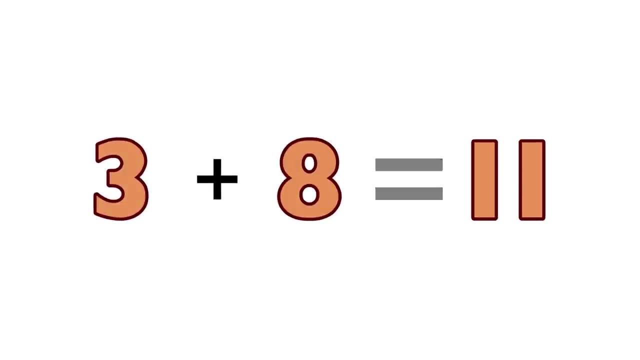 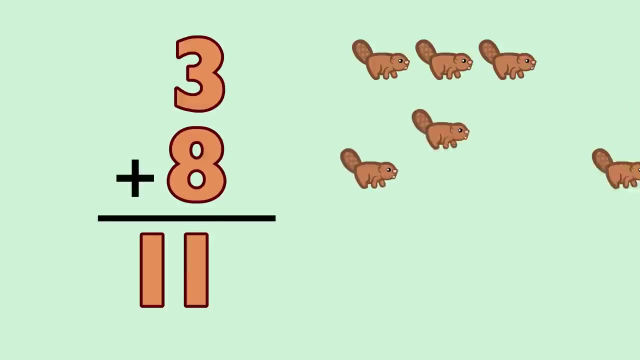 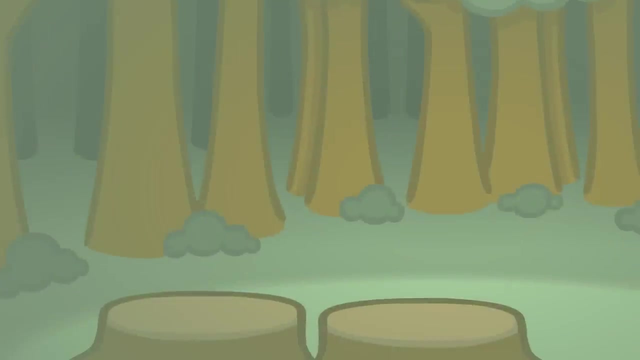 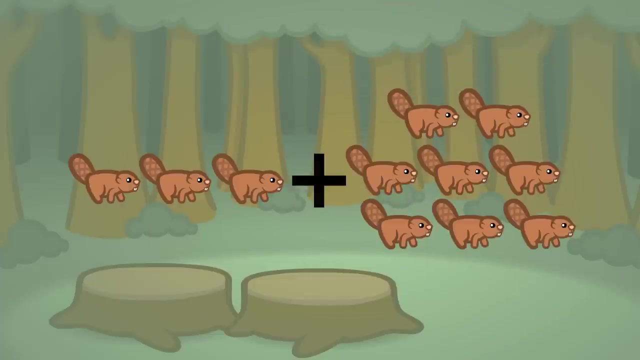 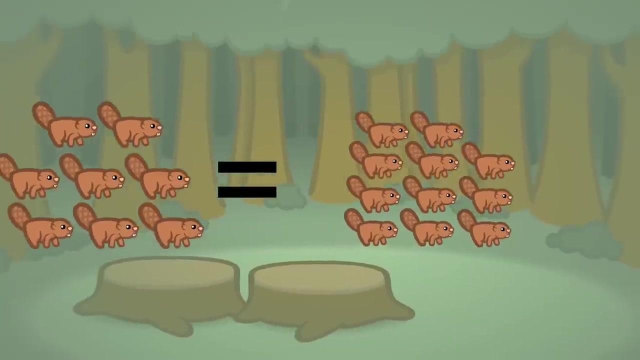 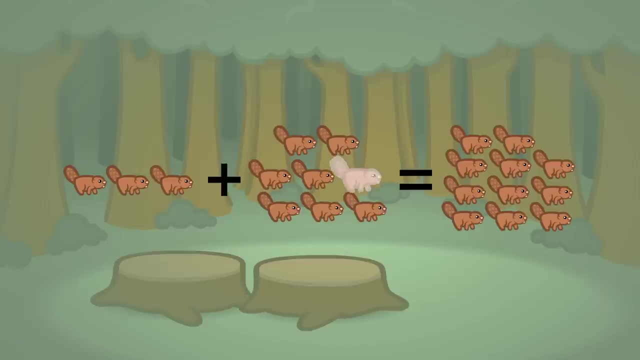 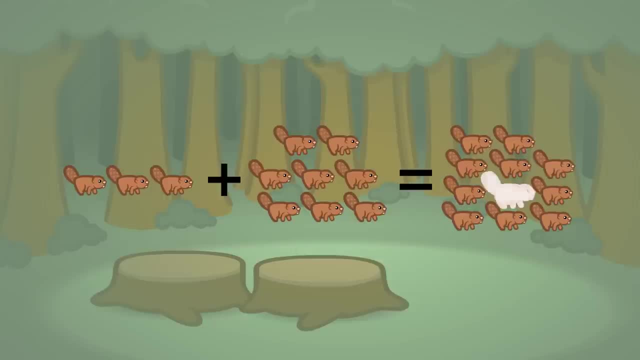 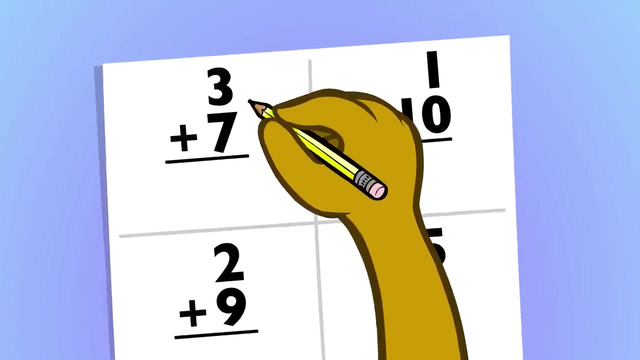 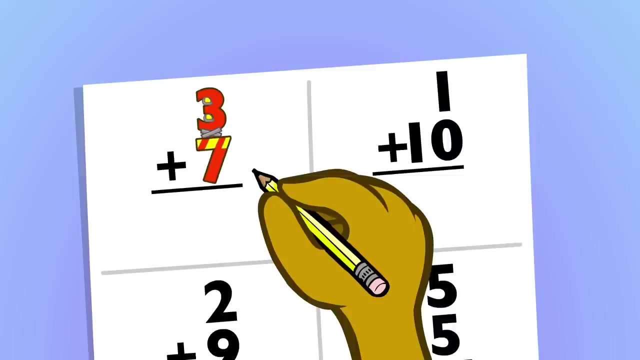 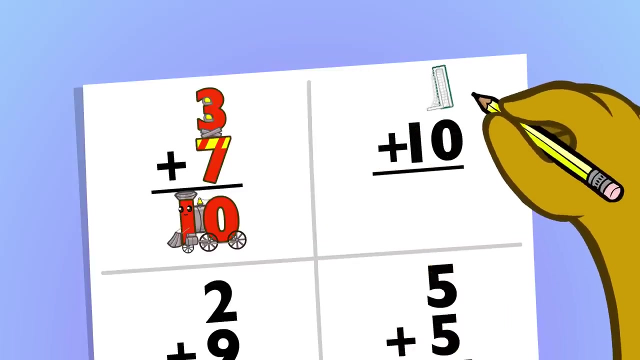 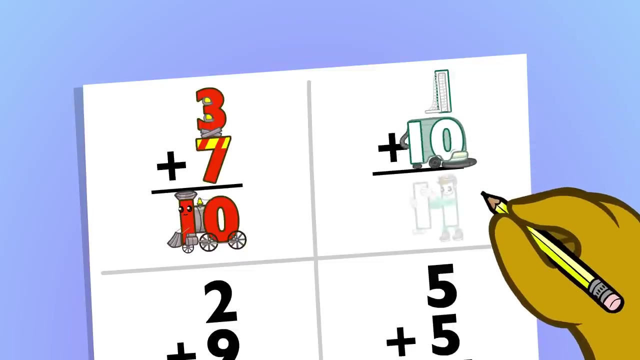 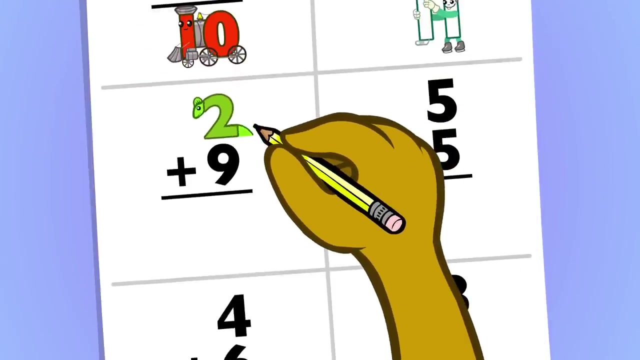 1,, 2,, 3,, 4,, 5,, 6,, 7,, 8,, 9,, 10, 11. 3 plus 7 equals 10. 1 plus 10 equals 11. 2, 3,, 4,, 5,, 6,, 7,, 8,, 9,, 10, 11. 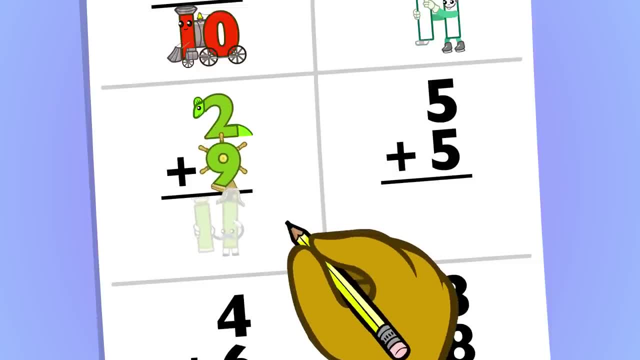 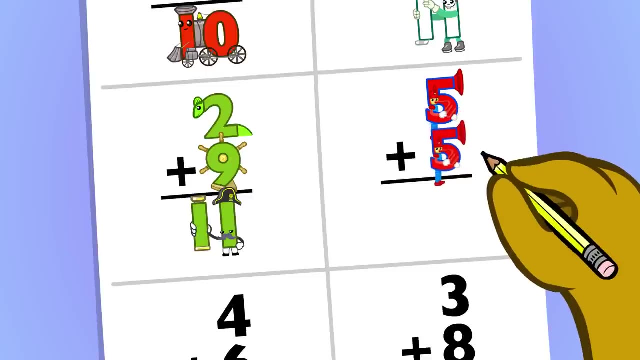 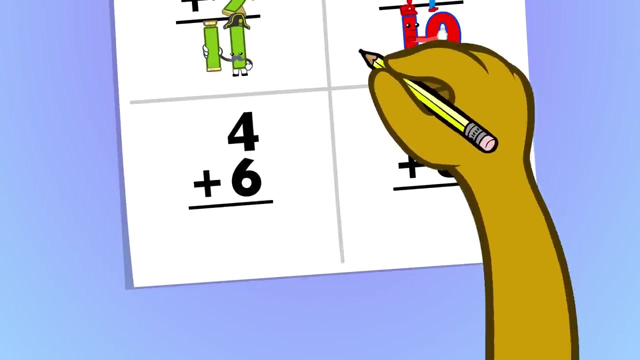 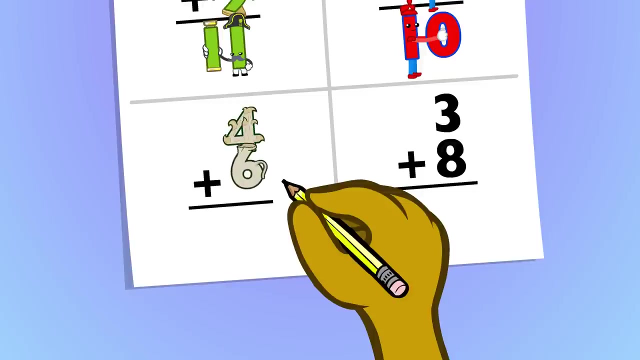 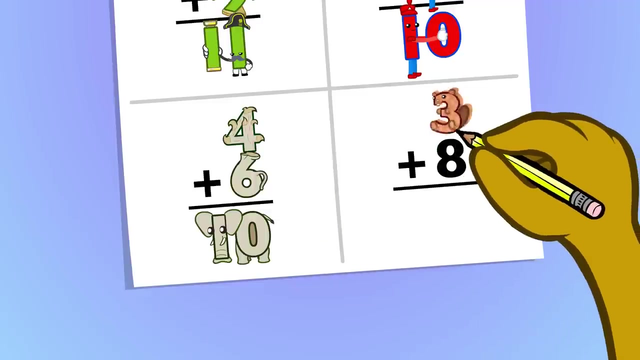 equals 1,, 2,, 3,, 4,, 5,, 6,, 7,, 8,, 9,, 10, 11. equals 1,, 2,, 3,, 4,, 5,, 6,, 7,, 8,, 9,, 10, 11. 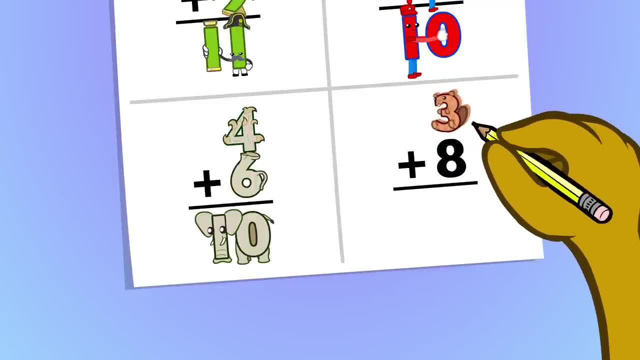 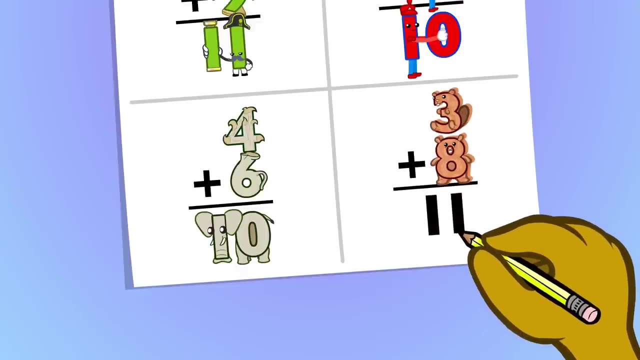 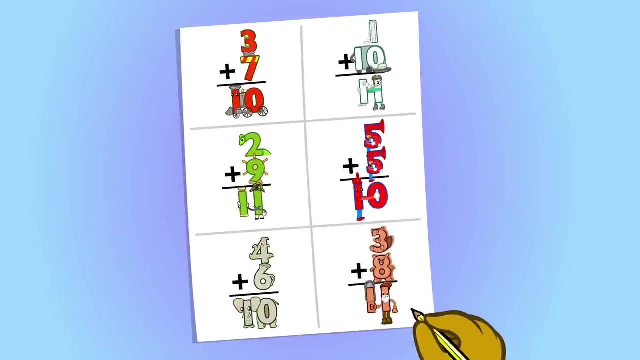 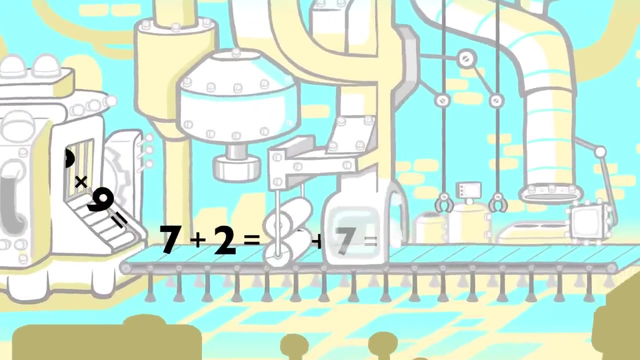 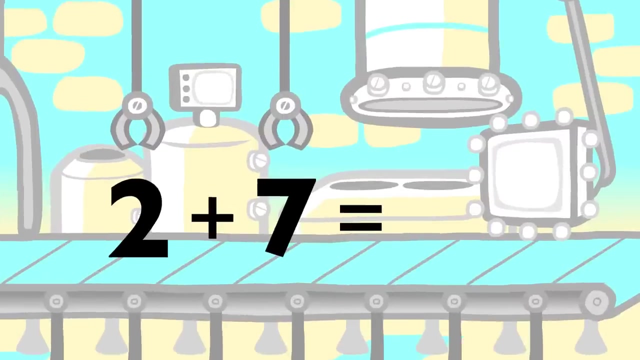 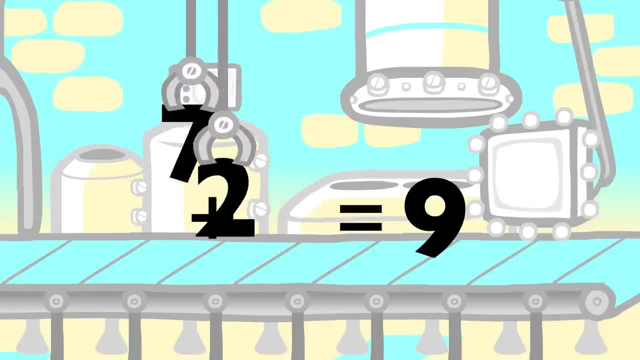 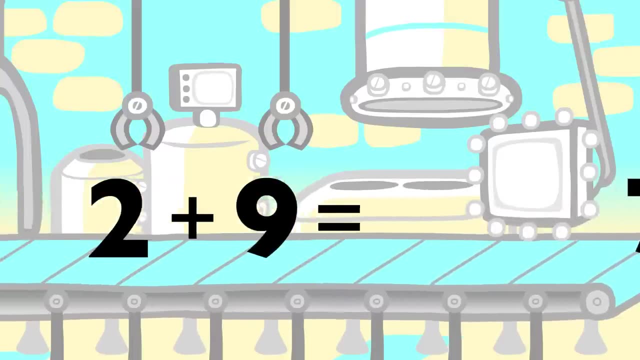 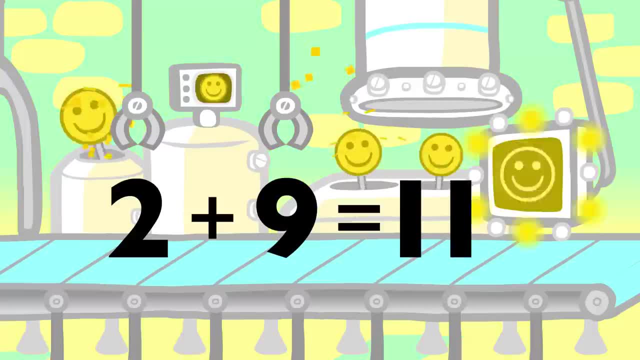 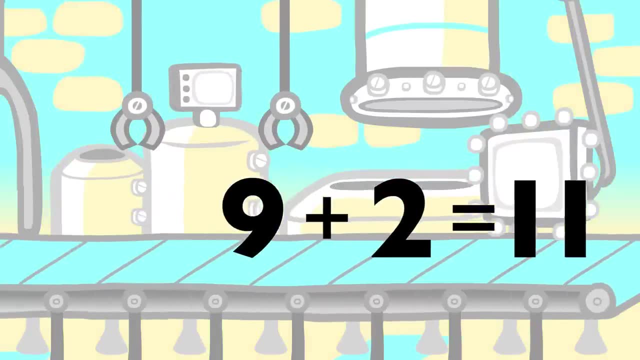 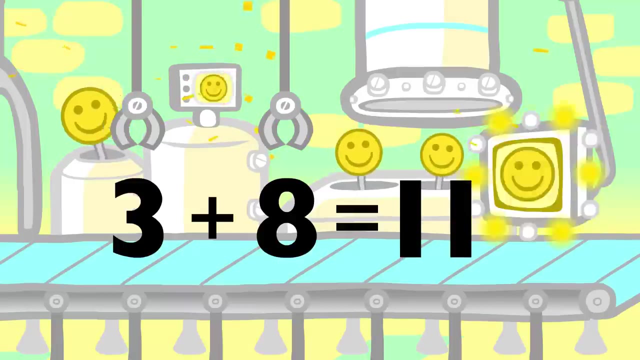 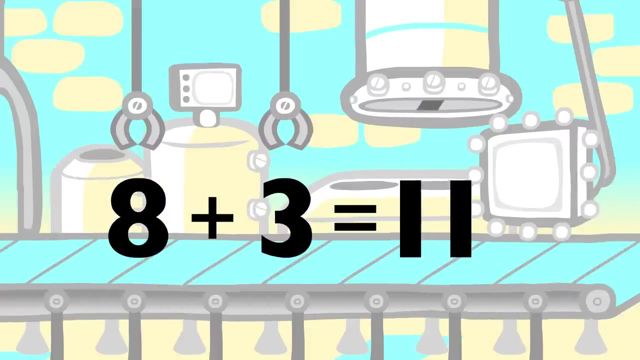 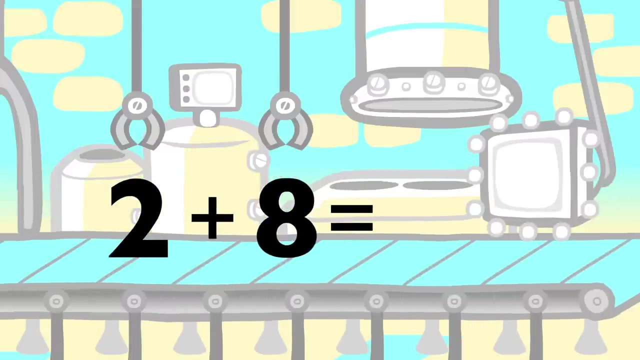 9 equals 11. And 9 plus 2 equals 11.. 3 plus 8 equals 11. And 8 plus 3 equals 11.. 2 plus 8 equals 10. And 8 plus 2 equals 10.. 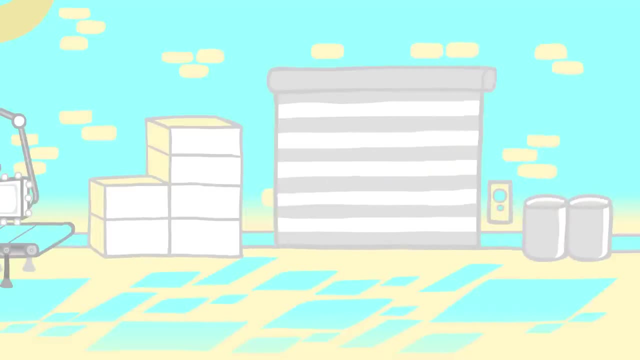 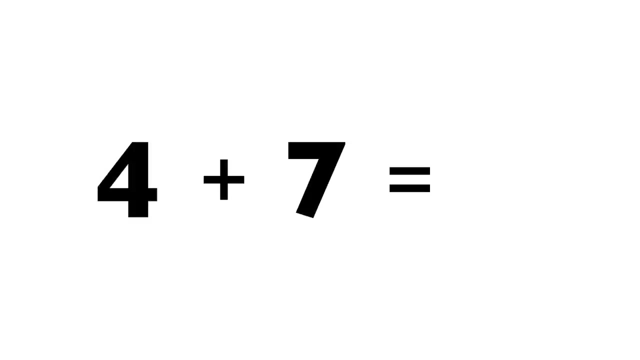 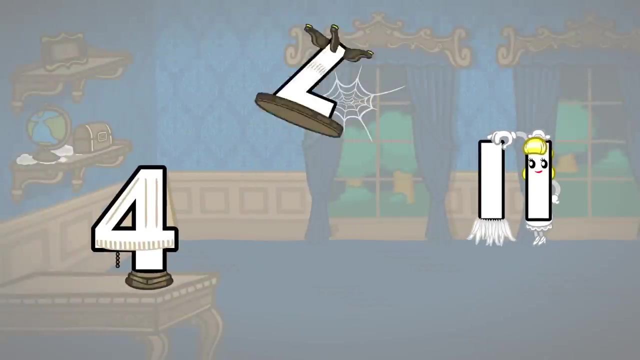 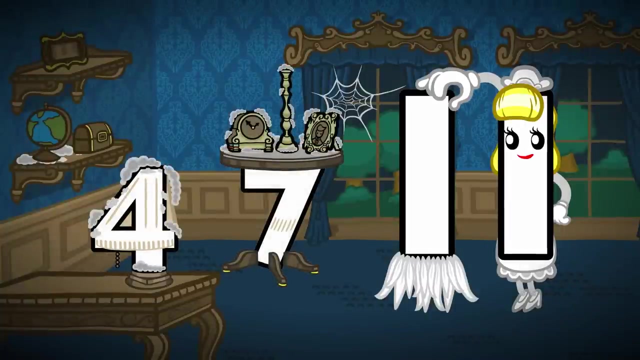 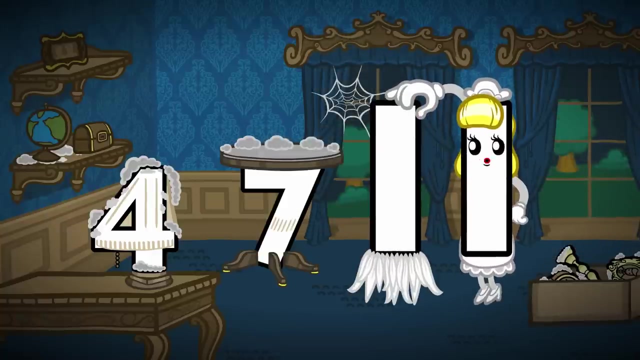 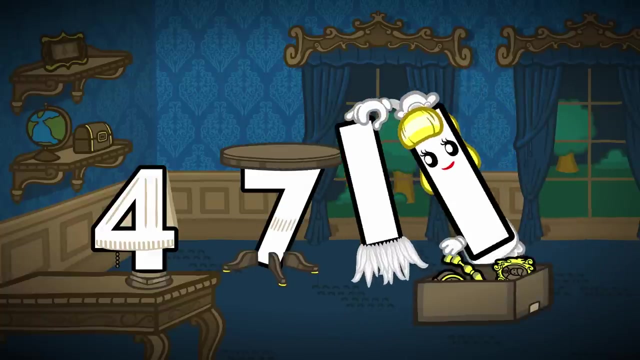 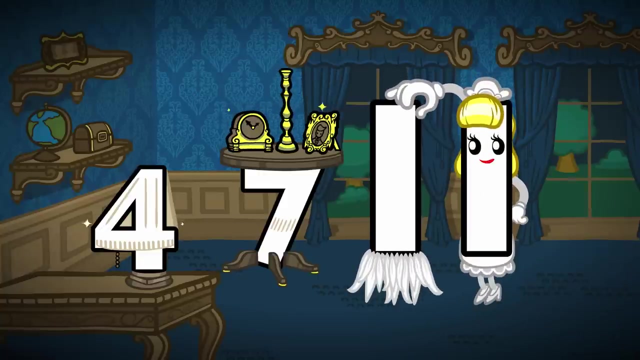 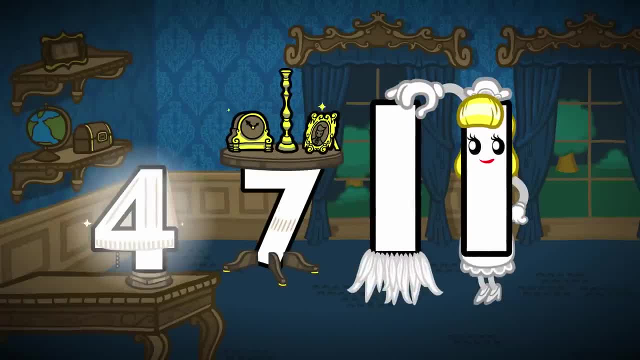 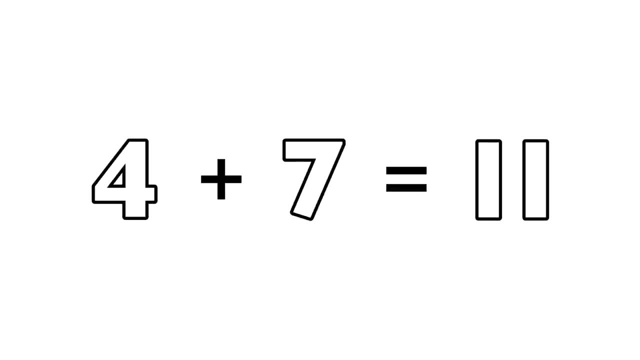 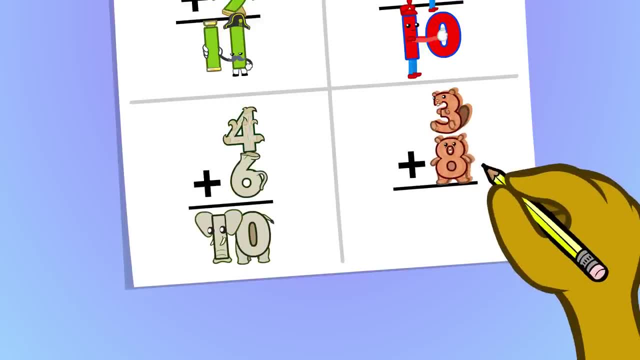 equals 2,, 2,, 3,, 4,, 6,, 7,, 7,, 9,, 10, 11. equals 2,, 3,, 4,, 5,, 6,, 7,, 7,, 8,, 9,, 10, 11. 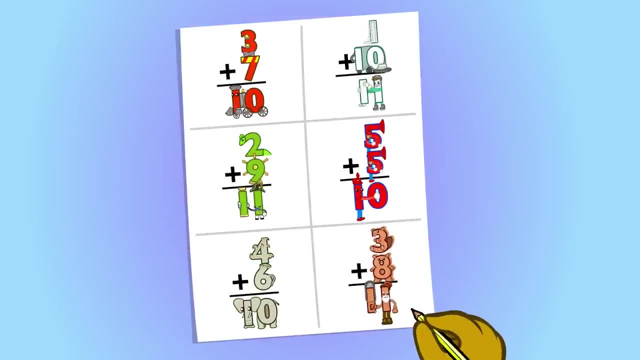 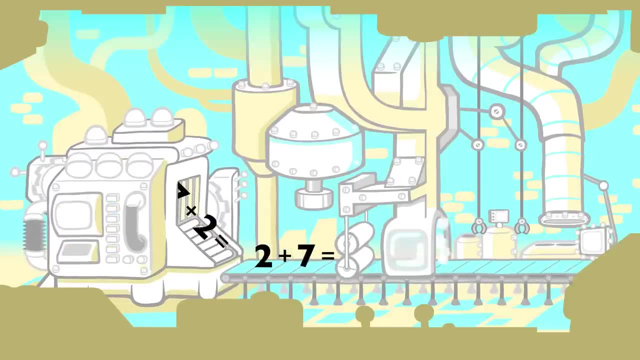 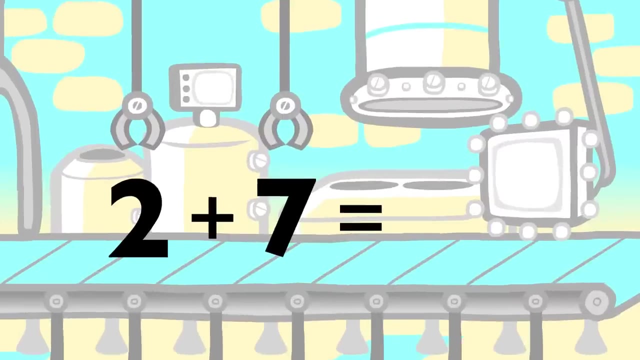 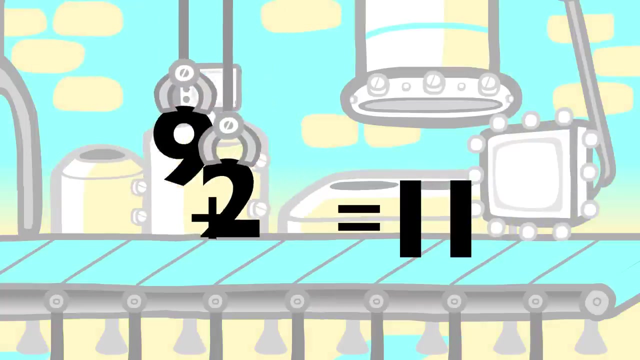 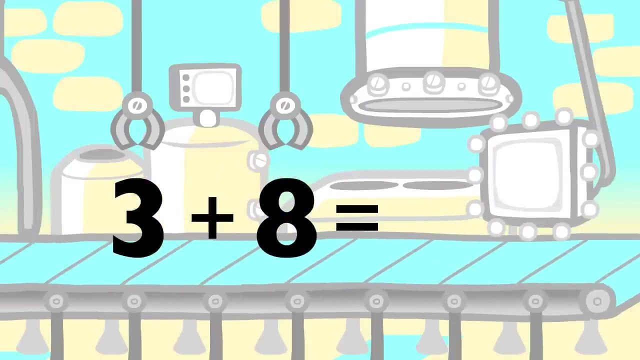 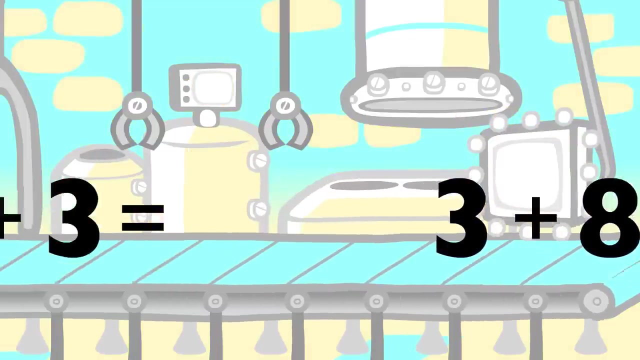 equals, let's Play 7. Let's Play 2. 1, 2, 2 plus 7 equals 9, and 7 plus 2 equals 9. 2 plus 9 equals 11, and 9 plus 2 equals 11. 3 plus 8 equals 11, and 8 plus 3 equals 11. 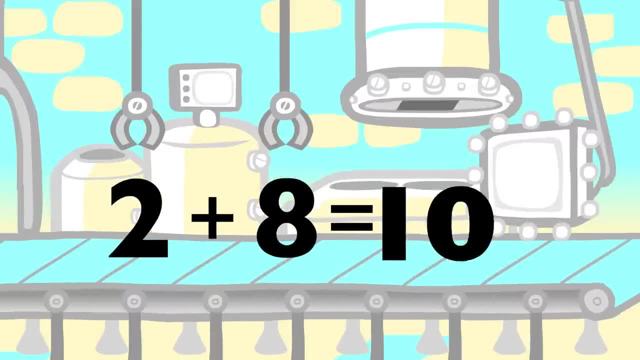 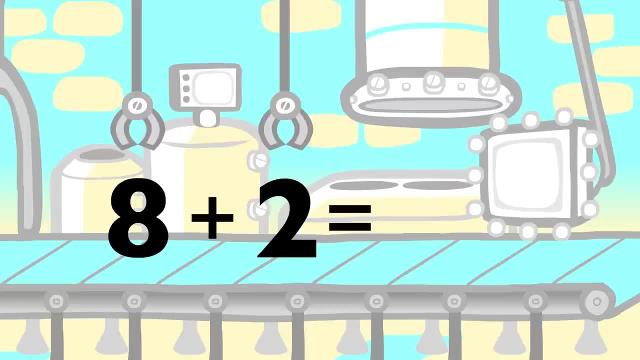 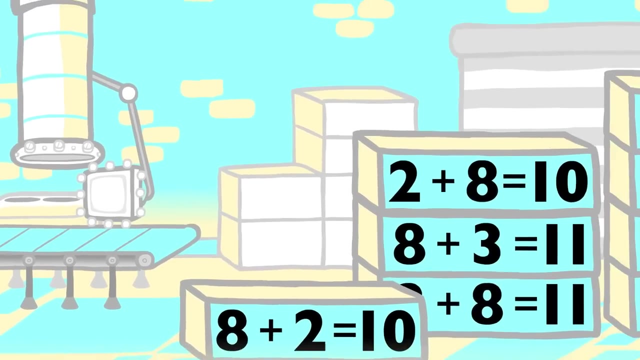 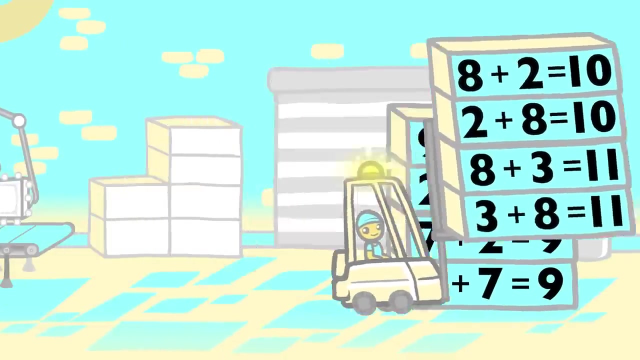 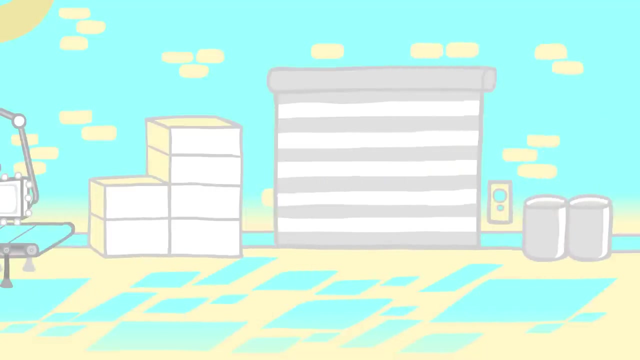 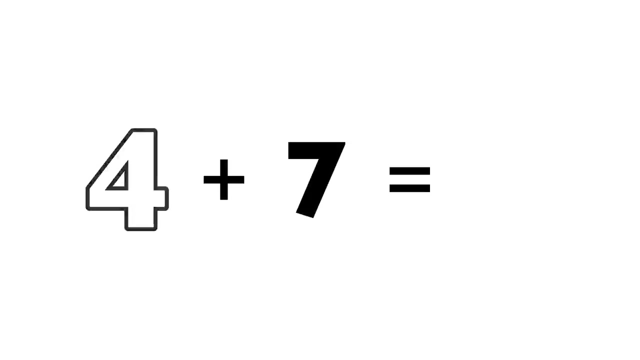 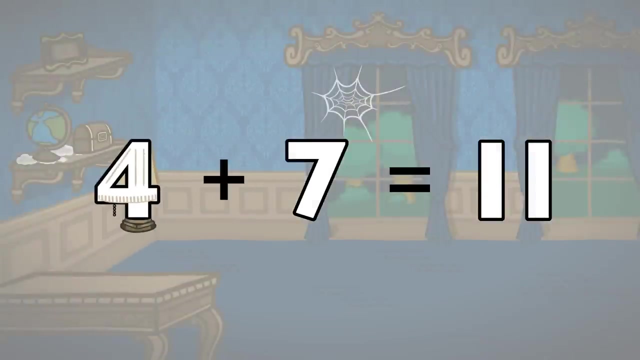 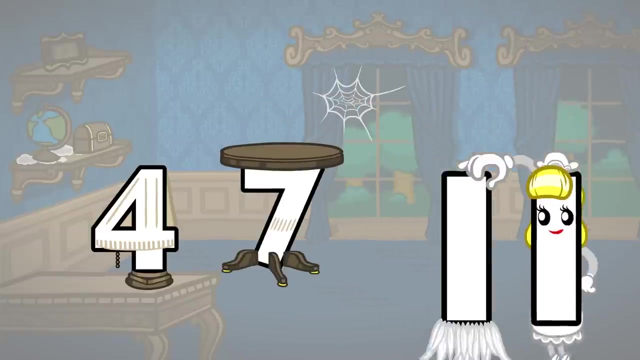 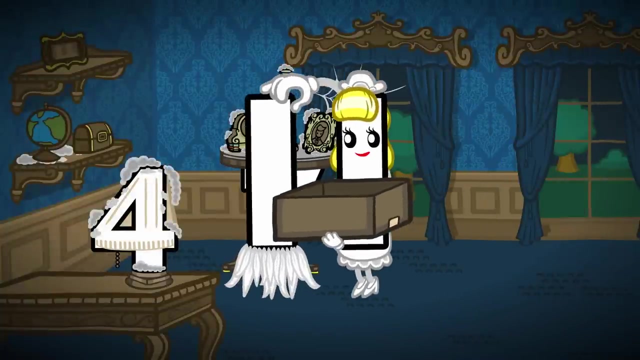 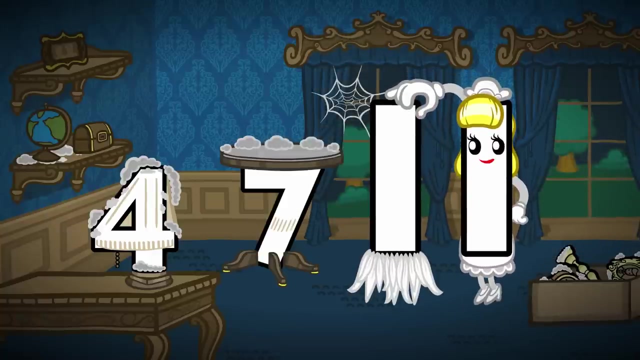 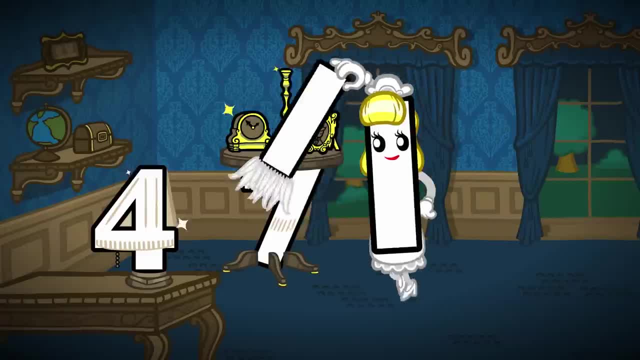 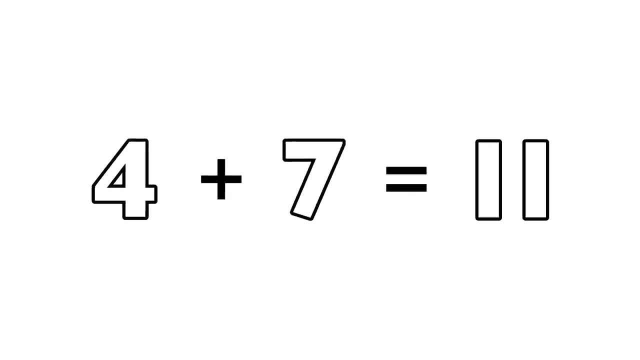 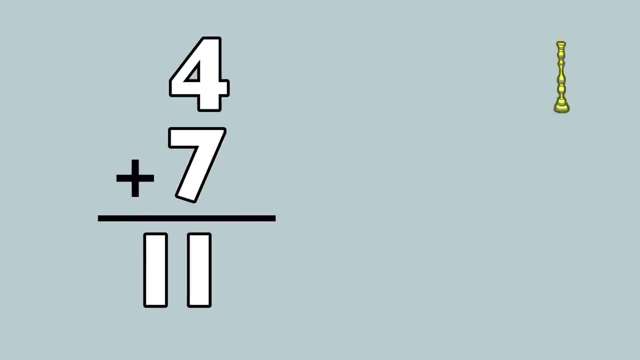 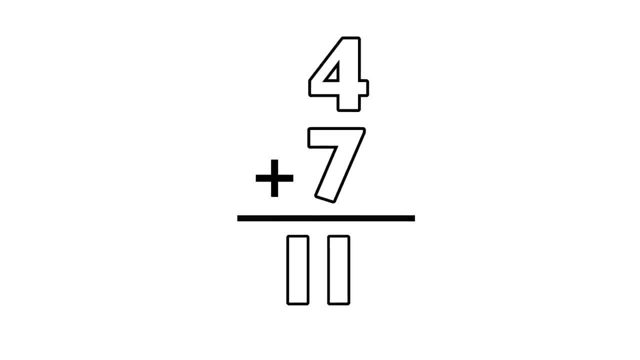 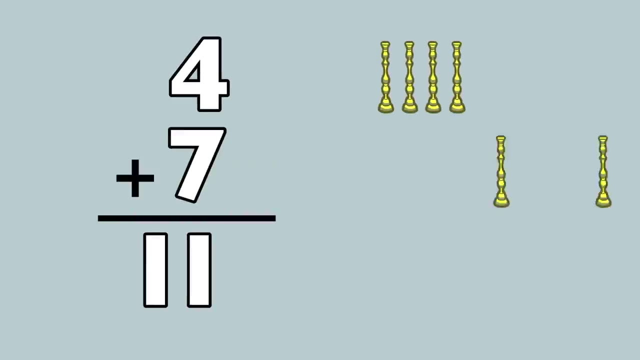 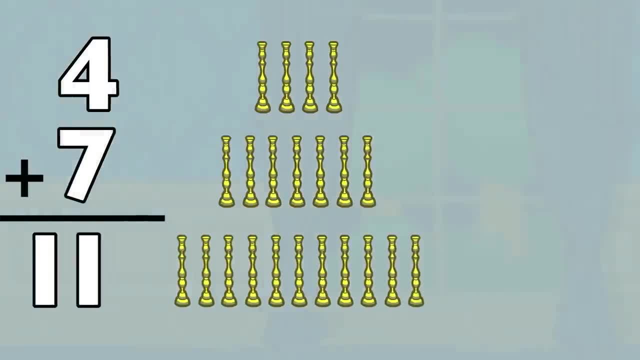 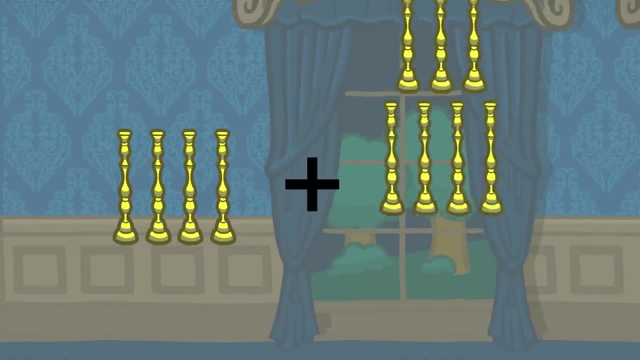 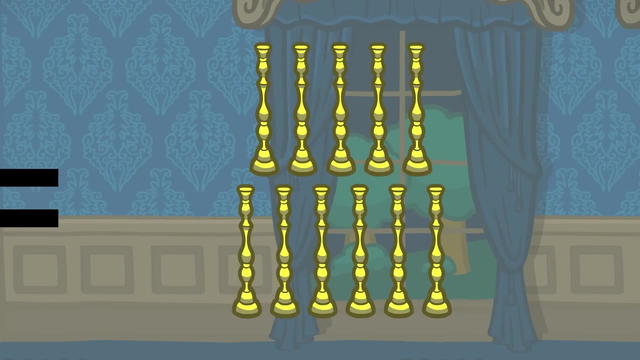 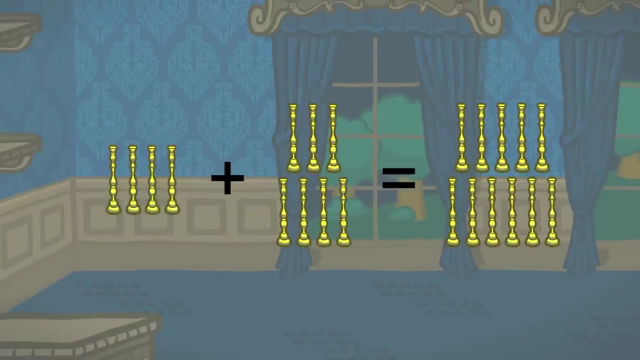 4 plus 7 equals 11.. 4 plus 7 equals 11.. 4 plus 7 equals 11.. 1,, 2,, 3,, 4,, 5,, 6,, 7,, 8,, 9,, 10,, 11.. 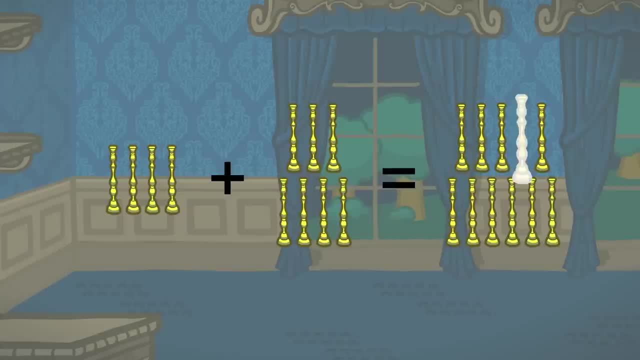 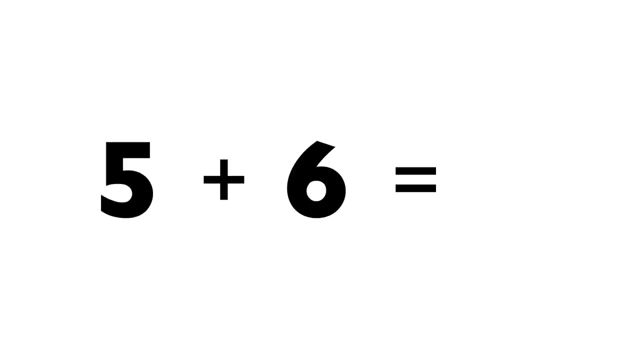 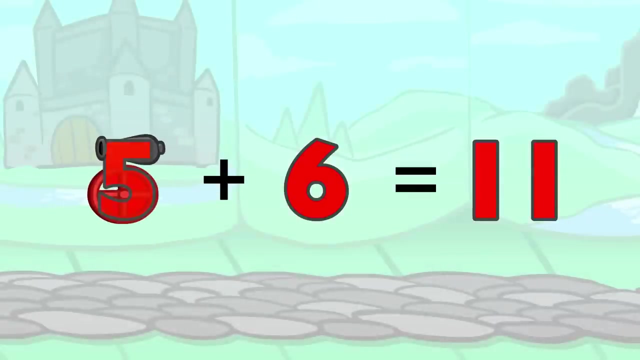 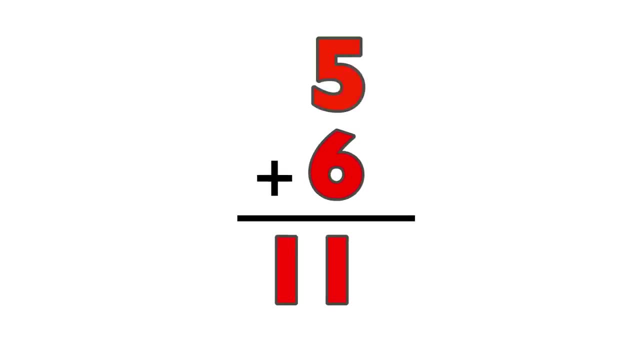 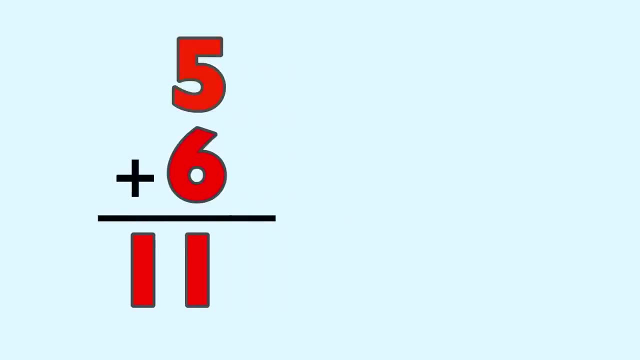 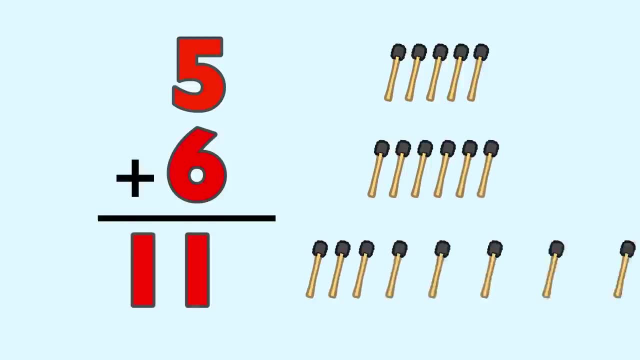 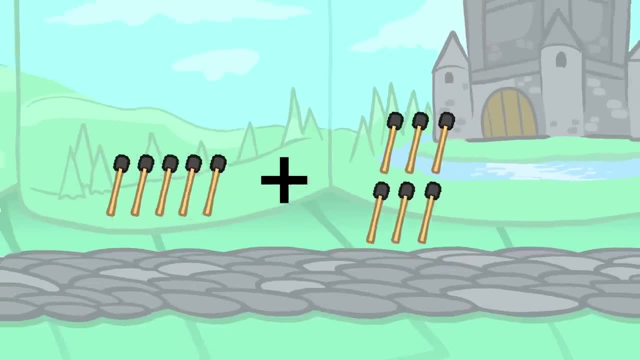 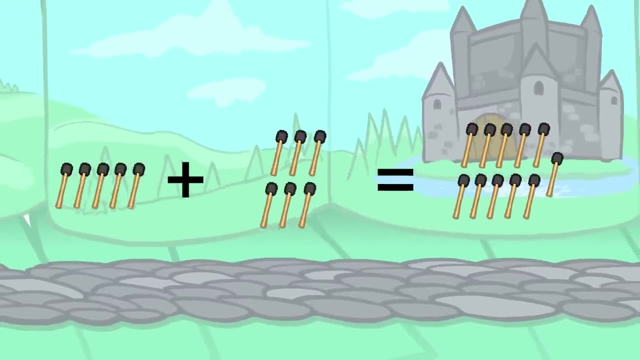 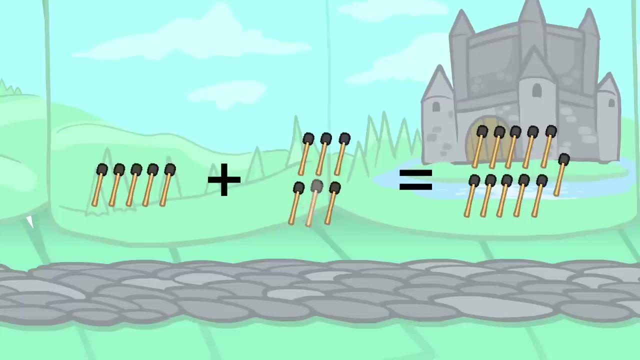 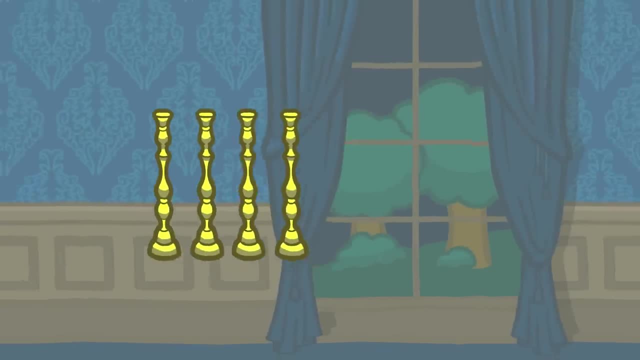 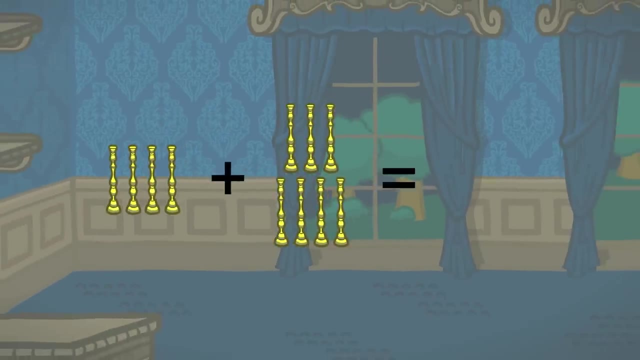 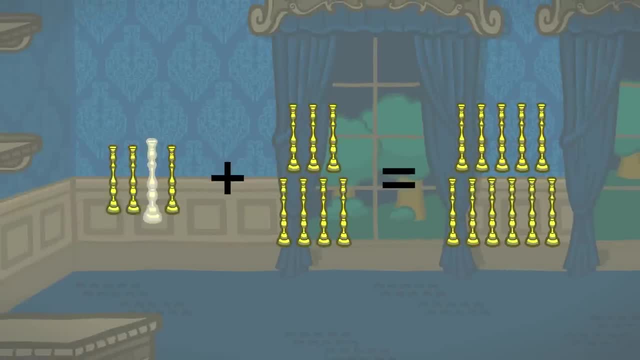 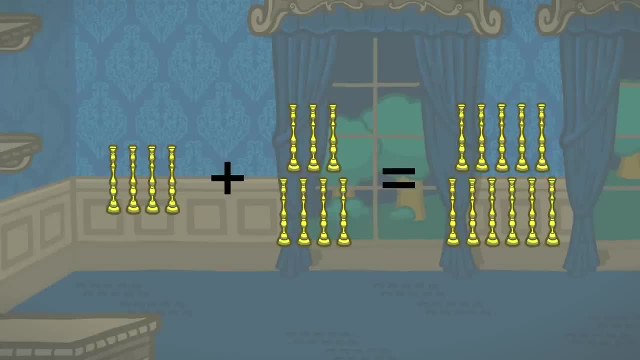 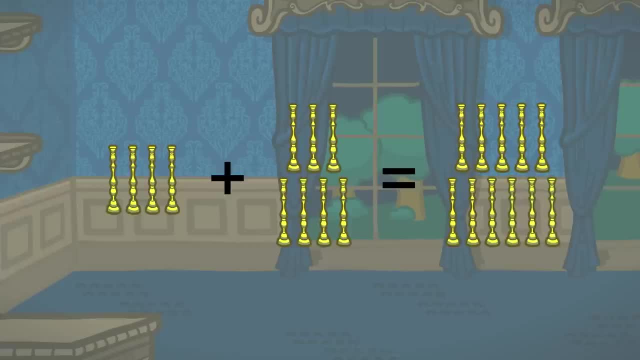 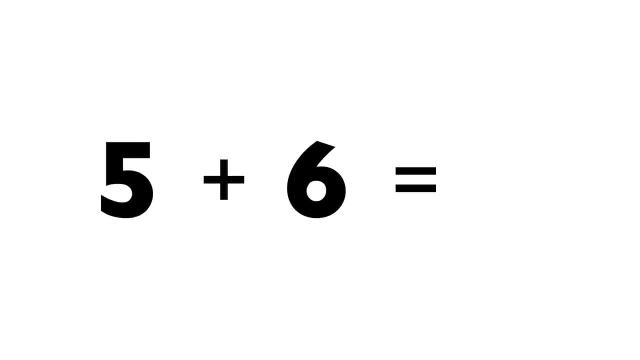 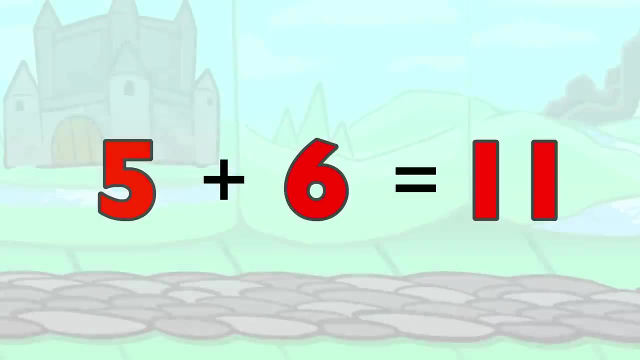 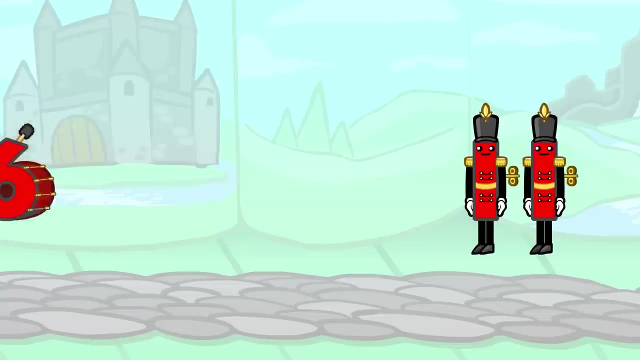 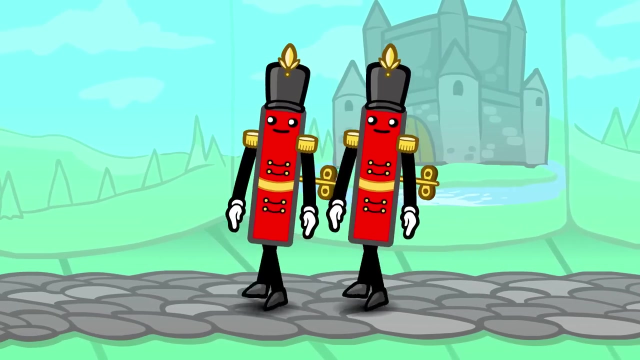 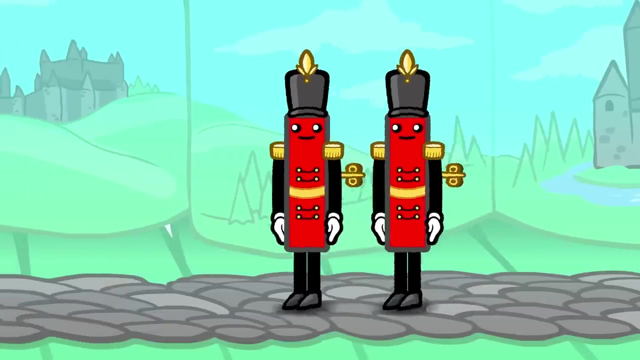 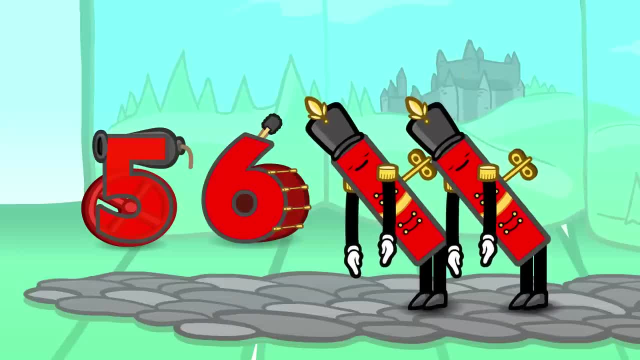 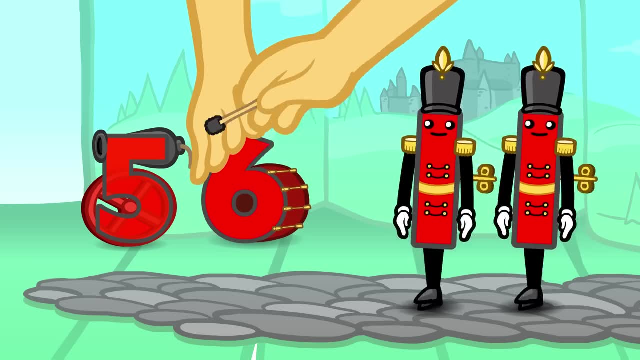 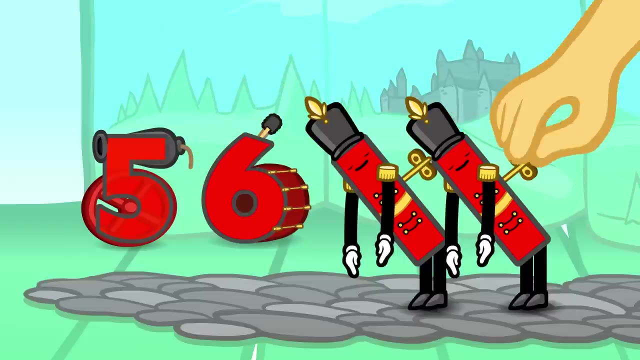 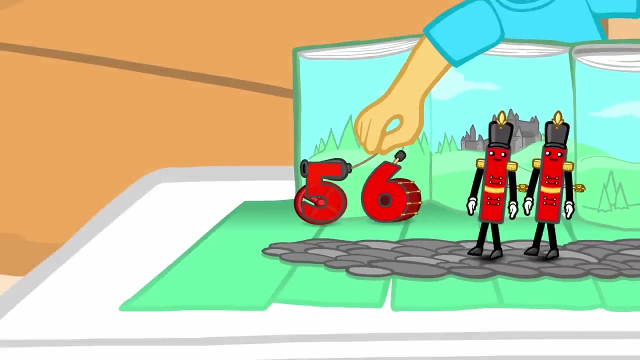 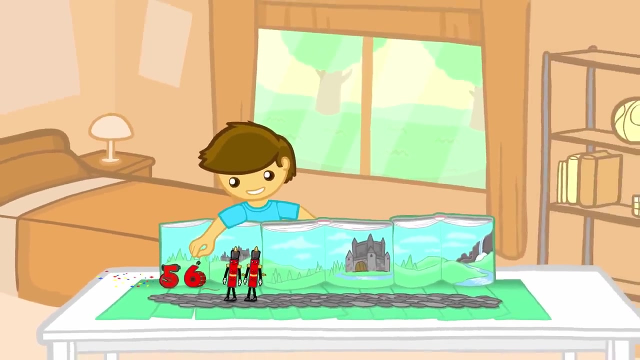 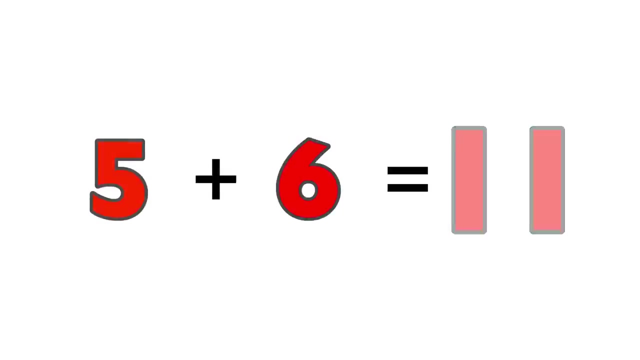 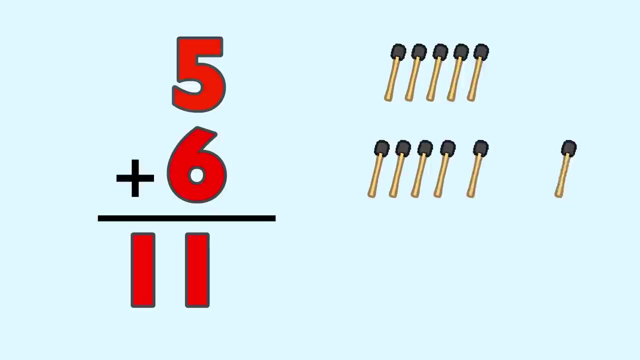 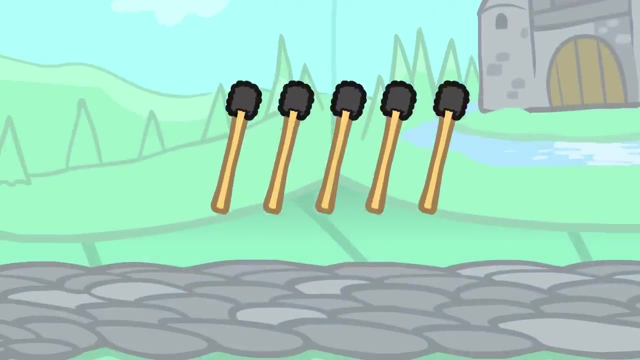 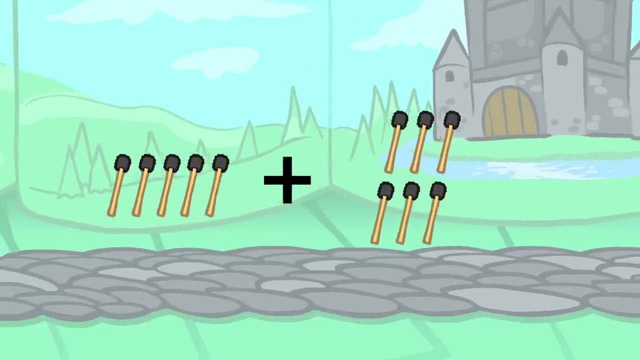 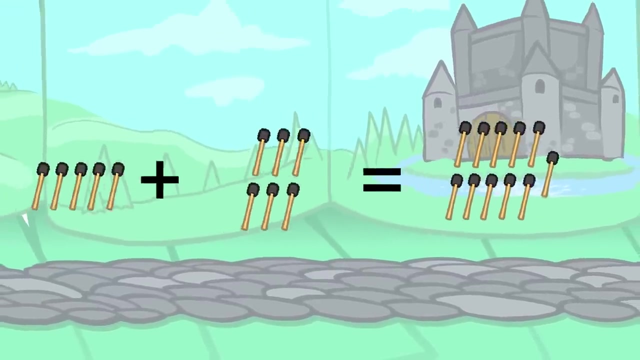 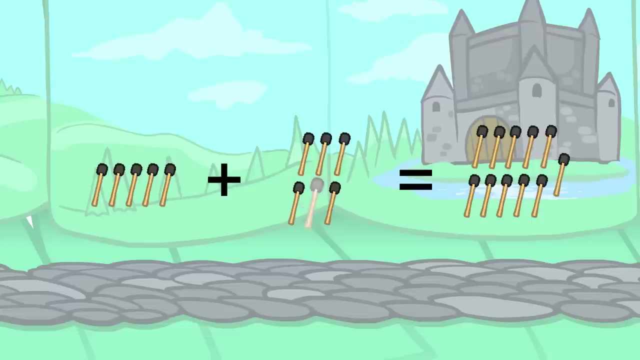 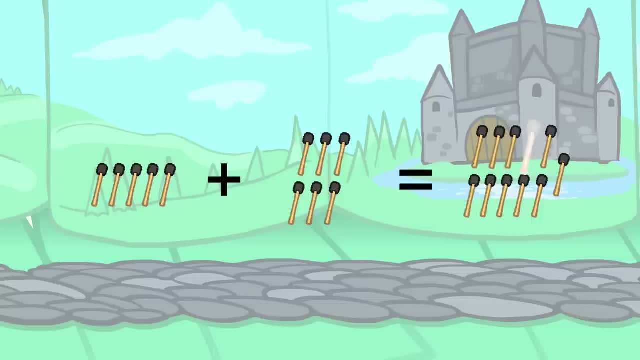 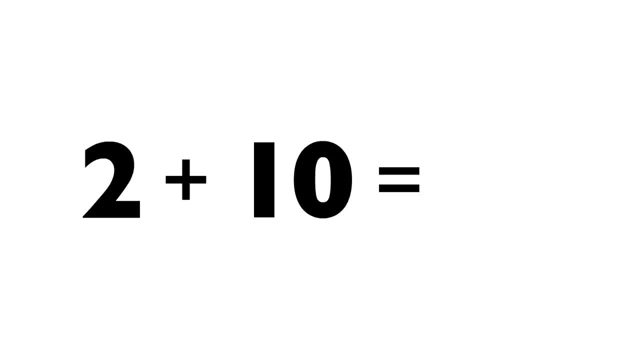 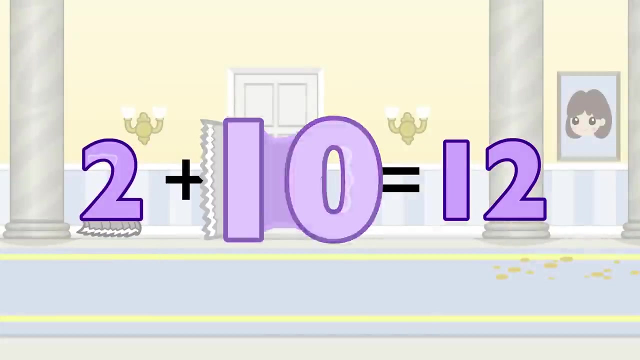 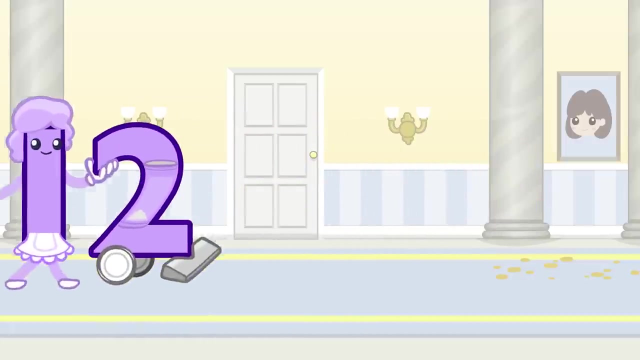 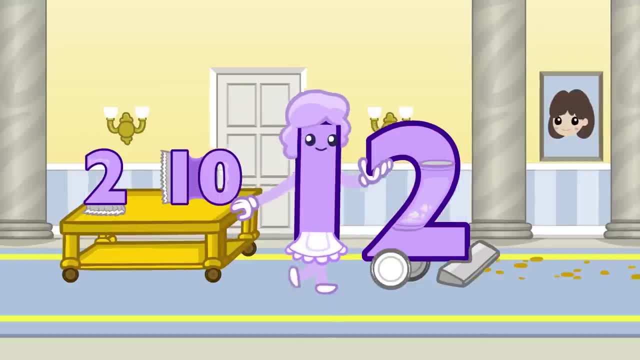 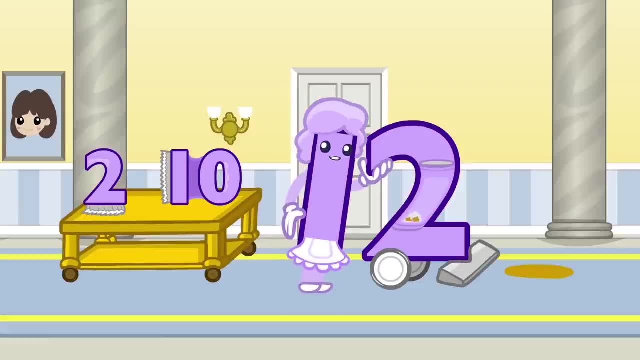 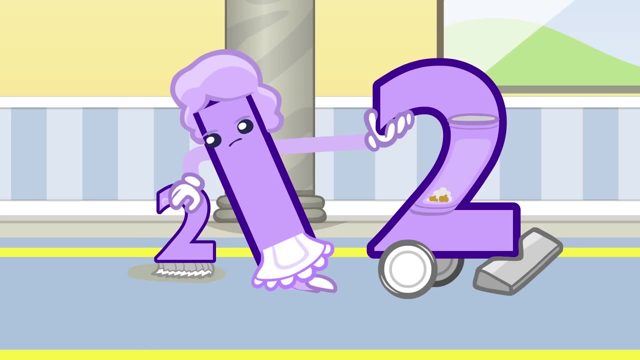 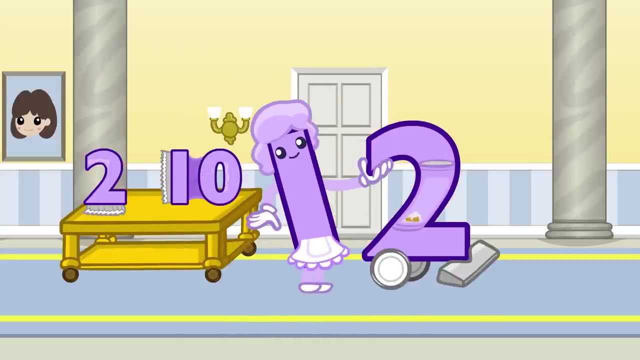 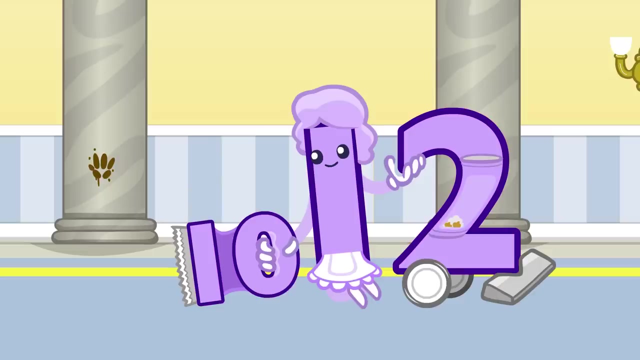 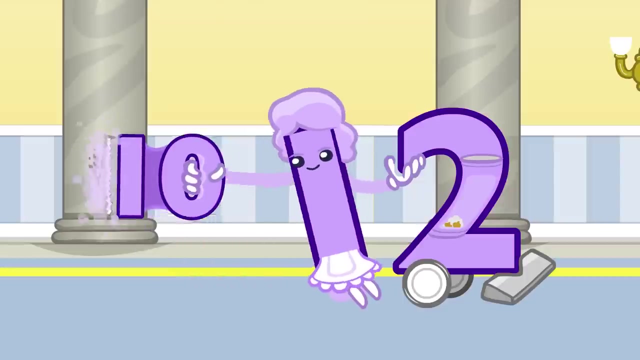 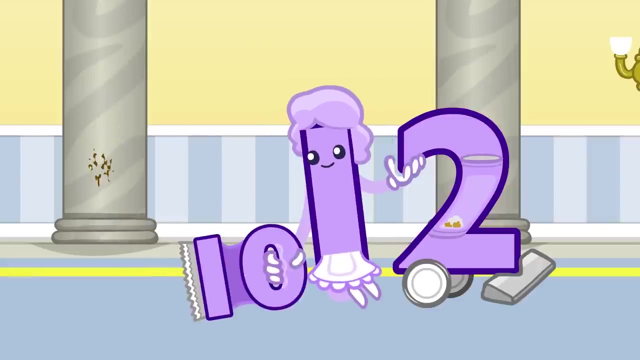 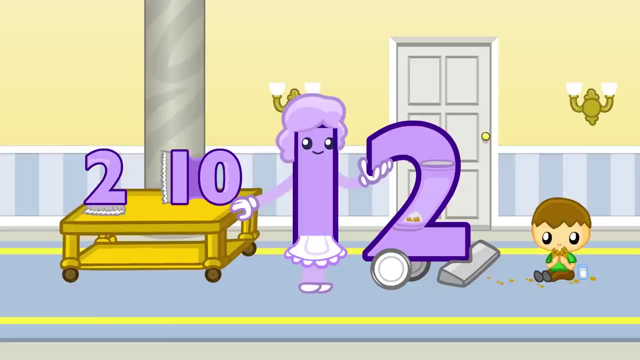 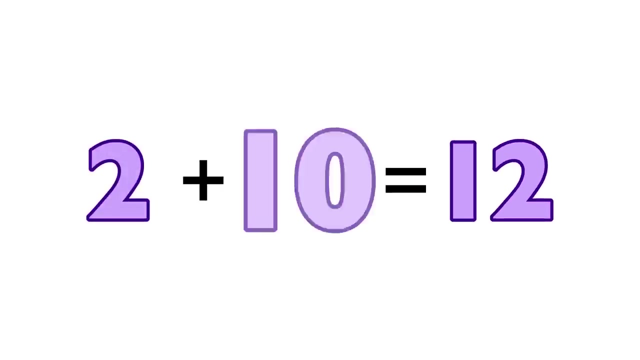 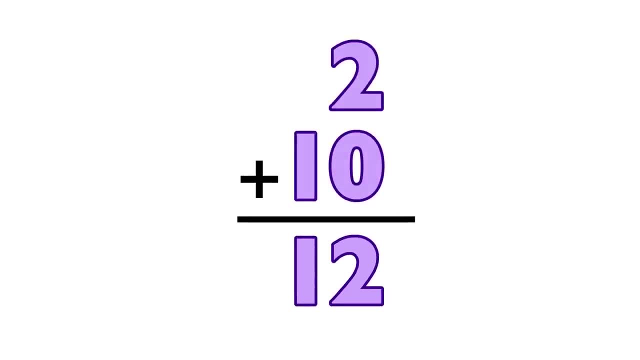 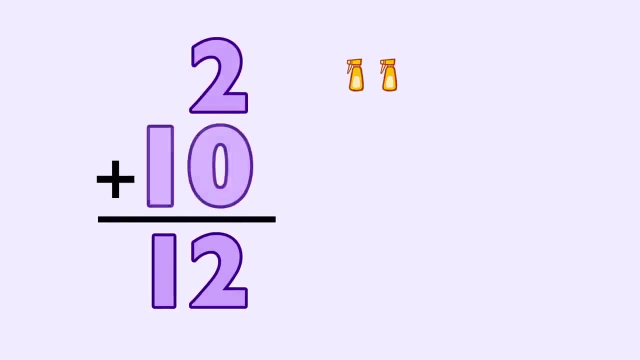 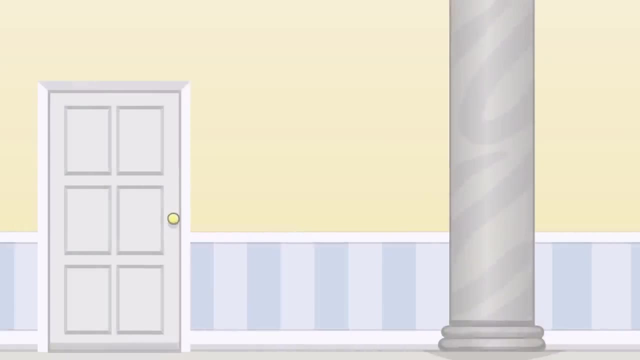 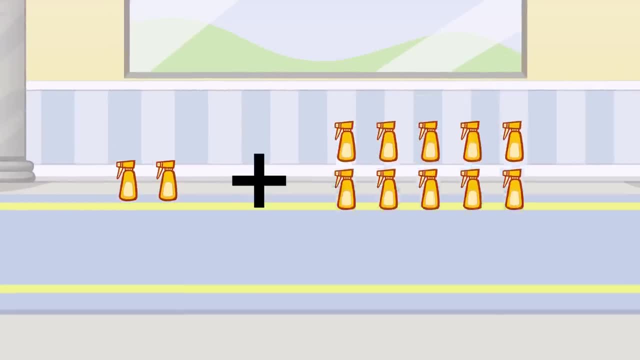 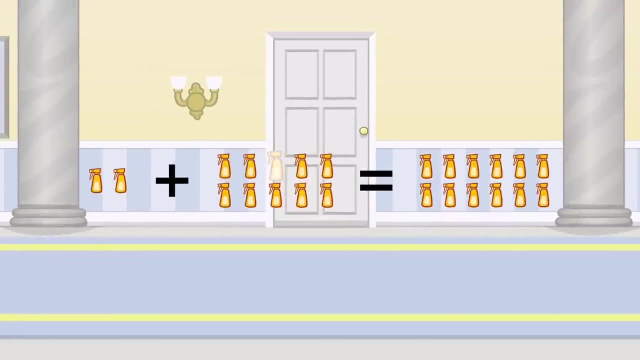 2 plus 10 equals 12.. 1,, 2,, 3,, 4,, 5,, 6,, 7,, 8,, 9,, 10,, 11, 12 equals 1,, 2,, 3,, 4,, 5,. 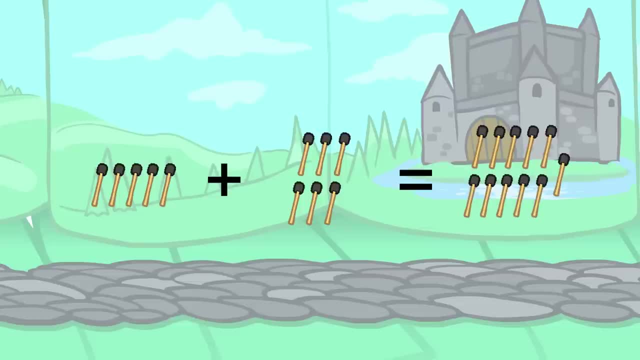 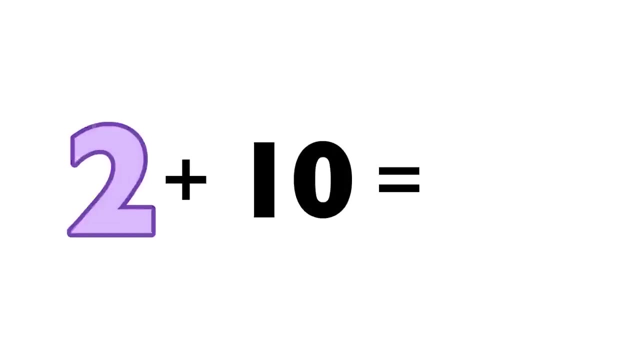 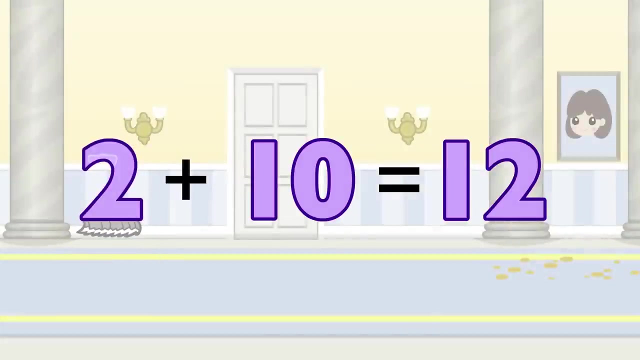 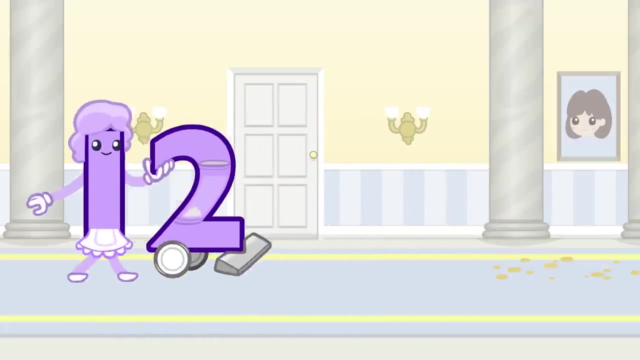 11,, 2,, 3,, 4,, 5,, 6,, 7,, 8,, 9,, 10,, 11,, 2,, 3,, 4,, 5,, 6,, 7,, 8,, 9,, 10,, 11.. 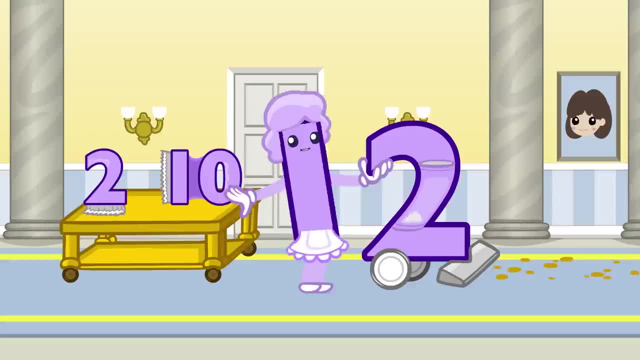 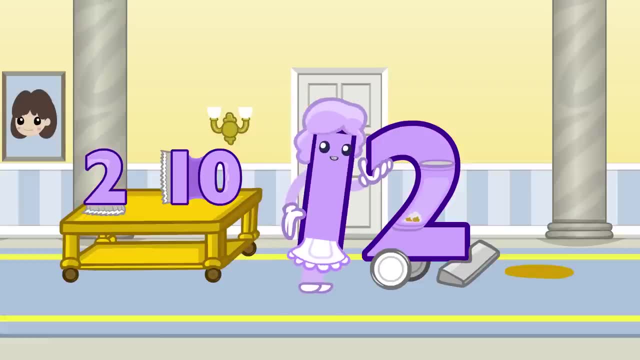 11,, 2,, 3,, 4,, 5,, 6,, 7,, 8,, 9,, 10,, 11.. 2 plus 10 equals 12.. 2 plus 10 equals 12.. 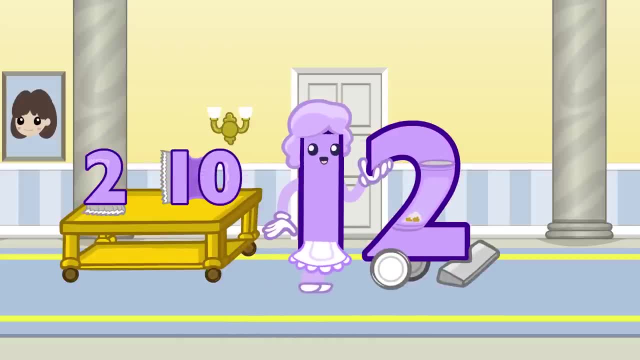 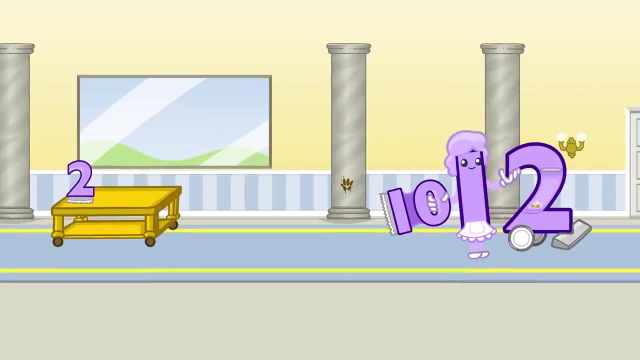 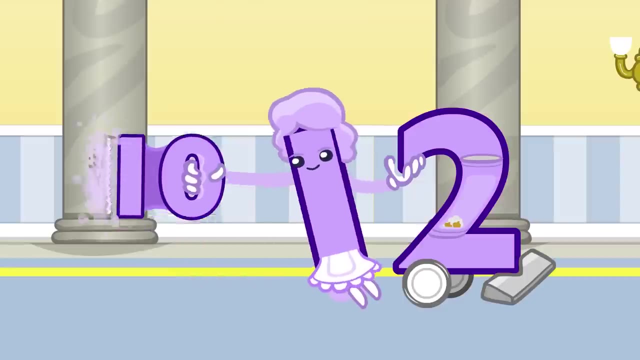 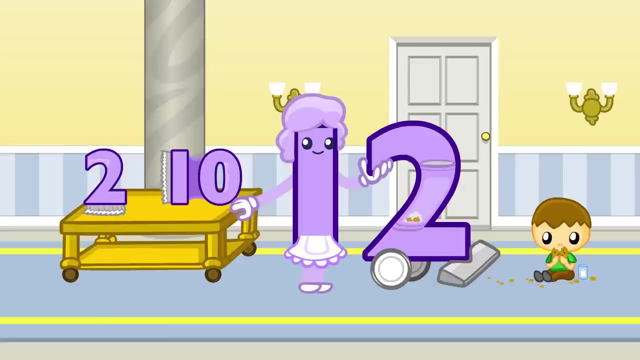 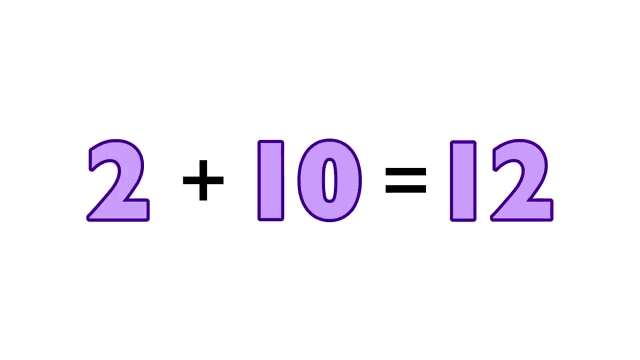 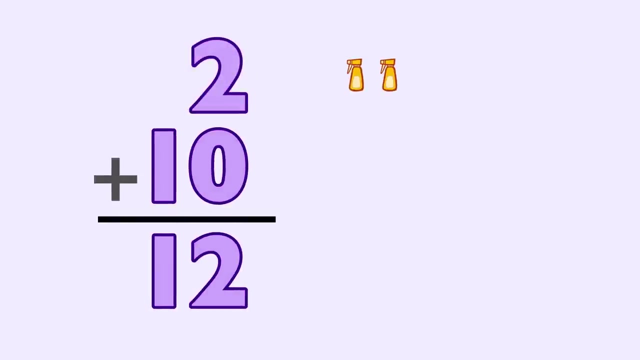 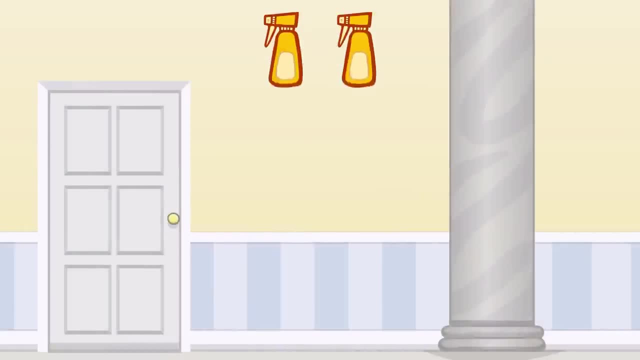 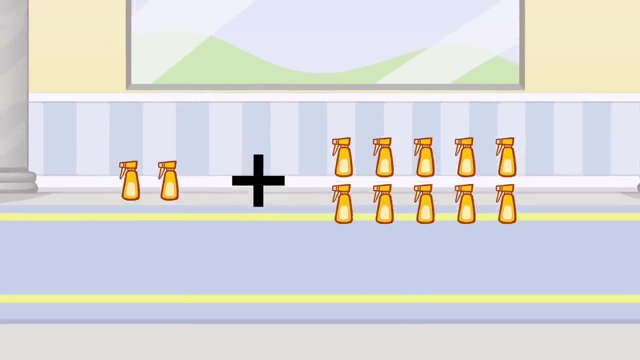 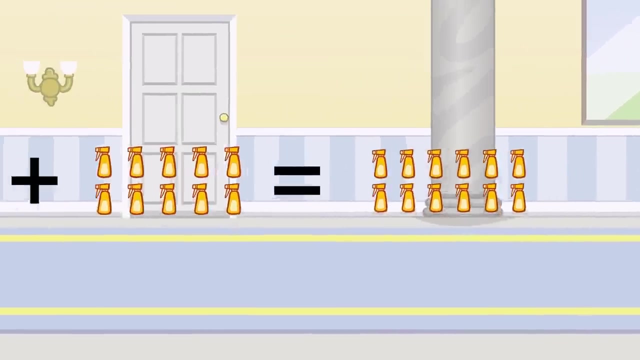 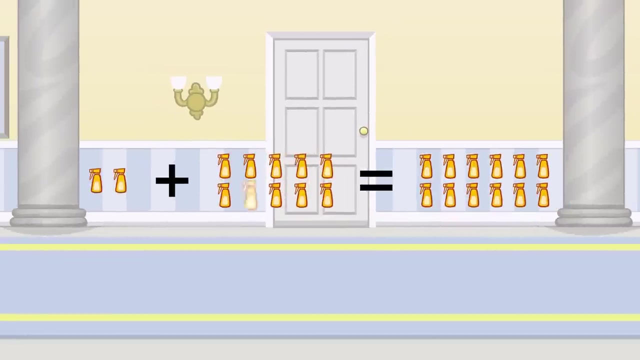 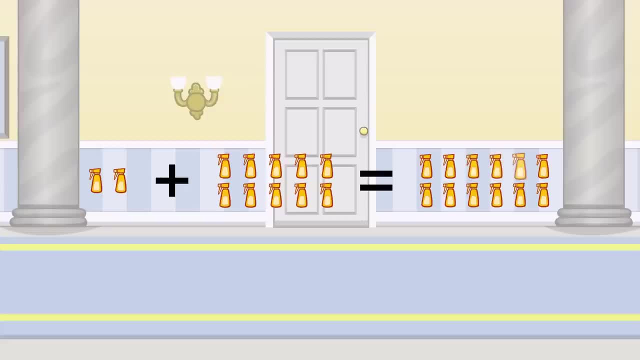 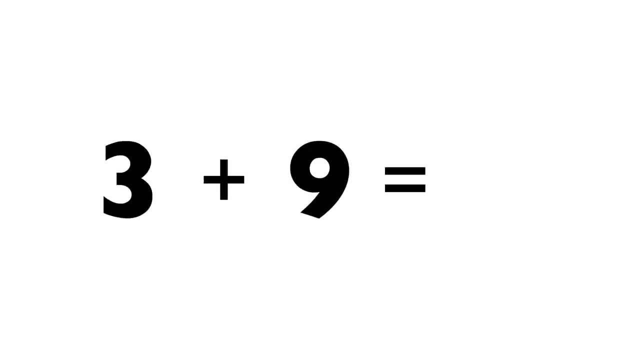 1,, 2,, 3,, 4,, 5,, 6,, 7,, 8,, 9,, 10,, 11, 12.. 3 plus 9 equals 3 plus 9 equals 12.. 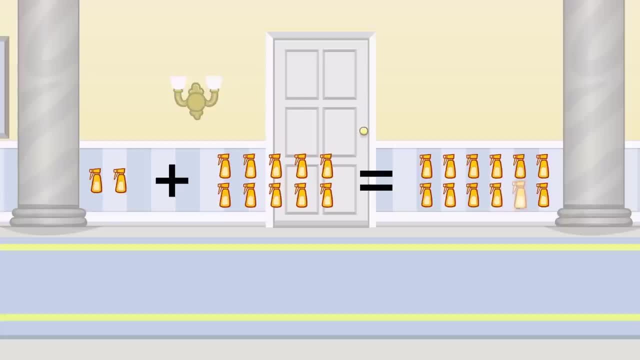 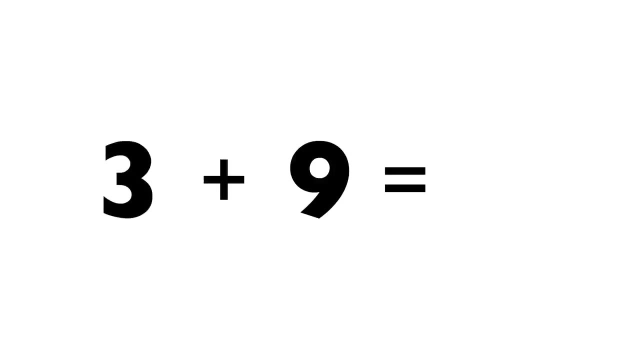 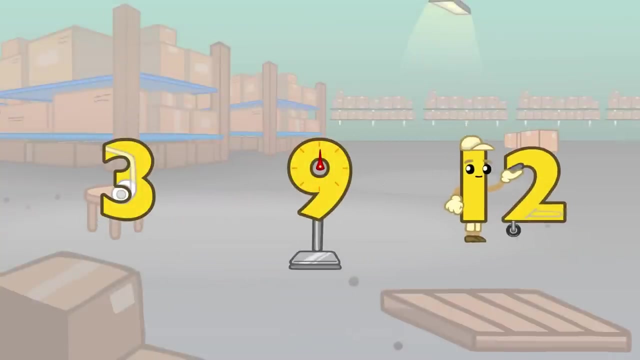 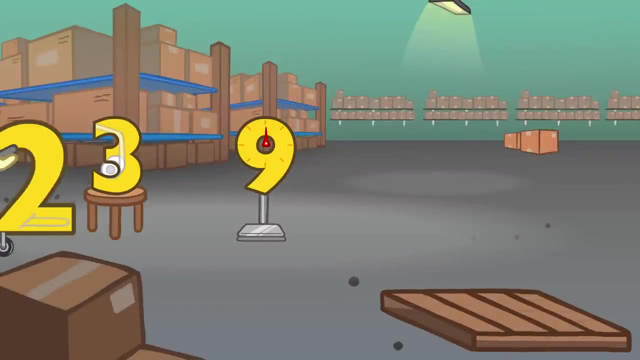 6,, 7,, 8,, 9,, 10,, 11,, 12.. 3 plus 9 equals. 3 plus 9 equals 12.. 3 plus 9 equals 12.. 3 plus 9 equals 12.. 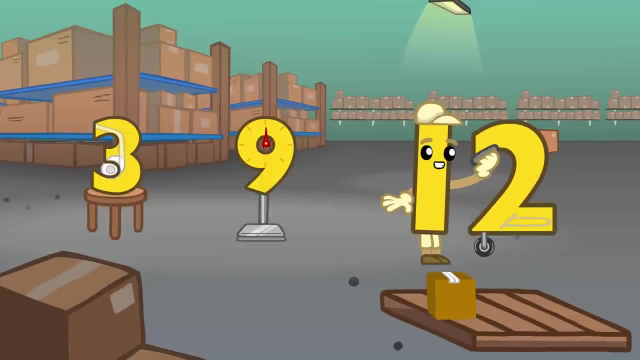 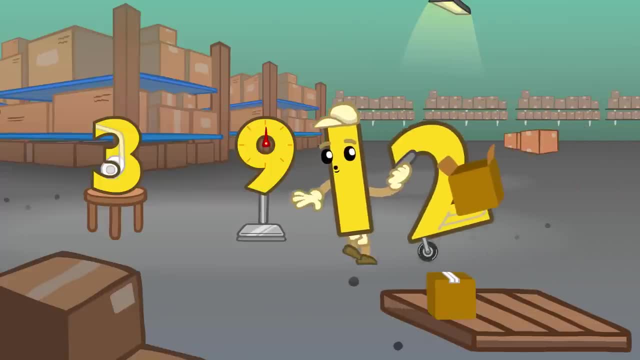 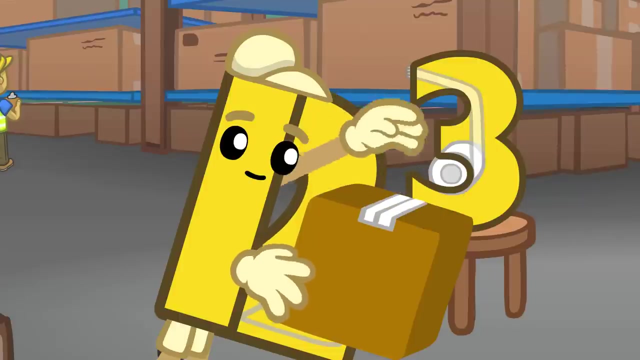 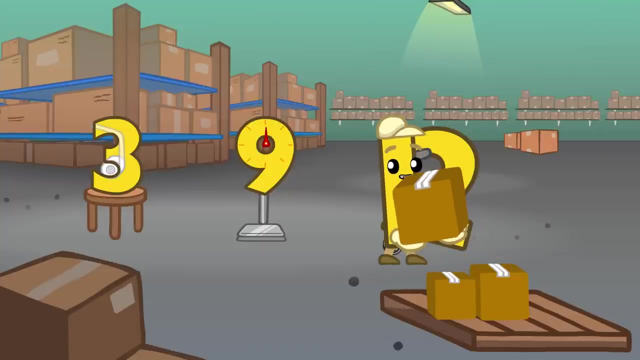 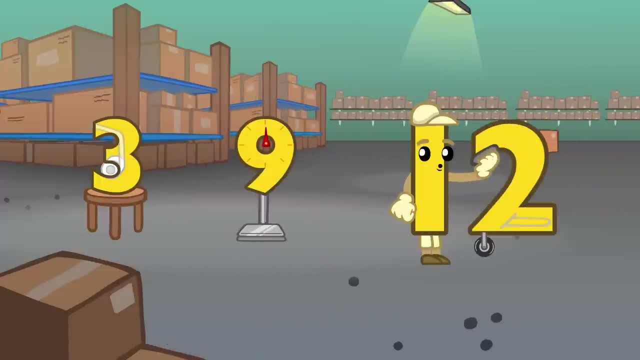 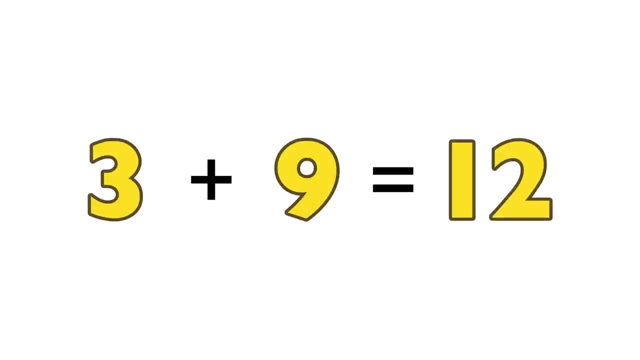 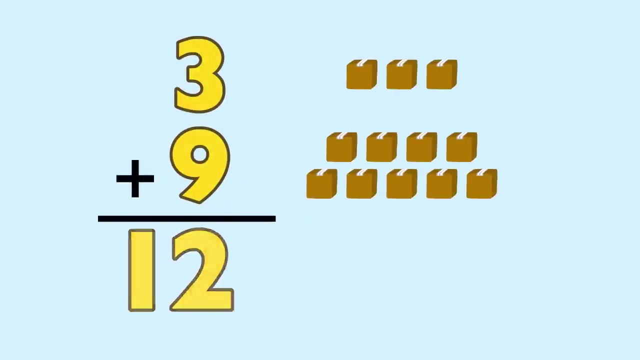 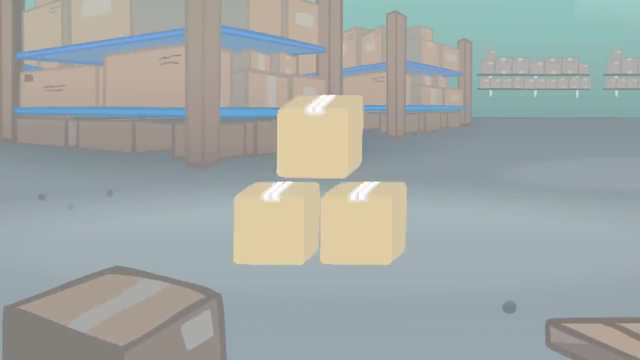 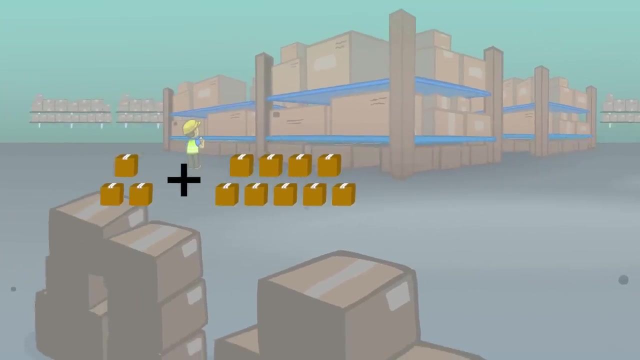 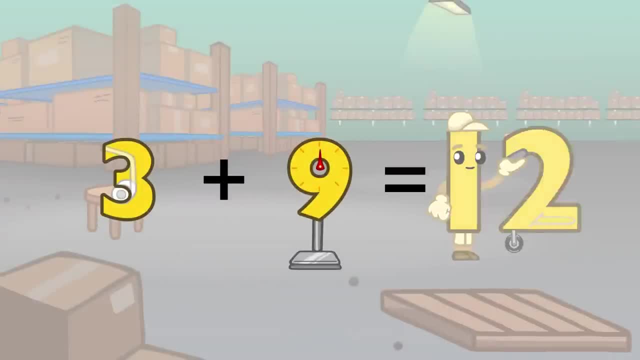 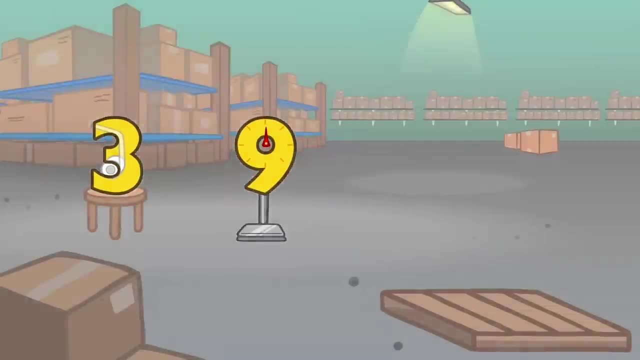 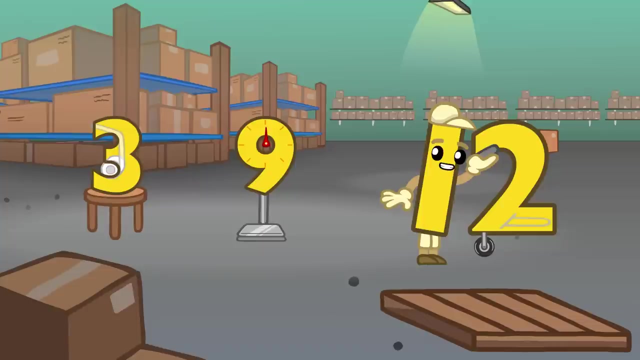 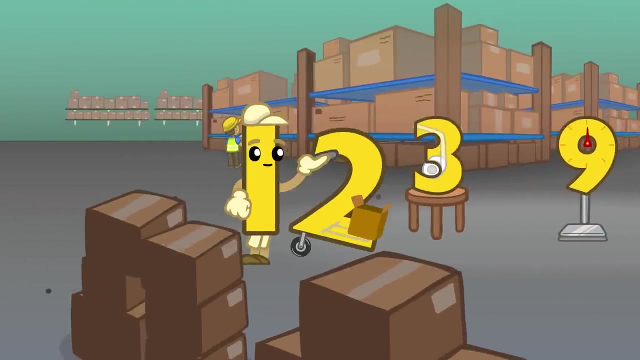 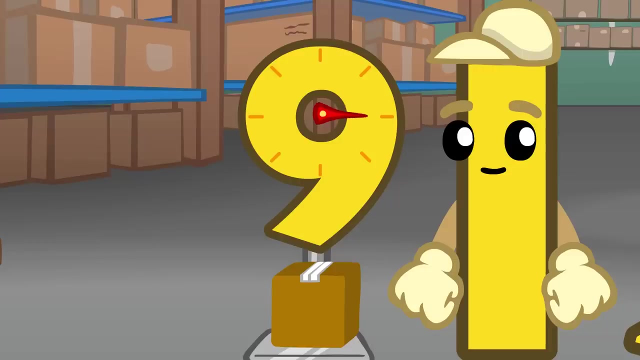 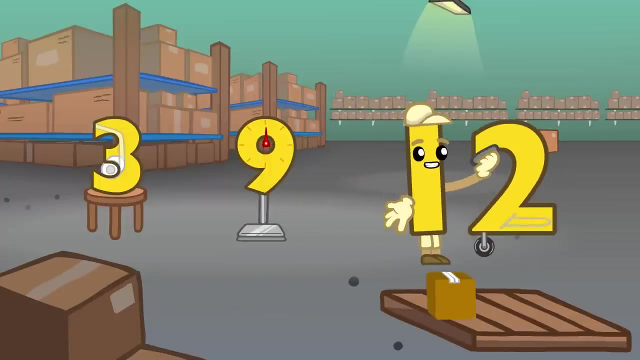 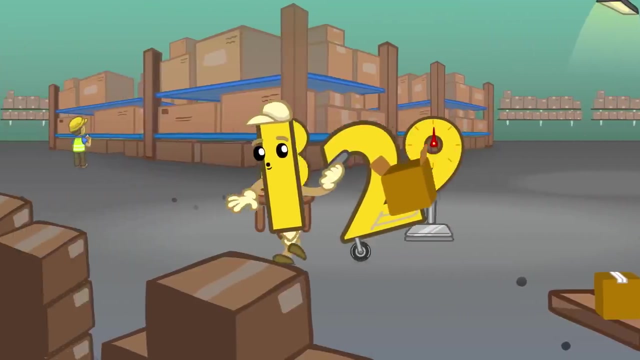 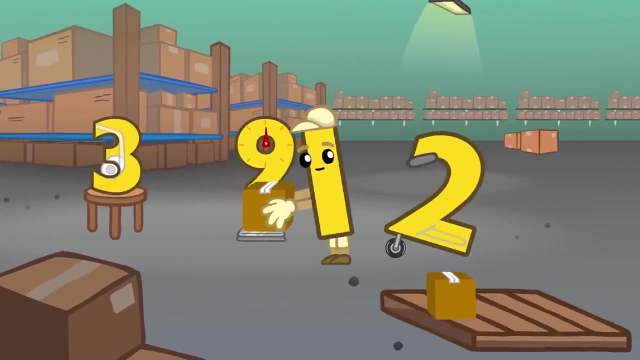 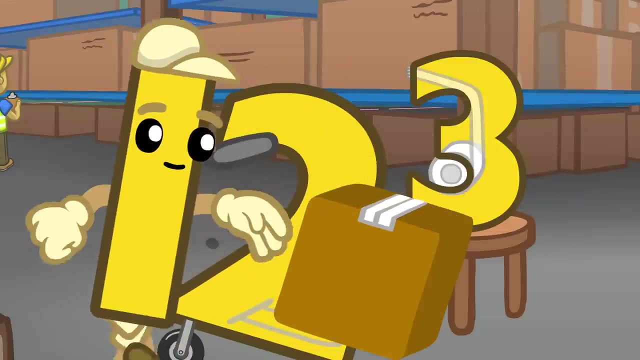 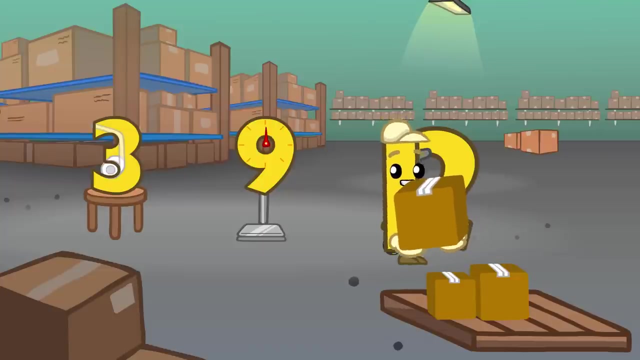 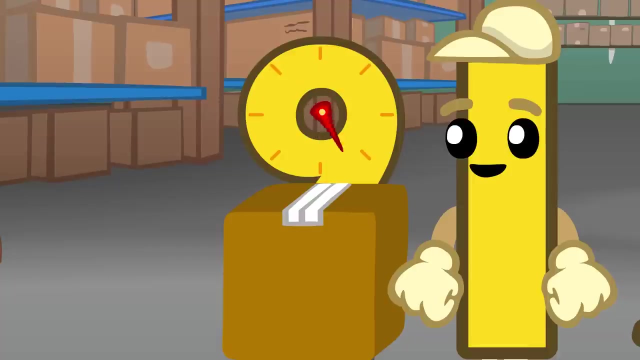 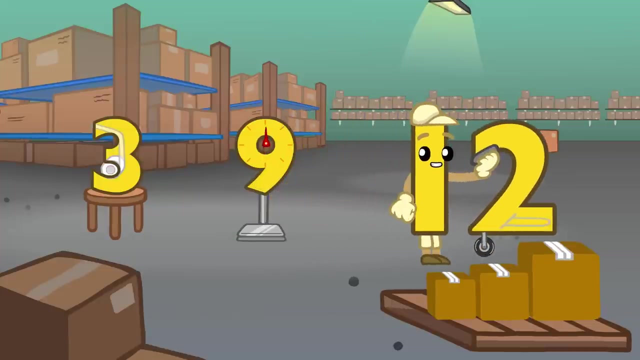 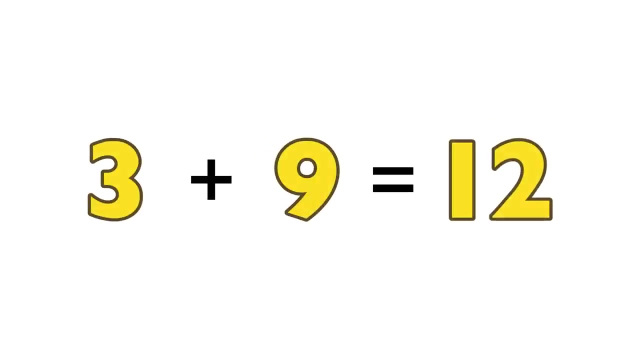 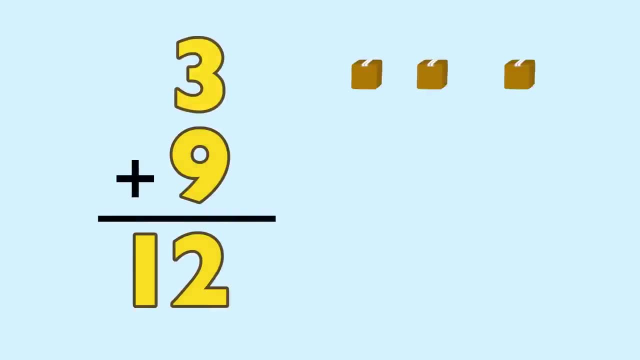 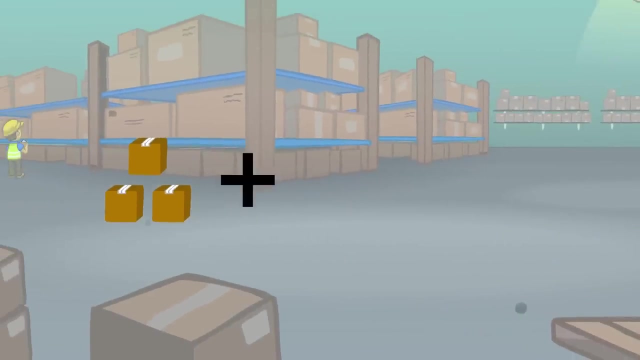 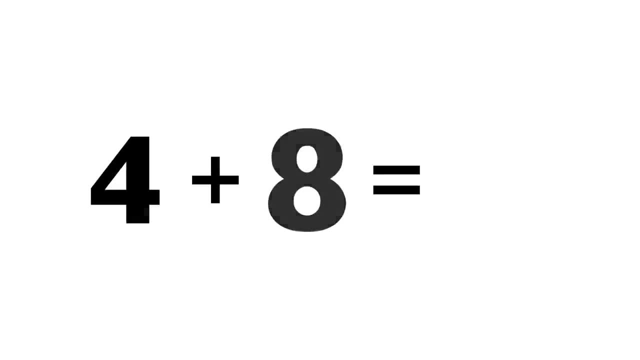 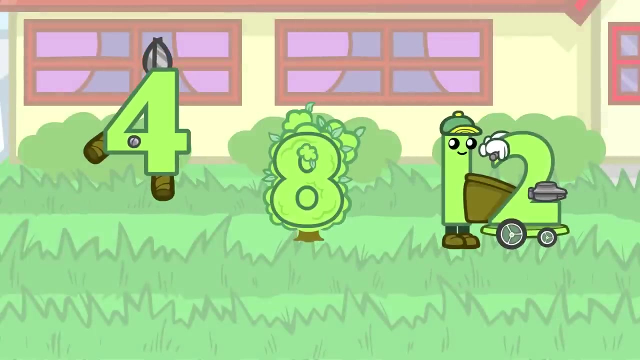 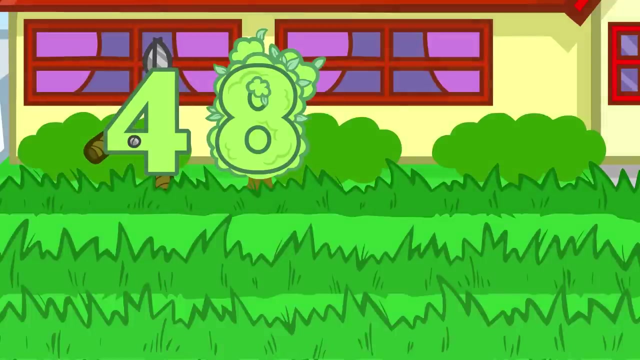 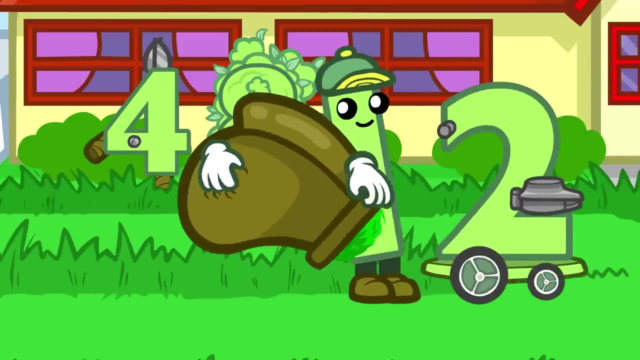 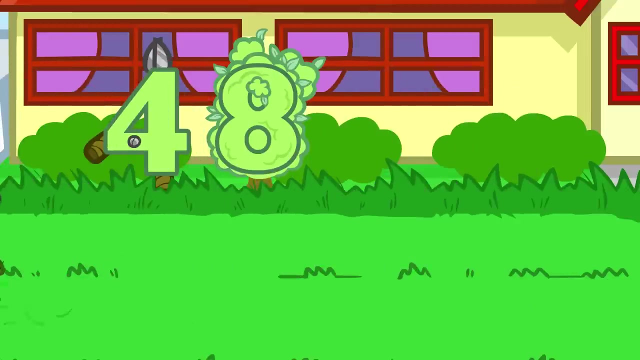 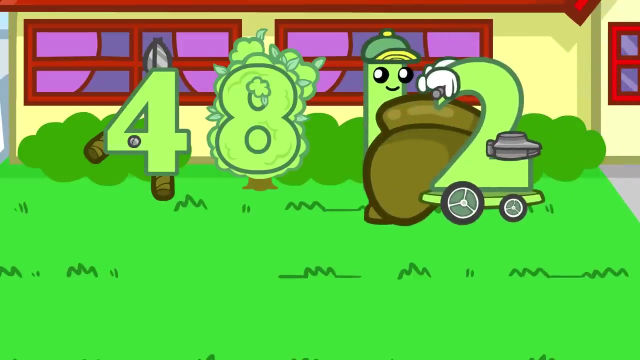 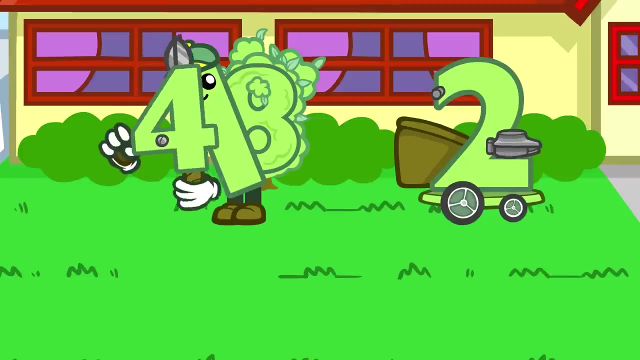 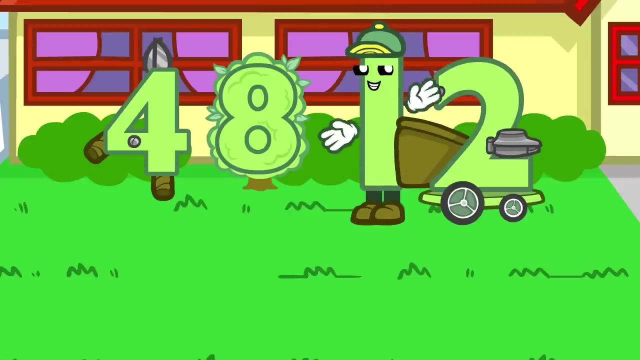 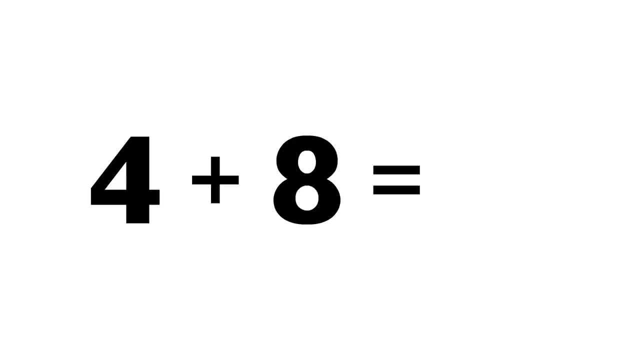 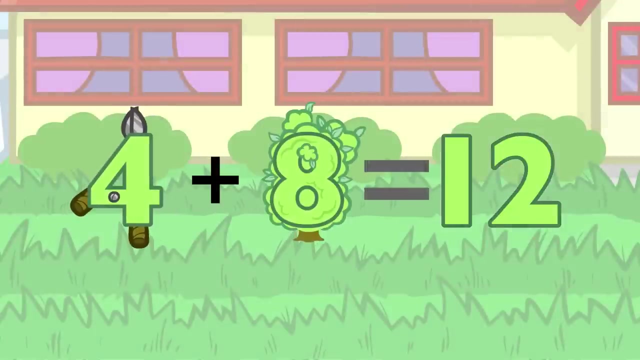 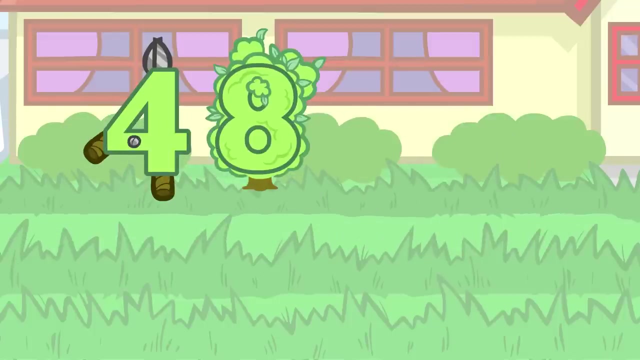 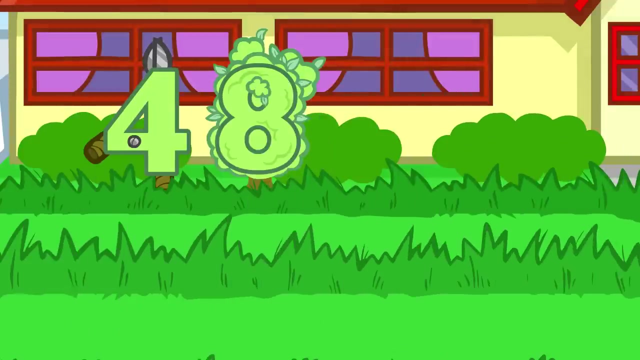 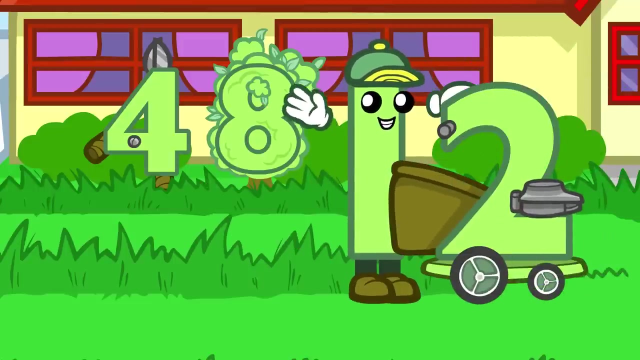 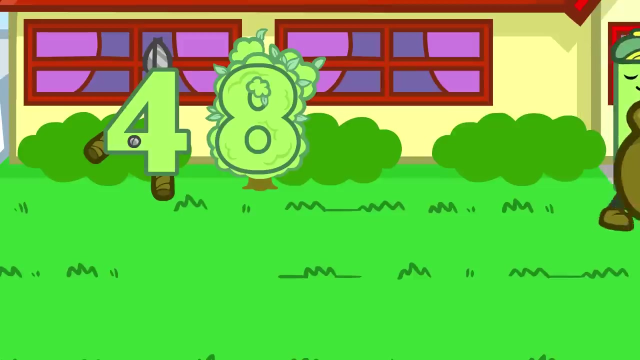 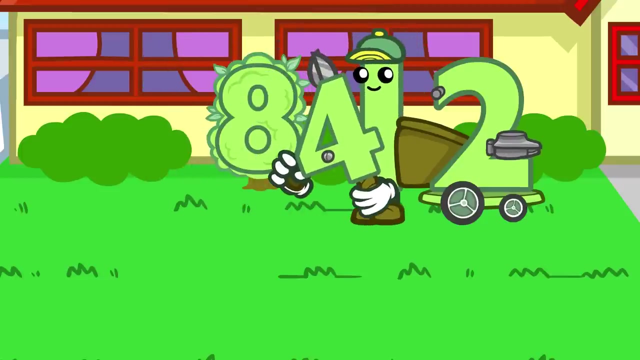 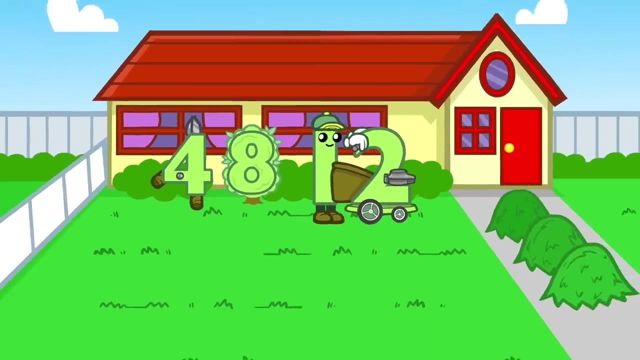 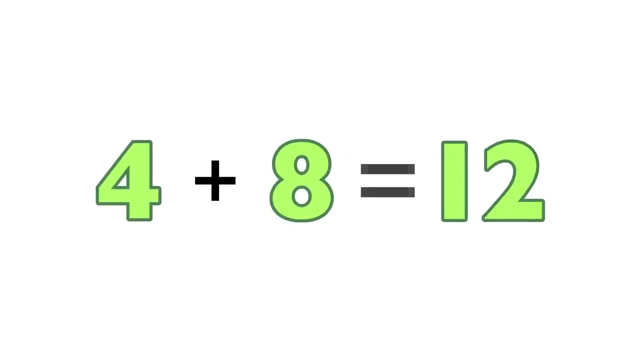 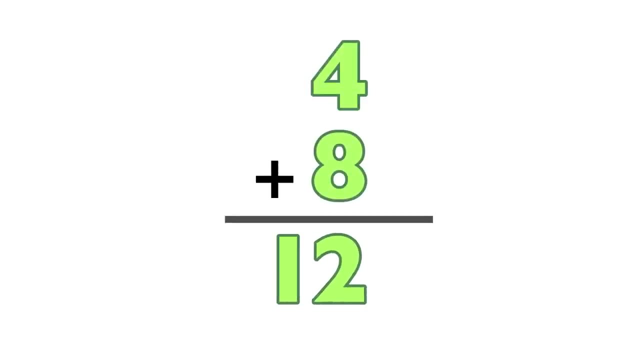 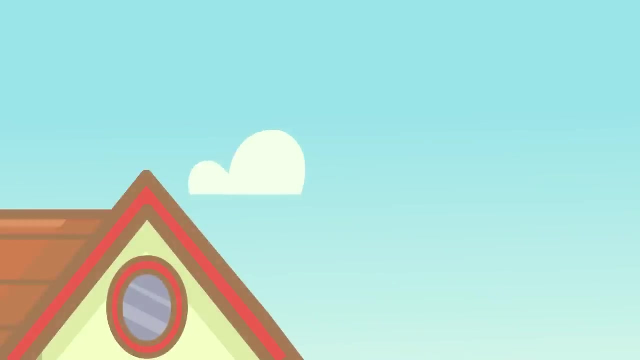 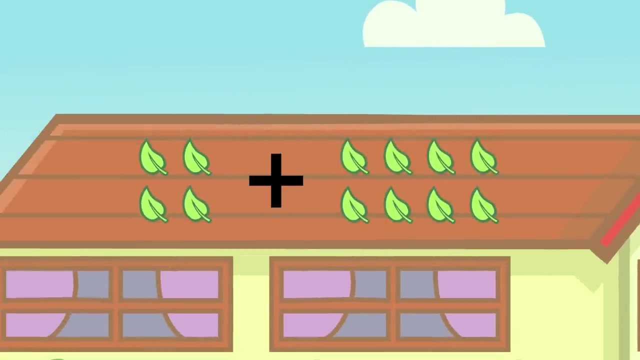 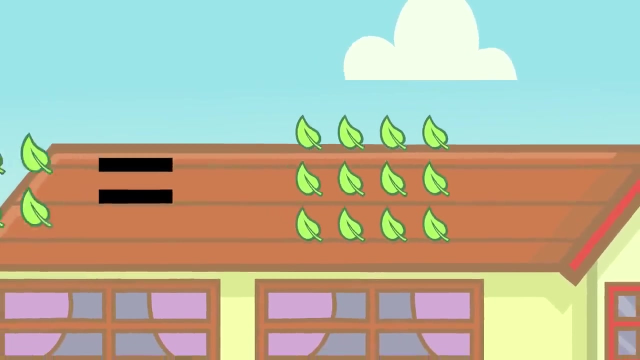 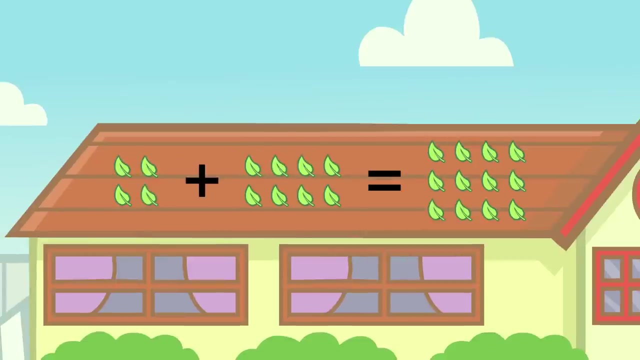 4 plus 8 equals 12.. 4 plus 8 equals 12.. 4 plus 8 equals 12.. 1,, 2,, 3,, 4,, 5,, 6,, 7,, 8,, 9,, 10,, 11,, 12 equals. 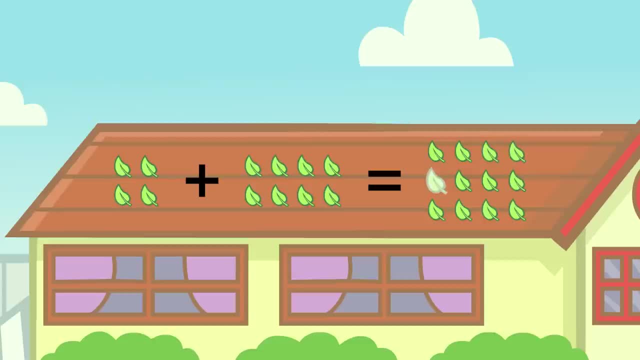 1,, 2,, 3,, 4,, 5,, 6,, 7,, 8,, 9,, 10,, 11, 12 equals 1,, 2,, 3,, 4,, 5,, 6,, 7,, 8,, 9,, 10,, 11,, 12.. 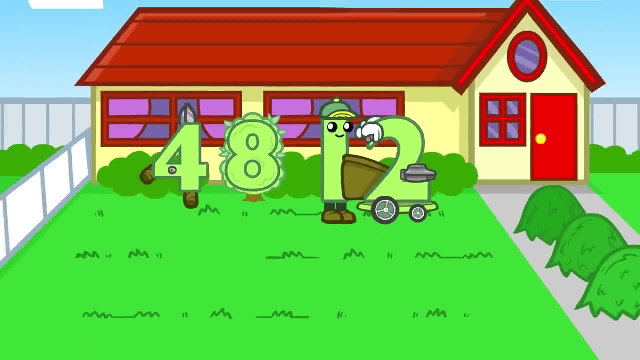 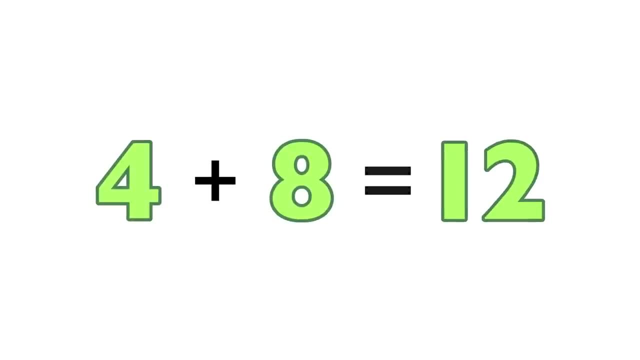 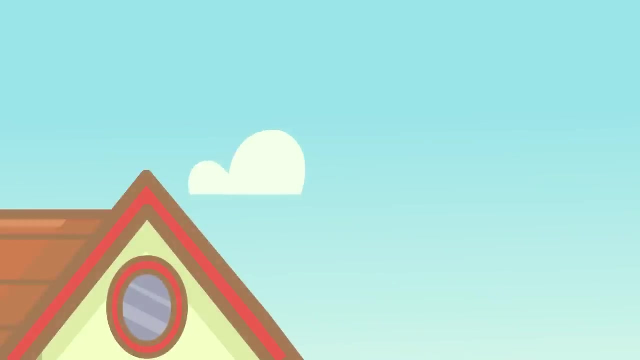 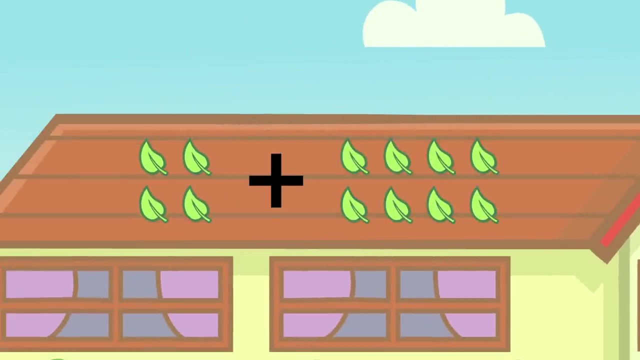 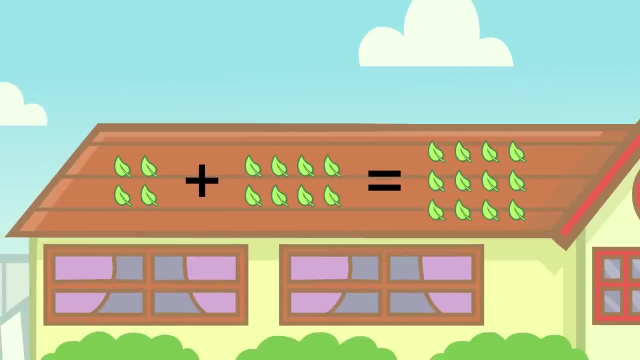 1,, 2,, 3,, 4,, 5,, 6,, 7,, 8,, 9,, 10,, 11, 12 equals 1,, 2,, 3,, 4,, 5,, 6,, 7,, 8,, 9,, 10,, 11, 12. 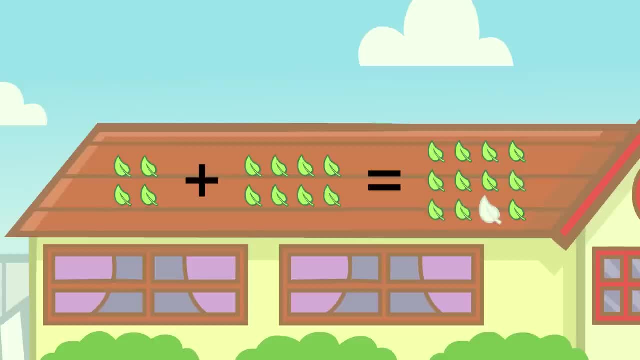 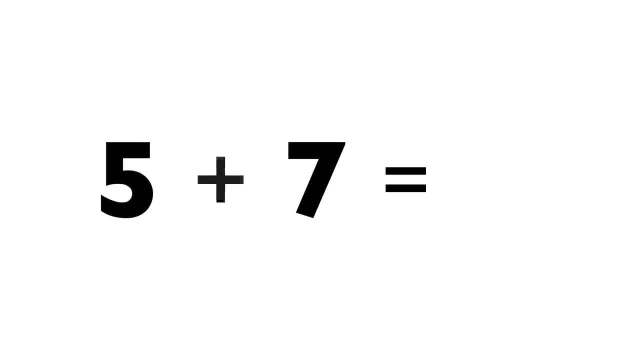 1,, 2,, 3,, 4,, 5,, 6,, 7,, 8,, 9,, 10,, 11, 12. 5 plus 7 equals 5 plus 7 equals 12. 5 plus 7 equals 12. 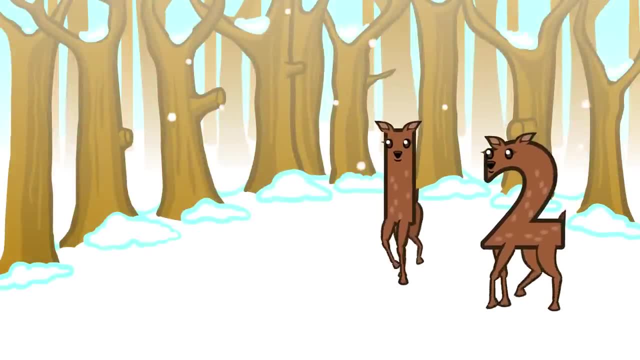 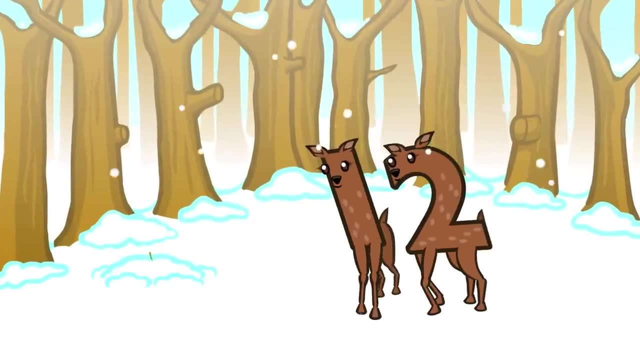 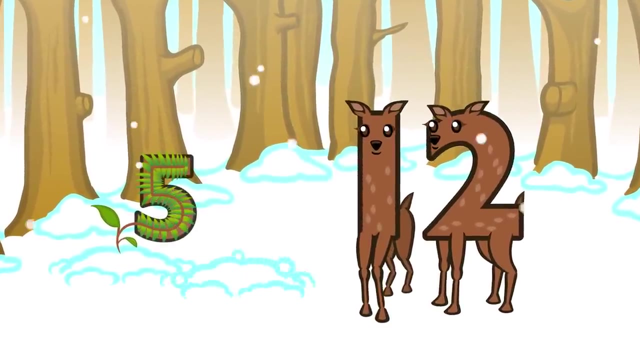 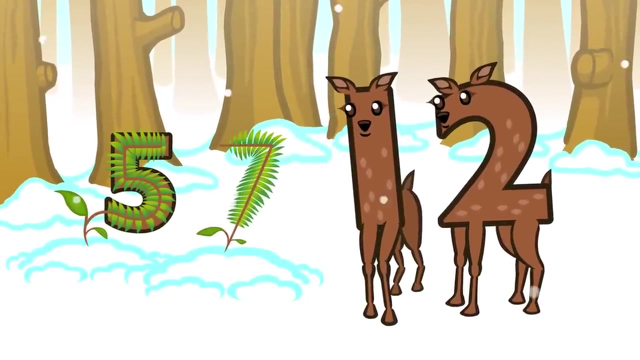 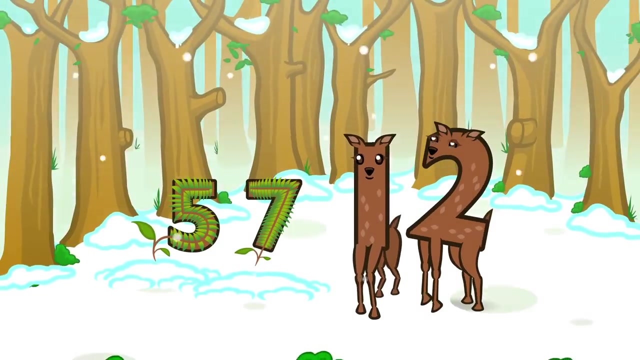 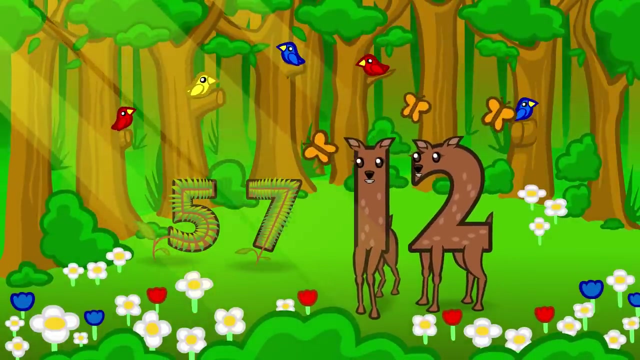 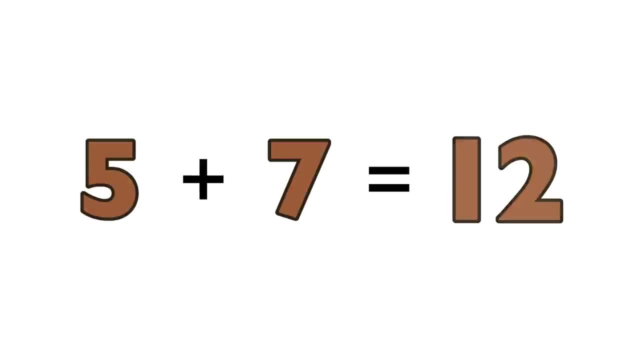 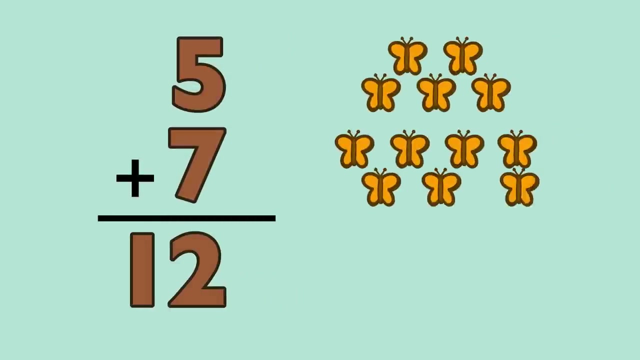 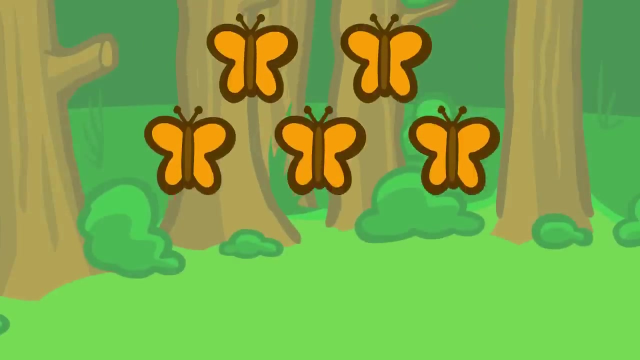 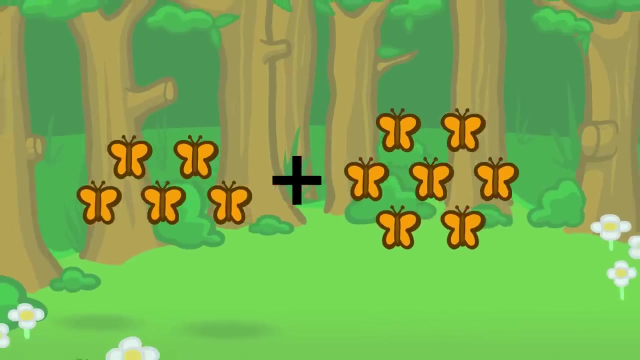 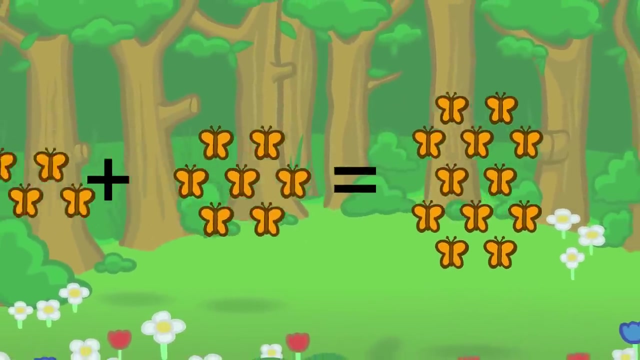 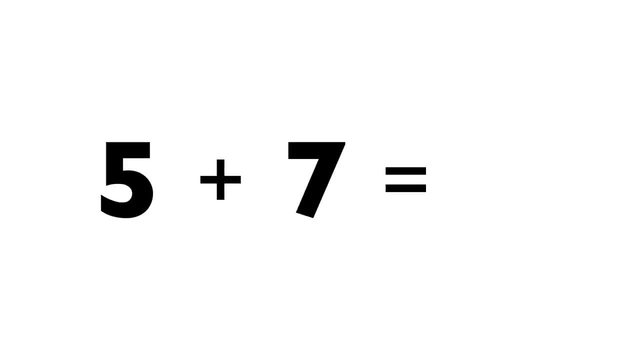 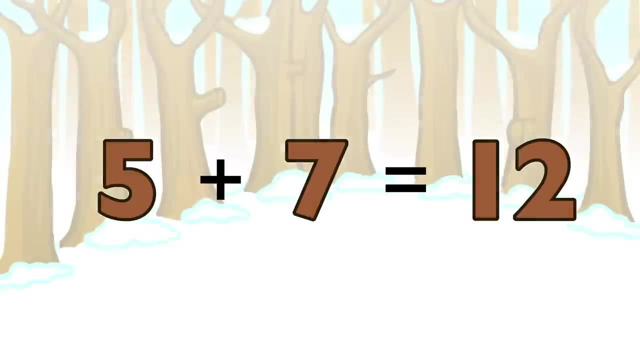 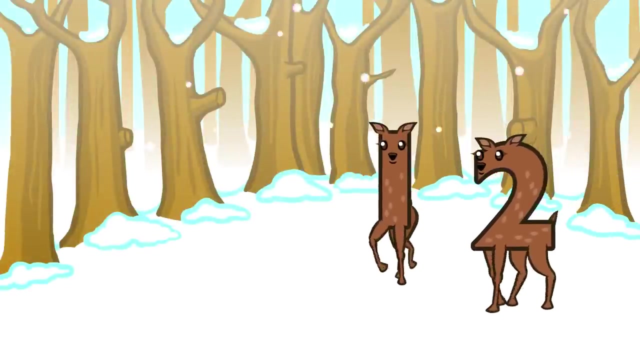 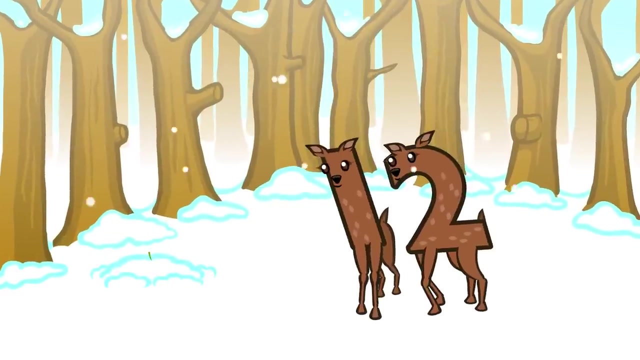 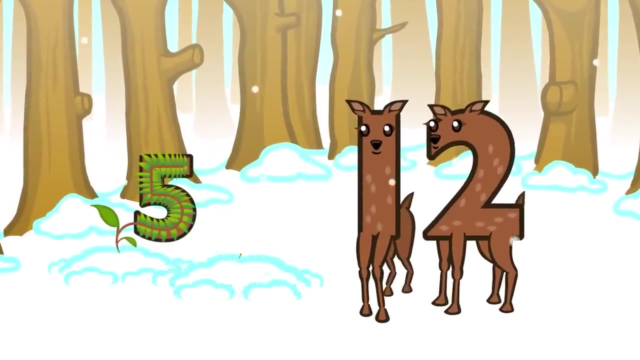 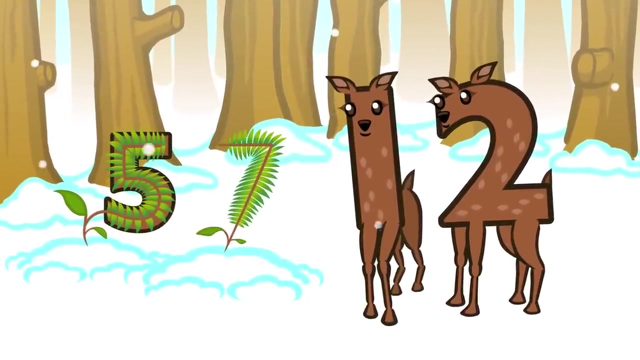 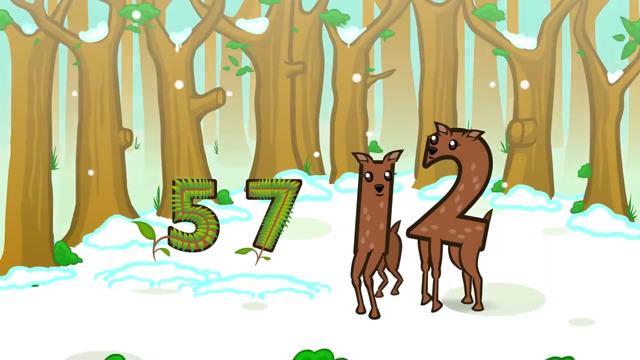 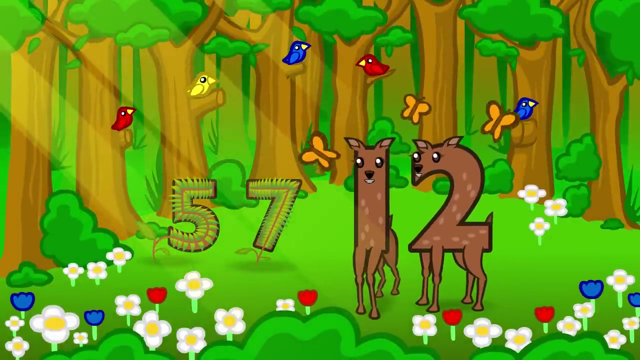 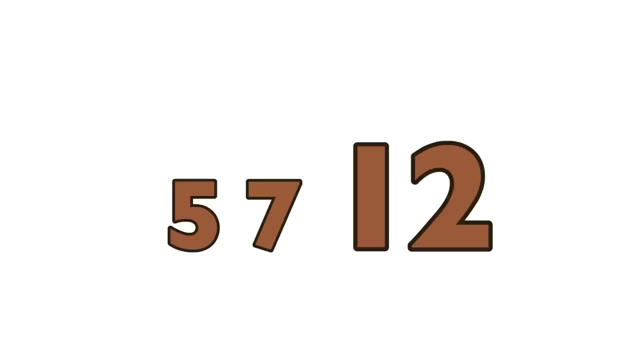 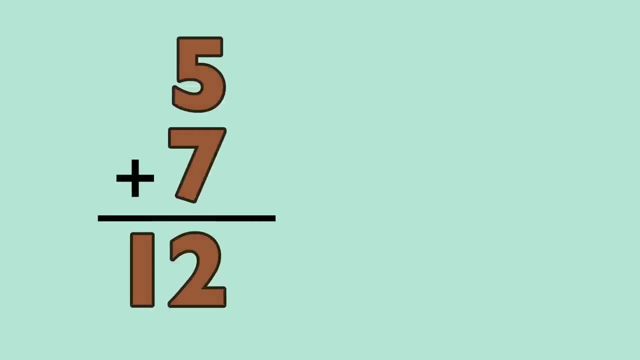 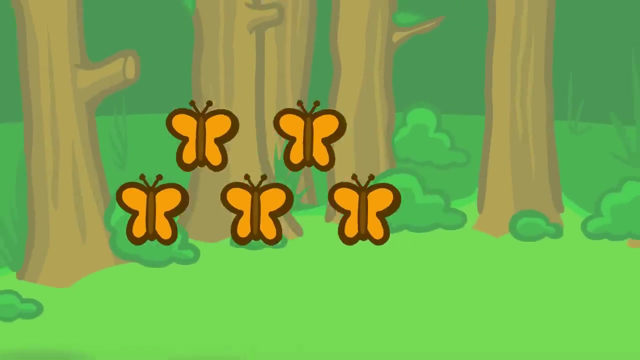 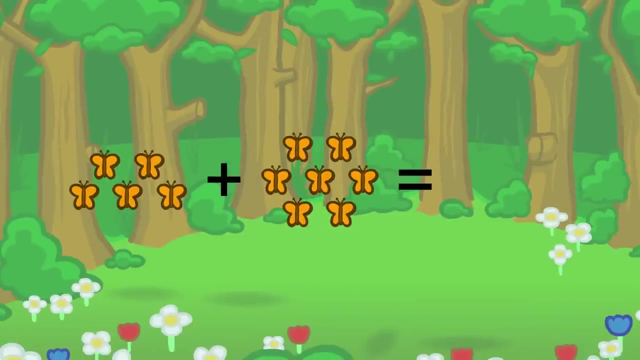 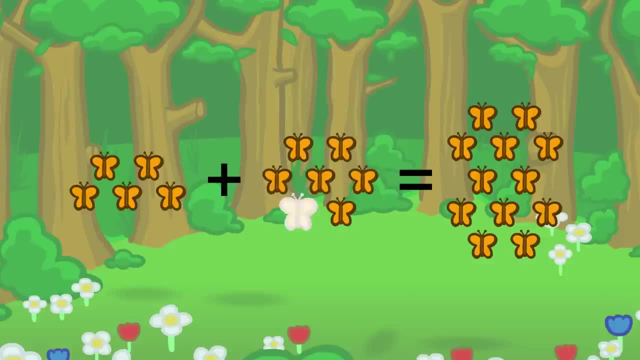 5,, 6,, 7,, 8,, 9,, 10,, 11, 12 equals 1,, 2,, 3,, 4,, 5,, 6,, 7,, 8,, 9,, 10,, 11, 12.. 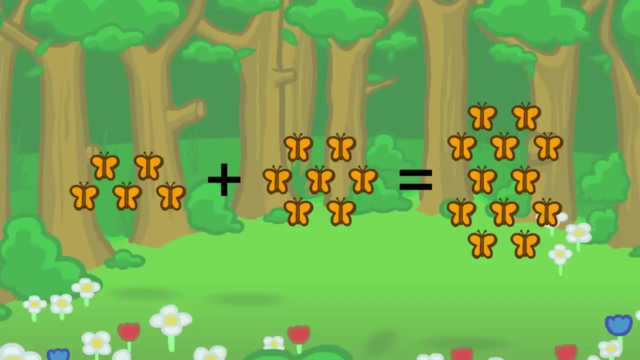 1,, 2,, 3,, 4,, 5,, 6,, 7,, 8,, 9,, 10,, 11, 12 equals 1,, 2,, 3,, 4,, 5,, 6,, 7,, 8,, 9,, 10,, 11,, 12.. 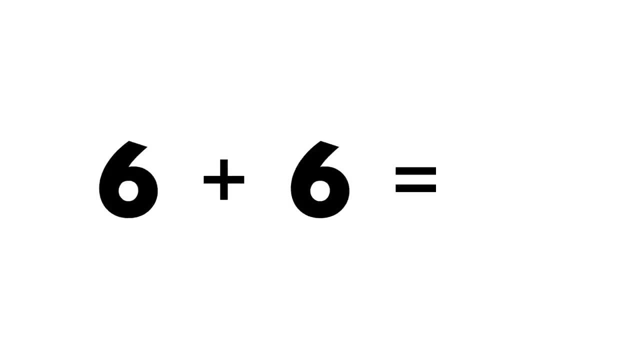 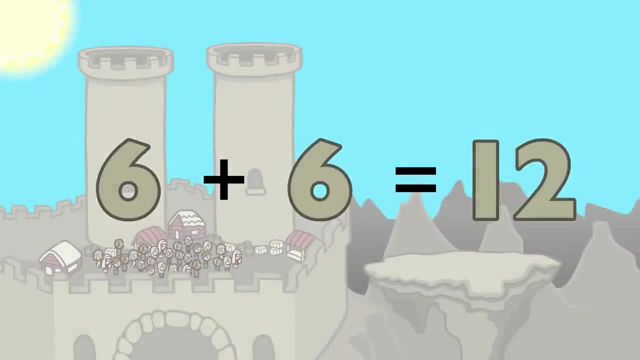 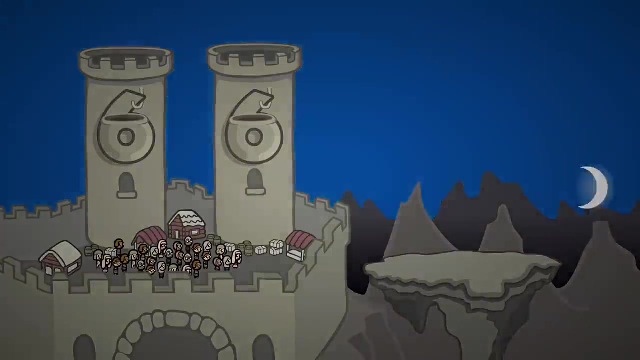 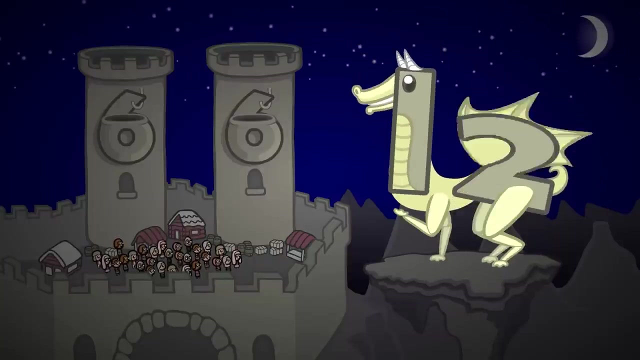 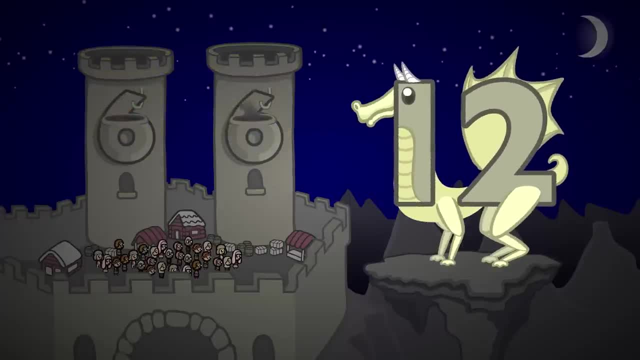 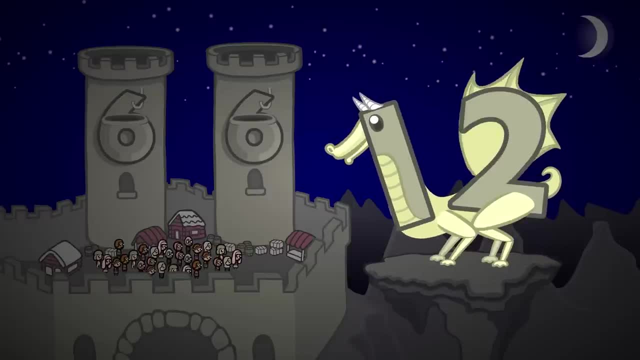 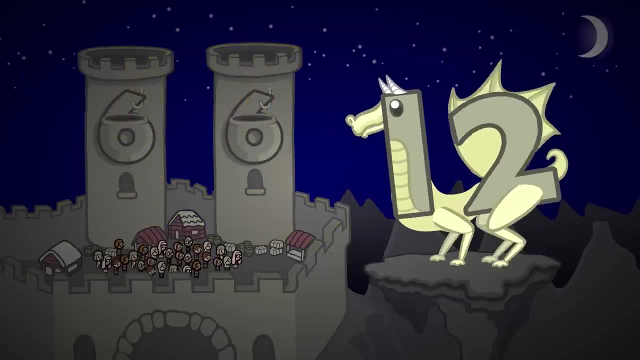 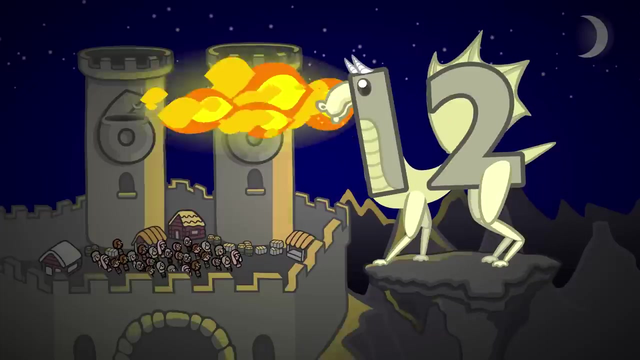 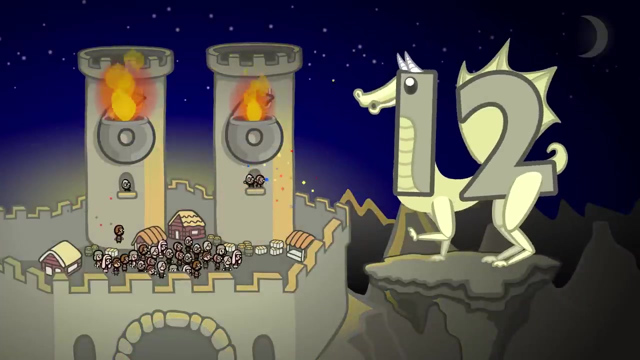 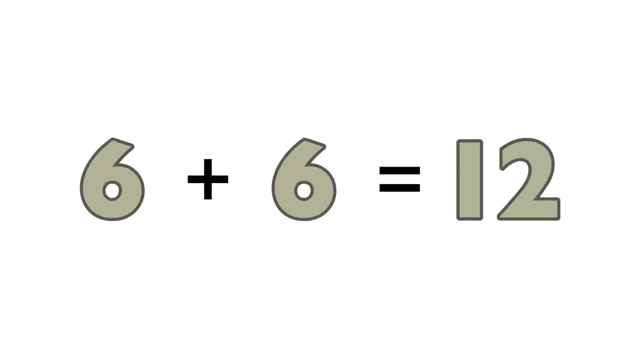 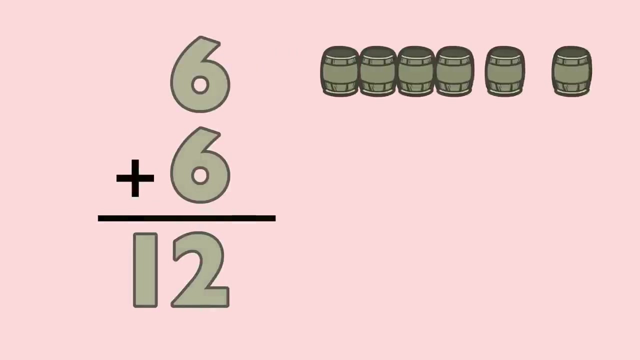 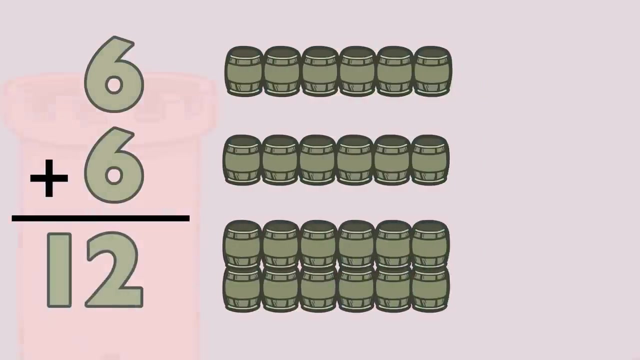 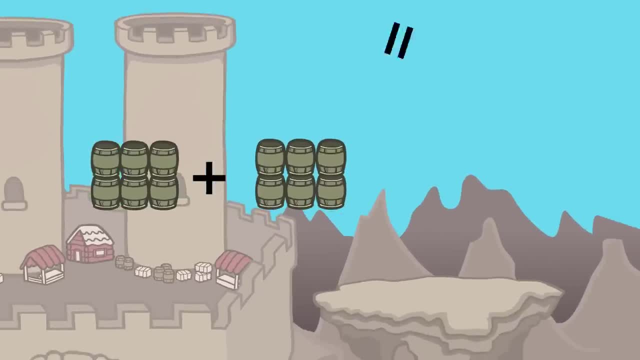 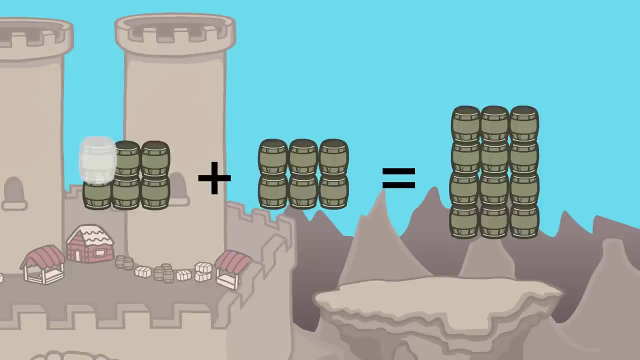 Six equals twelve: One, two, three, four, five, six, seven, eight, nine, ten eleven twelve equals One, two, three, four, five, six, seven, eight, nine, ten, eleven, twelve. 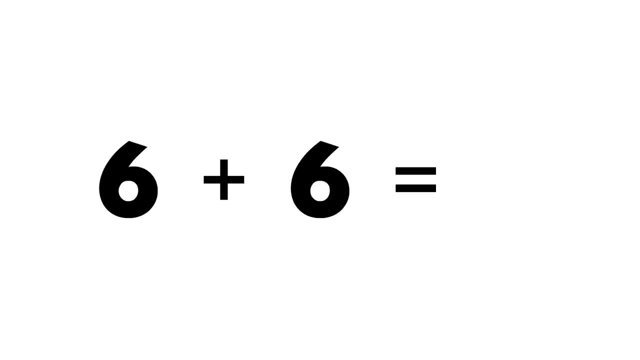 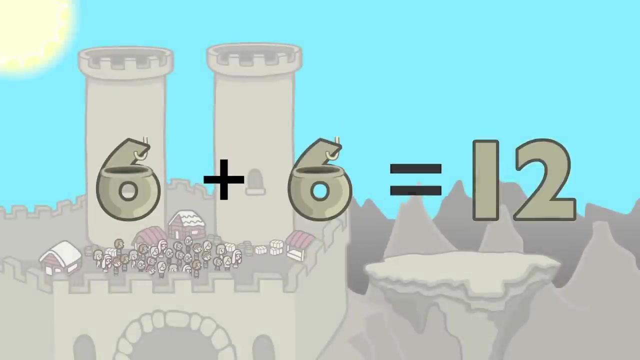 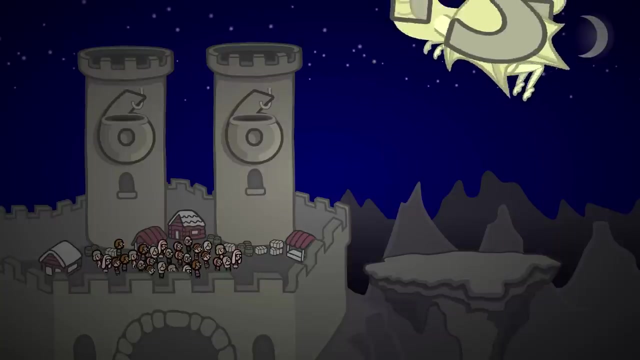 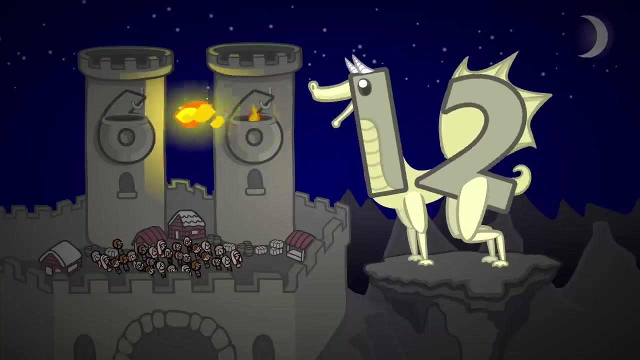 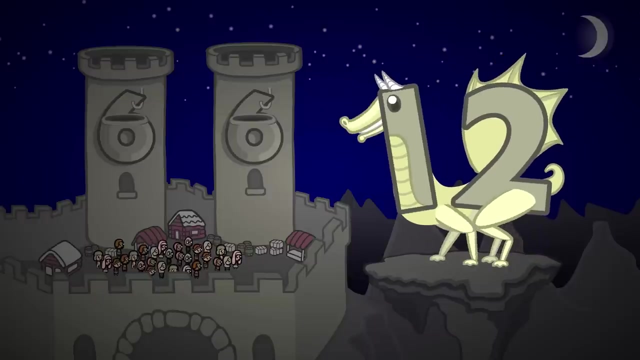 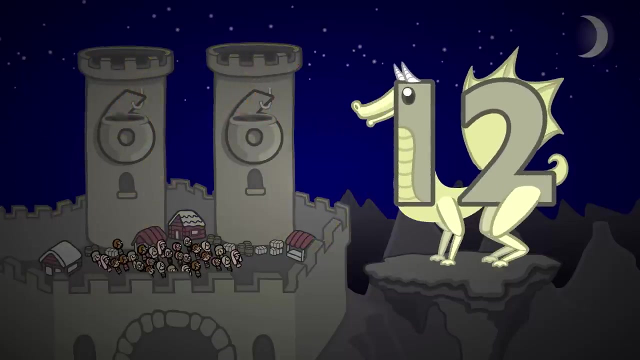 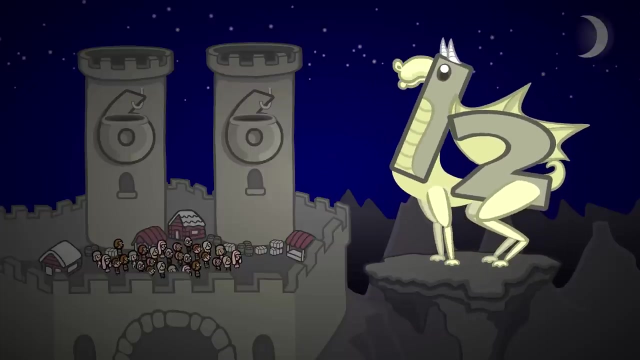 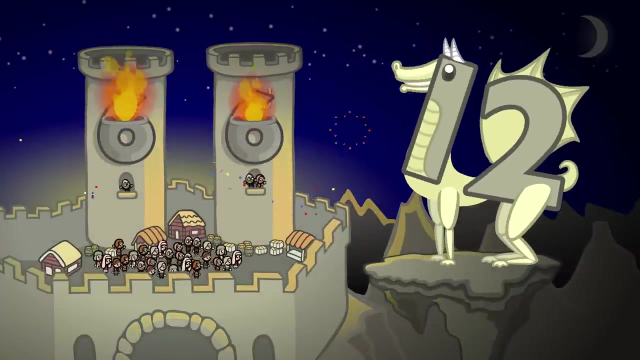 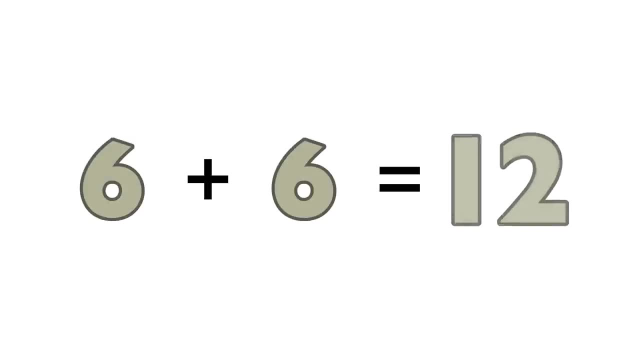 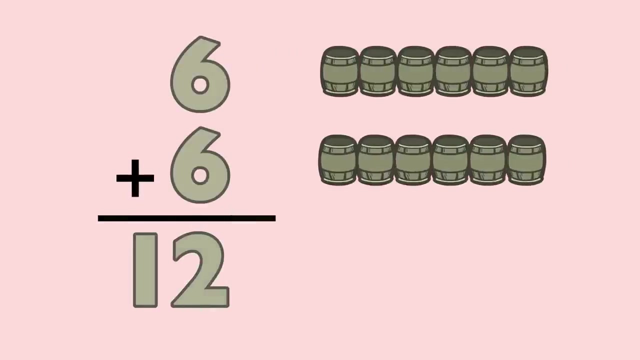 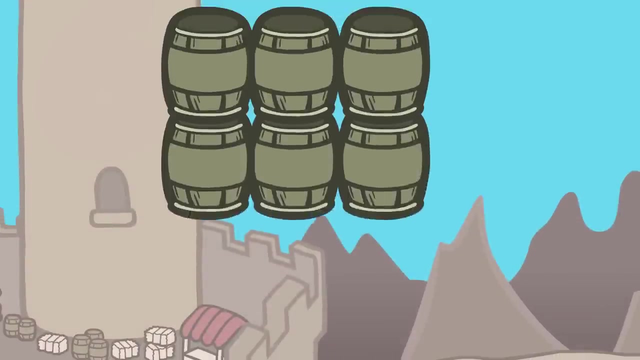 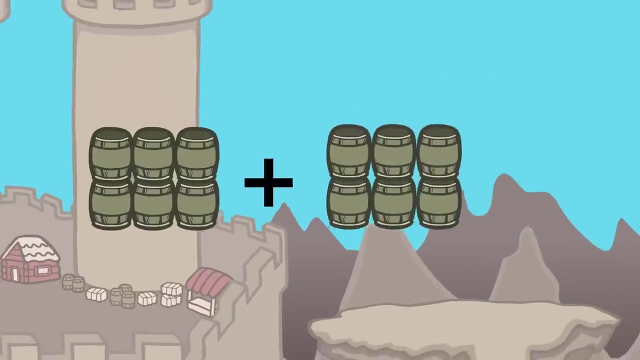 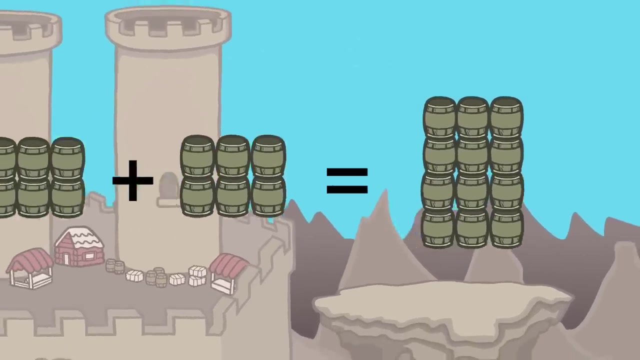 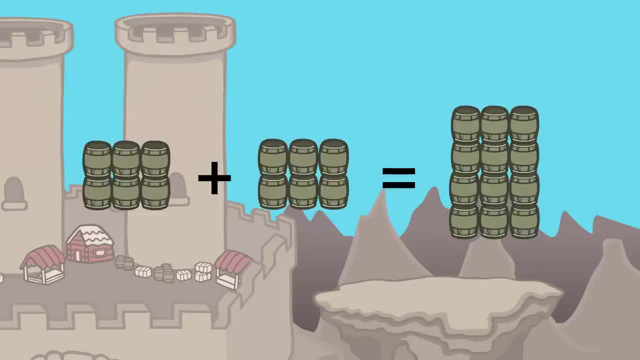 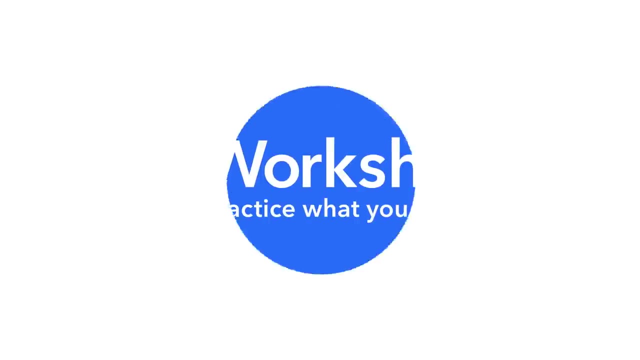 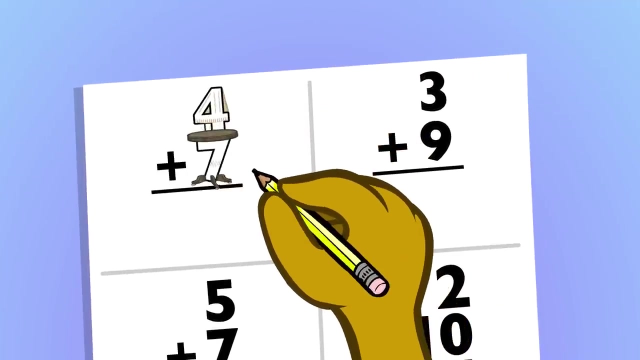 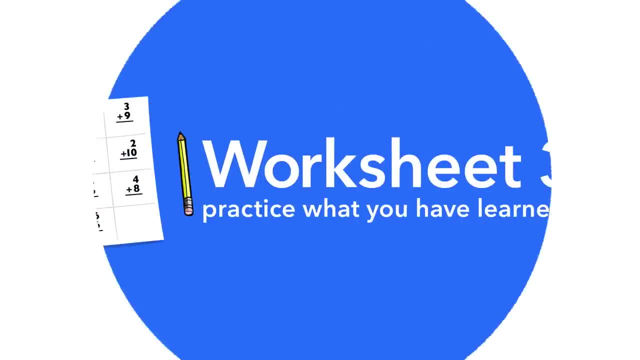 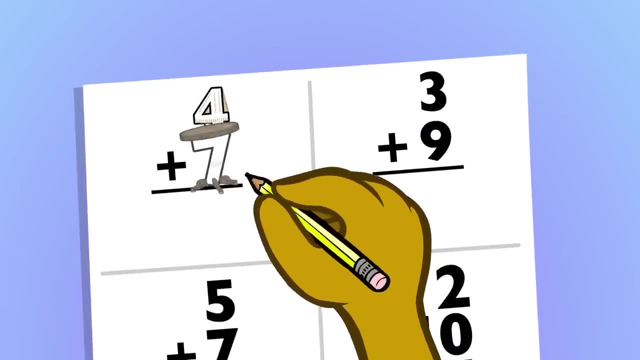 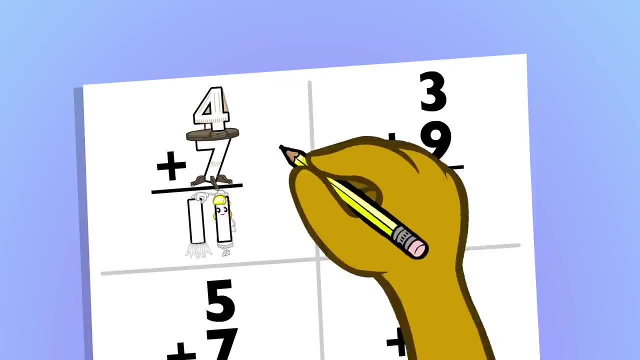 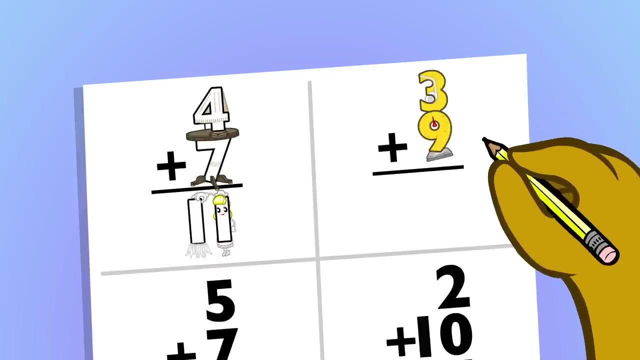 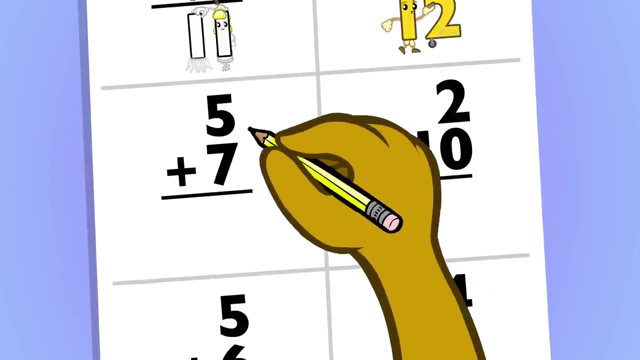 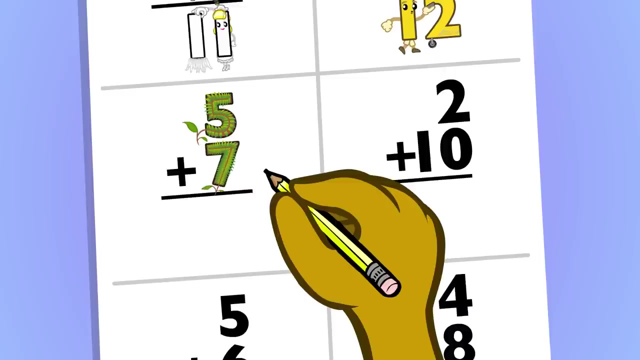 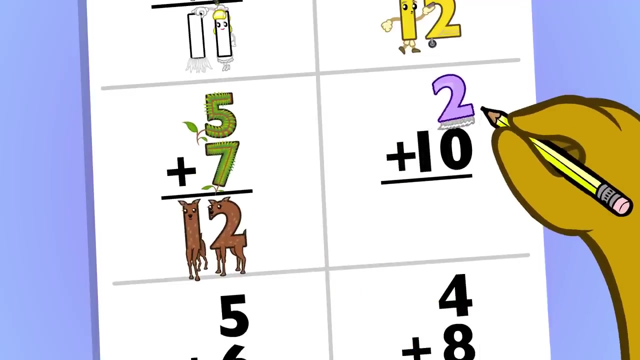 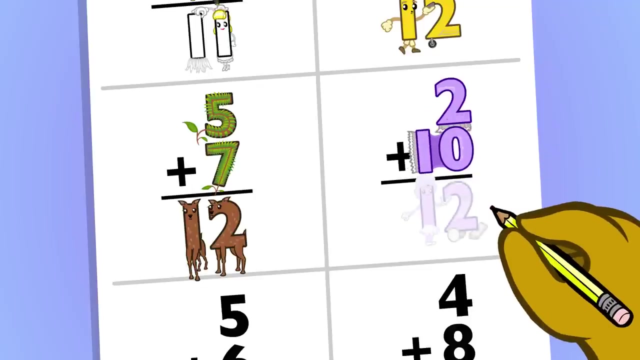 One, two, three, four, five, six, seven, eight, nine, ten, eleven. twelve Four plus seven equals Eleven. Three plus Nine equals Twelve. Five plus seven equals Twelve. Two plus ten equals. 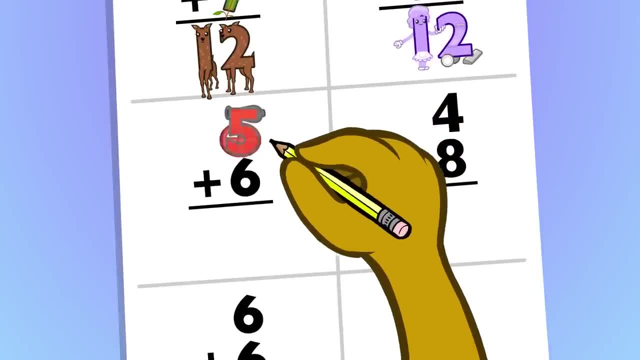 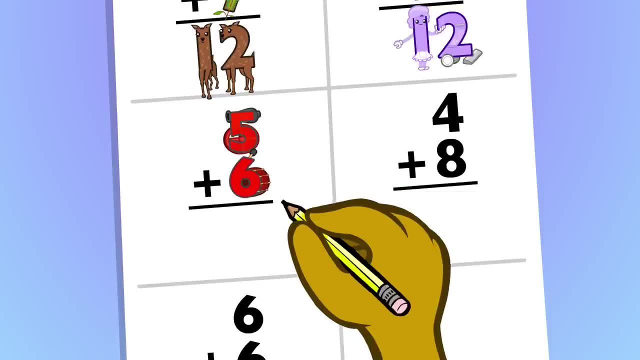 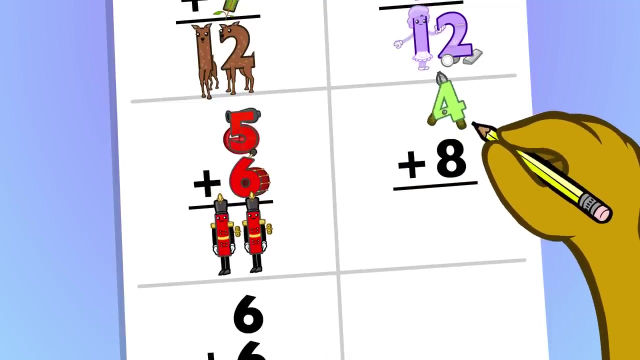 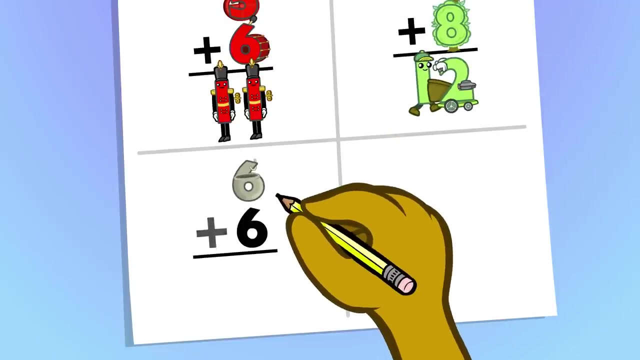 Twelve Five plus six equals Twelve. Eleven plus eight equals Eleven Four plus eight equals Four plus eight: equals Twelve Four plus eight: equals Ten plus seven: equals Ten plus eight. equals. Seven plus nine equals Twelve Six. 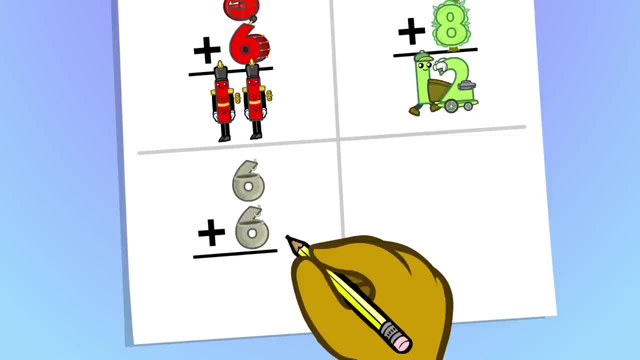 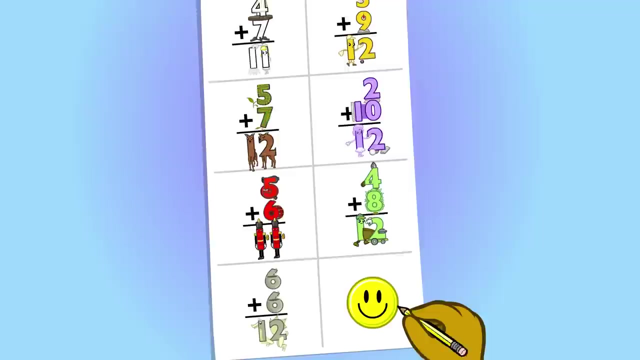 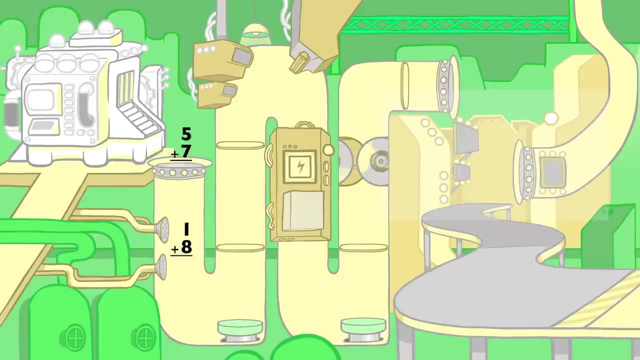 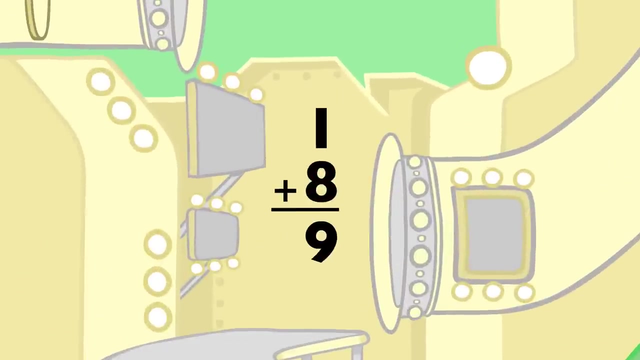 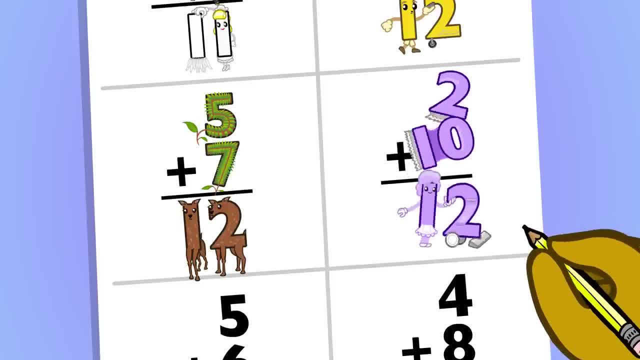 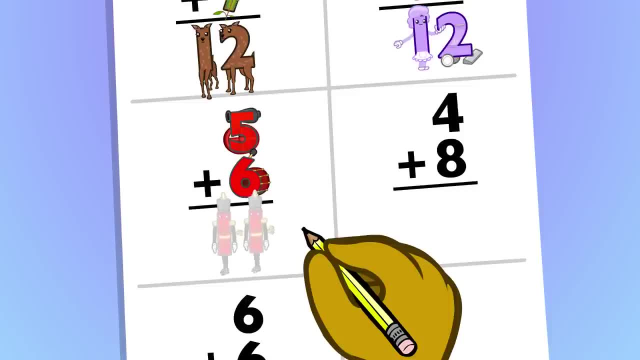 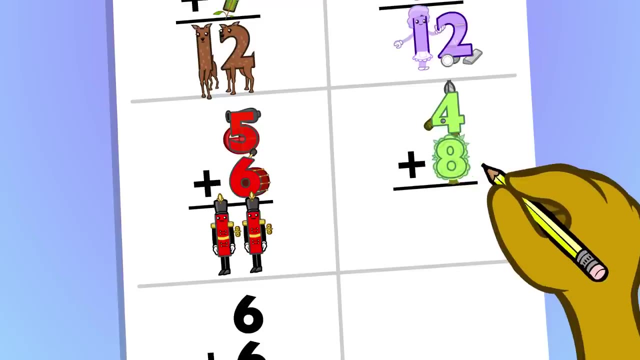 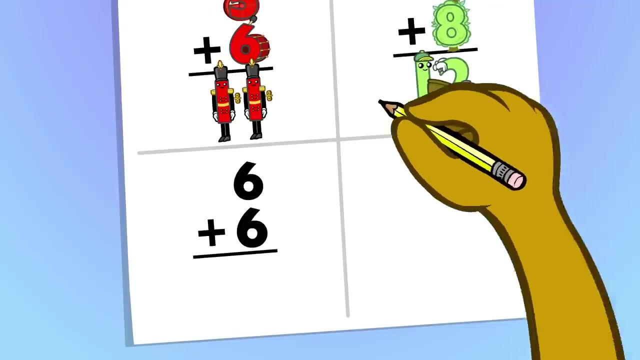 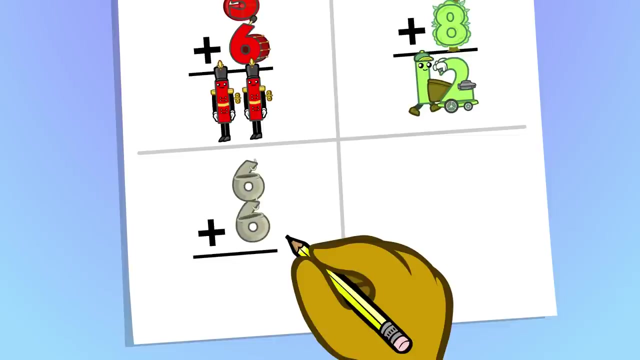 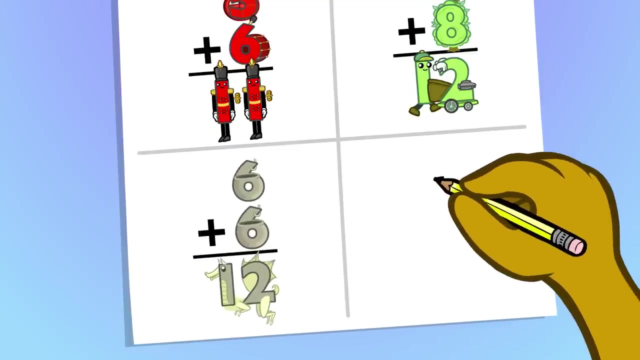 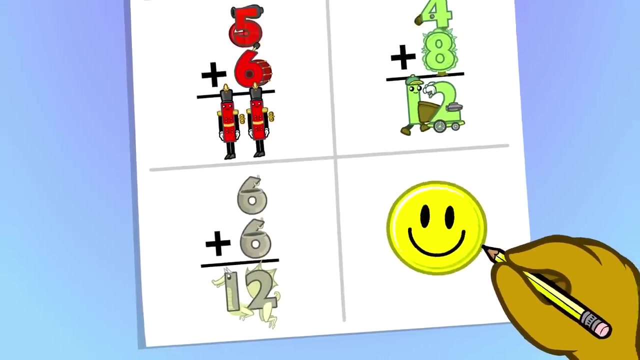 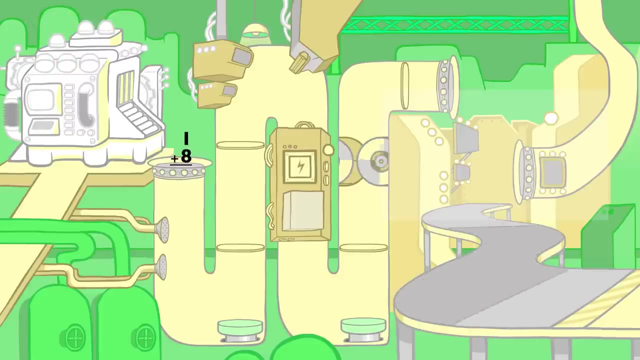 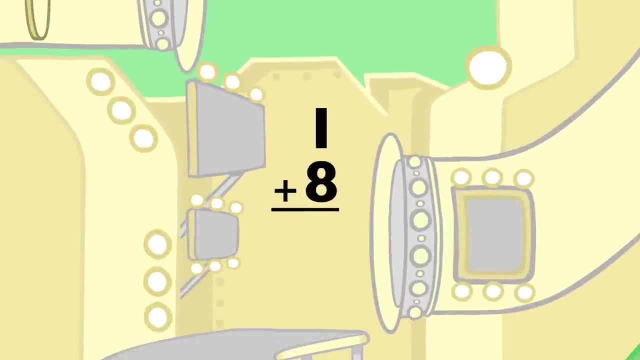 1, 2, 7, 9, 10, 11 equals 12.. 11, 4 Plus 8 Equals 12. 6 Plus 6 Equals 12. 1 Plus 8, Equals 9 And 8 Plus 1. 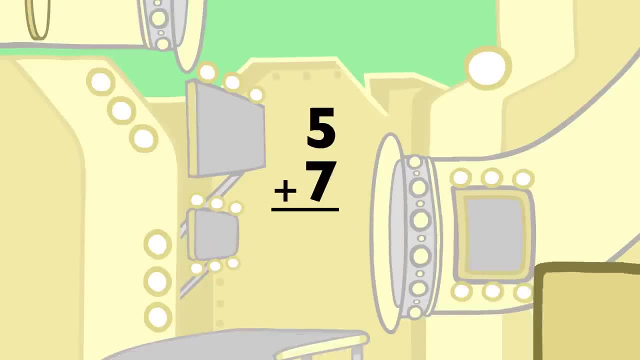 Equals 9, 5 Plus 7 Equals 12, And 7 Plus 5 Equals 12. 2 Plus 10 Equals 12. 10 Plus 2 Equals 12, 3 Plus 7 Equals 10. 7 Plus 3 Equals 10. 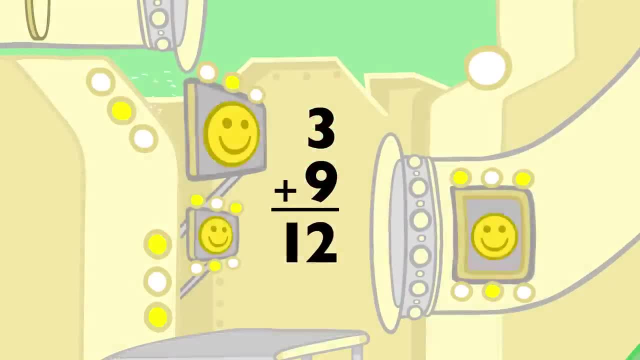 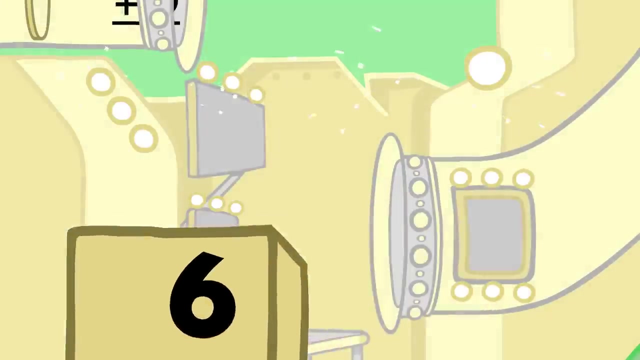 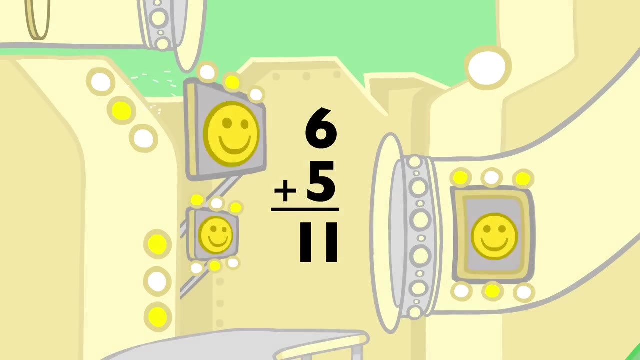 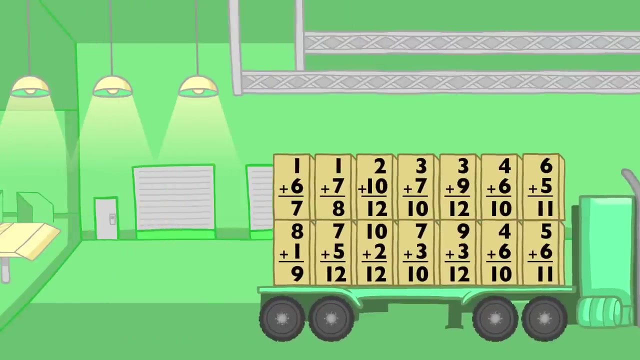 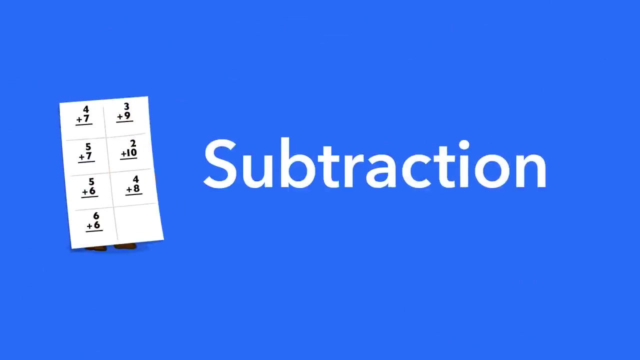 3 Plus 9- Equals 12. 9 Plus 3- Equals 12. 4 Plus 6- Equals 10. 6 Plus 4- Equals 10. 5 Plus 6- Equals 11. 6 Plus 5- Equals 11 Plus 7. 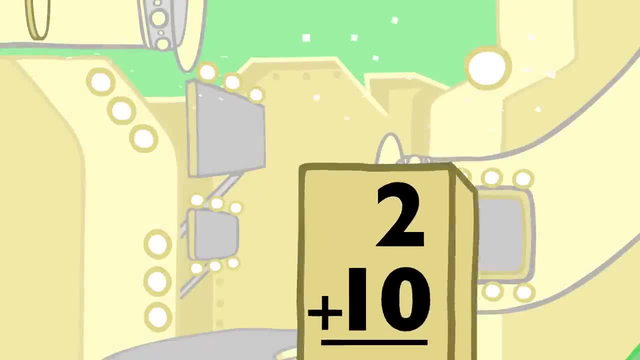 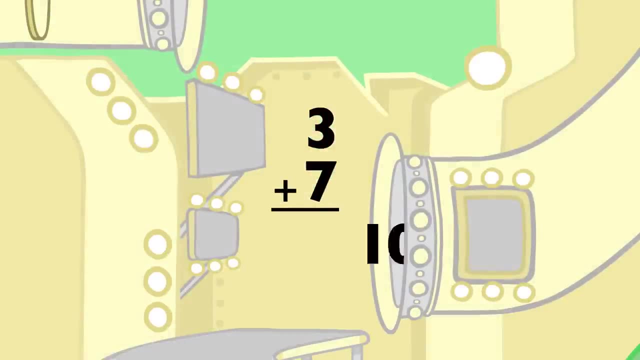 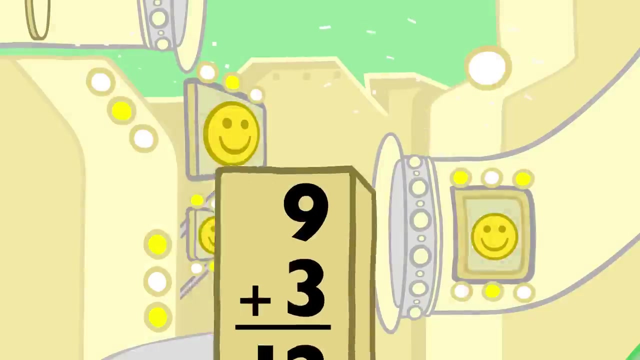 2 plus 10 equals 12. 10 plus 2 equals 12. 3 plus 7 equals 10. 7 plus 3 equals 10. 3 plus 9 equals 12. 9 plus 3 equals 12. 4 plus 6 equals 10. 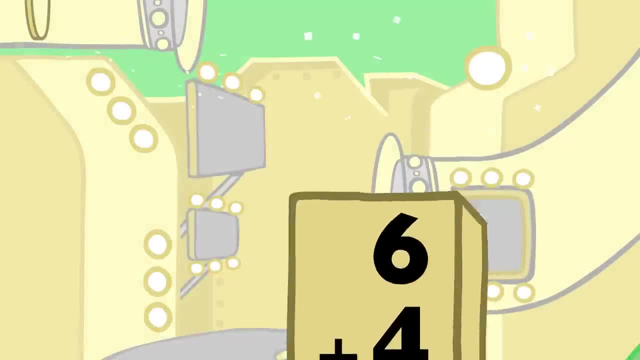 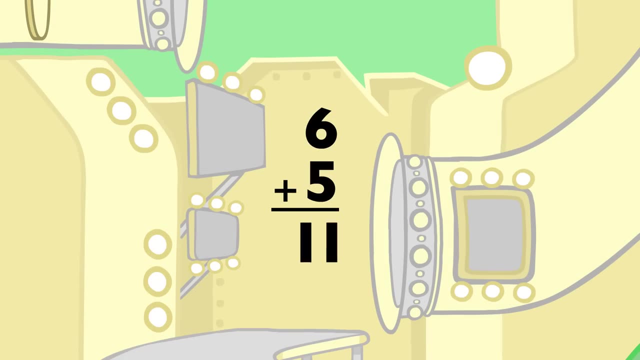 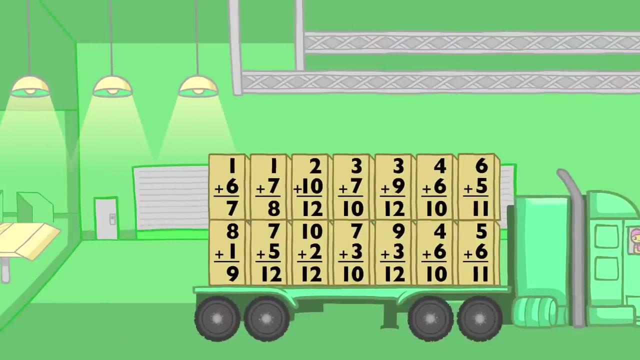 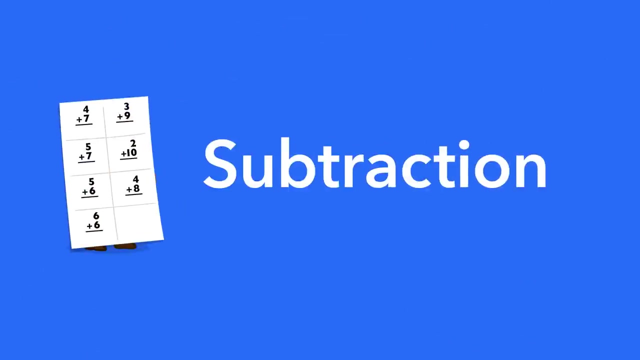 6 plus 4 equals 10. 5 plus 6 equals 10. 6 plus 5 equals 11. 6 plus 5 equals 11. Now that you've learned the math facts, did you know, you can use them for subtraction. 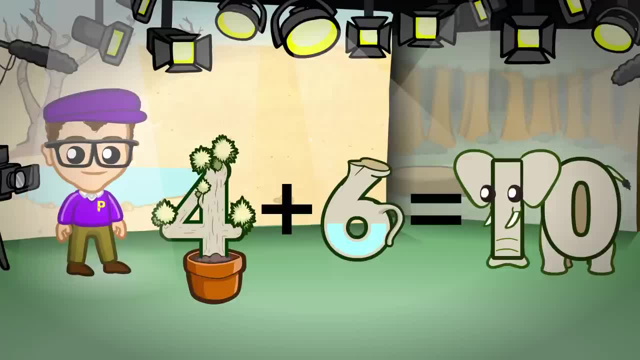 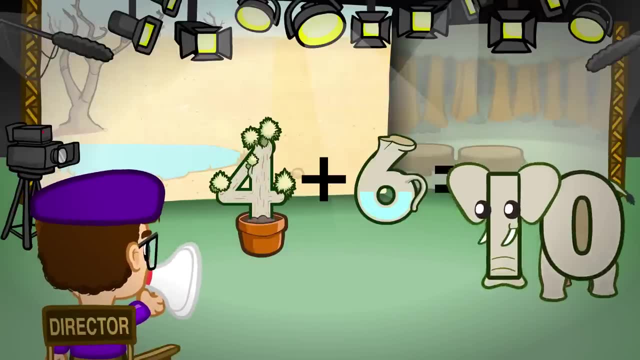 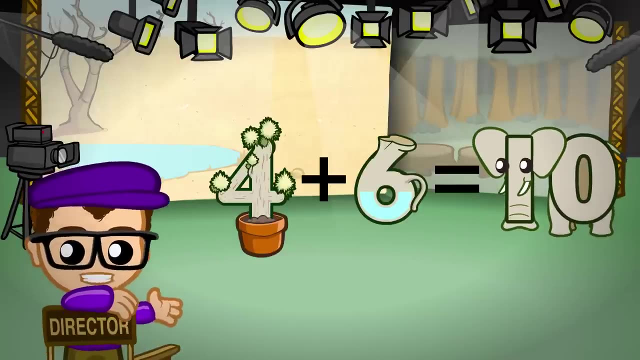 It's easy. I'll show you how. We'll start with the largest number, With the largest number. please step forward. Great, Great. Now we just move the largest number to the beginning. Now we just move the largest number to the beginning. 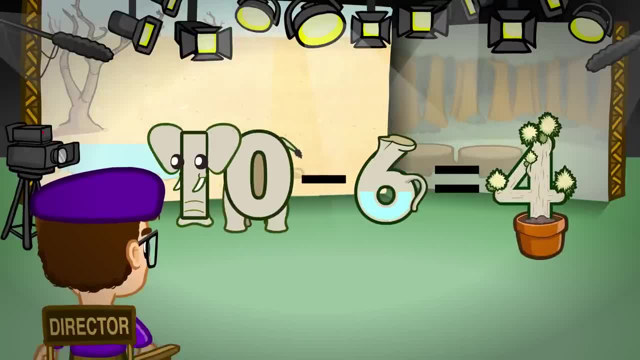 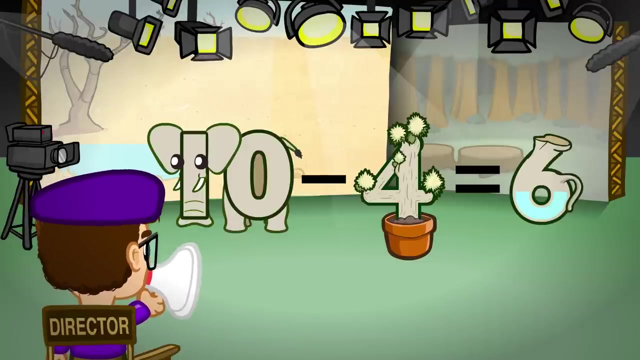 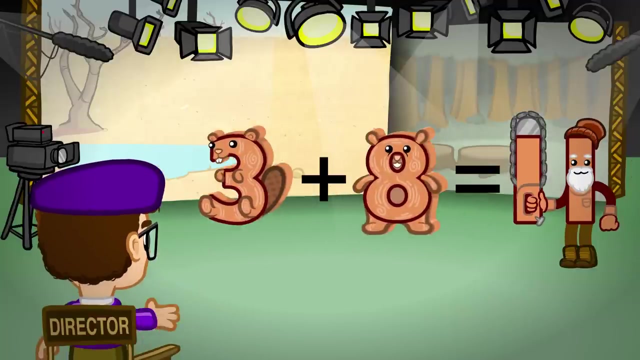 And action: 10 minus 6 equals 4, 10 minus 6 equals 4, 10 minus 6 equals 4. And 10! minus four equals six. cut next group. please would three, eight and eleven take the stage with the largest number. please step forward. great, okay, biggest number. 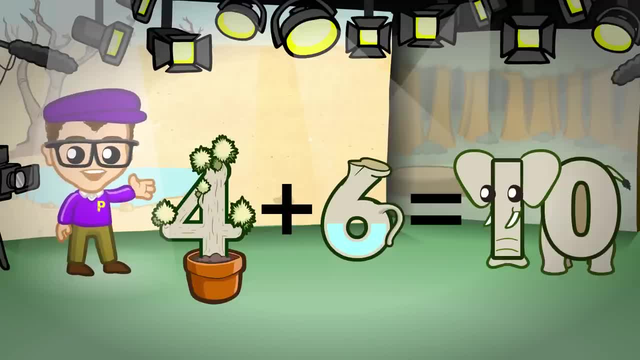 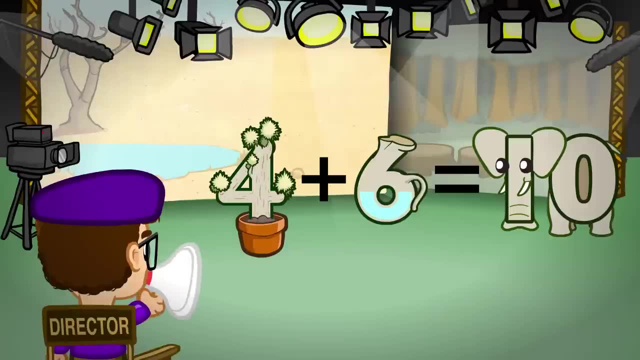 Now that you've learned the math facts, did you know you can use them for subtraction? It's easy. I'll show you how. With the largest number, please step forward. Great, Now we just move the largest number to the beginning. 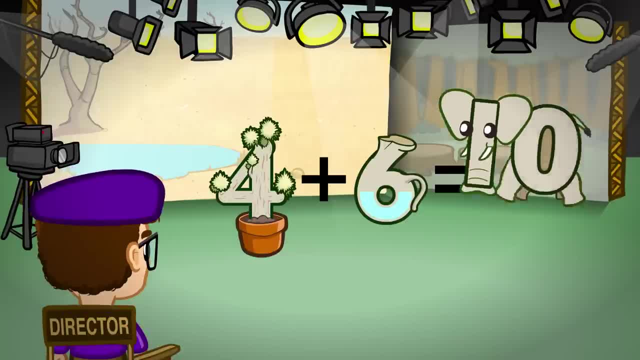 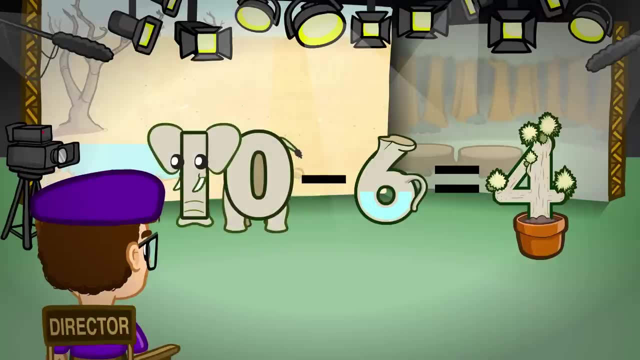 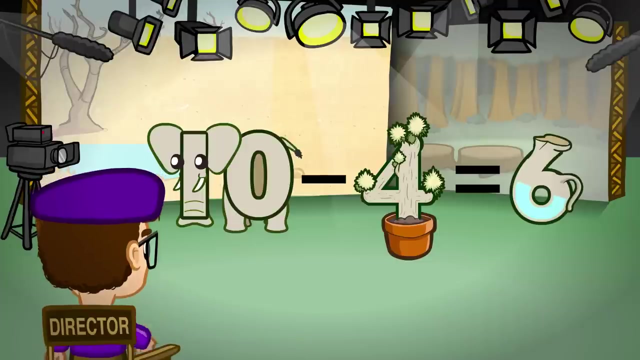 I just moved the largest number to the beginning And Action: 10 Minus 6 Equals 4 And 10 Minus 4 Equals 6. Cut Next group. Please Would 3,, 8, and 11 take the stage. 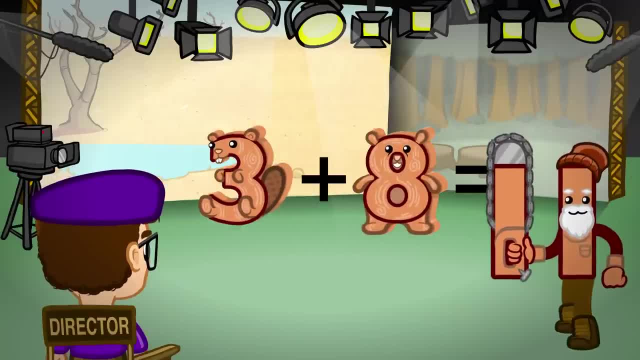 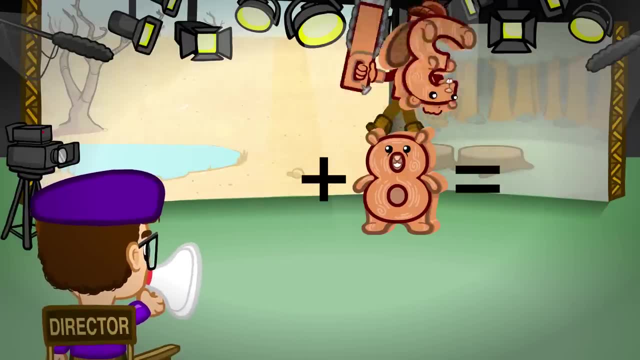 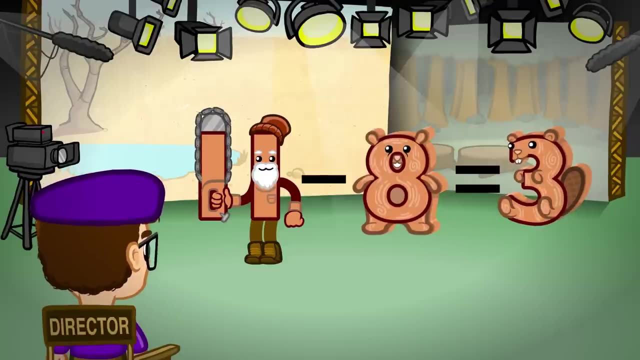 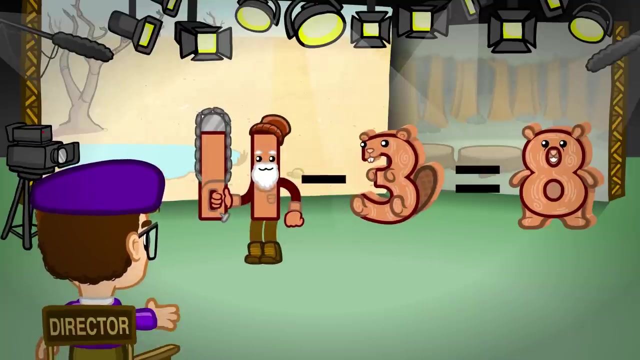 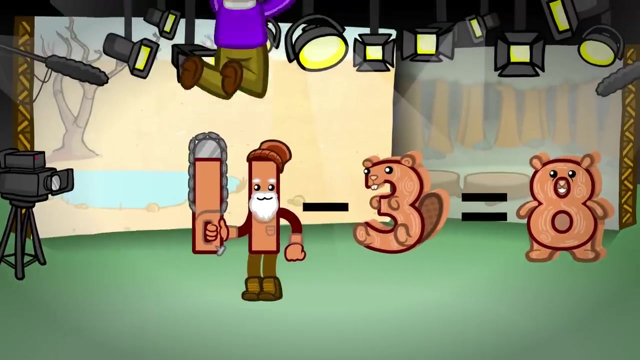 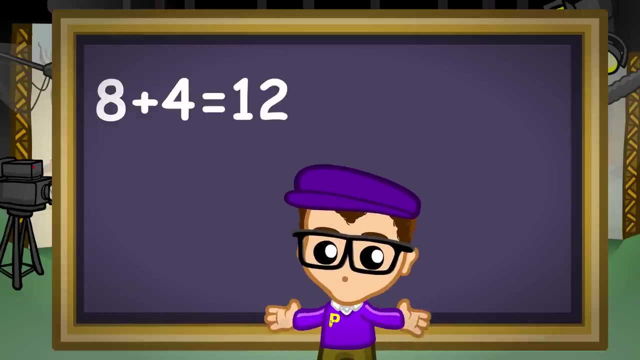 Would the largest number please step forward. Great, Okay, biggest number, Please move to the beginning. 11 Minus 8 Equals 3, And 11 Minus 3 Equals 8. Now you try a few: 8 Plus 4. 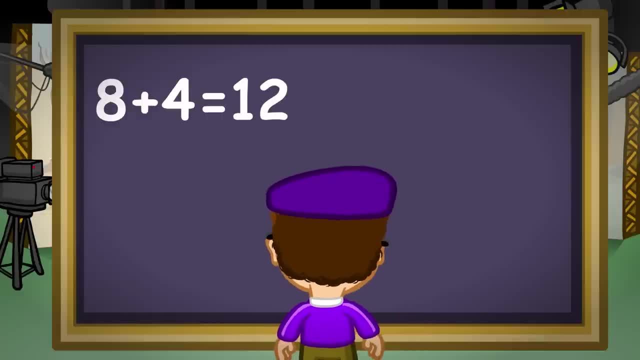 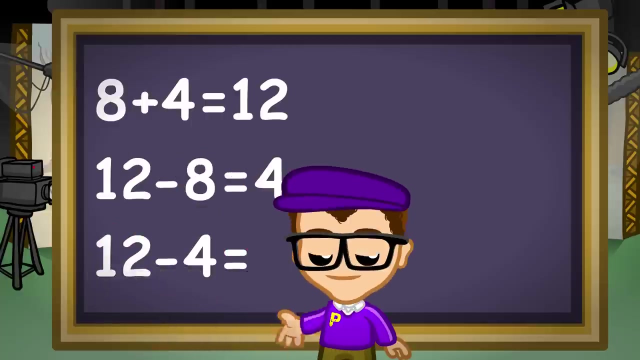 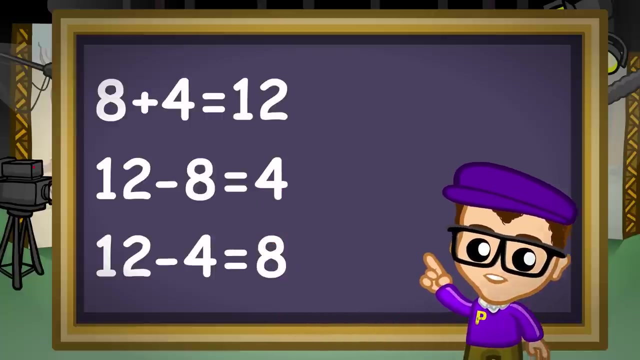 Equals 12. So 12 Minus 8 Equals 4!- Right 4!. And 12 Minus 4 Equals 8!. That's right 8!. Let's try another: 12 Minus 4. 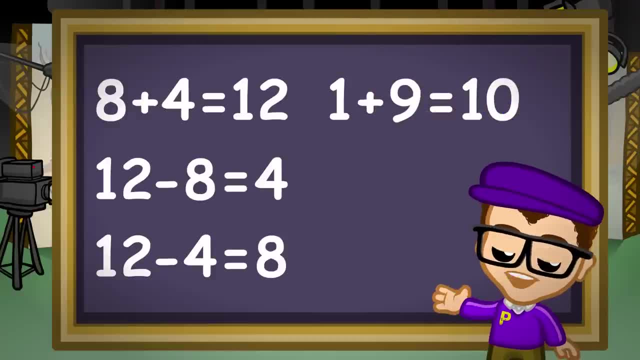 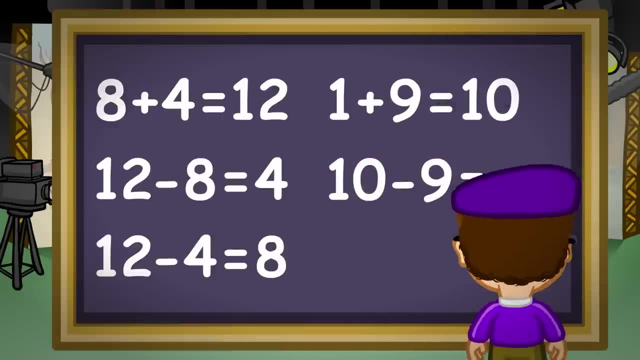 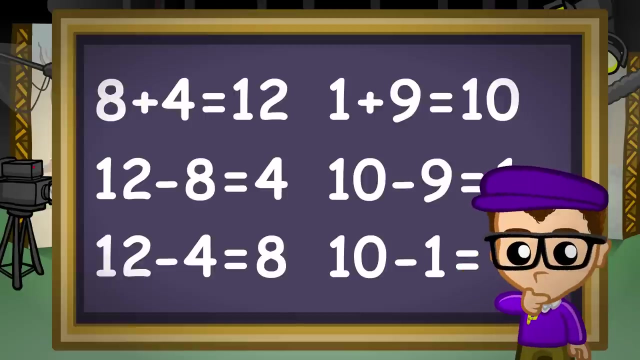 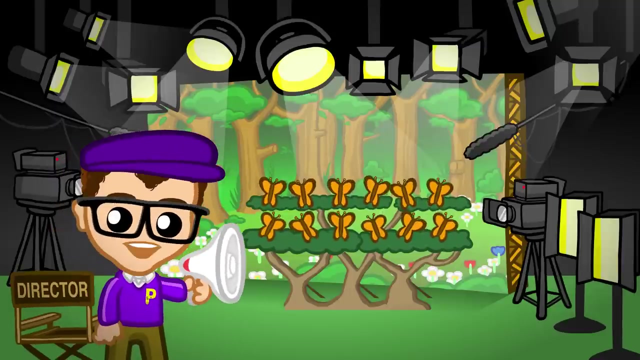 Equals 1 Plus 9 Equals 10! So 10 Minus 9 Equals 1! Right, And 10 Minus 1 Equals 9! Right. 12 Minus 5 Equals. 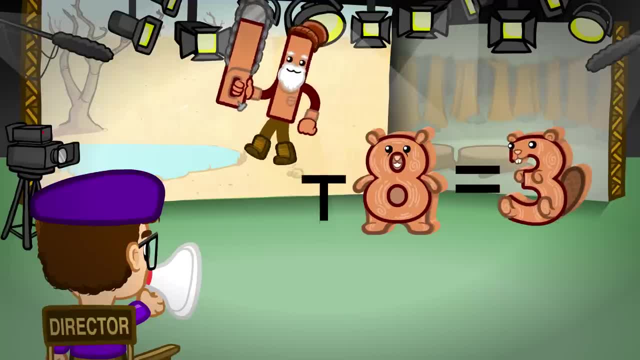 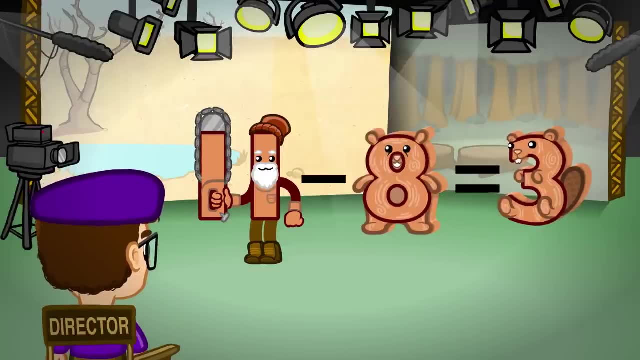 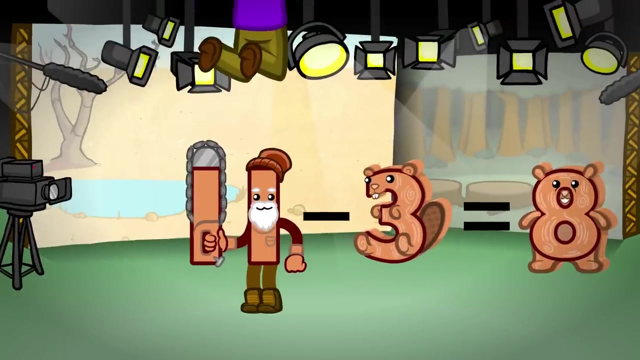 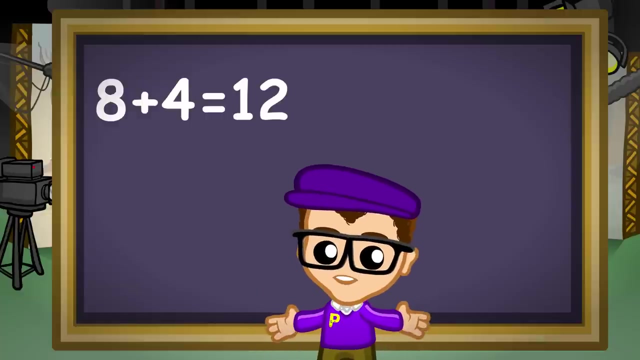 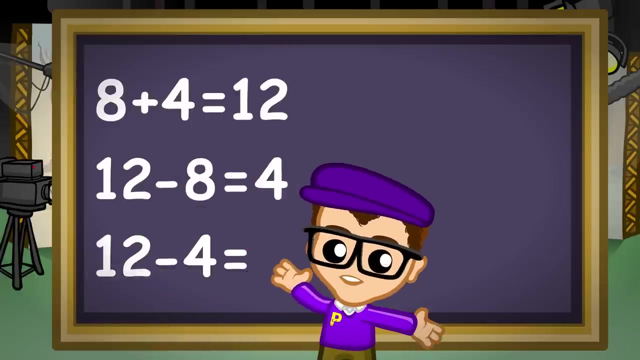 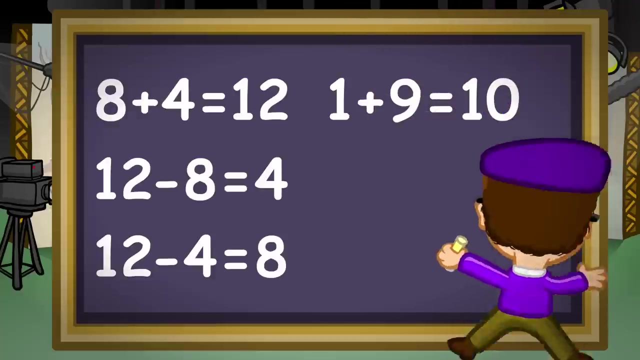 please move to the beginning. eleven minus eight equals three, and eleven minus three equals eight. now you try a few. eight plus four equals twelve. so twelve minus eight equals right four, and twelve minus four equals equals eight. that's right eight. let's try another. one plus nine equals ten. 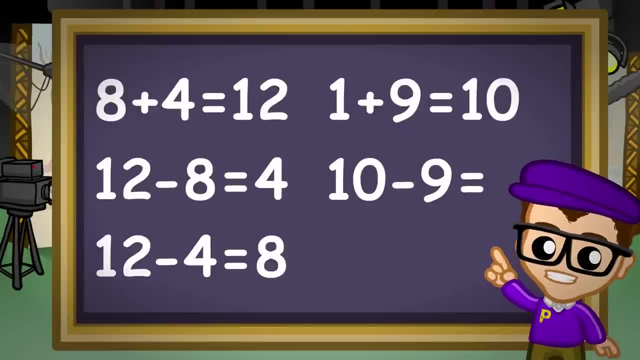 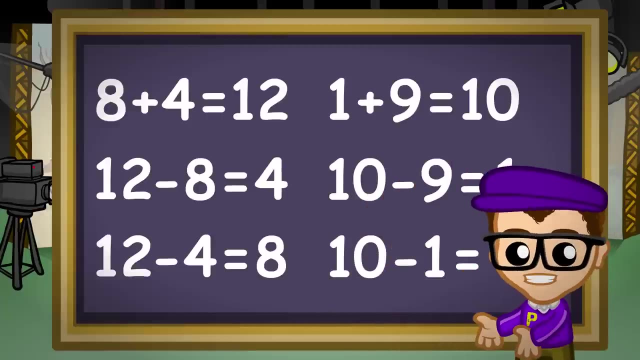 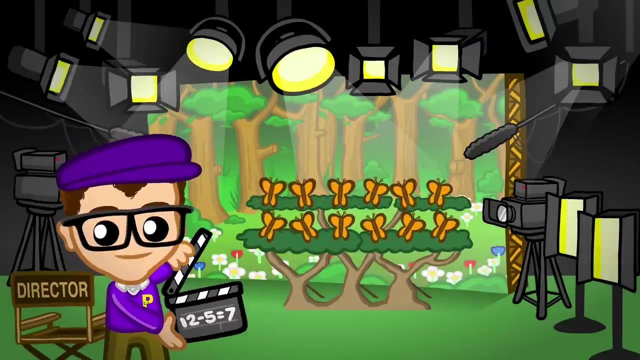 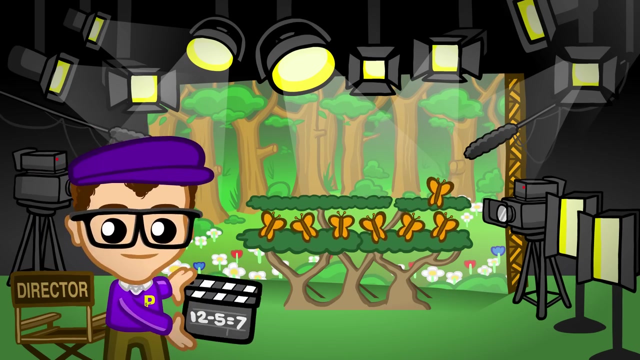 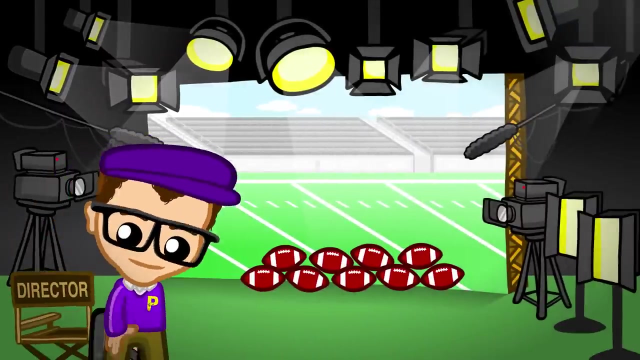 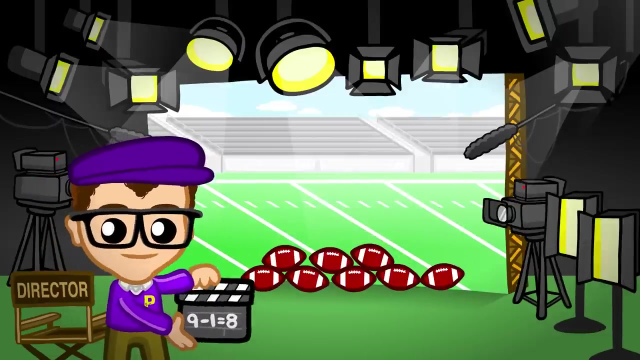 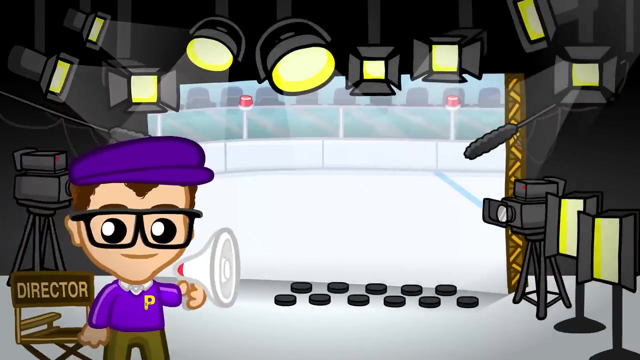 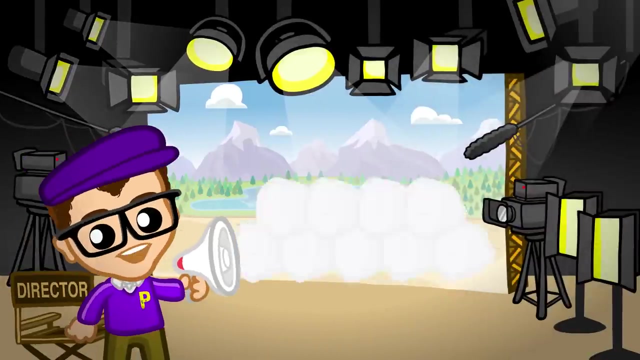 so ten minus nine equals one right, and ten minus one equals nine right. twelve minus five equals nine right. twelve minus five equals seven. twelve minus five equals seven. nine minus one equals eight. nine minus one equals eight. eleven minus ten equals one. equals 1.. 9 minus 7. 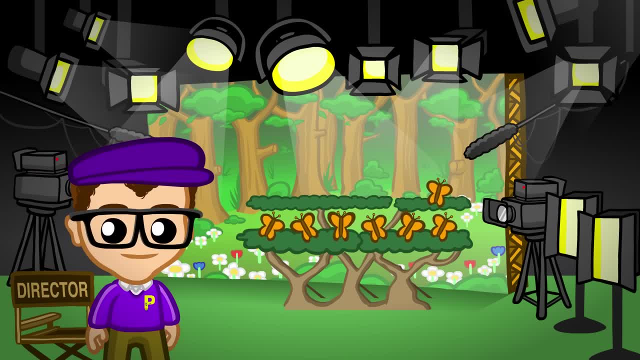 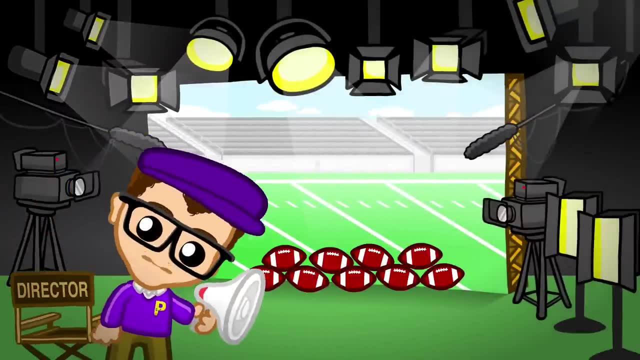 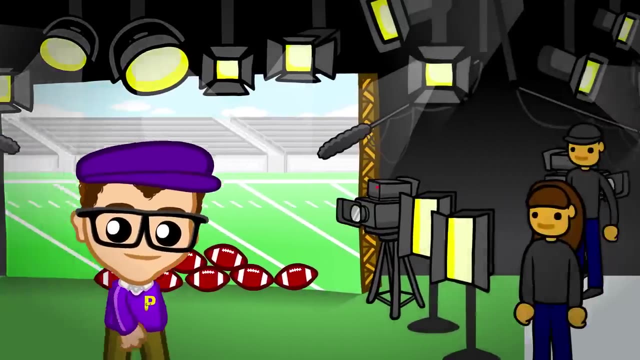 7! 9 Minus 1- Equals 7! 9 Minus 1 Equals 7! 9 Minus 1. 9 Minus 1- Equals 8, 9 Minus 1. 11 Minus 10. 11 Minus 10. 12 Minus 10: 10 9-7 equals 2. 10-3 equals 7. 11-7 equals 4. 9-6 equals 3. 12-2 equals 10- 11-5. 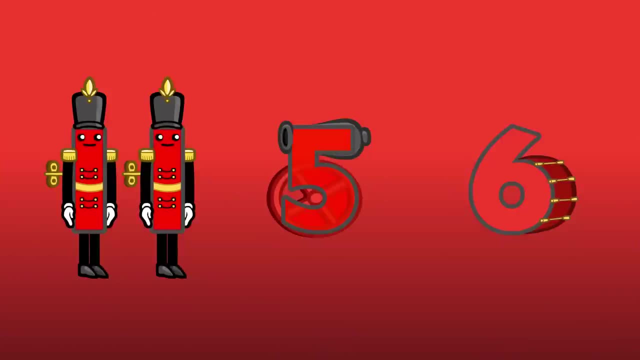 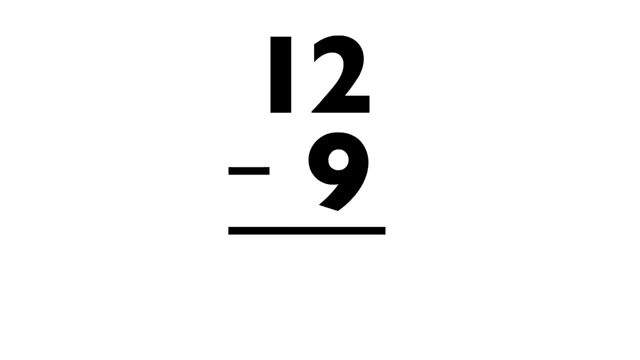 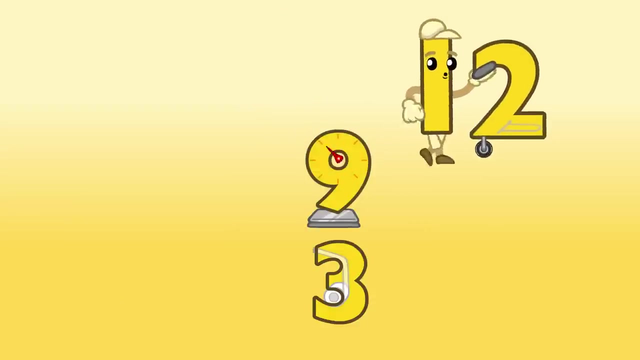 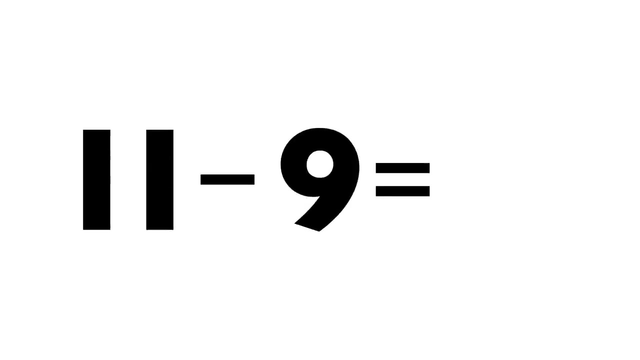 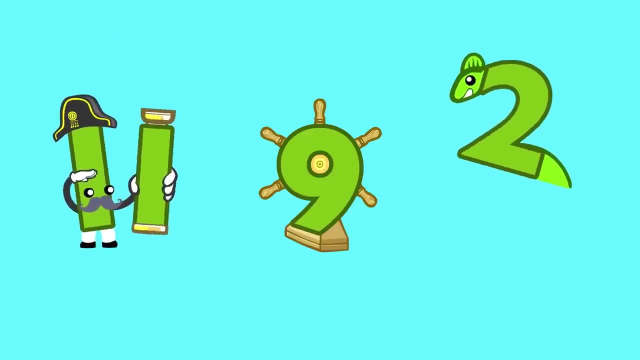 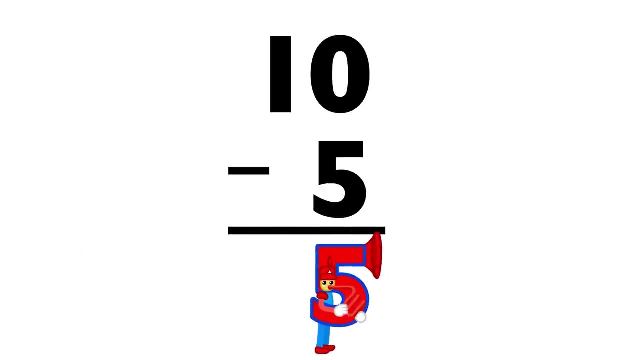 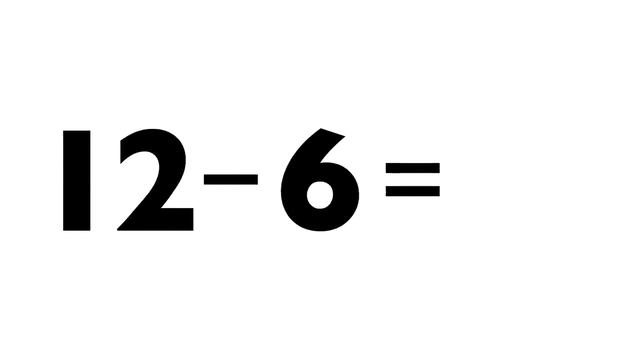 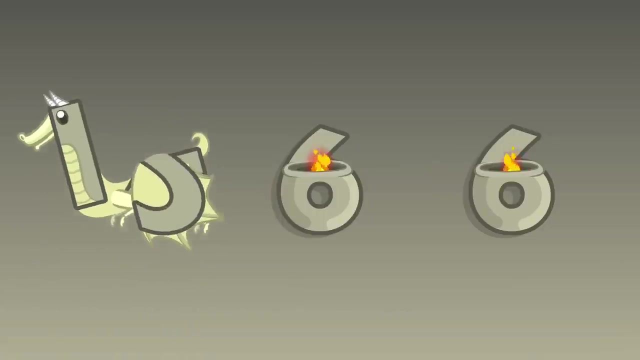 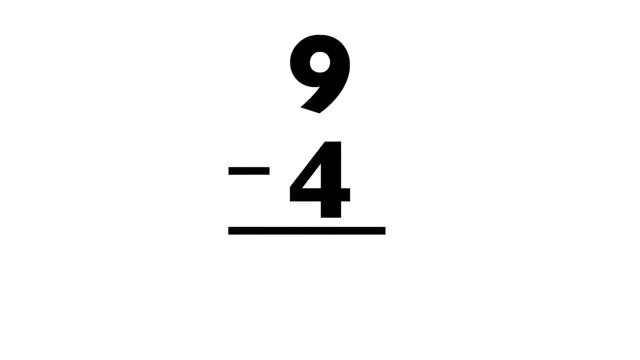 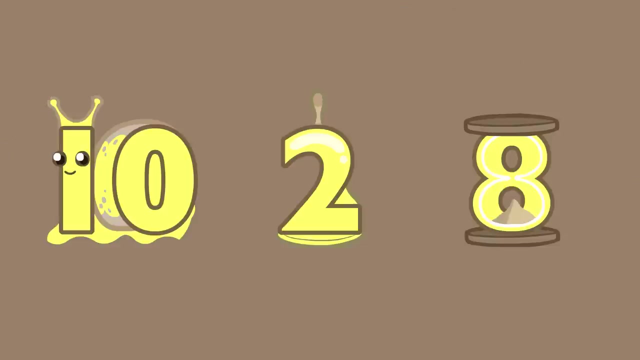 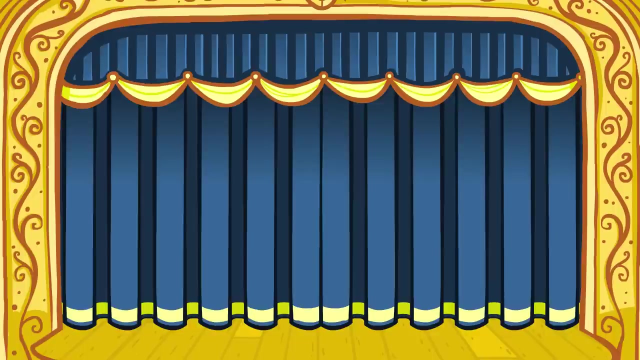 equals 6- 12-9, equals 3 11-9 equals 2. 10-5, equals 5. 12-3 minus 6 equals 6. 9-4 equals 5 10-2, equals 8 20-1. 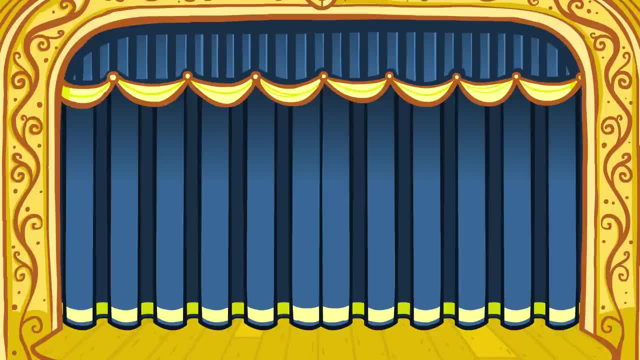 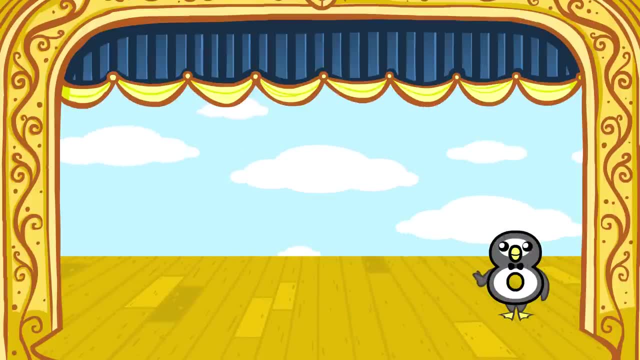 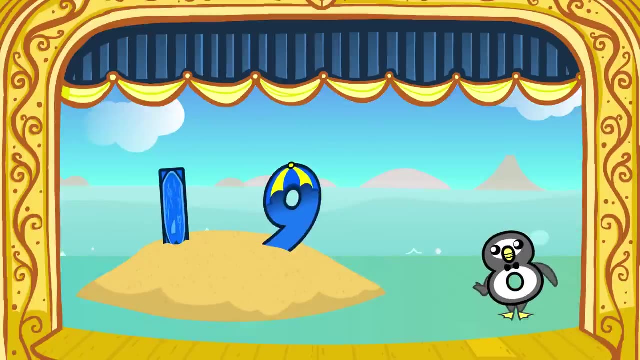 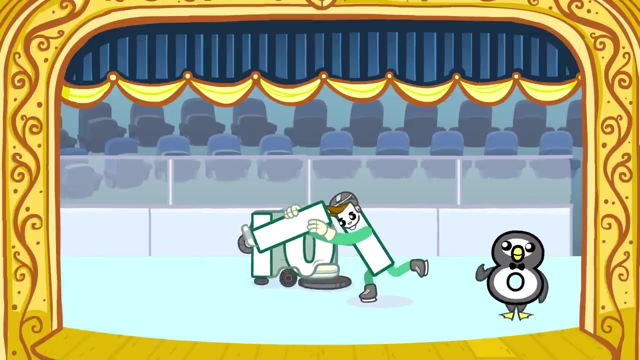 gets inside the box. Ladies and gentlemen, please give a round of applause to Meet the Math Facts. Math Facts- Math Facts: 1 plus 8 equals 9. 1 plus 9 equals 10. 1 plus 10 equals 11. 1 plus 10 equals 11. 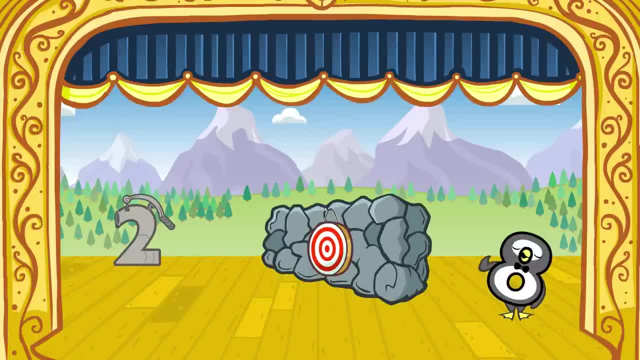 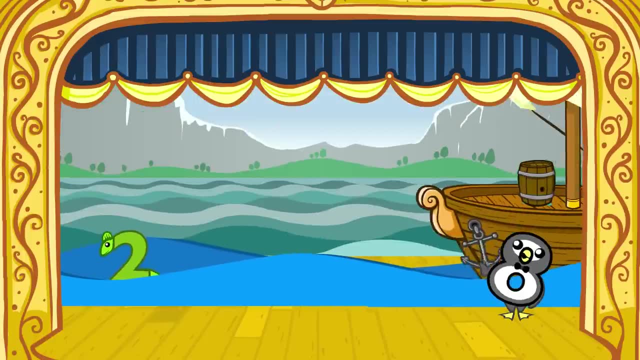 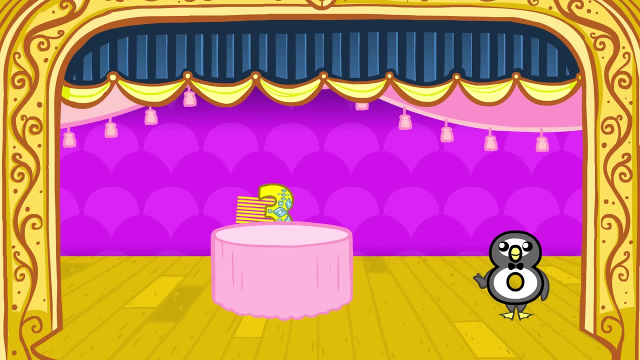 1 plus 10 equals 11. 2 plus 7 equals 9. 2 plus 8 equals 10. 2 plus 9 equals 11. 2 plus 10 equals 12. 3 plus 6 equals 9. 3 plus 7: equals 10. 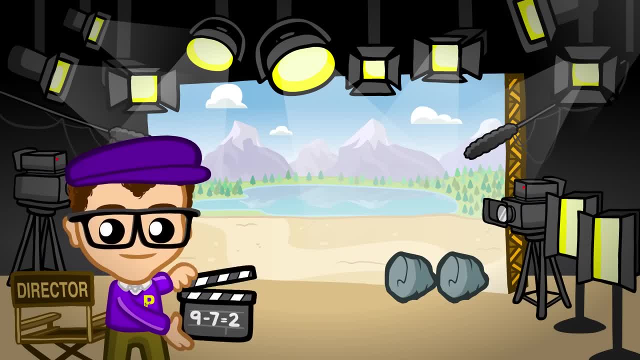 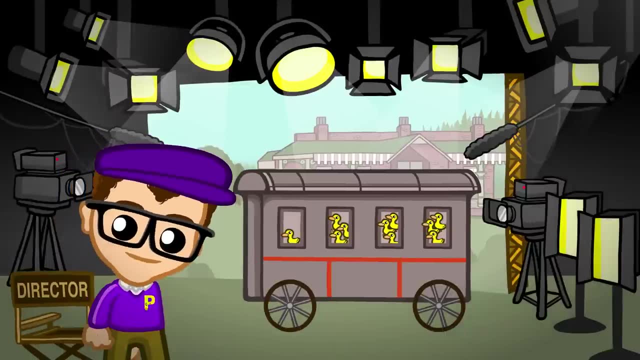 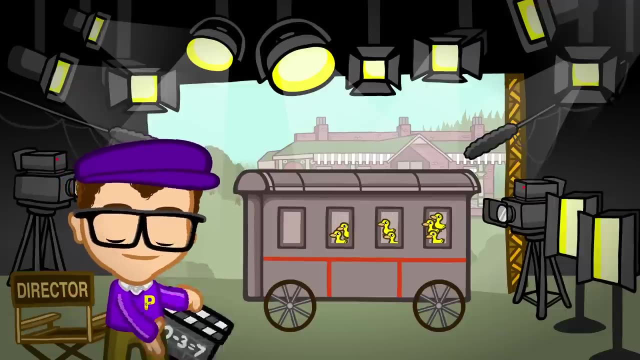 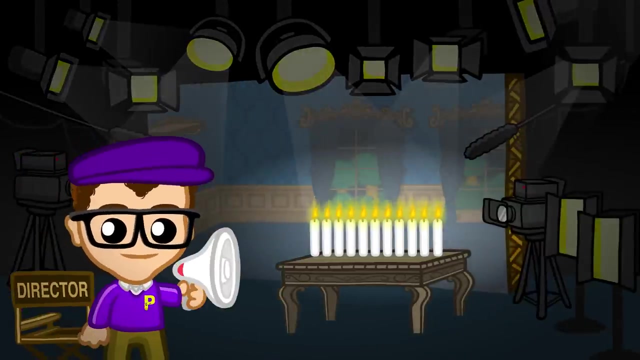 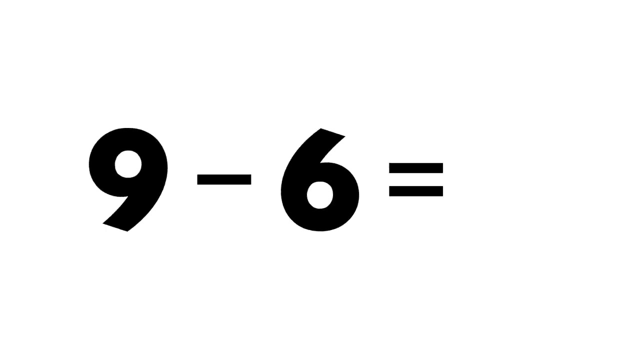 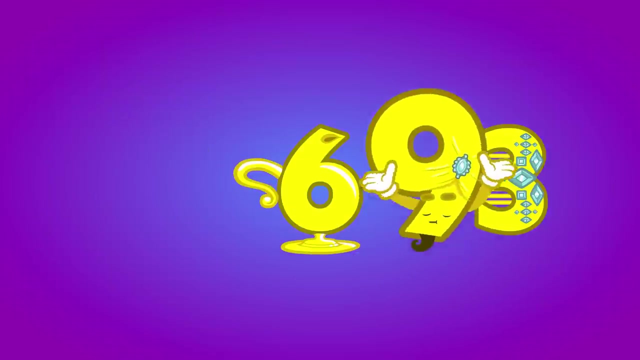 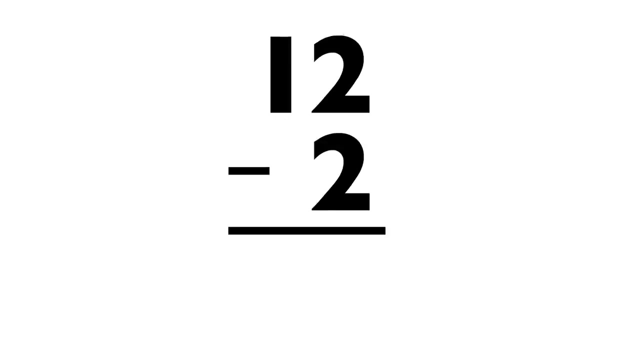 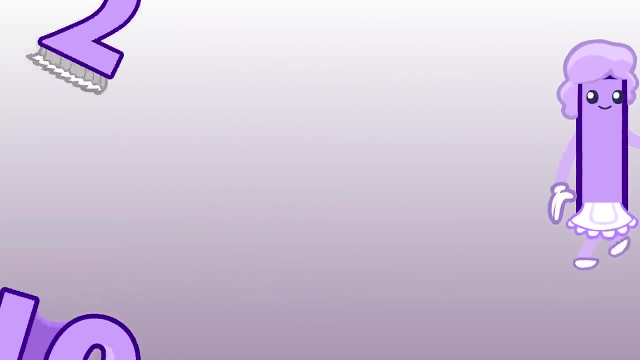 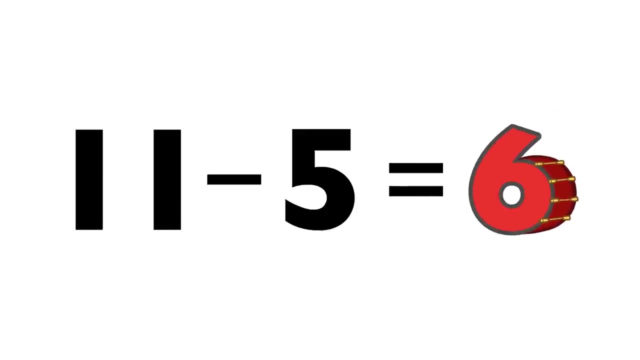 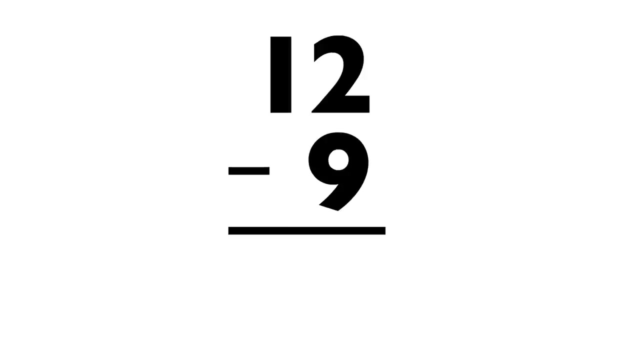 equals 2. 10 minus 3- equals 7.. 11 minus 7- equals. 4.. 9 minus 6- equals 3.. 12 minus 2 equals 10. 11 minus 5: equals 6. 12 minus 9. 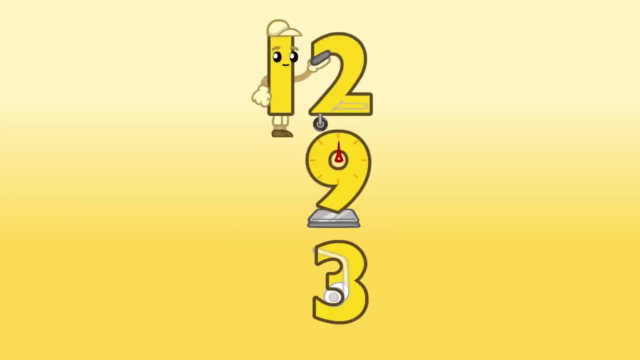 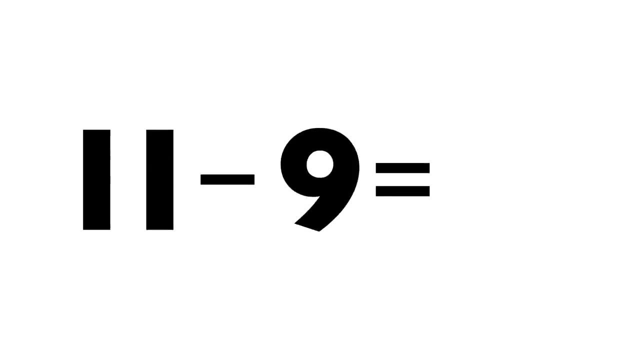 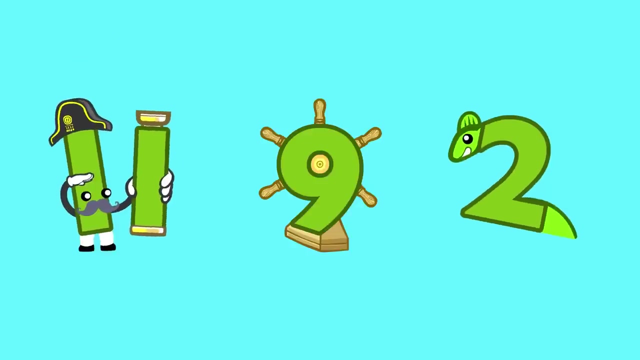 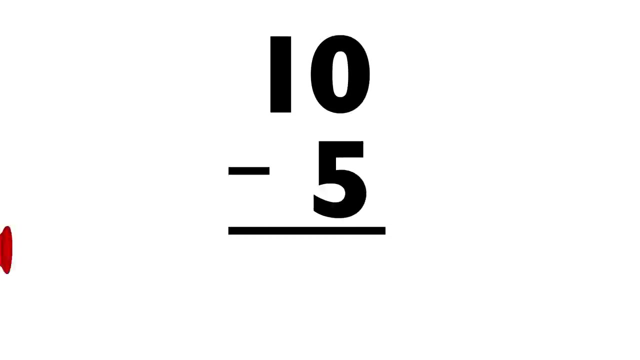 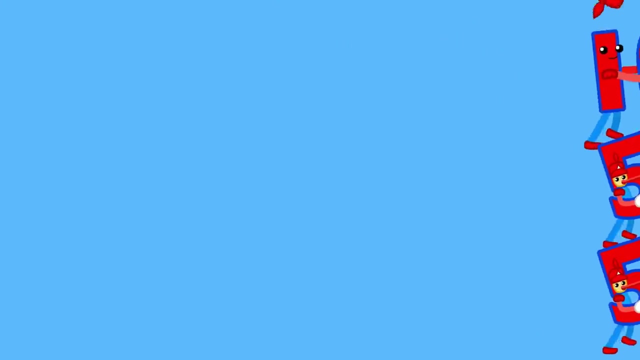 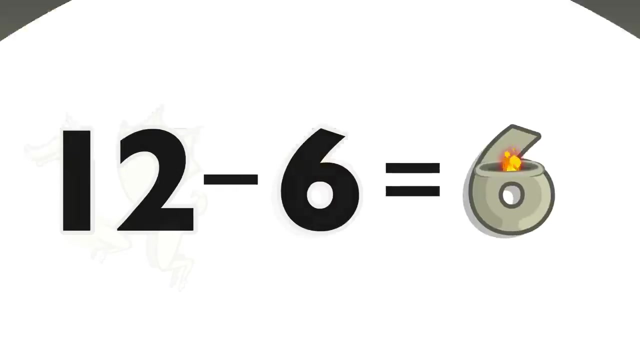 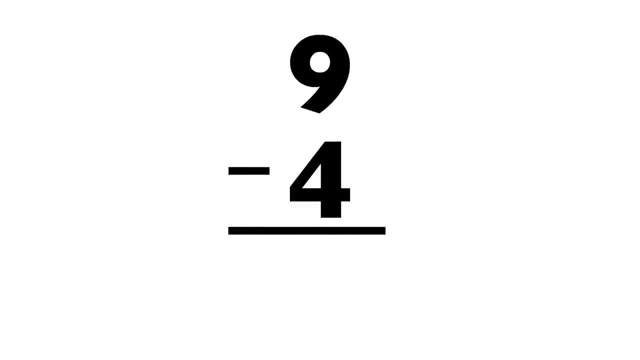 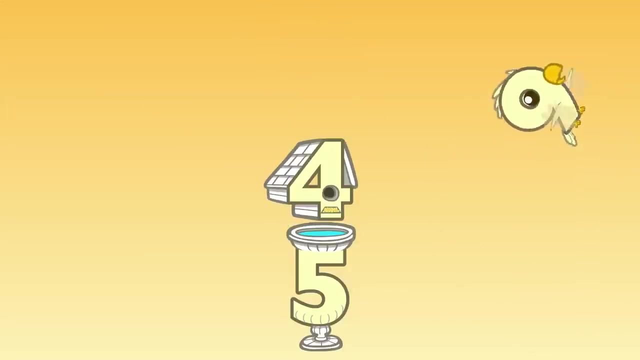 equals 6. 12 minus 9: equals. 6. 11 minus 9 equals. 3.. 10 minus 5 equals. 5.. 12 minus 6 equals. 6. 9 minus 4: equals. 5. 10 minus 2. 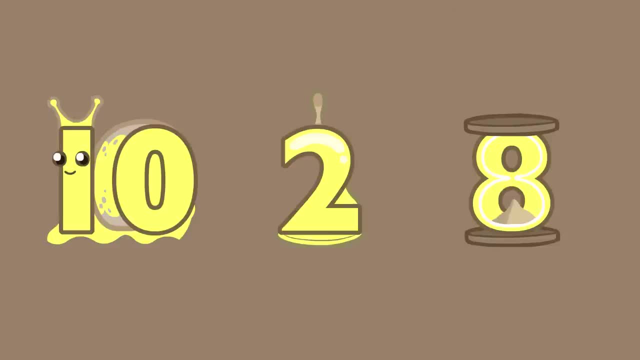 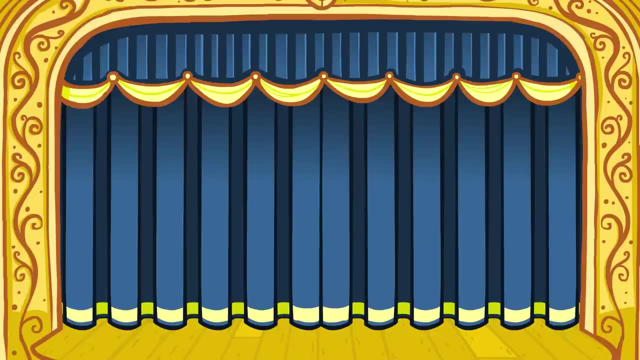 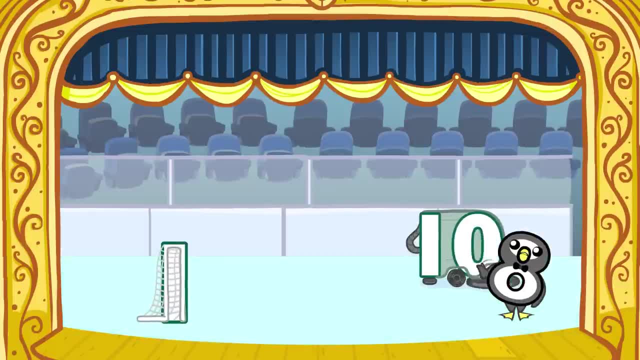 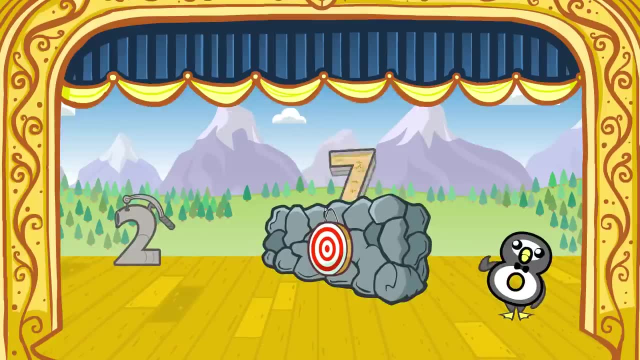 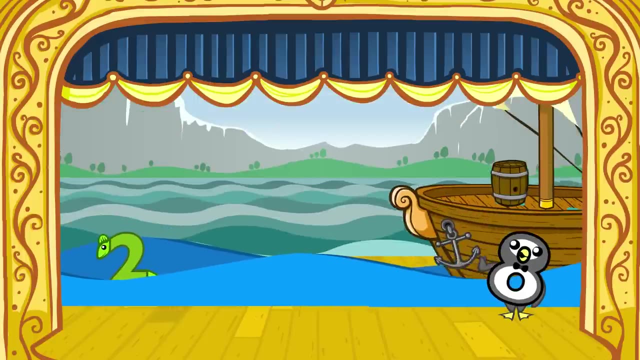 equals 8.. 10 minus 7 equals 8.. 10 minus 7: 10 equals 11.. 2 plus 7 equals 9.. 2 plus 8 equals 10.. 2 plus 9 equals 11.. 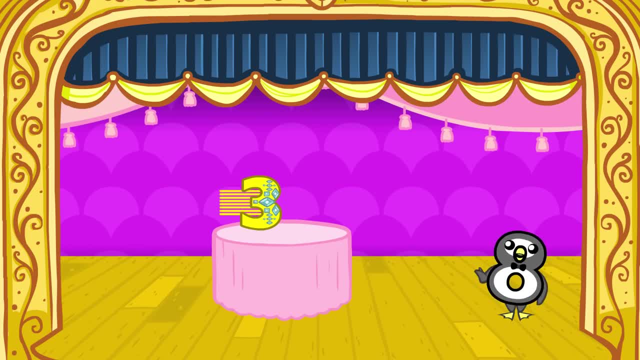 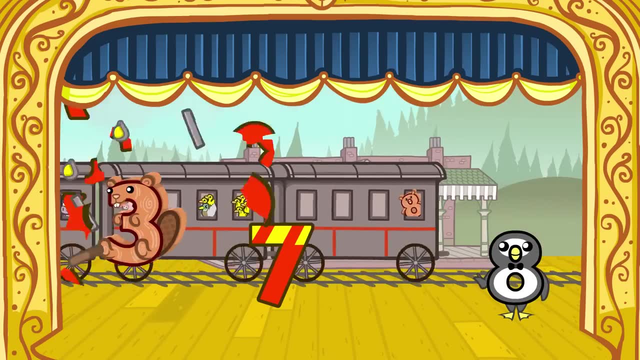 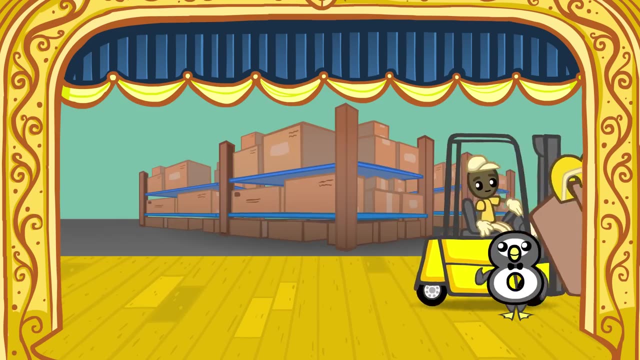 2 plus 10 equals 12.. 3 plus 6 equals 9.. 3 plus 7 equals 10.. 3 plus 8 equals 11.. 3 plus 9 equals 12.. 4 plus 5 equals 9.. 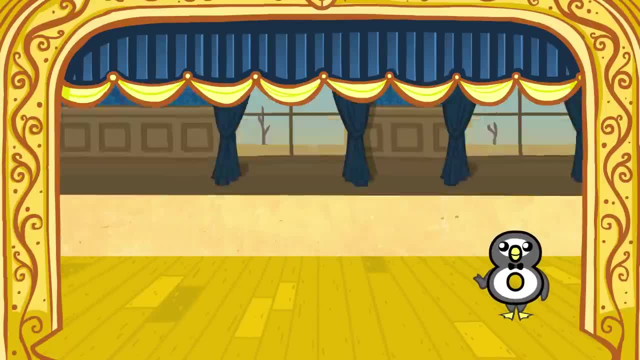 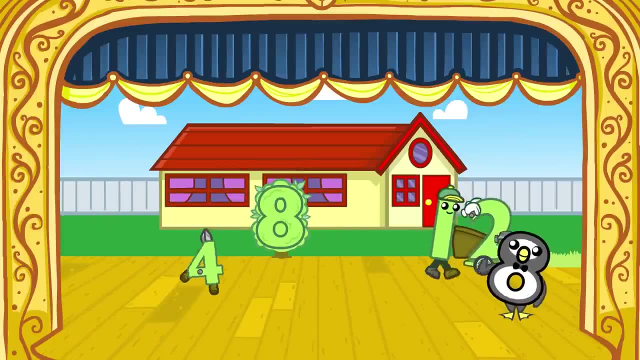 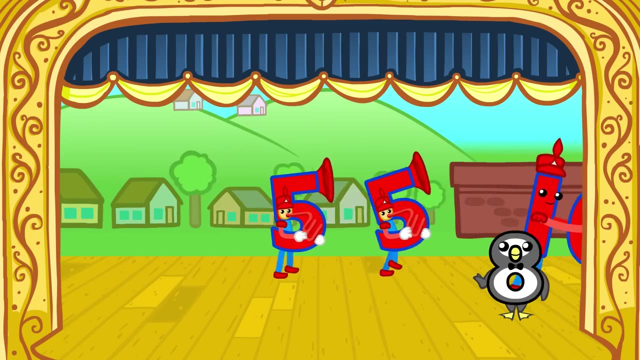 4 plus 6 equals 10.. 4 plus 7 equals 11.. 4 plus 8 equals 12.. 5 plus 4 equals 9.. 5 plus 5 equals 10.. 5 plus 6 equals 11.. 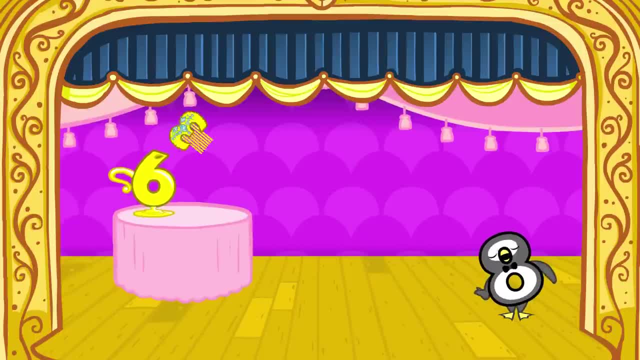 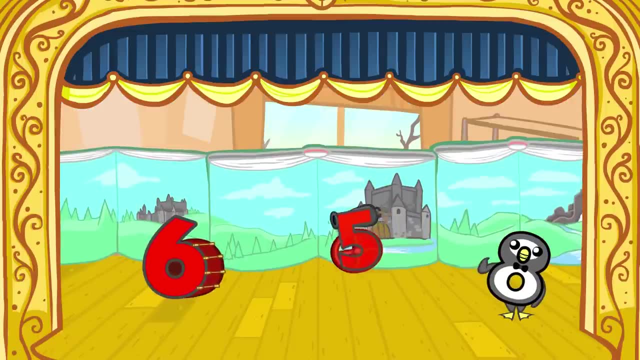 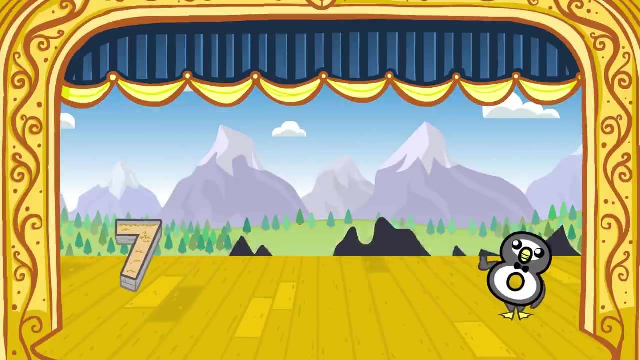 5 plus 7 equals 12.. 6 plus 3 equals 9.. 6 plus 4 equals 10.. 6 plus 5 equals 11.. 6 plus 6 equals 12.. 7 plus 2 equals 9.. 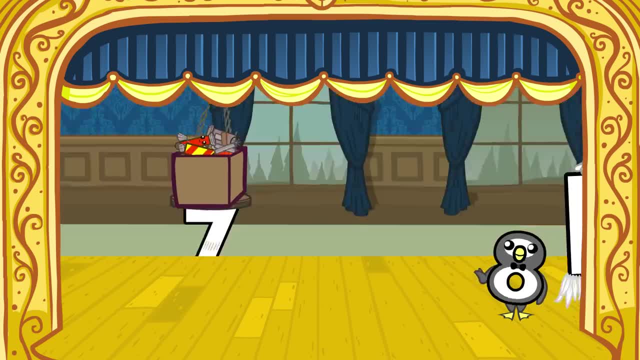 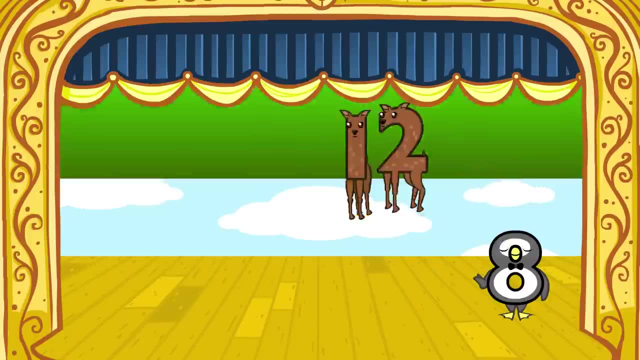 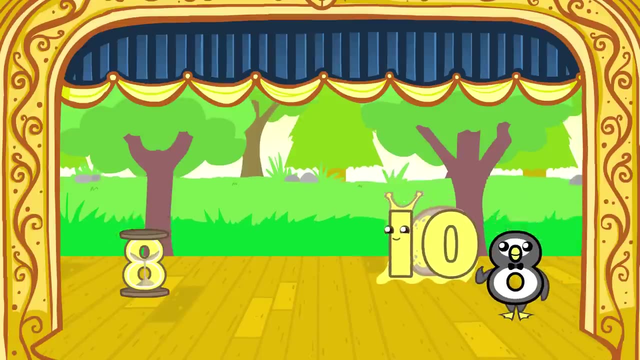 7 plus 3 equals 10.. 7 plus 4 equals 11.. 7 plus 5 equals 12.. 8 plus 1 equals 9.. 8 plus 2 equals 10.. 8 plus 3 equals 11.. 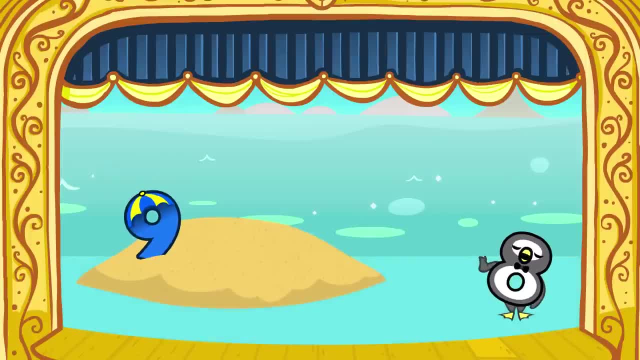 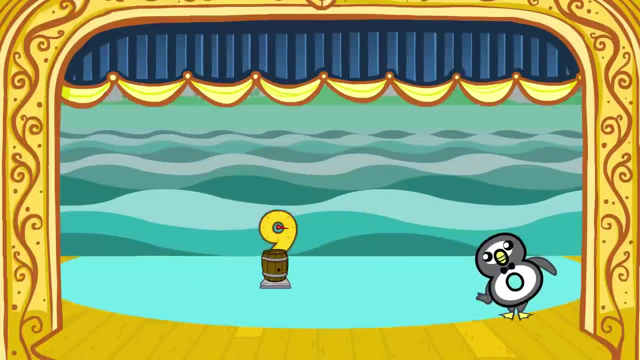 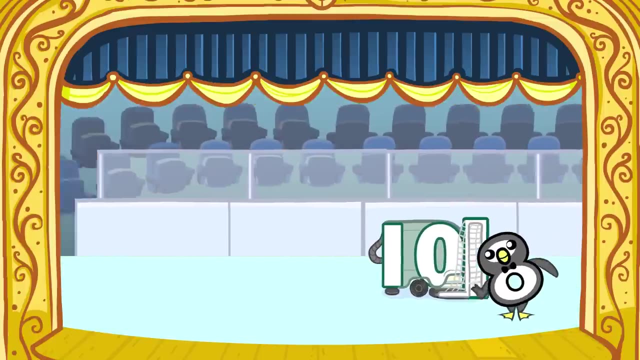 8 plus 4 equals 12.. 9 plus 1 equals 10.. 9 plus 2 equals 11.. 9 plus 3 equals 12.. 10 plus 1 equals 11.. 10 plus 2 equals 12.. 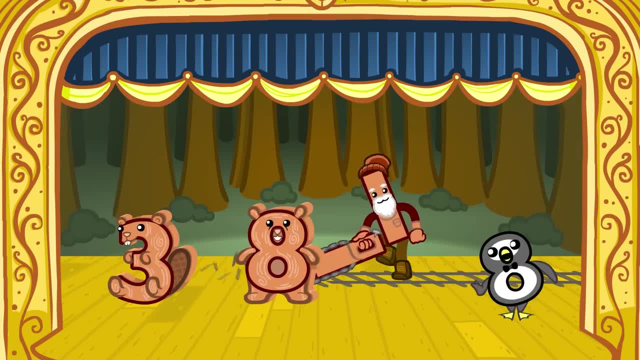 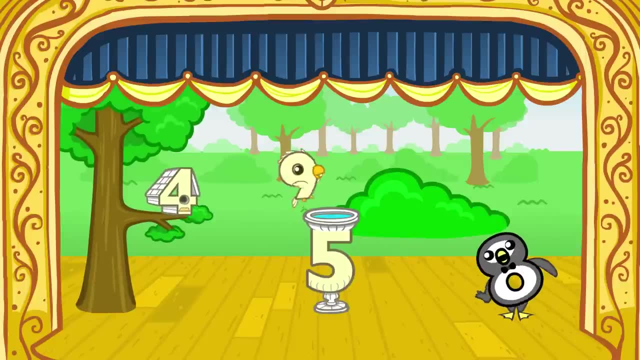 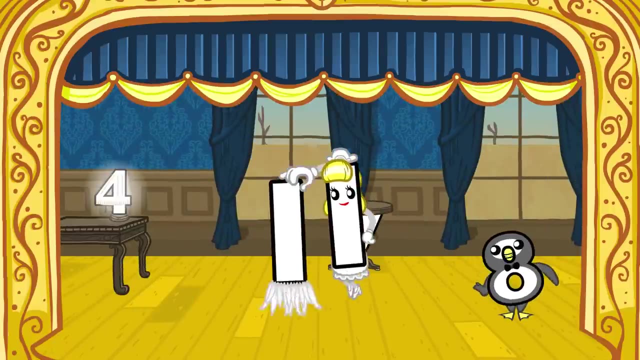 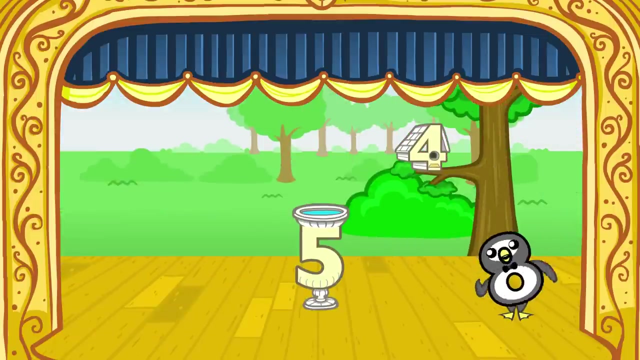 3 plus 8: equals 11. 3 plus 9: equals 12. 4 plus 5 equals 9. 4 plus 6 equals 10. 4 plus 7 equals 11. 4 plus 8: equals 12. 5 plus 4: equals 9. 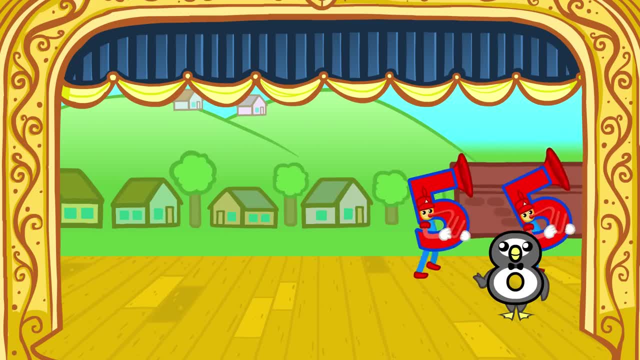 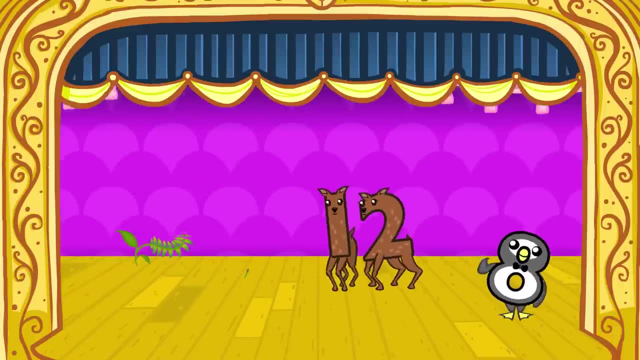 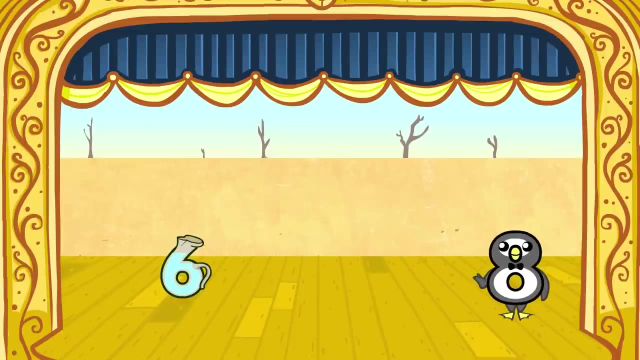 5 plus 5 equals 10. 5 plus 6 equals 11. 11. 11 5 plus 7 equals 12. 6 plus 3 equals 9. 6 plus 4 equals 10. 6 plus 5 equals 11. 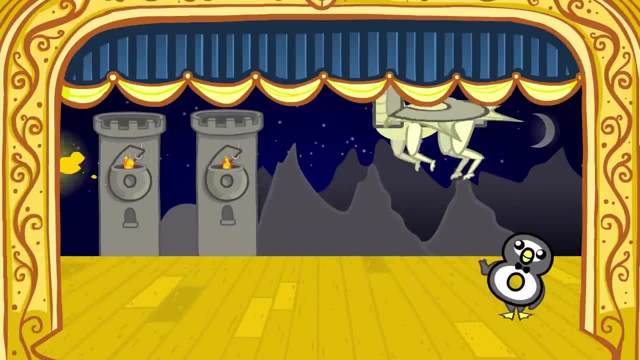 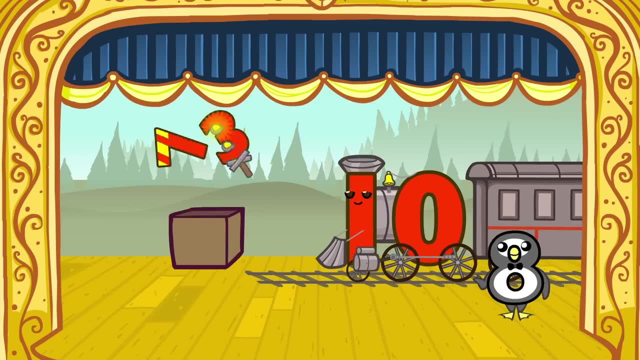 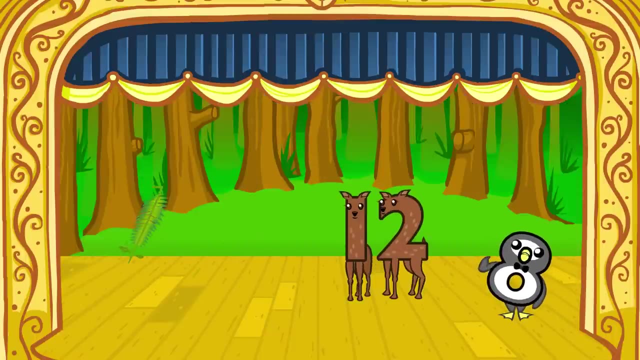 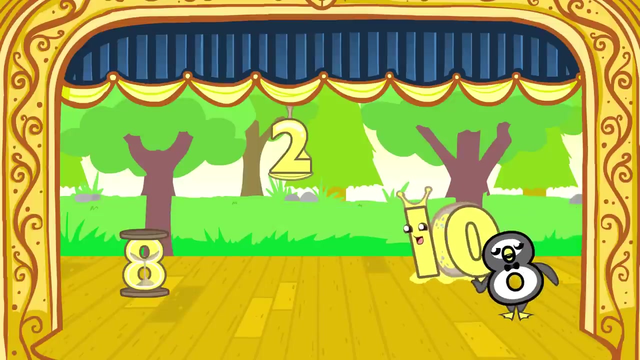 6 plus 6 equals 12. 7 plus 2 equals 9. 7 plus 3 equals 10. 7 plus 4 equals 11. 7 plus 5 equals 12. 8 plus 1 equals 9. 8 plus 2 equals 10. 8 plus 3 equals 11. 8 plus 4 equals 12. 9 plus 1 equals 10. 9 plus 2 equals 11. 9 plus 3 equals 12. 10 plus 1 equals 11. 10 plus 2 equals 12. 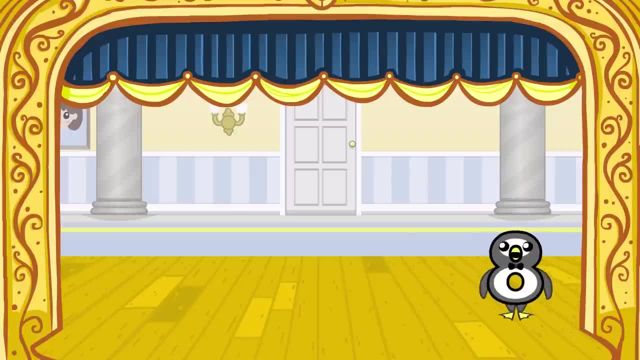 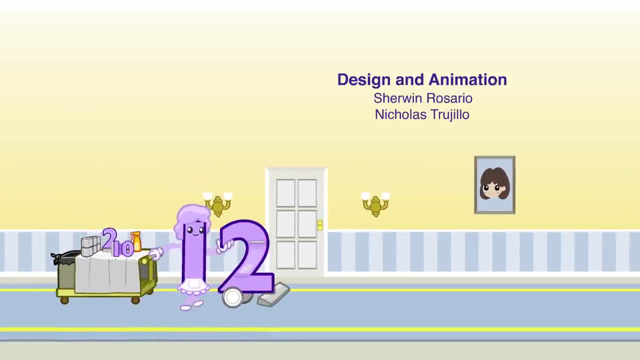 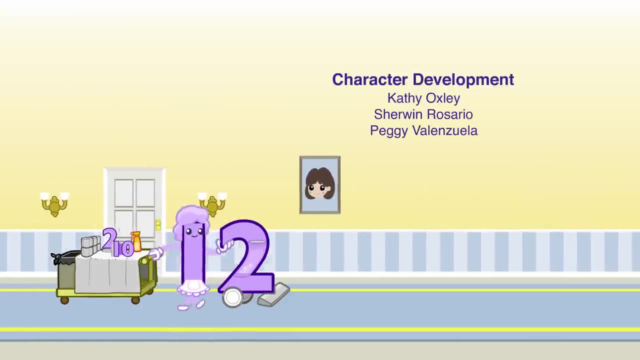 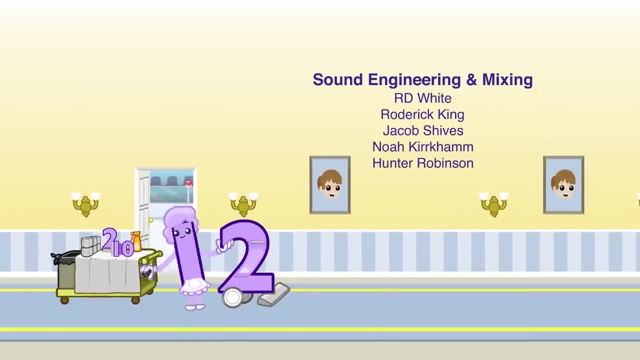 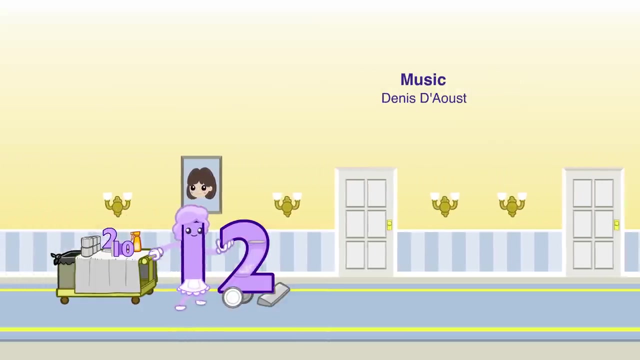 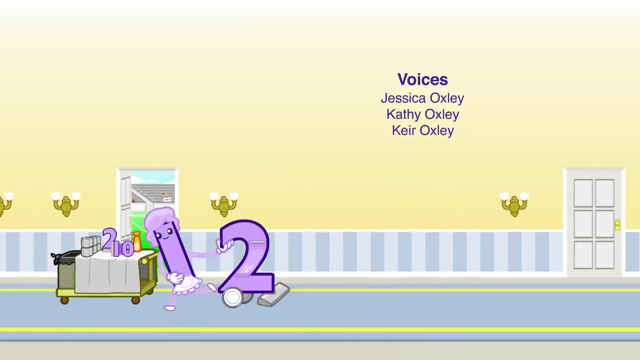 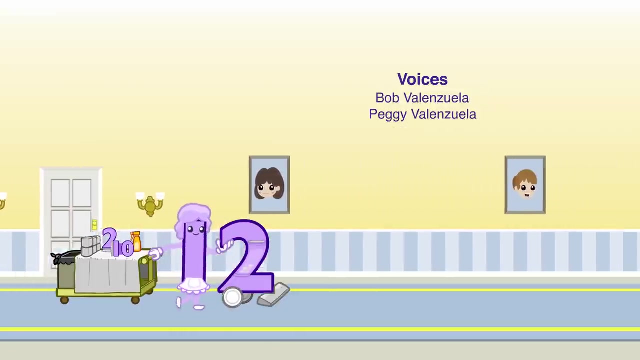 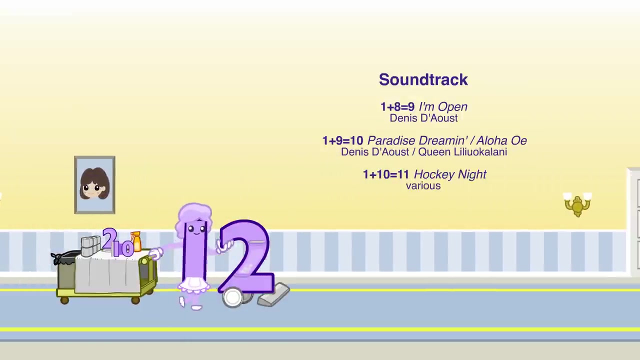 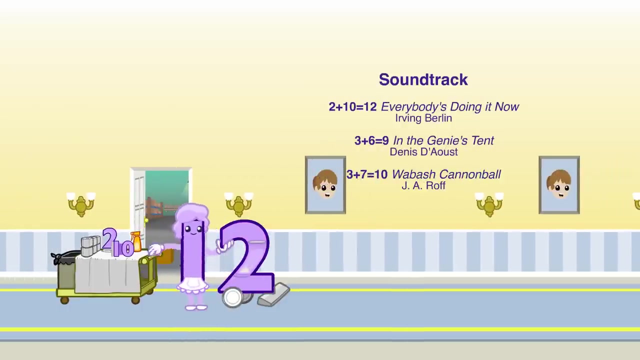 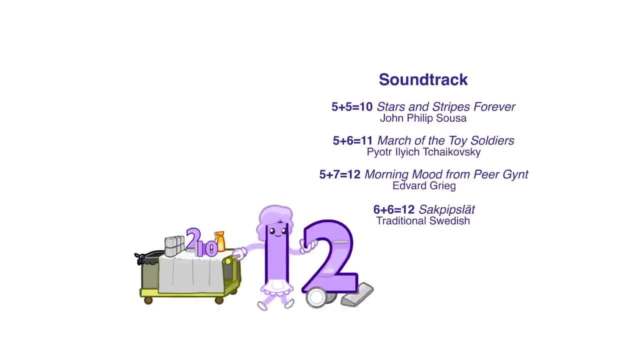 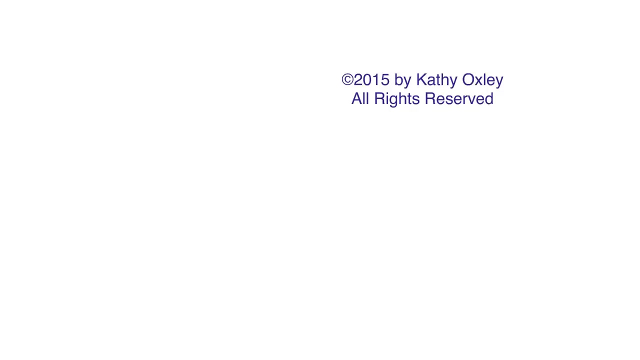